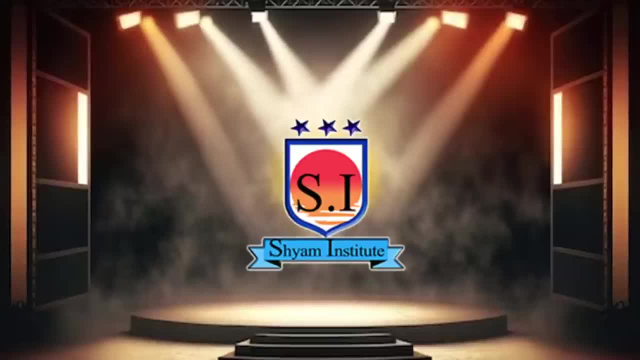 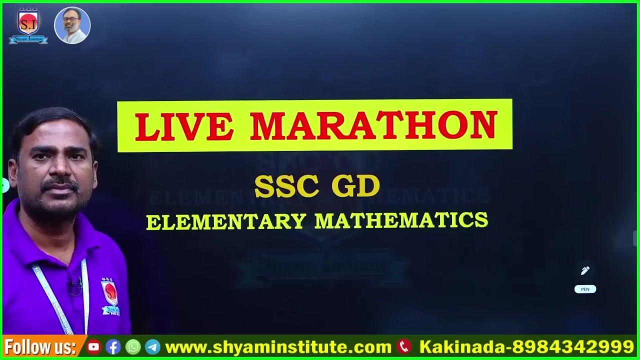 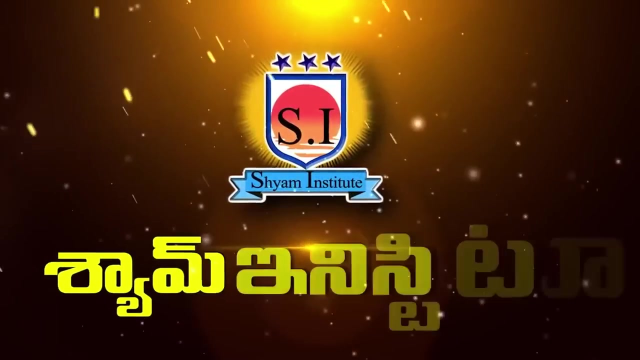 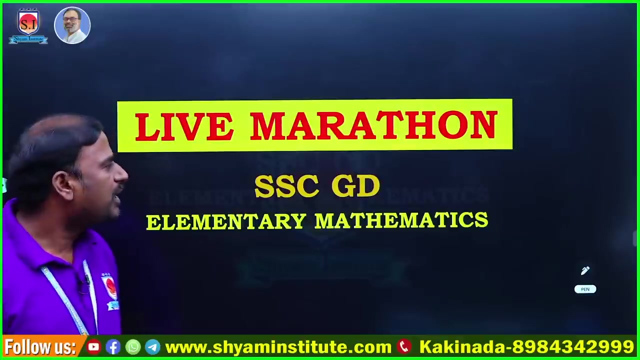 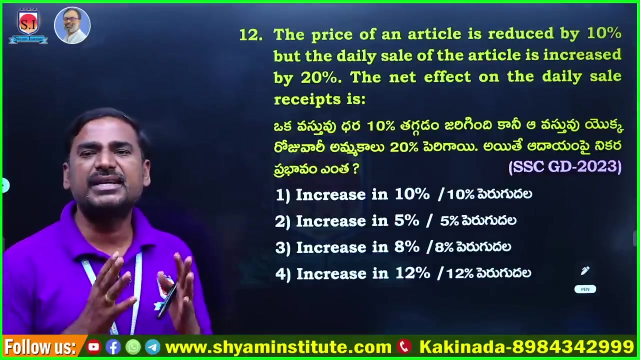 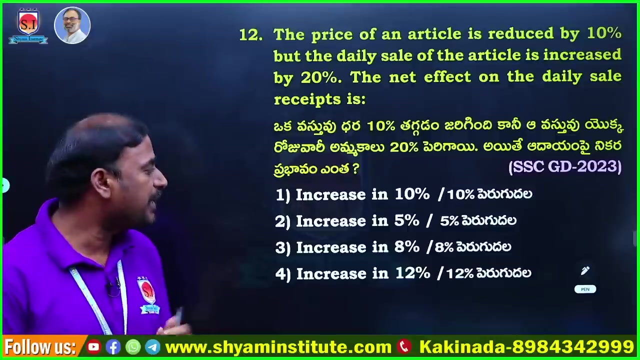 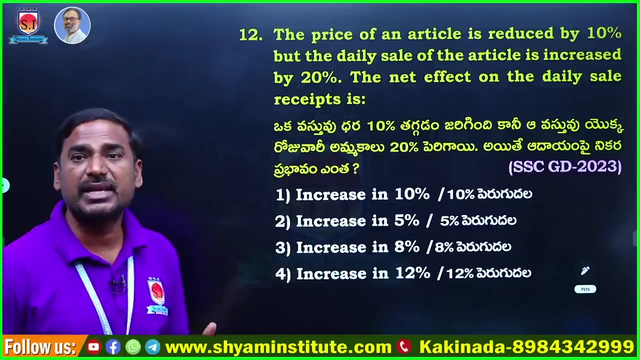 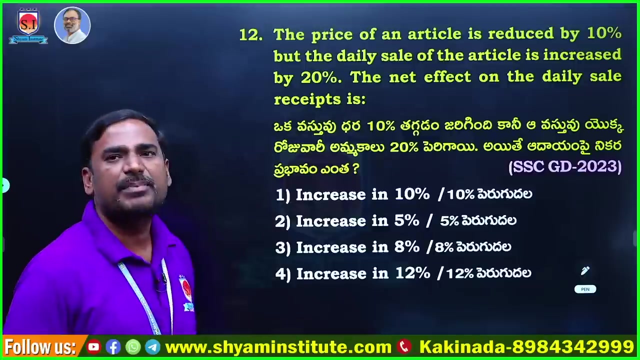 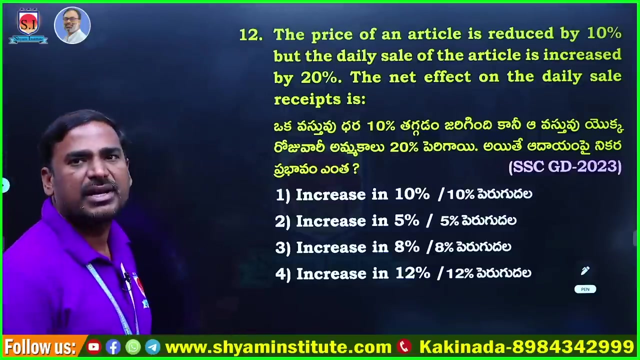 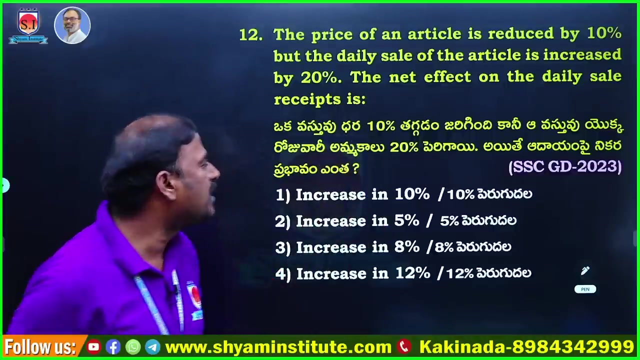 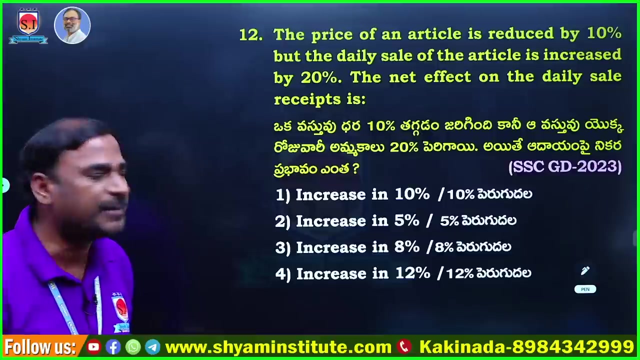 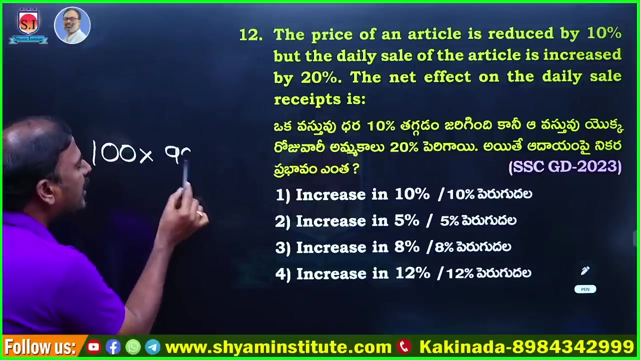 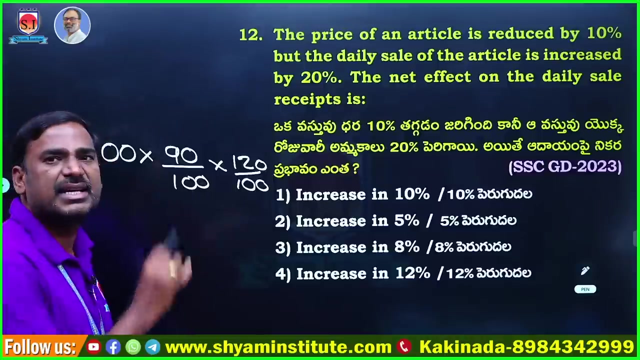 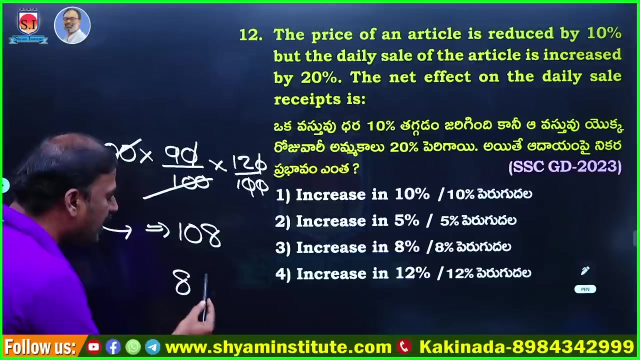 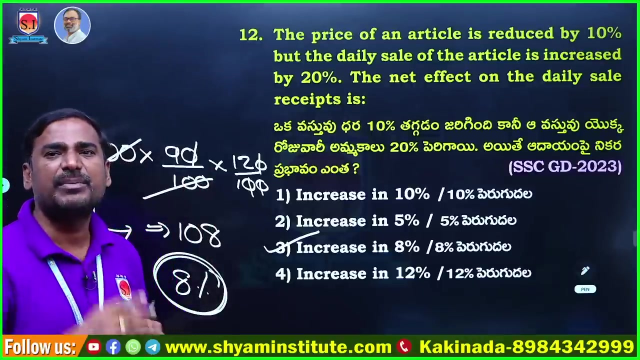 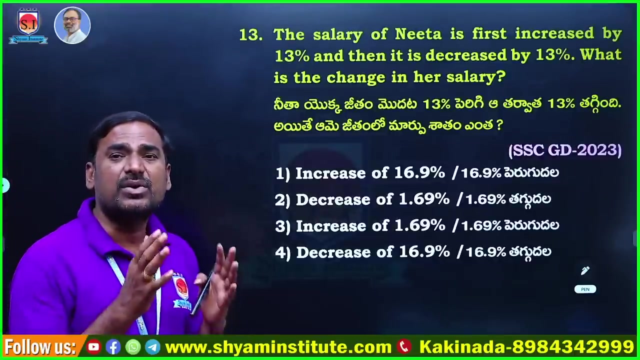 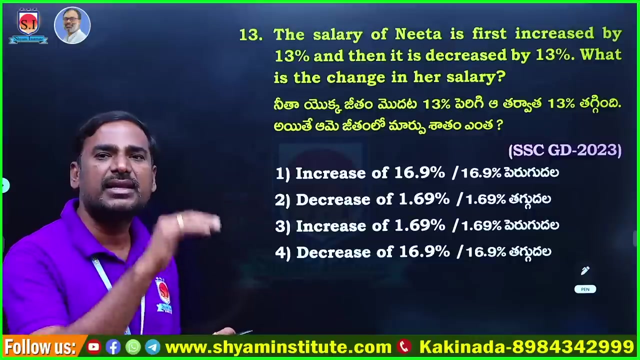 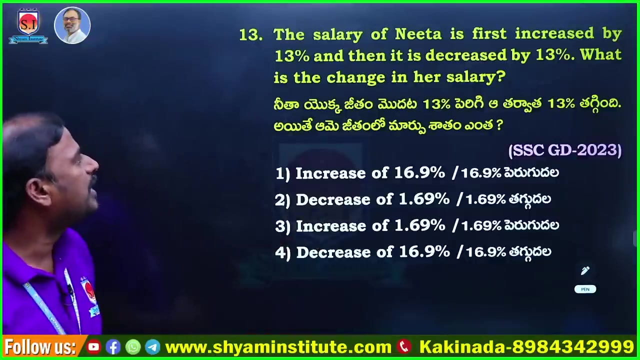 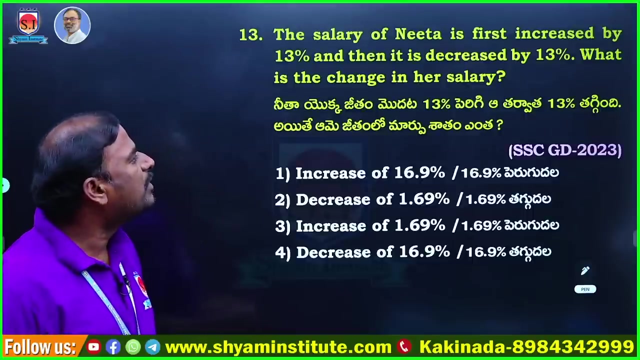 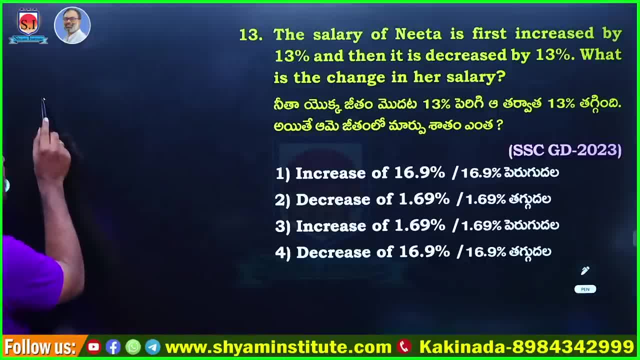 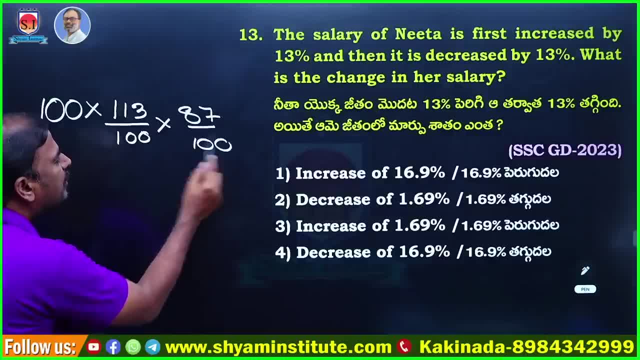 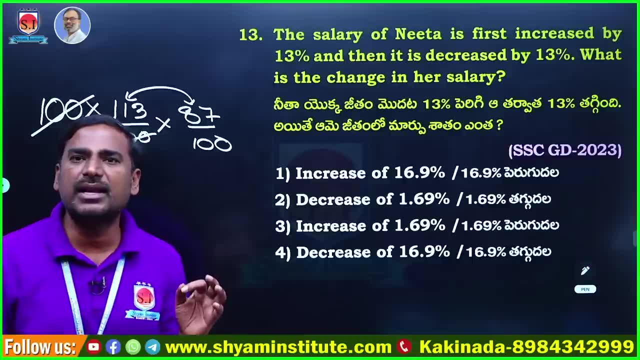 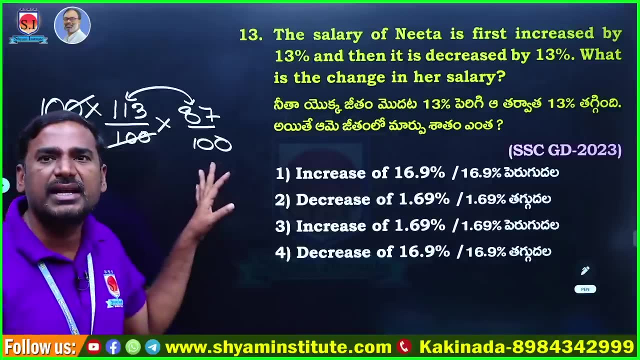 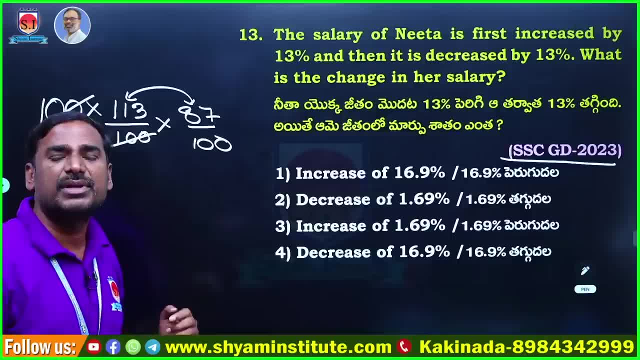 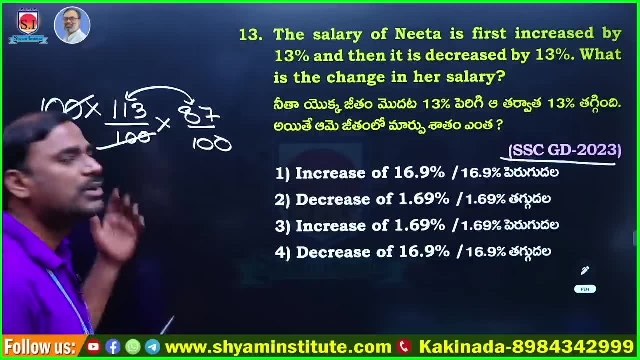 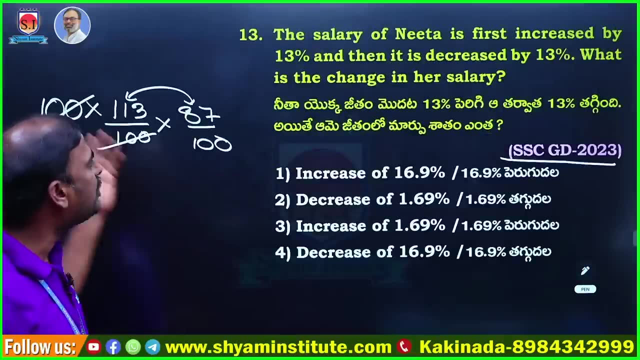 What are your last name? Is it Anwaar? Well finished, My name is Anwar. If the numbers are difficult to do by the chain method, then you go for the formula method. Let's see the formula method carefully. Here the salary increases by 13% and decreases by 13%. 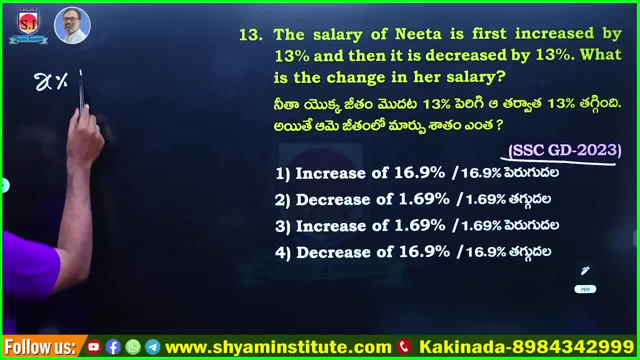 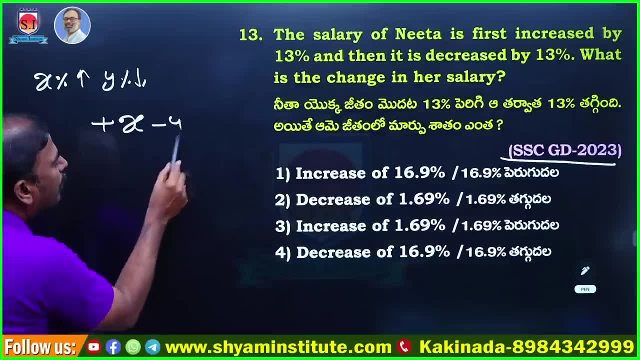 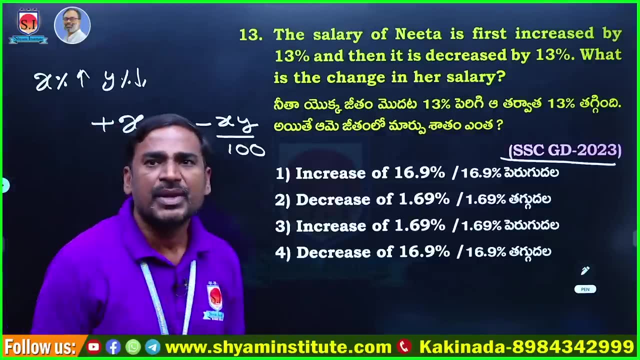 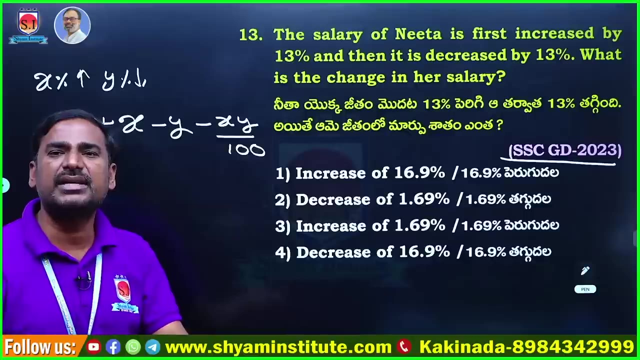 Whenever x% increases and y% decreases, the formula we have to take is plus x minus y, plus into minus minus xy by 100. The concept given here is first time increased by x% and later decreased by y% overall. If we apply this concept, it is very simple. 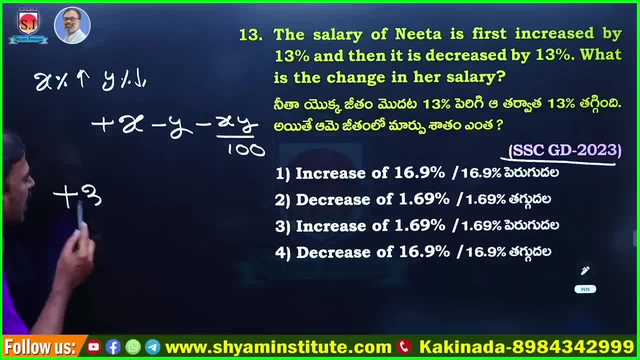 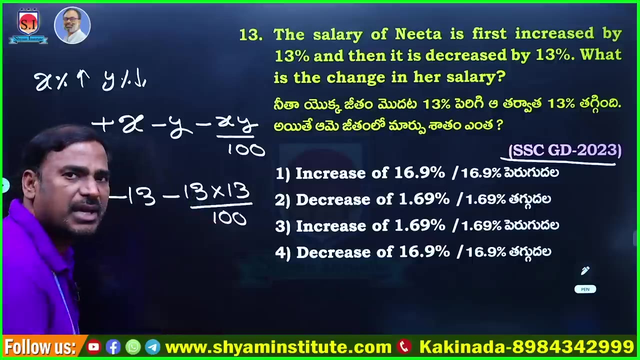 First, I took the salary increased by 13 and plus 13.. Next, I took the salary decreased by 13 and minus 13.. Since it is plus into minus minus 13 x 13 by 100.. 13 increased by 13,, 13 decreased by 13, and plus into minus minus 13 x 13 by 100. 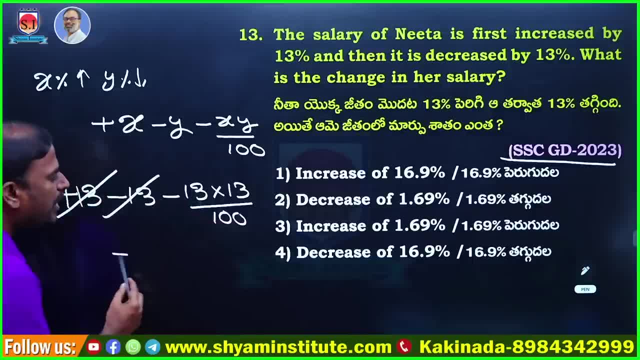 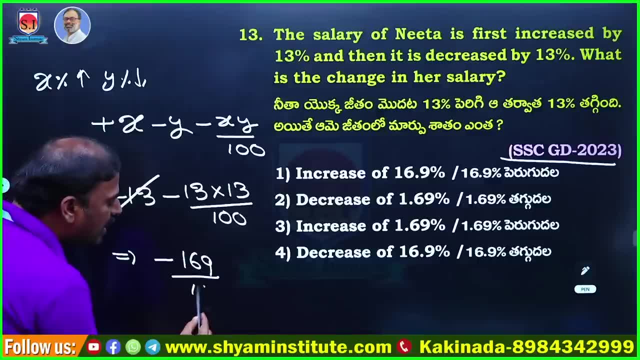 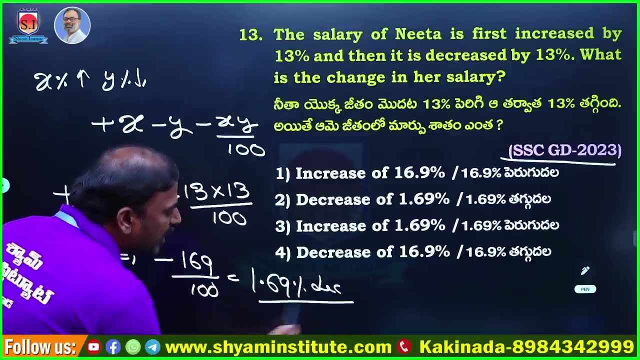 As you can see, 13 x 13 is cancelled. So minus into minus minus 13 is cancelled. We can write it as 1313169 by 100 and we can also write it as 1.69, which is a decrease. 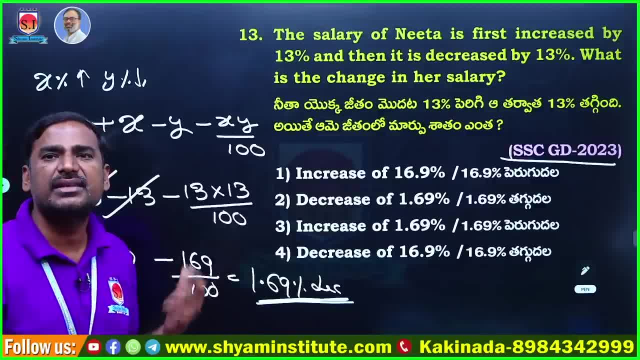 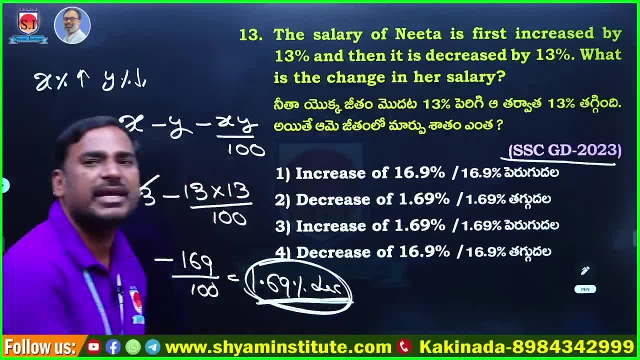 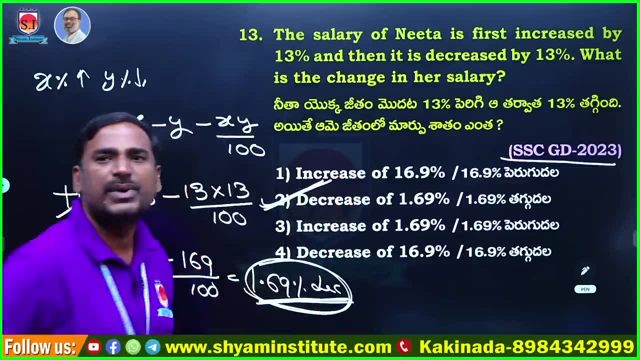 Why do we write it as a decrease? Because when it is negative, it should be taken as a decrease and when it is positive, it should be taken as an increase. In general, let us say that the salary of that person is decreased by 1.69%. So since it is option 2, we can take 2 as the correct answer. 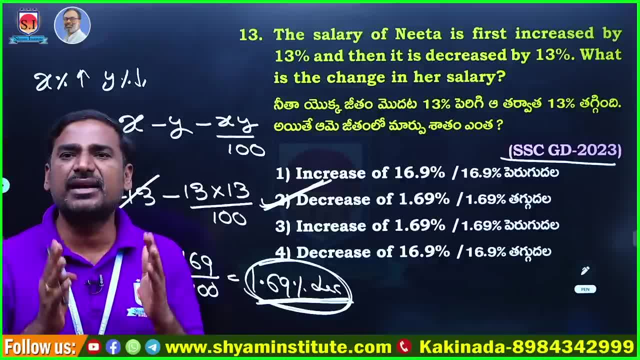 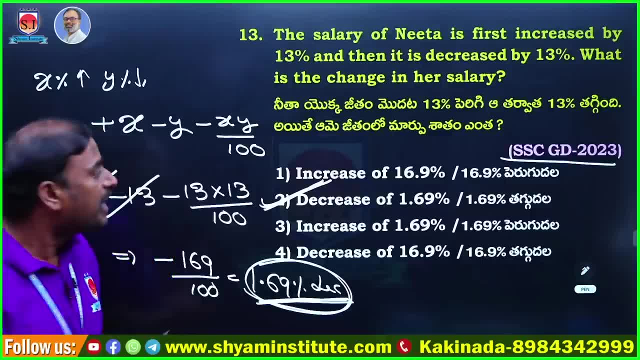 Here you can see that when we have difficulty in multiplication and when we have difficulty in the chain method, it will be easy for us if we do it in this formula method. Another thing is that if these numbers are equal, we can do it even more easily. 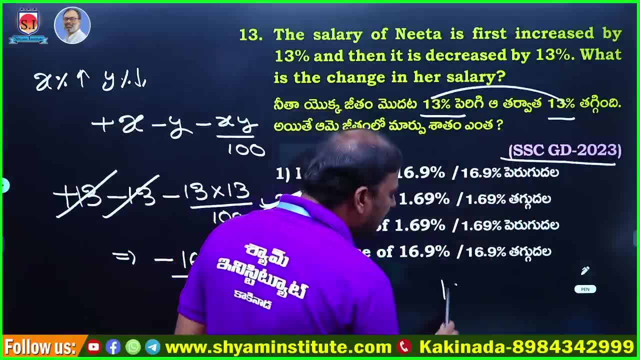 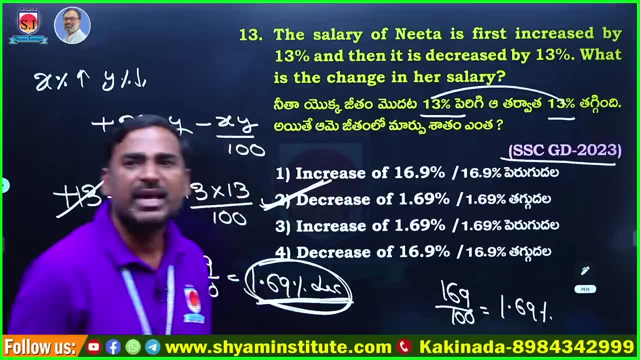 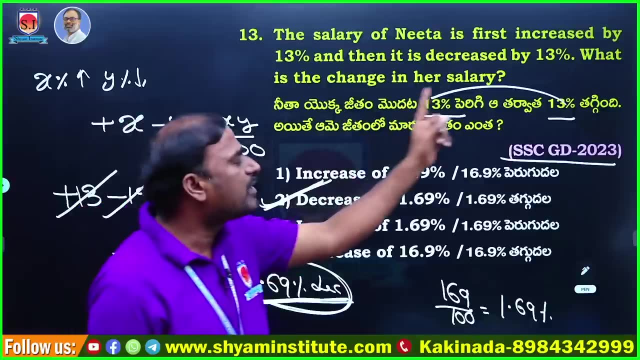 The direct shortcut is 1313169 by 100 and we can always take it as a decrease. If there is an increment and a decrease from the same percentage, we can write 1313169 by 100 as 1.69, which is a decrease. 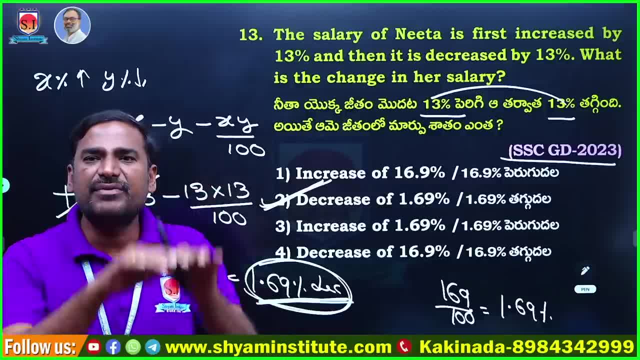 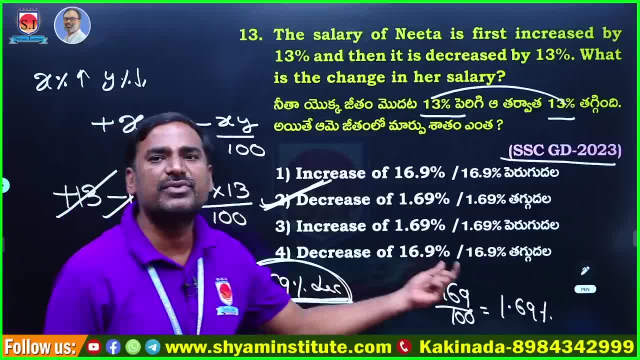 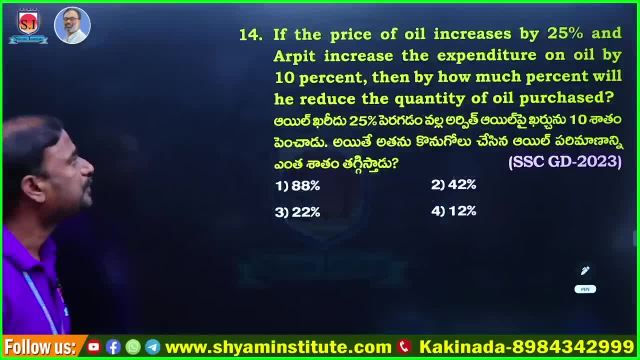 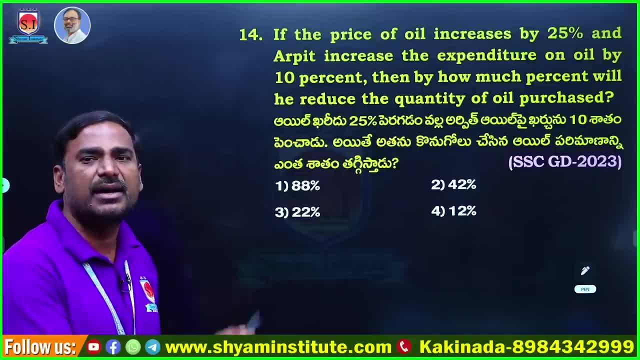 For example, if 15% is increased and 15% is decreased, we can write 1515169 by 100 as 1.69.. Let's see the next question, Question number 14.. Let's see the next question which was asked from SSCGD last year, in 2023. 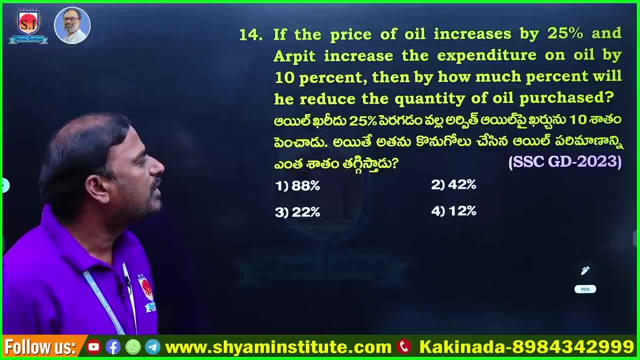 Since the oil price has increased 25%, the share prices have increased 10% on the oil. So how much is the oil of that person's purchase? The price of an oil increased by 25% and RPT increased the expenditure on oil by 10%, then by how much prices will he reduce the quantity of oil purchased? 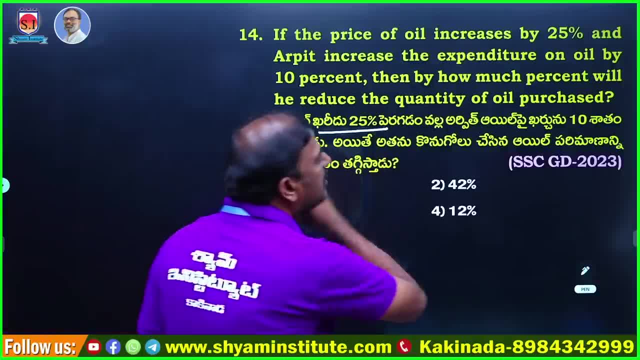 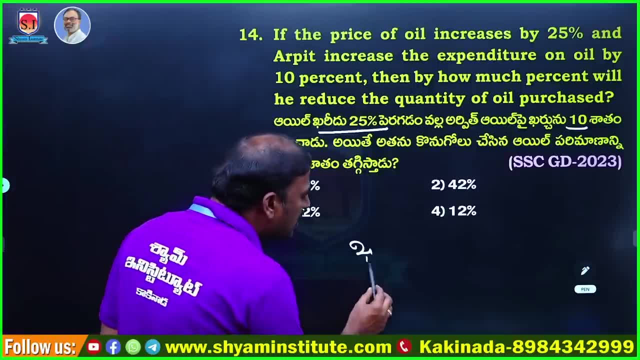 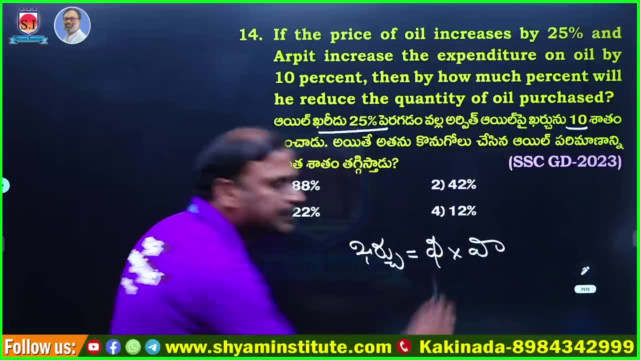 The question is the price of an oil increased by 25% and RPT increased the quantity of oil purchased, So normally the formula for the cost is Dara x Vodakam. These types of examples are frequently asked by the regular customers. 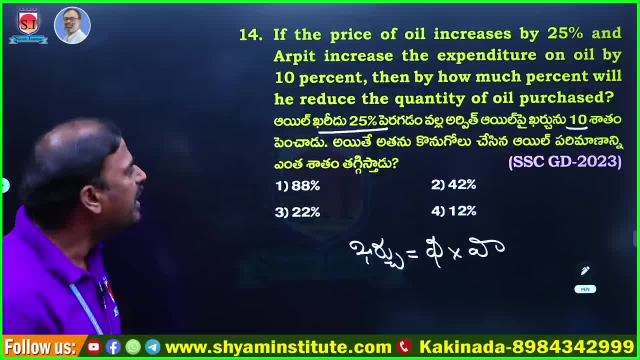 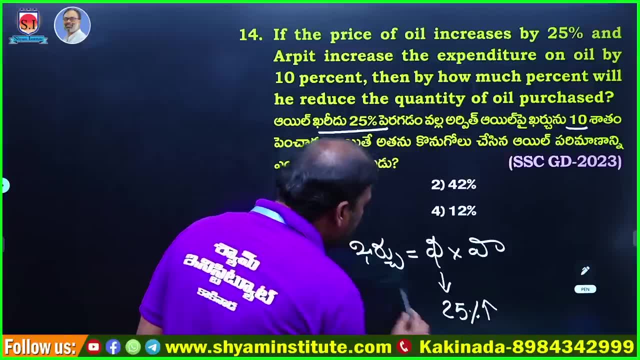 Cost is Dara x Vodakam. What he gave is The price of an oil increased by 25% and RPT increased the quantity of oil purchased. So the price of an oil increased by 10% and RPT increased the quantity of oil purchased. 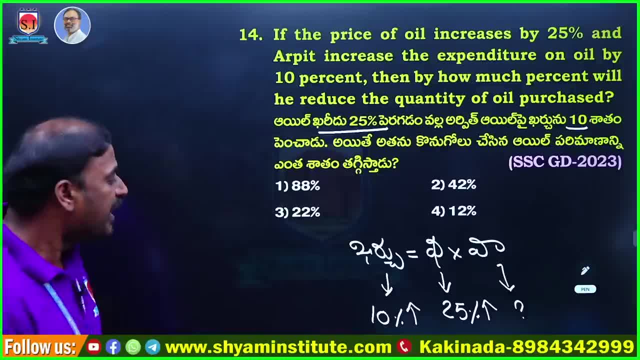 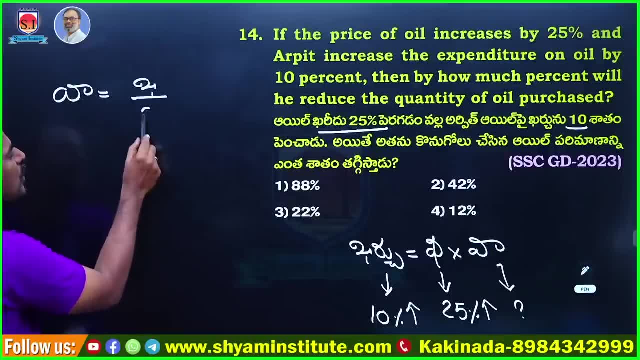 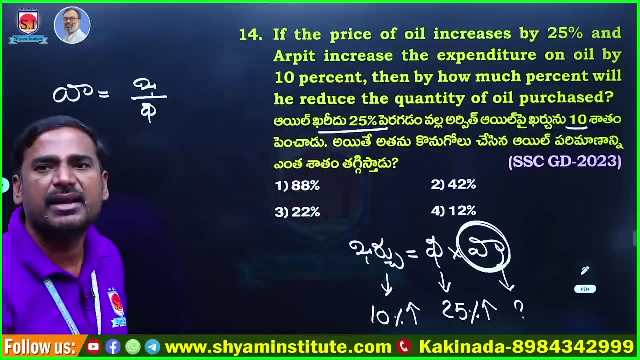 So the question is: what is the condition of Vodakam? The formula for Vodakam is Cost x Dara x RPT, So we need Vodakam here. Vodakam is equal to Cost x Dara x RPT. 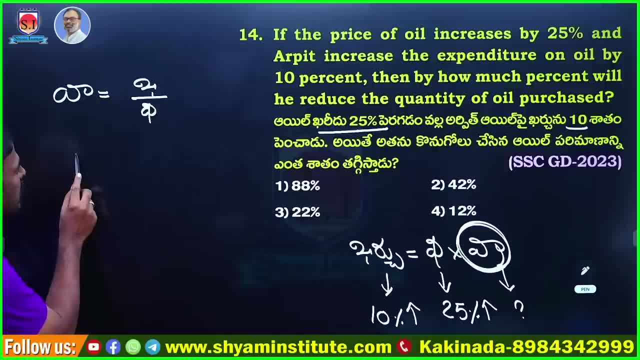 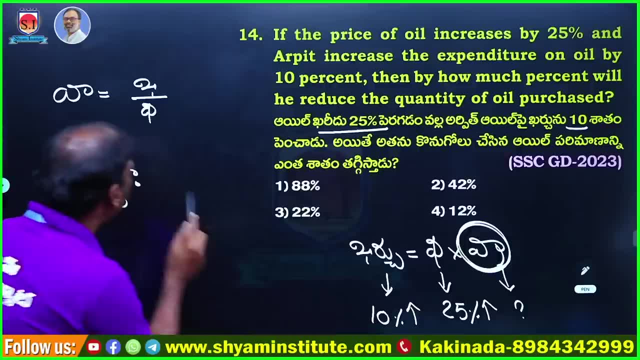 So if we see here, So if we assume that the actual cost is 100, and the actual rate is 100,, then the new cost increased by 10%, so we take 110, and the rate increased by 25%. so we take 125.. See What is the actual cost 100.. What is the actual rate: 100.. Then, since the cost increased by 10%, what is the new cost? 110.. Then, since the cost increased by 25%, 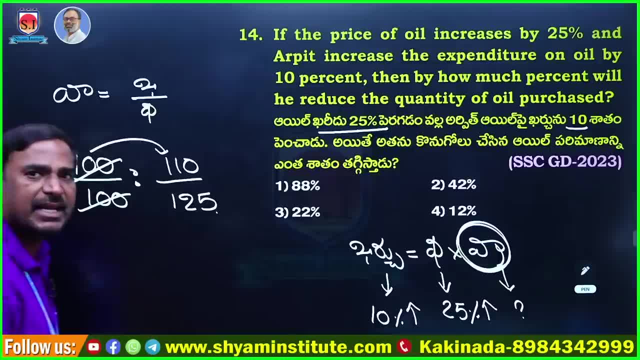 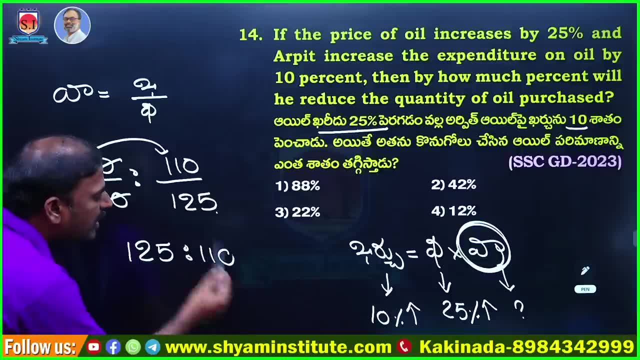 what is the new cost? 125.. Now, if we calculate 100 by 100,, what will be the value of this value? It will be 125.. What will be the value of this value? It will be 110.. So Vodakam with 125,. 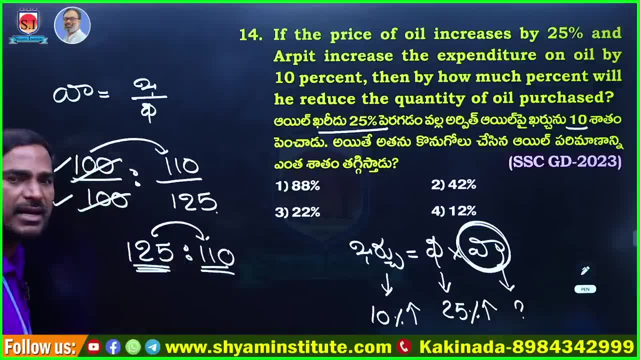 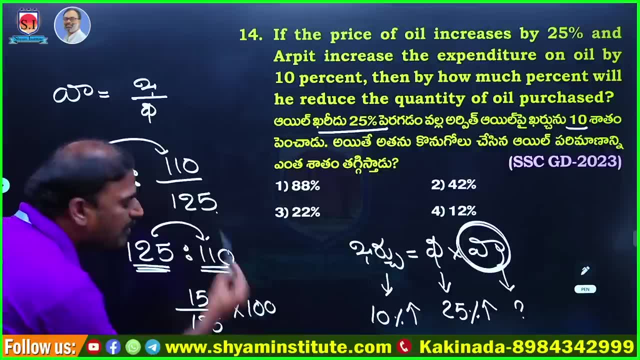 if it is 110, how much is Vodakam reduced? Let's say, 15 is reduced On whom? it is reduced On 125.. So how much is Vodakam reduced in 125?? On 125, it is 125. 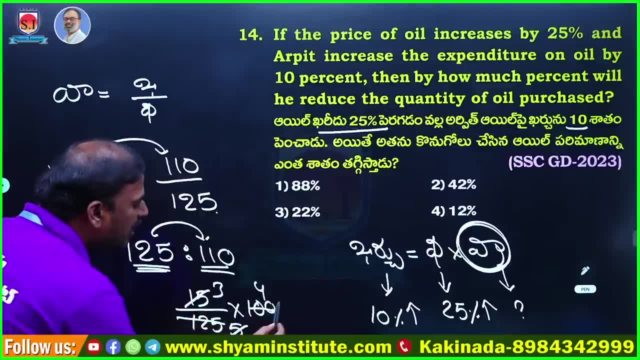 On 125, it is 400.. On 5, it is 315.. So how much is Vodakam reduced in 3 and 4?? Let's say Vodakam reduced by 12%. Let's say Vodakam reduced by 12%. 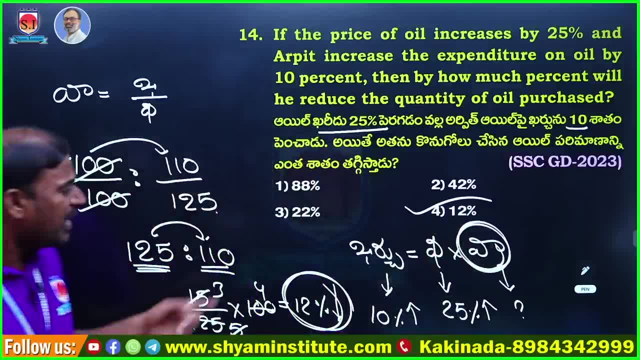 So option 4 is the right answer. So, option 4 is the right answer. If you want to do it more simply, if you consider this question as an option, if you consider this question as an option. if you consider this question as an option. 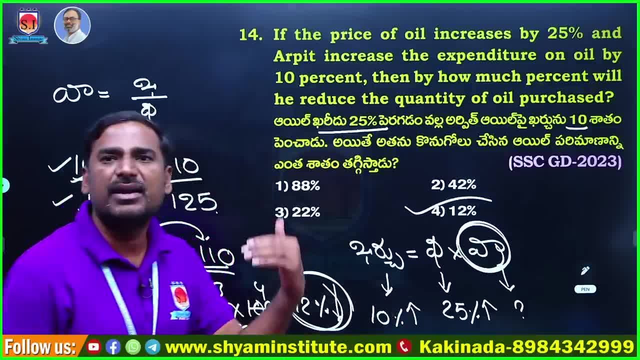 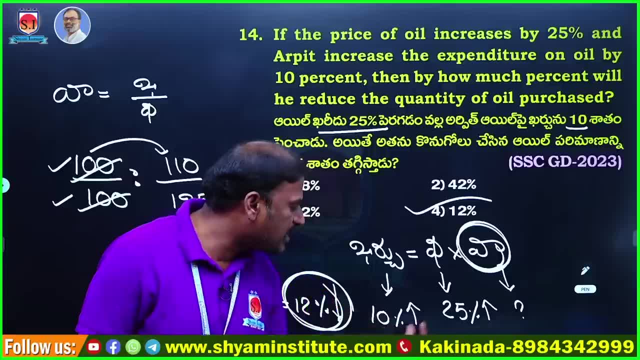 the cost increased by 10%, the rate increased by 25%, how much should Vodakam be reduced? Here it is 10 and here it is 25,. since it is 25,, what is the chance of us coming here automatically? 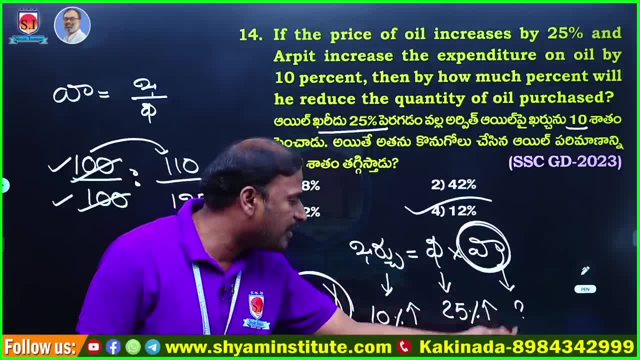 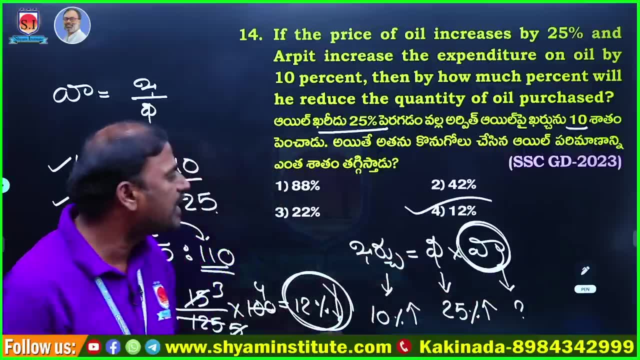 If the rate increased by 10% and increased by 25%, definitely we will reduce by 15%. If you look at the answer of 15 approximately, if you look at the answer of 15 approximately, you can take it as 12%. 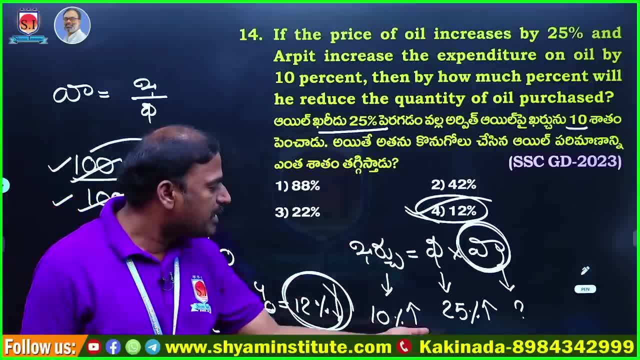 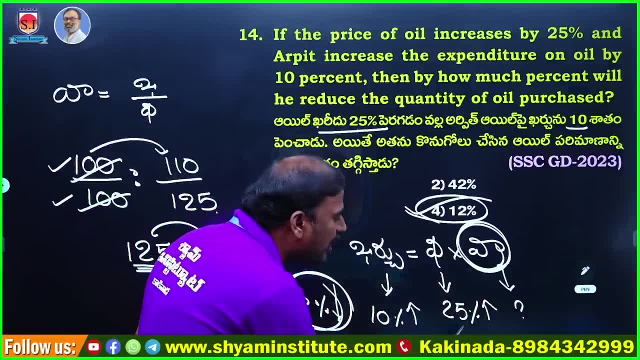 Once you think about it, the cost increased by 10%, the rate increased by 25%, Vodakam will not reduce by 42% Because these two are combined. if this is increased by 25%, if this is reduced by 42%, 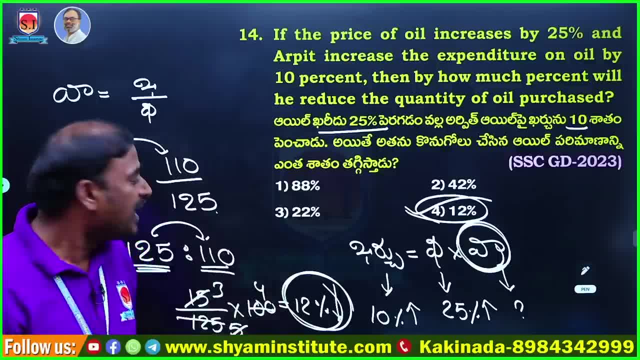 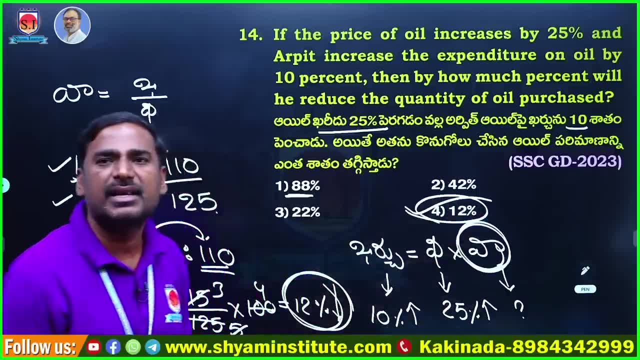 the cost will be reduced automatically. If you look at the second option, the first option is 88%. if this is increased by 25%, if this is reduced by 88%, the cost will be reduced. That is why, since this is increased by 10% and this is increased by 25%, 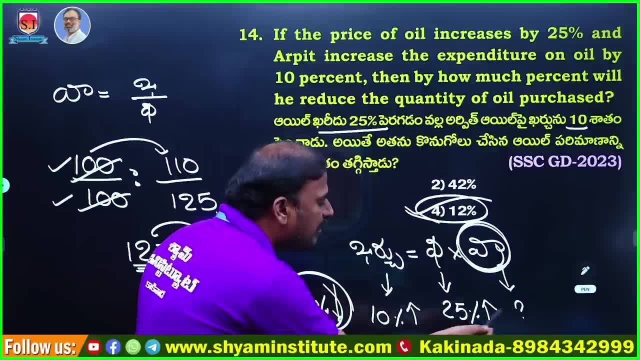 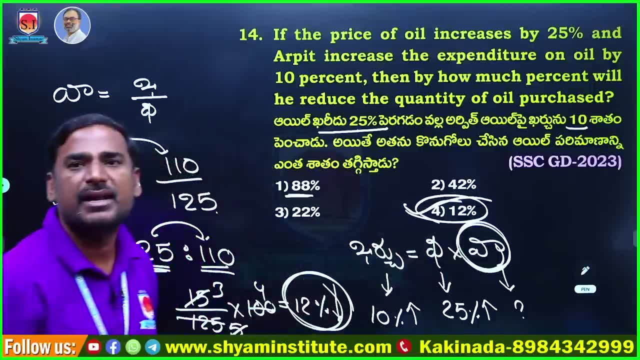 automatically. how much should we reduce? If we do 25 minus 15,, it will be plus 10, since there is only one option at 15 approximately, we can directly tick this. So all the options are there. So option number 4 is the right answer. 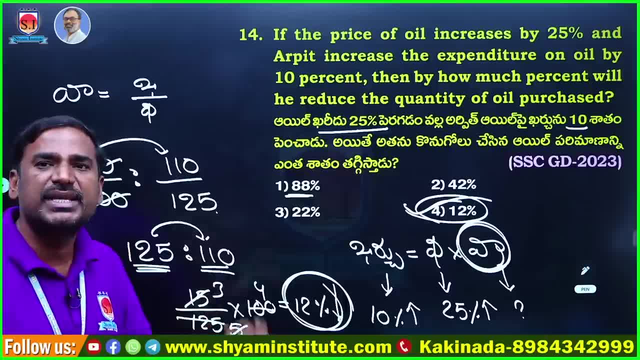 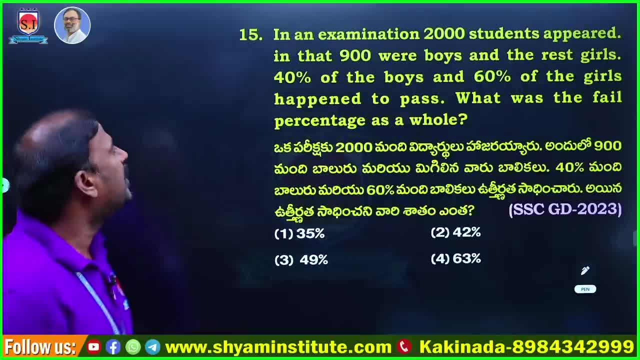 Similarly, we can see the correct answers by looking at the values through the option. Let us see the next question. Let us see the question number 15.. So what we have done so far is we have seen the problems related to int. 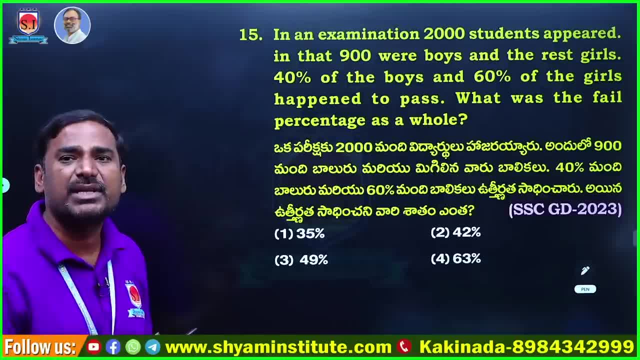 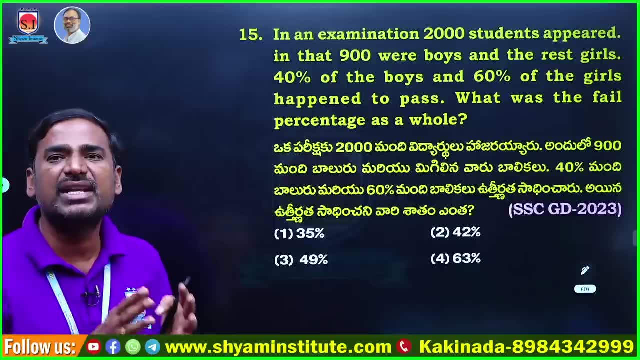 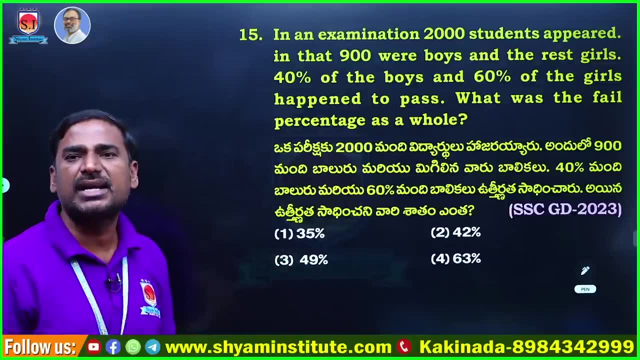 we have seen the problems related to plus and we have seen the problems related to successive, As we have seen this problem once. we have seen the problems related to addition. So, very simply, we can use the shortcut. Let us see the shortcut carefully. 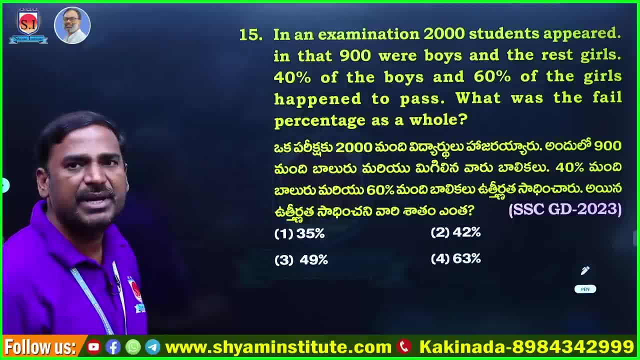 In an examination 2000 students appeared In that 900 were boys, the rest are girls. 40% of the boys and 60% of the girls happened to pass. What was the fail percentage in the whole? So what he meant was: 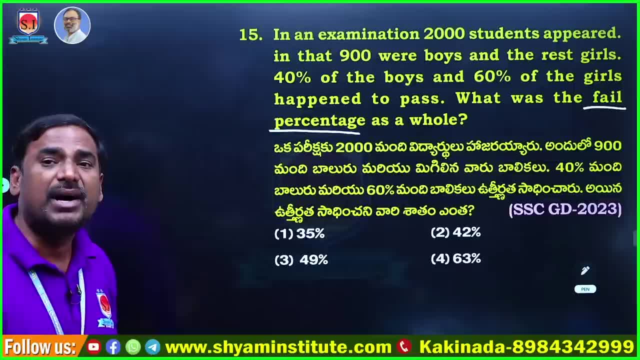 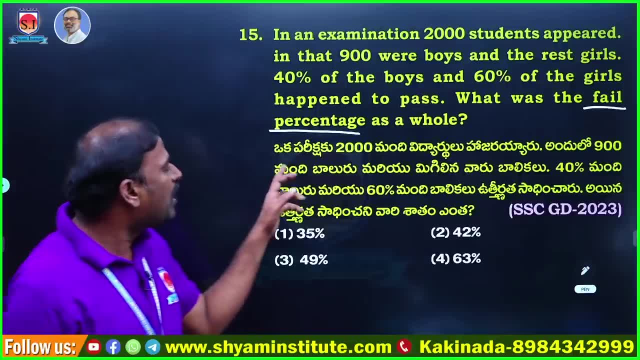 we have to calculate the fail percentage. Let us see how to calculate the fail percentage. In an examination, 2000 students appeared In that 900 were boys, the rest are girls. 40% of the boys and 60% of the girls happened to pass. 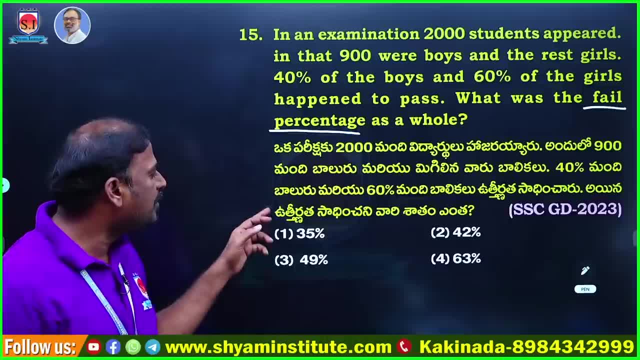 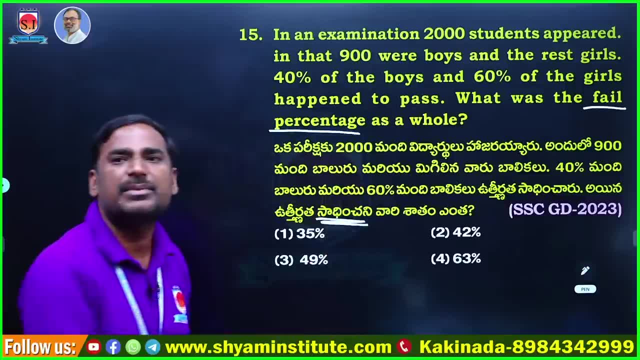 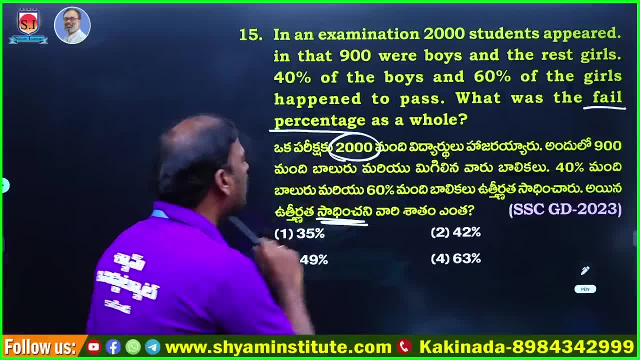 How many of them are there? What percentage of them are there in all, Sir, the percentage of those who come to school is 200.. Sir, spoiler face 2: 2000 students As 4 2 0, 0 members have passed. 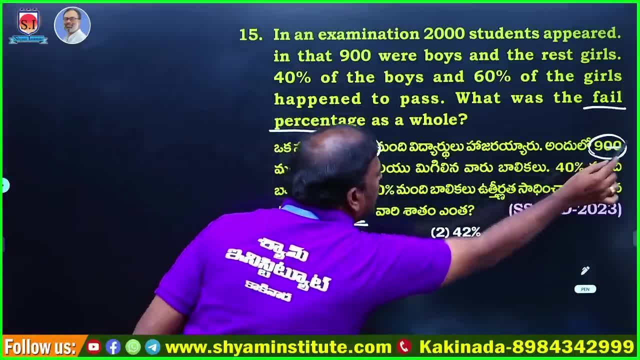 they could have very clearly given 0 as a test. Here the measure is 2 brothers, come in, Sir. how many did they trouble you? now, Sir, the India food is less than 1 111 medicines when they came and took the Wat. 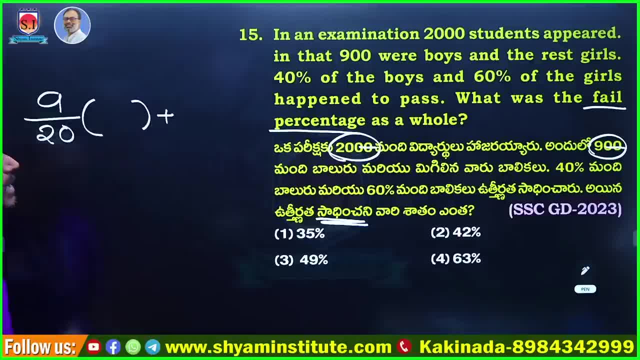 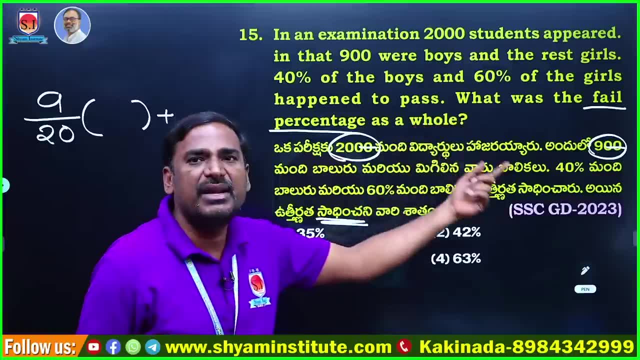 Sir 2 is the first food they should be taken a 맞아 after a flight. That means that they escaped first because they had to bring food after the flight, Sir. The remaining 11 parts will be taken by girls. 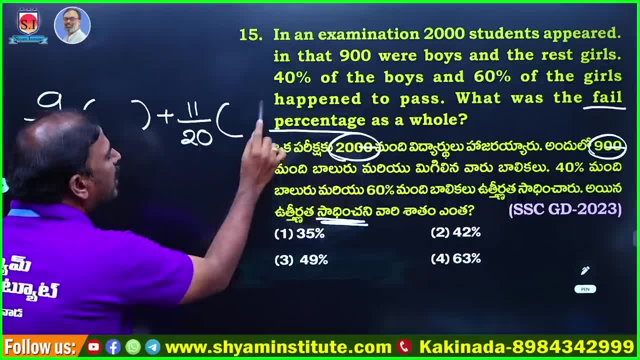 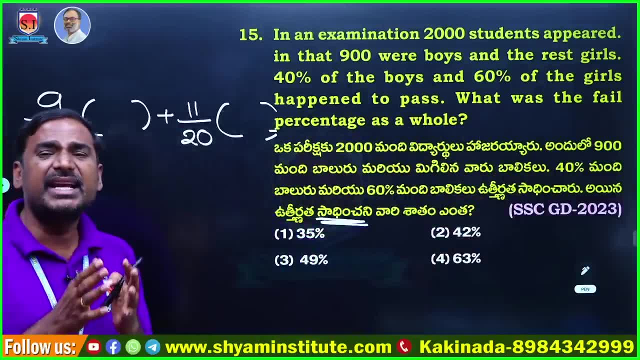 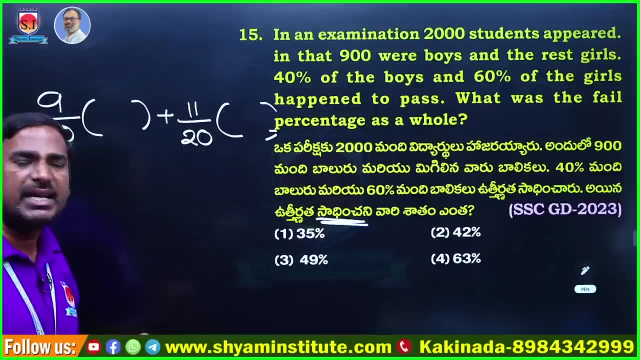 The total number of girls here is 10, and the total number of boys is 20.. You can apply this shortcut directly to any problem related to edition. What is this shortcut? There are 2000 boys in total and 900 girls. 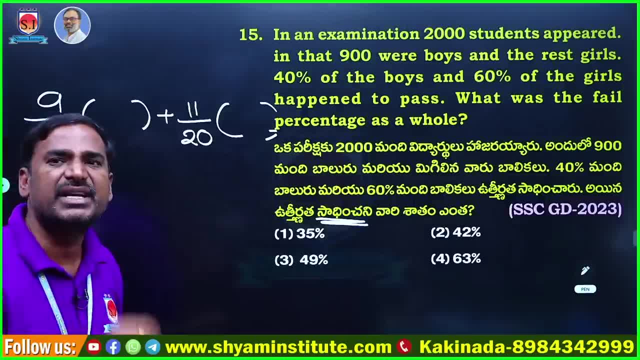 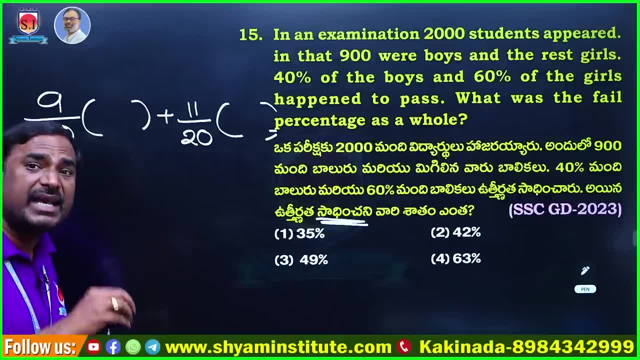 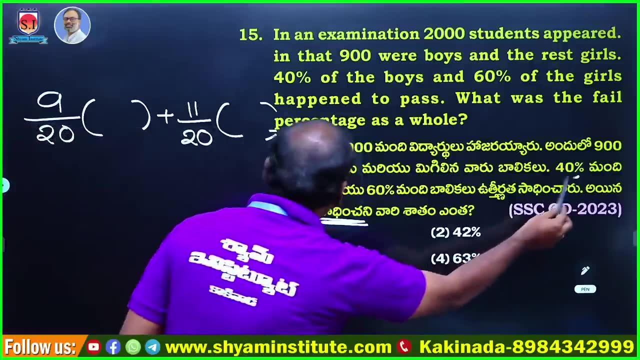 If we subtract 0,0,0,0,, the total number of boys is 9 out of 20.. Girls are 11 parts out of 20.. He said that 40% of boys and 60% of girls achieved success. 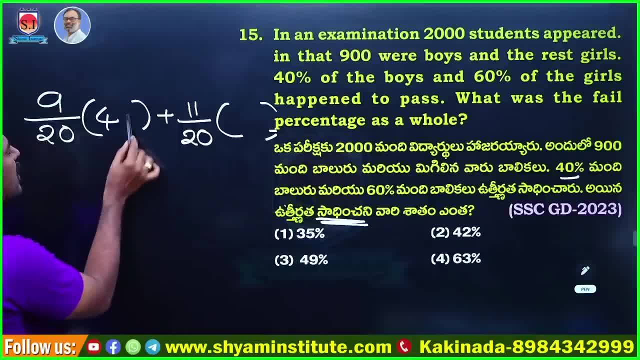 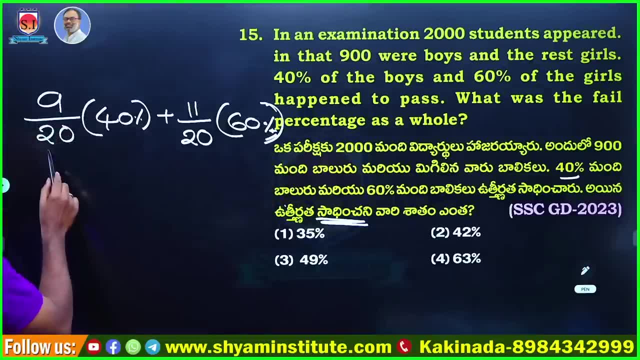 Here, 40% of boys achieved success and 60% of girls achieved success. Boys achieved success and girls achieved success. Now, 21 parts are cancelled in 22 parts and 21 parts are cancelled in 23 parts. 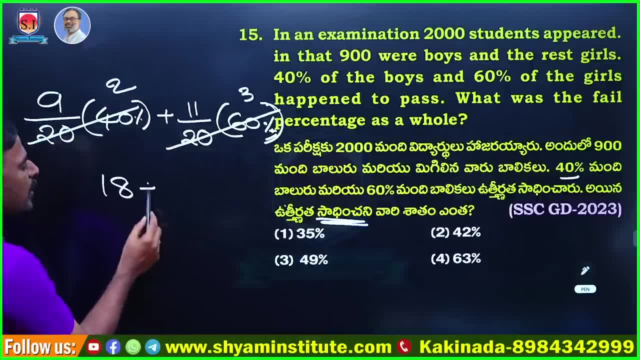 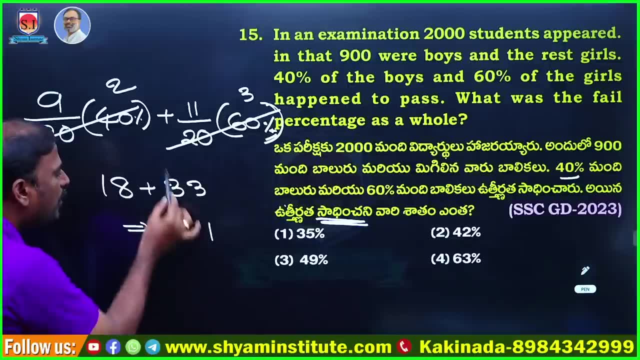 Now 19 parts out of 92,, 33 parts out of 19, and 33 parts out of 33.. The number of people who achieved success is 8,, 3,, 11,, 1,, 1, 3,. 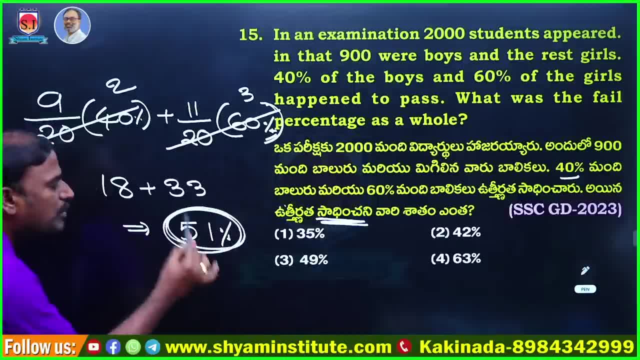 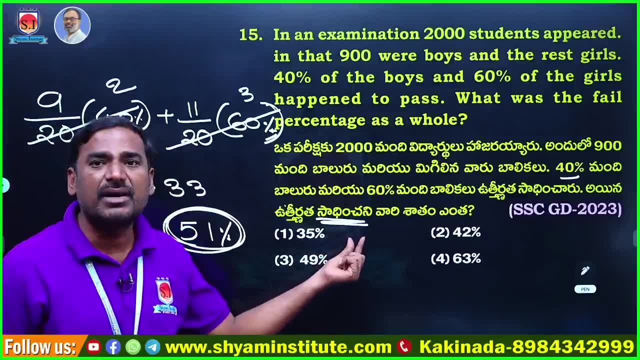 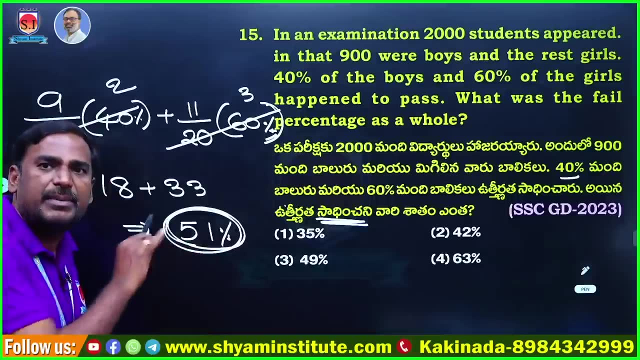 4, 1, 5.. So the number of people who achieved success is 51%. But the question he asked is not the number of people who achieved success, but the number of people who didn't achieve success. If the number of people who achieved success is 51%, 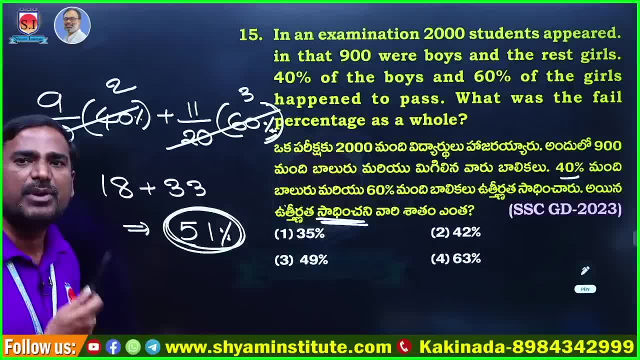 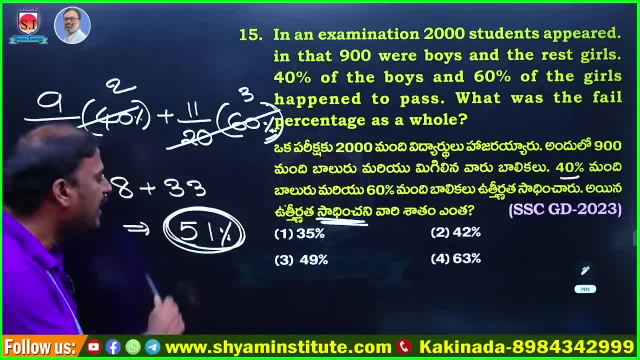 how many people achieved success? We always take 100%. So in the condition that no one achieved success, they should take 100%. If we take 50% of people, then we have to take 100 out of 100, how many people did we achieve success? 1, 1, 0,, 1, 3,, 2, 3,, 4,, 5,, 6, 7,, 7, 8, 9, 7, 8, 9,. 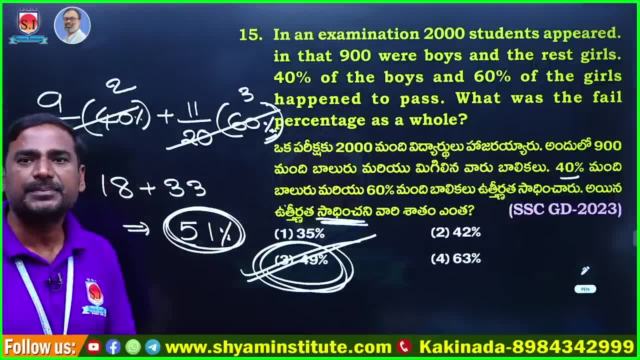 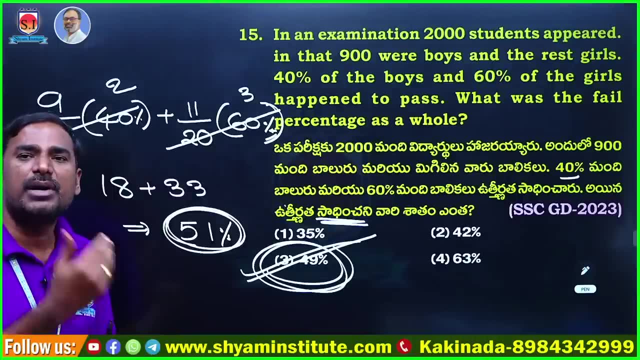 10,. This is just a sample. Let's see how the question is being asked on the addition base. What is the need for the addition base? What should we do at this time? The people living in a village are men and women. 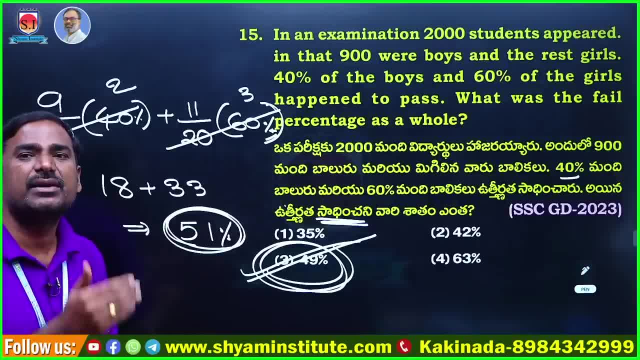 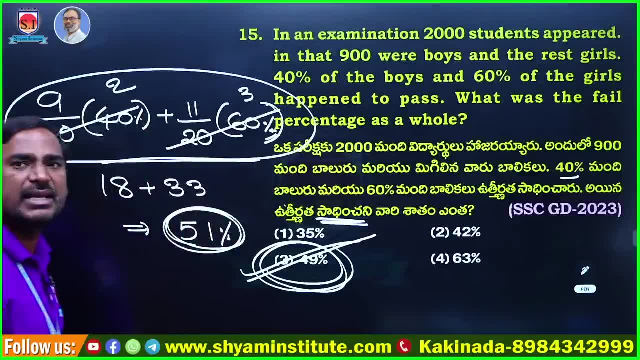 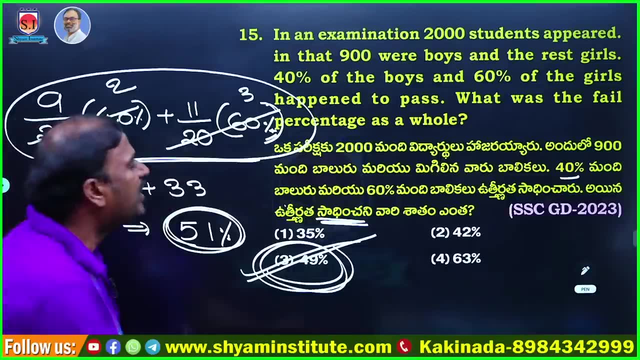 The cost plus income is equal to income. What is the shortcut you should apply for any such problem? You should apply this: What is the ratio between the number of children and the number of children? We don't have to pay the cost of Rs 9000 to Rs 2000.. 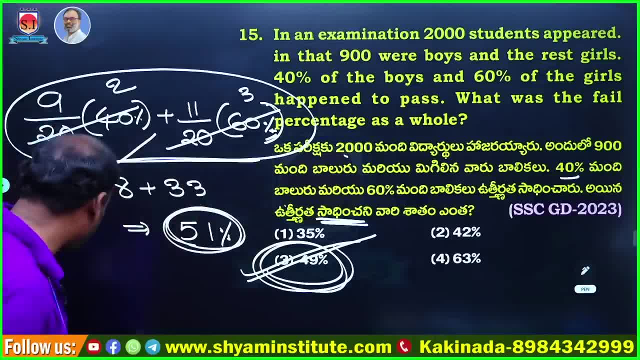 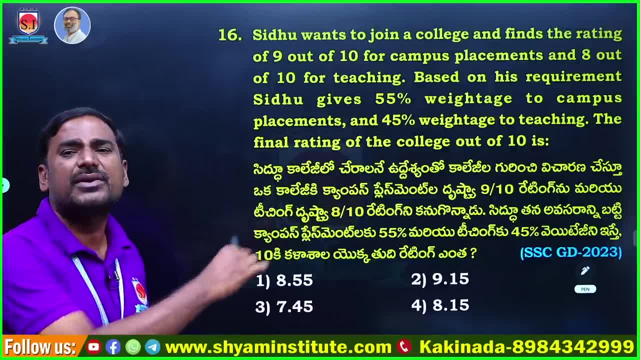 We can solve it directly with this. Let's see the next question. Look at question no 16.. Last year he asked a very simple question on this. Let's see it once. Siddhu wants to join a college and finds the rating of 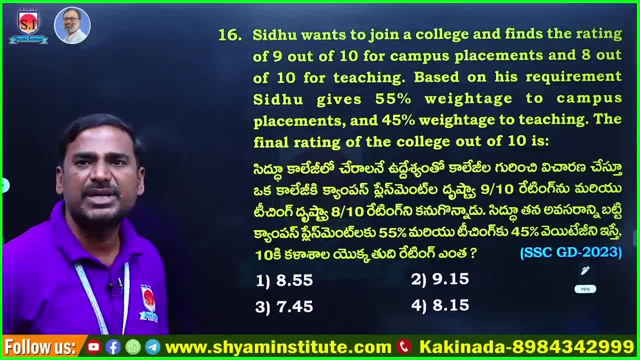 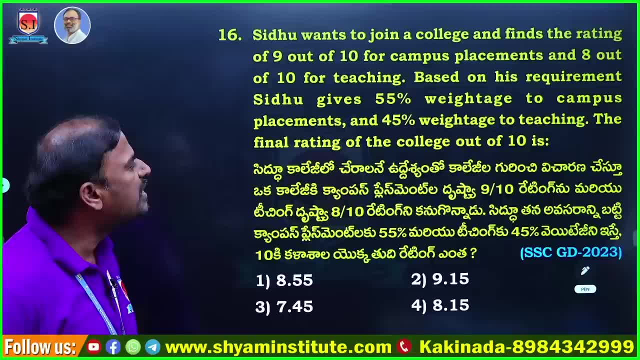 9 out of 10 for campus placement and 8 out of 10 for teaching. Based on this requirement, Siddhu gives a 55% weightage to campus placement and a 45% weightage to teaching. The final rating of the college is out of 10.. 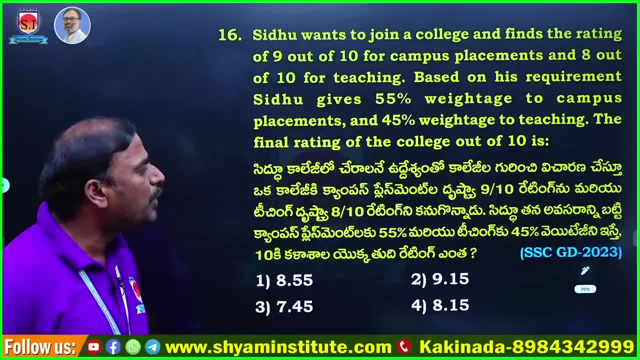 So Siddhu wants to join a college. He thinks about the college. For a college, the rating of campus placement is 9 out of 10.. And the rating of teaching is 8 out of 10.. Siddhu thinks the rating of campus placement is 50%. 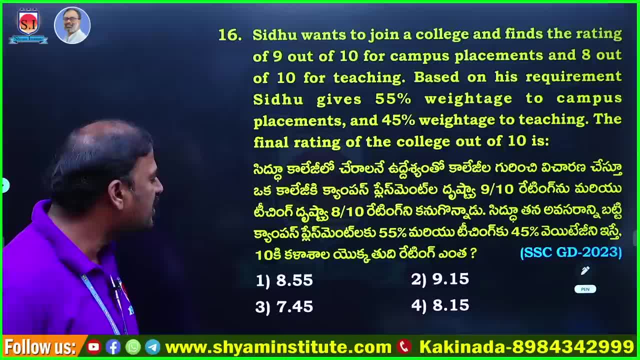 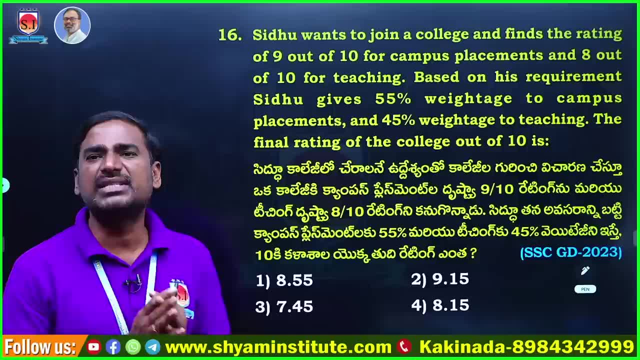 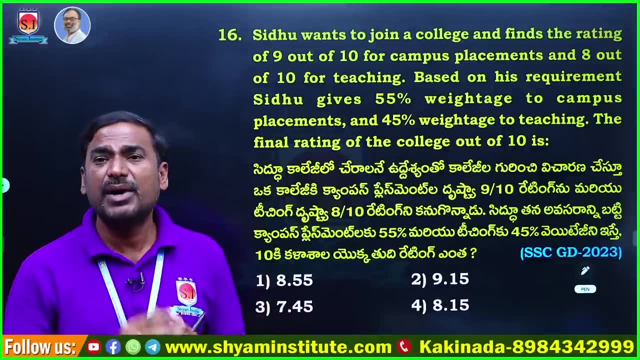 and the 40% weightage to teaching is 10 out of 10.. When Siddhu investigates the concept of joining a college, he focuses on two things: One is whether there are placements and the other whether the teaching is good or not. 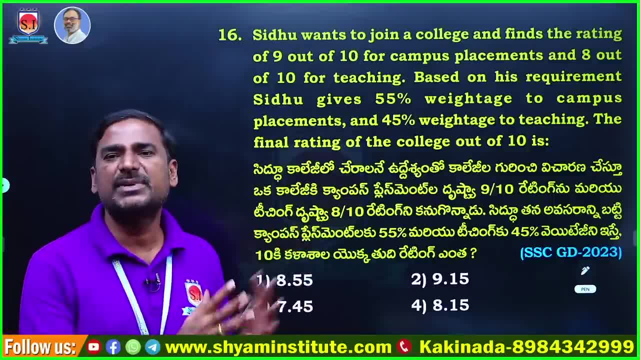 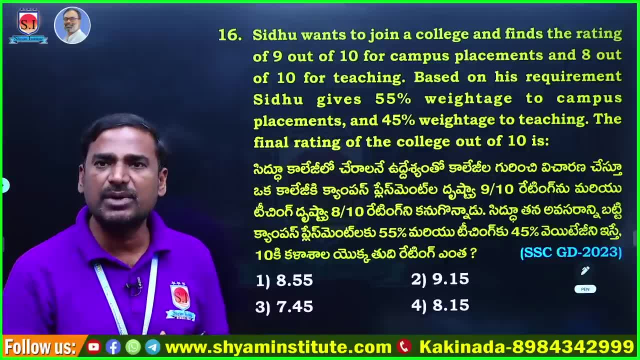 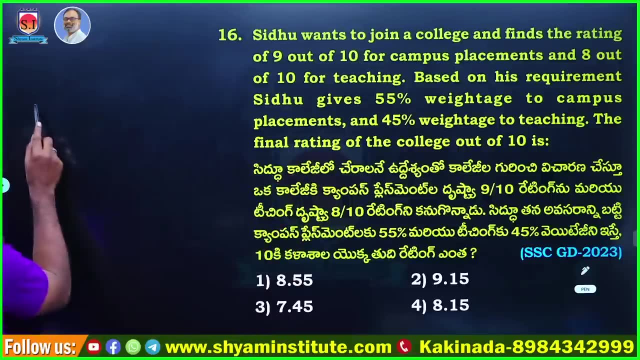 If we want to join a college. So we will see whether they are showing any placement or not. Next we will see whether the classes they teach are good or not. Here there are two behaviors. One is the rating of the placement is 9 by 10.. 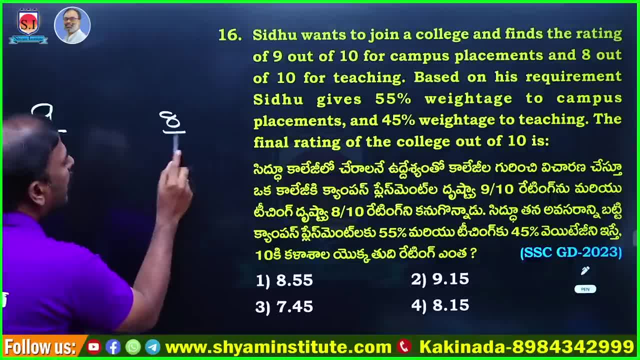 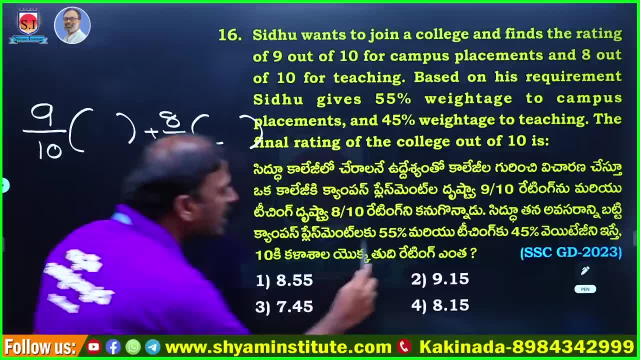 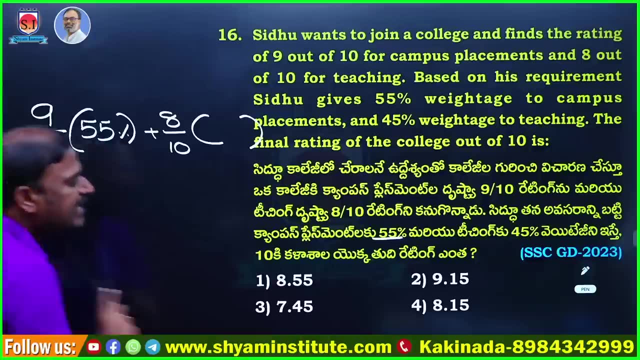 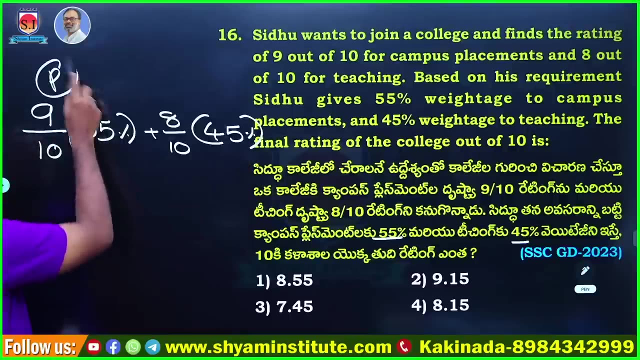 The rating of the teaching is 8 by 10.. So the rating given by Sidhu is that he gave 55% for campus placement. He gave 55% for campus placement. He gave 45% for teaching. The placement rating is 9 by 10.. 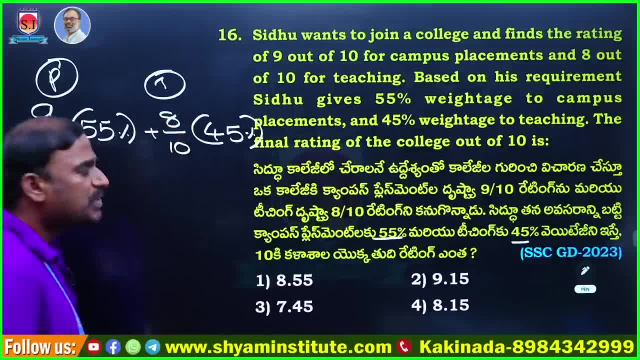 And the teaching rating is 8 by 10.. Sidhu gave 55% for this and 40% for this. The overall rating is 9 by 10.. Sidhu gave 55% for this and 40% for this. 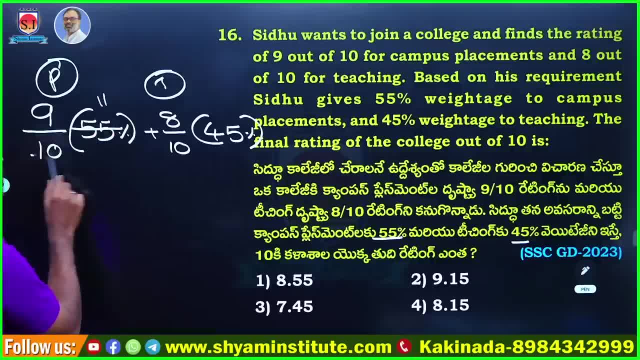 Now, as you can see, 5 by 11 is cancelled, 5 by 2 is cancelled, 5 by 9 is cancelled, 5 by 2 is cancelled. So we will write: 9 by 11 is 99.. 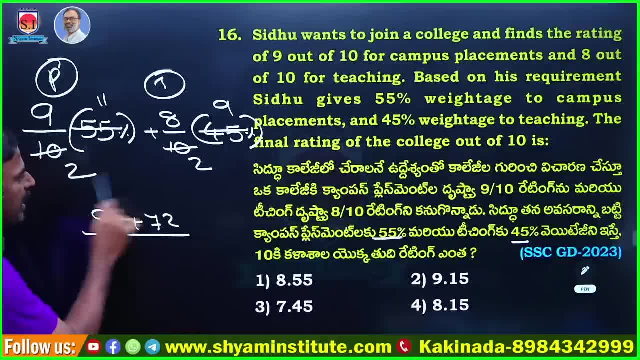 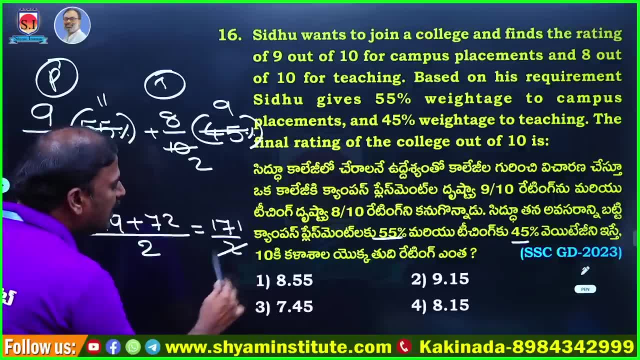 8 by 9 is 72.. Let's take LCM 2 for both. We will write it as 171 by 2.. The value we get is: 2 by 8 is 16.. 2 by 5 is 10.. 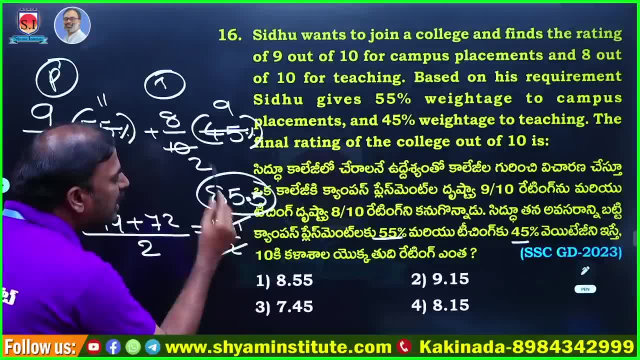 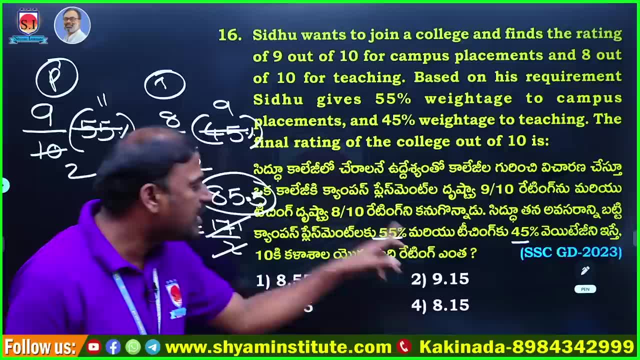 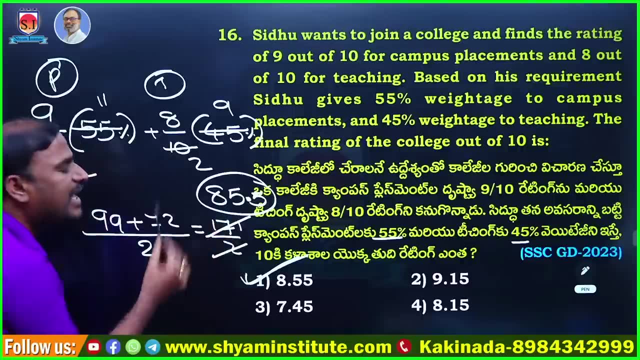 2 by 5 is 2.. So we will write it as 85.5.. 85.5 is the right answer for the 8 by 5 option, If you think about it, Since 10 is the rating. 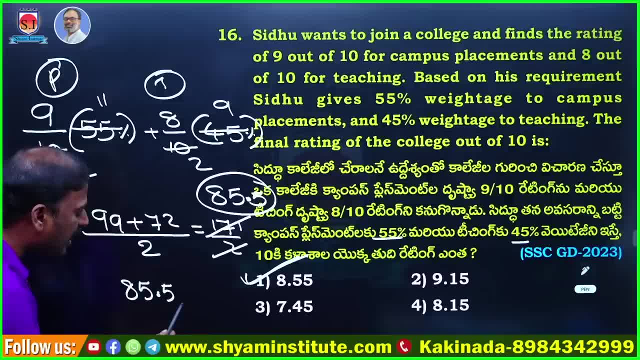 85.5 is the percentage. If we take 10 as the rating, it will be by 10.. We will write it as 8.55.. If we take 10 as the rating, it will be by 10.55.. 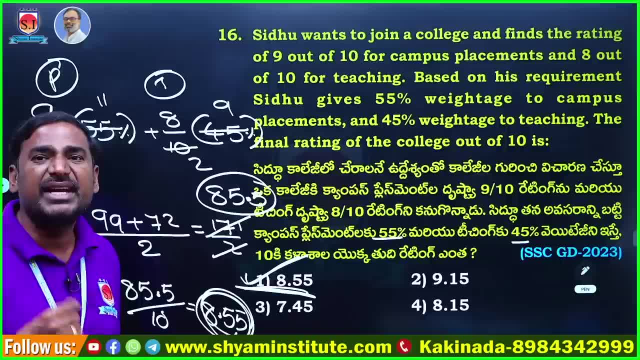 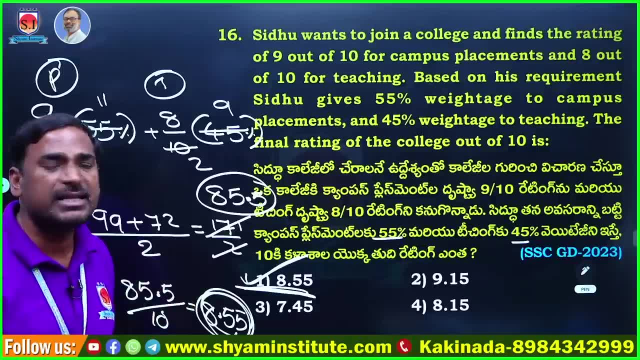 We will write it as 8.55.. Option 1 is the right answer. Who is this problem for? It is a problem related to edition. Earlier we saw that we have done the concept of Baluroo plus Balika, So we have to do the same for this too. 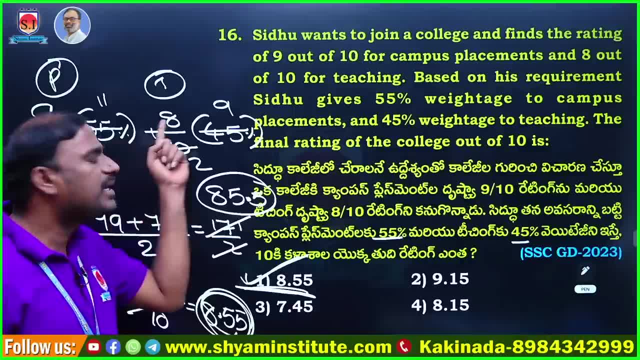 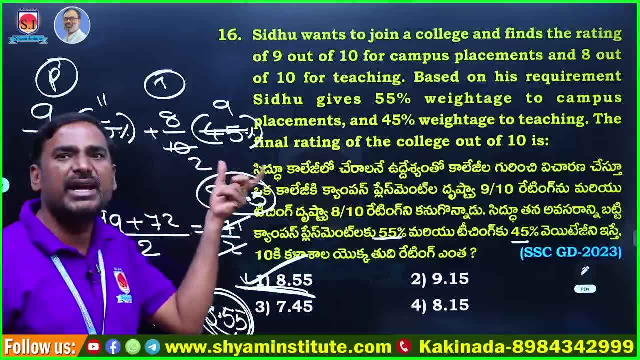 Here we have to do it in two ways. One is placement and the other is teaching. If placement is 9 by 10, teaching is 8 by 10. In this, Sidhu's rating is 45% for 8 by 10.. 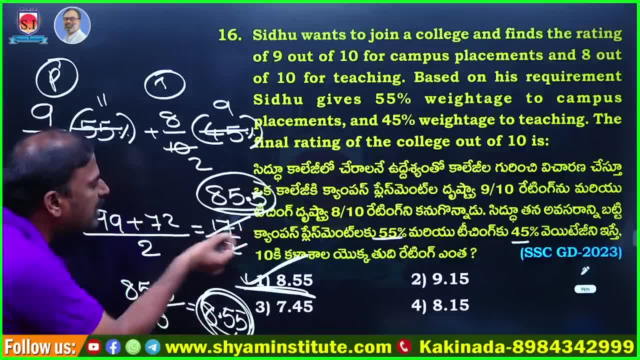 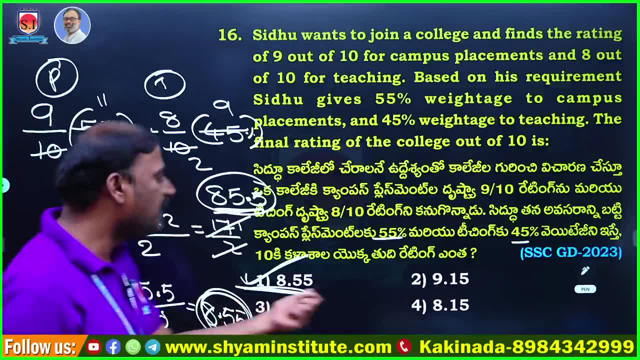 The percentage given by Sidhu is 85.5.. If we write the name out of 10, it will be 8.55.. So this is the answer. So this is the answer. So this is the answer. 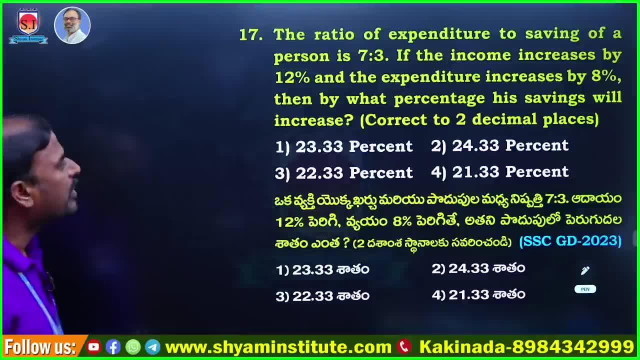 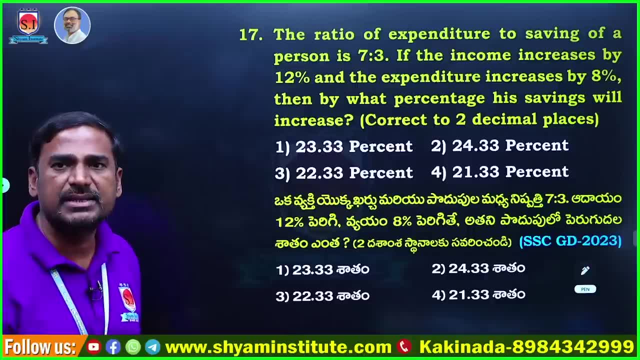 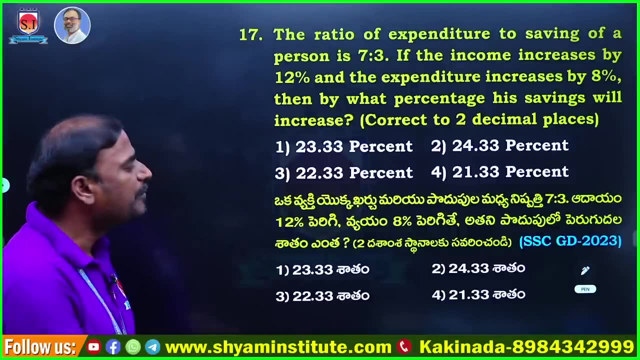 Next question, Question 17.. Question 17.. In the previous problem we said Baluroo plus Balika, boys plus girls. After that we said the ratio of the expenditure plus saving is 7, is 2, is 3.. 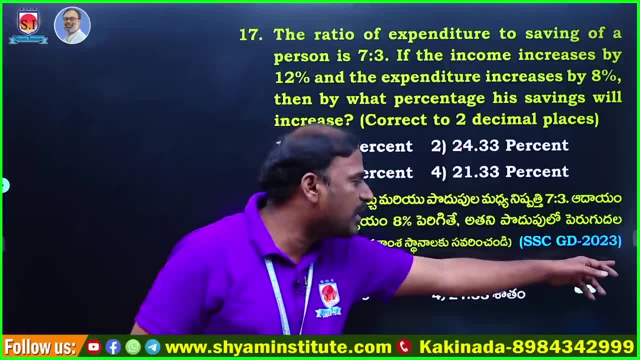 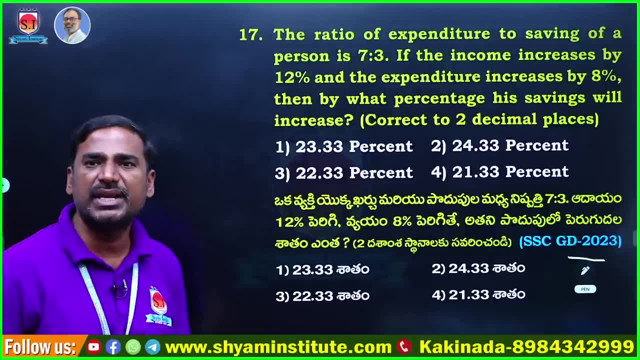 So, on this same problem, how can we ask this question in SSE GD 2023?? Look at the question and see how we can ask the question on that question. So the ratio of the expenditure to saving of a person is 7, is 2- 3.. 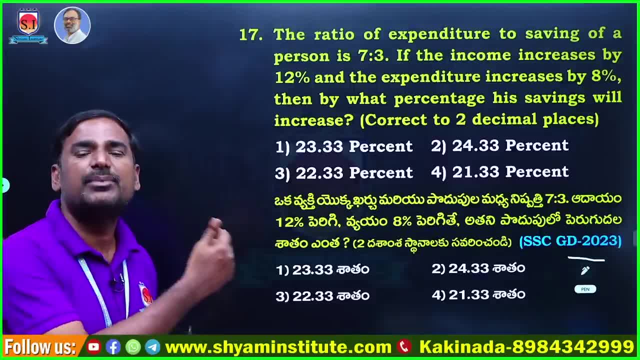 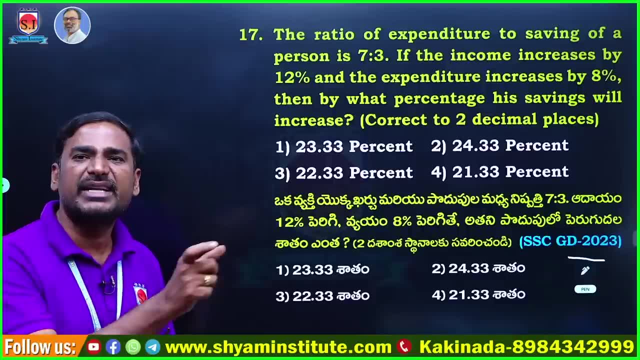 What did he give there? He gave 7 parts of the expenditure and 3 parts of the saving. So what is equal to expenditure plus saving is Income. So Income is equal to expenditure plus saving. This is a problem related to addition. 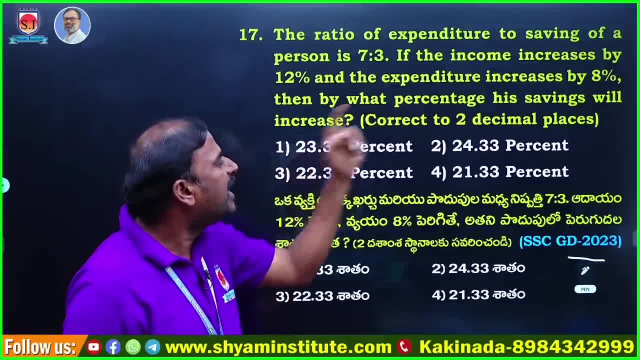 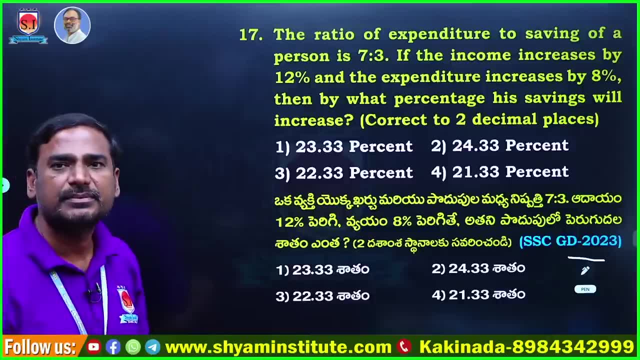 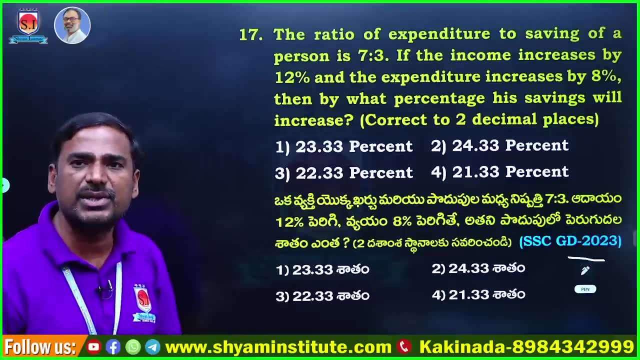 So the income increased by 12% and the expenditure increased by 8%, then by what percentage is saving will be increased? One person's income and daily income is 7.3%. What is the rate of income and daily income? It is 7.3%. 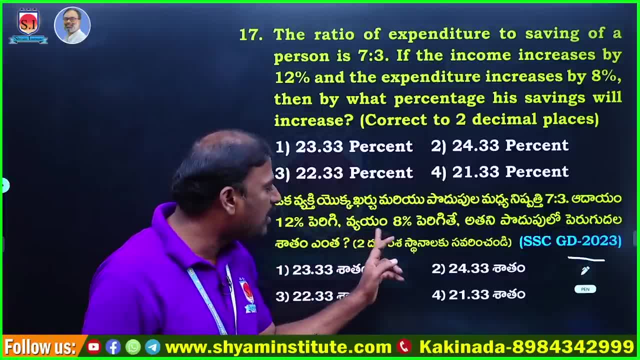 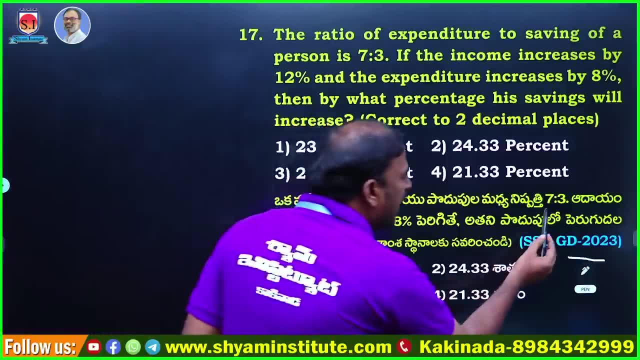 So the income increased by 12% and the daily income increased by 8%, What is the rate of increase in daily income? Think about it: If 7 is equal to 3, then the expenditure is 7.3% and the daily income is 3.3%. 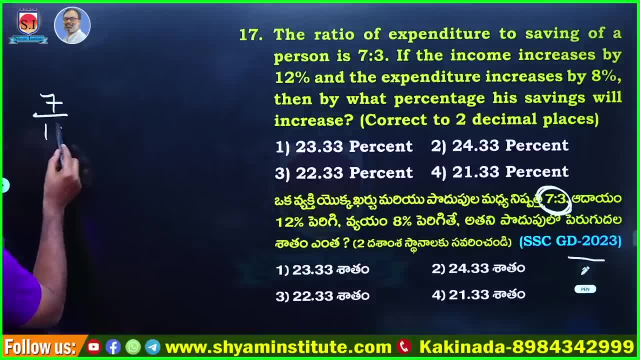 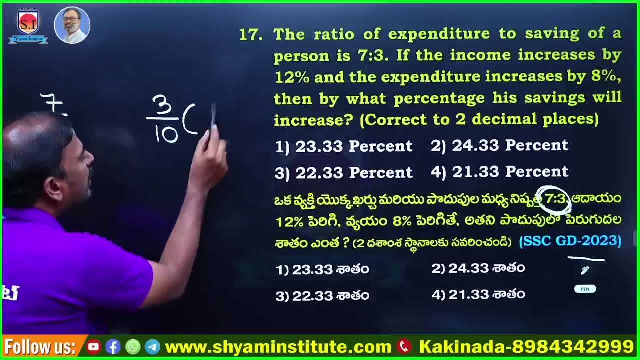 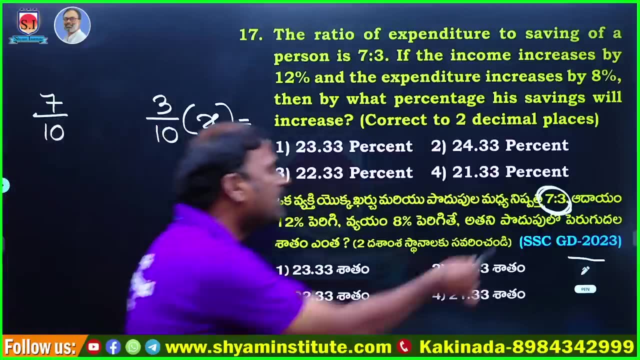 The expenditure is 7.3% and the total is 10.3%. The daily income is 3.3% and the total is 10.3%. The question is: what is the rate of change in the daily income? The expenditure is 7.3% and the total is 10.3%. 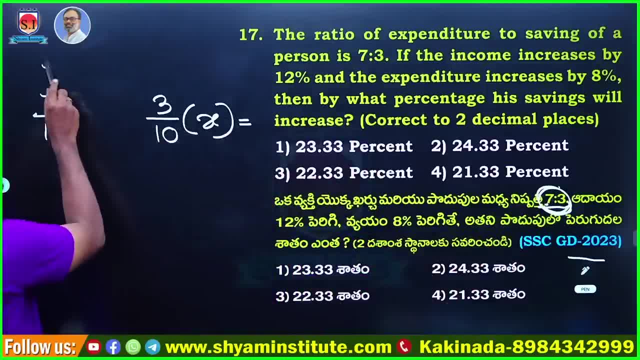 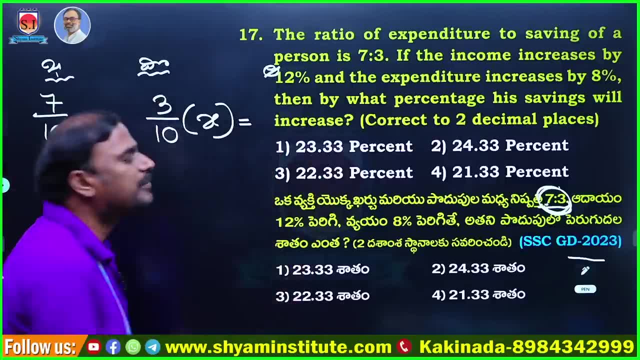 The daily income is 3.3%, That is 10.. So the expenditure is 7.10% and the daily income is 3.10%. So what will be the monthly income? сколько? The expenditure and daily income is equal to the monthly income. 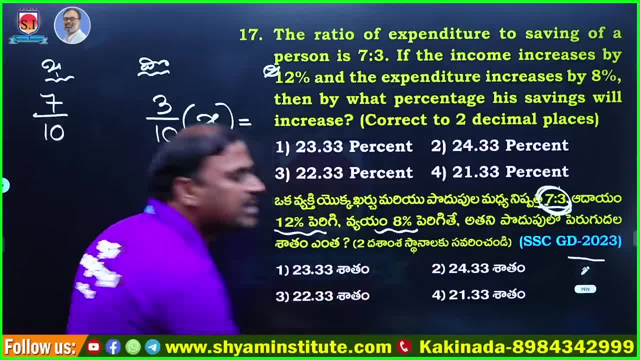 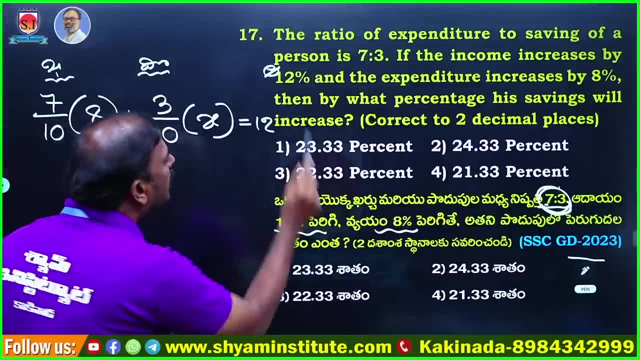 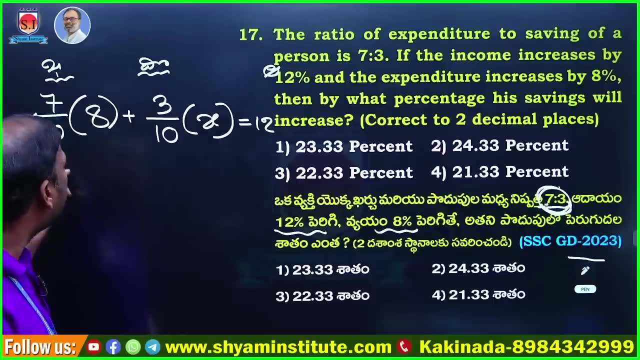 So the говорすごい, the daily incomeω. So the cost is 7 by 10,, the income is 3 by 10, the cost is 8% and the income is 8.5%. what is the income? 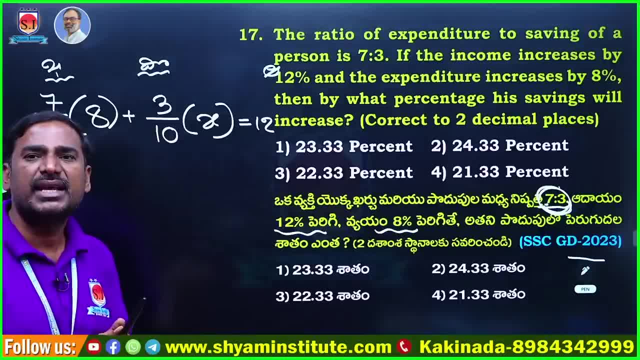 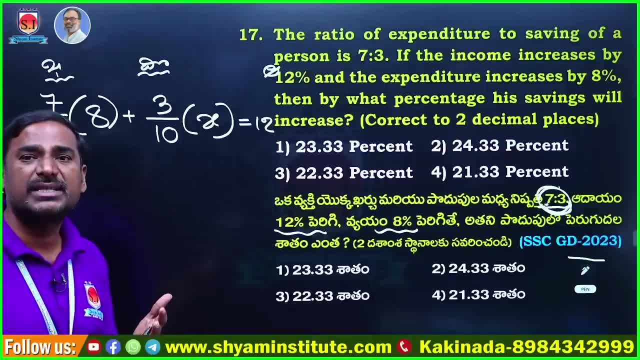 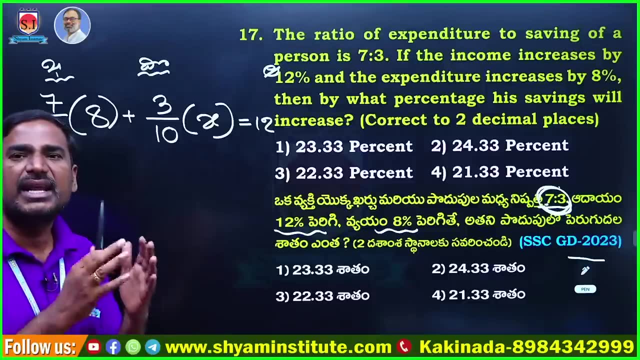 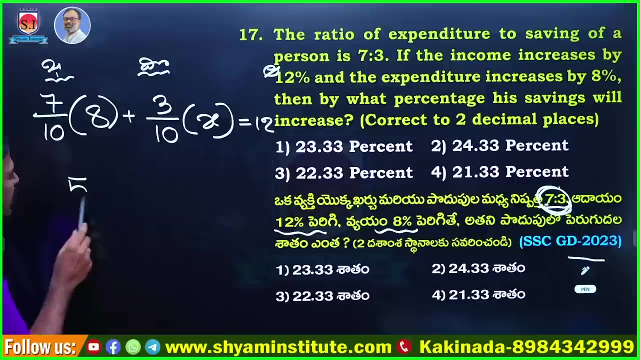 So you can apply this shortcut to any problems related to plus. This shortcut applies to boys plus girls, men plus women, placement plus teaching expenditure, plus saving any type of problems. So 7 by 8 is 56, this is 3x. 10 by 12 is 120. 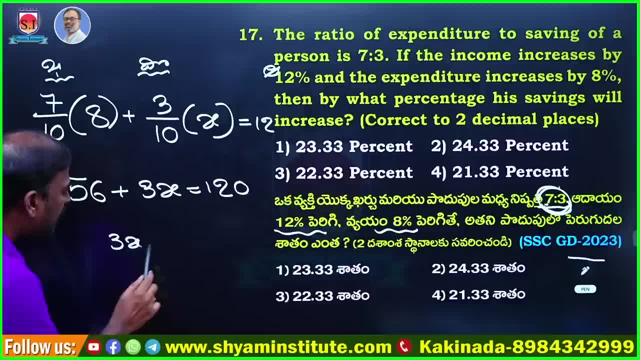 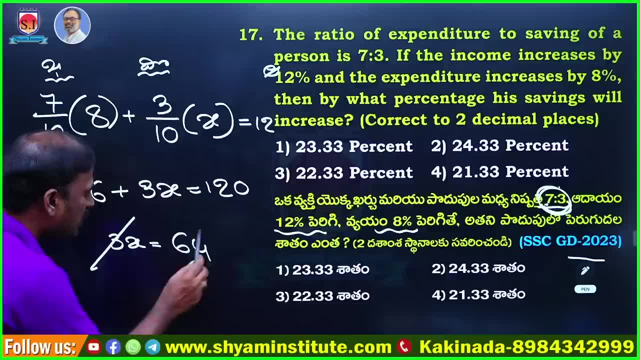 So, if we calculate this 3x, If we calculate this 56, 120 minus 56 is 64. This value is 3x2 is 6, so 3x1 is 3.. See: 3x2 is 6 and 3x1 is 3.. 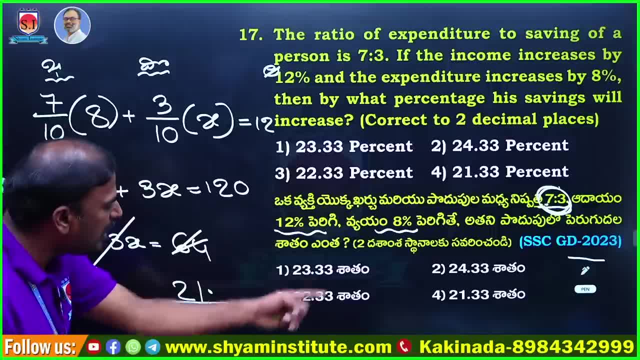 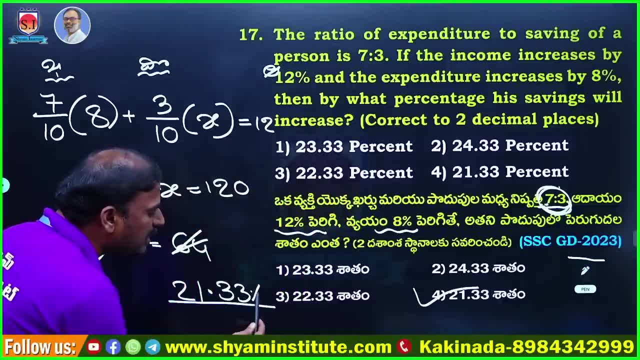 We don't have to do this anymore, Because there are so many options here. See, there are so many options here. See, there are so many options here. So we are taking it as 21.33%. So we are taking it as 21.33%. 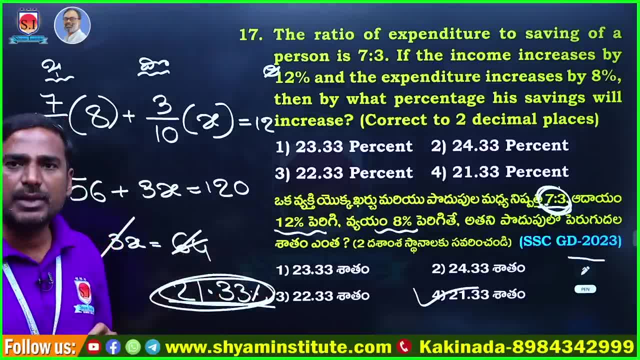 Whenever you do the calculation, you don't have to do anything. Whenever you do the calculation, you don't have to do anything. Just take attention to the options here. Once you do that, you will see the value there. Once you do that, you will see the value there. 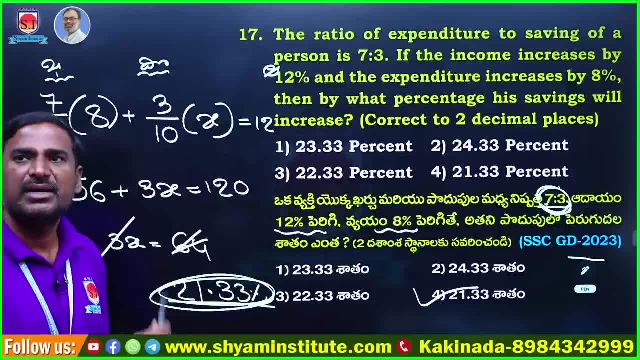 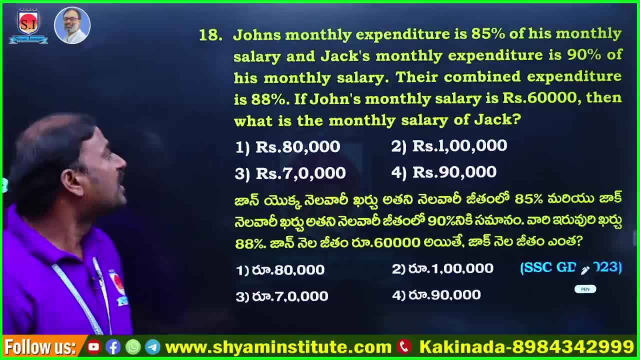 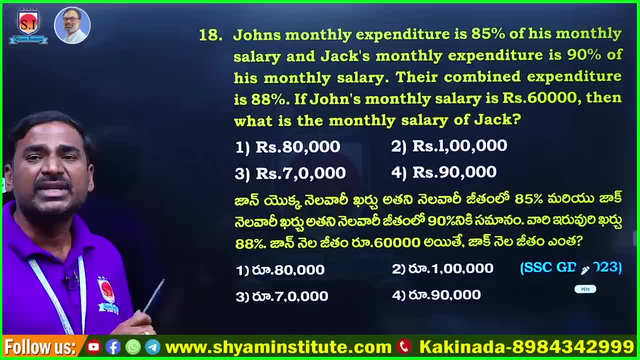 Don't do the calculation until the last position. even you do the last check. Don't do the calculation until the last position. even we do the last check. Let's see the next question, Question number 18. We have seen how you can do questions for plus and int. 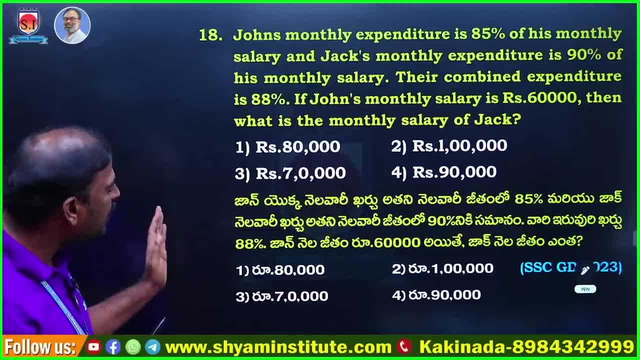 We have seen how you can do questions for int. Let's see how we can've done this discussion. Let's see how to do this question in SSCGD 2023.. Let's see how to do this question in SSCGD 2023. 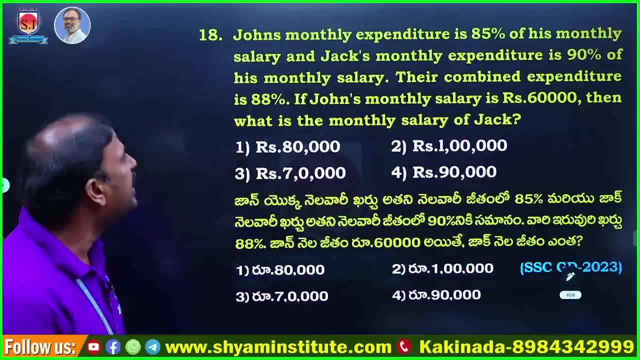 Let's see how to do this question in SSCGD 2023.. The question given is: John's monthly expenditure is 85% of his monthly salary. John's monthly expenditure is 85% of his monthly salary. John's monthly expenditure is 85% of his monthly salary. 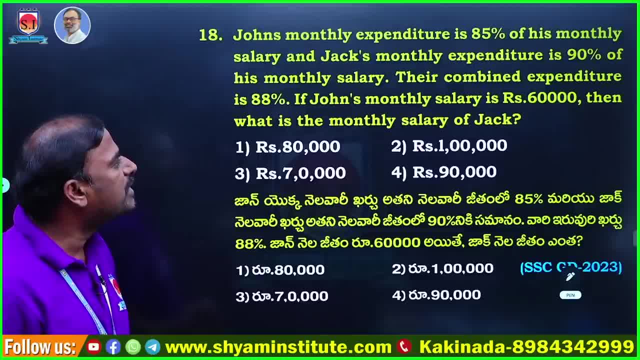 Jock's monthly expenditure is 90% of his monthly salary. Jock's monthly expenditure is 90% of his monthly salary. Their combined expenditure is 88%. Their combined expenditure is 88%. John's monthly salary is 60,000 rupees. 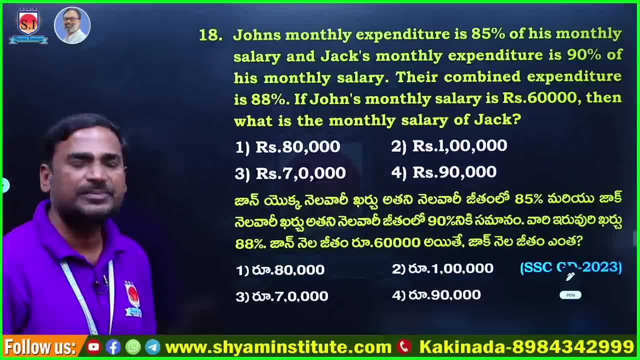 Then what is the monthly salary for Jock? Then what is the monthly salary for Jock? So John's monthly expenditure is 85% of his monthly salary. So John's monthly expenditure is 85% of his monthly salary. So John's monthly expenditure is 95% of his monthly salary. 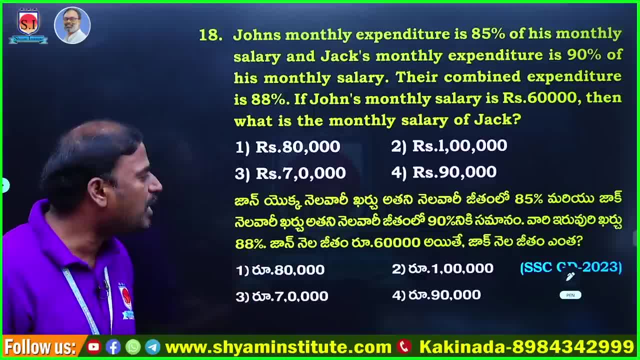 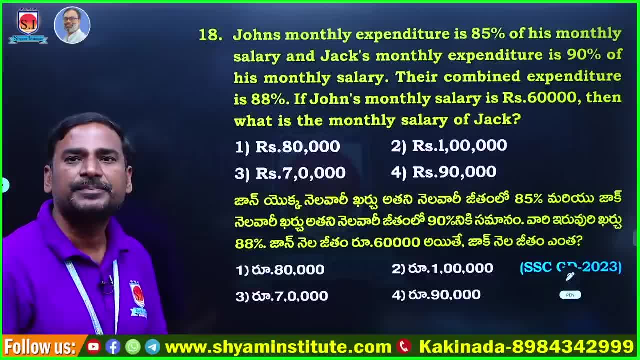 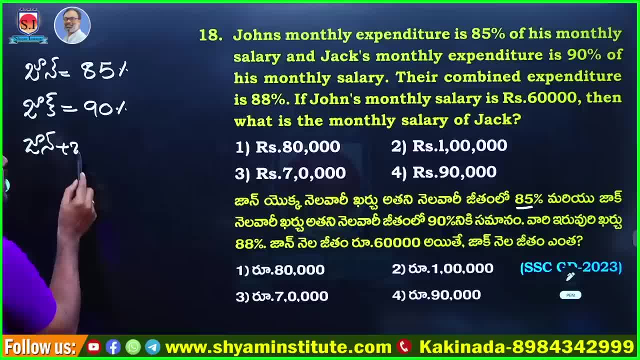 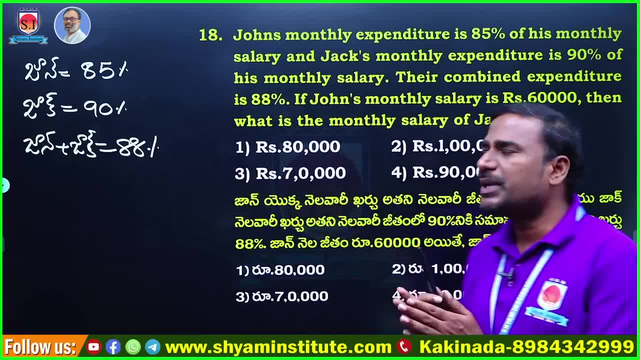 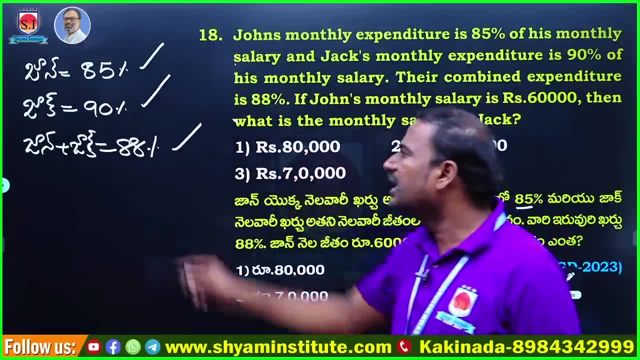 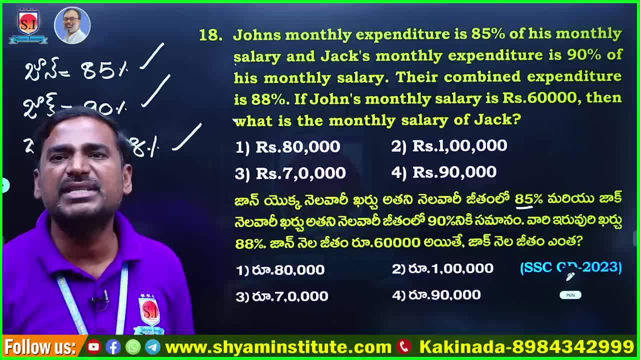 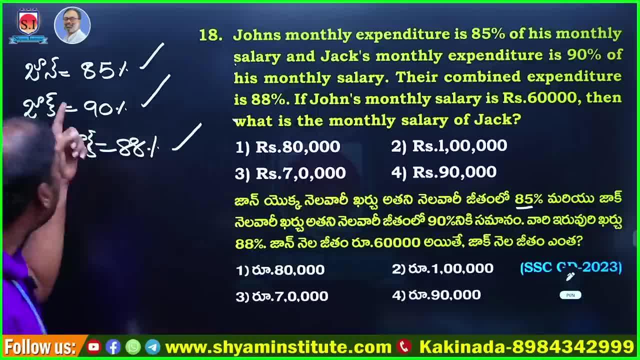 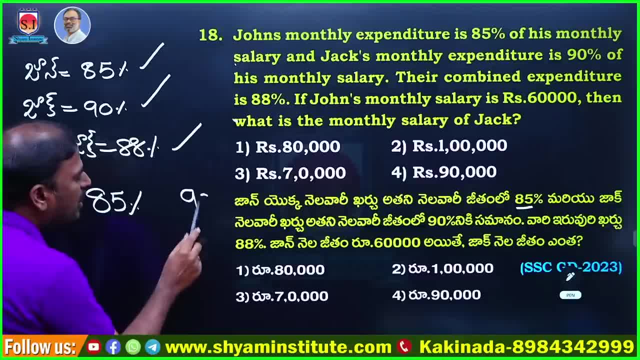 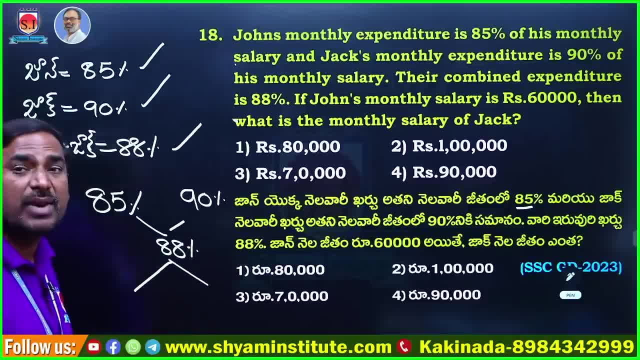 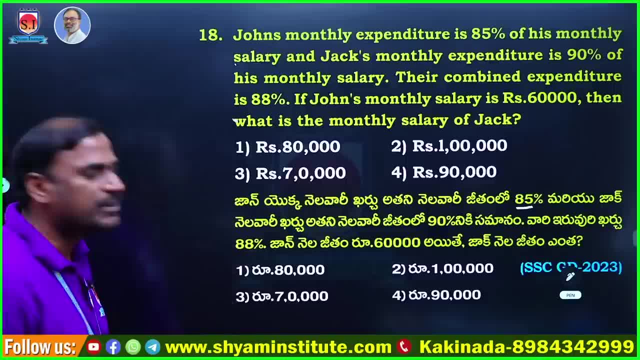 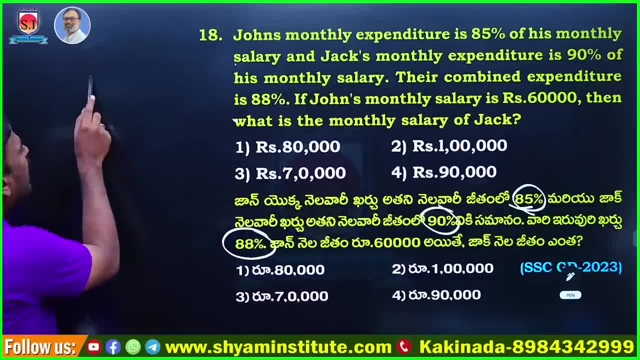 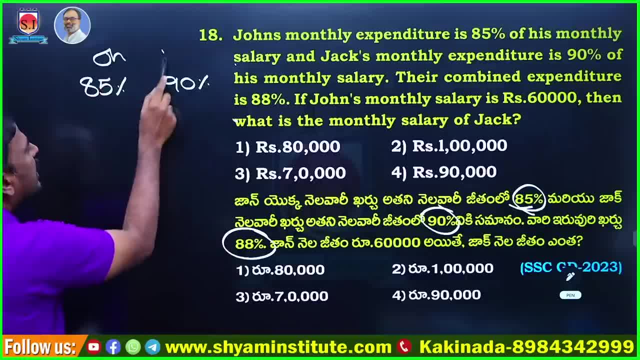 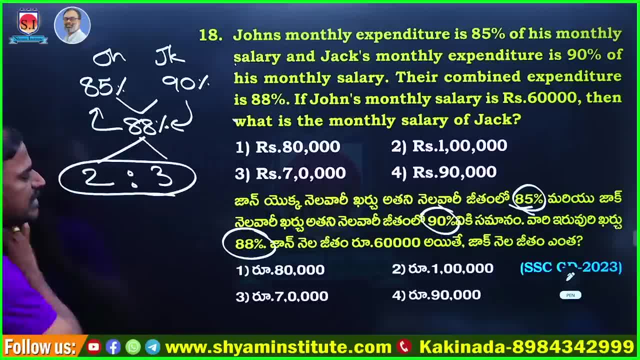 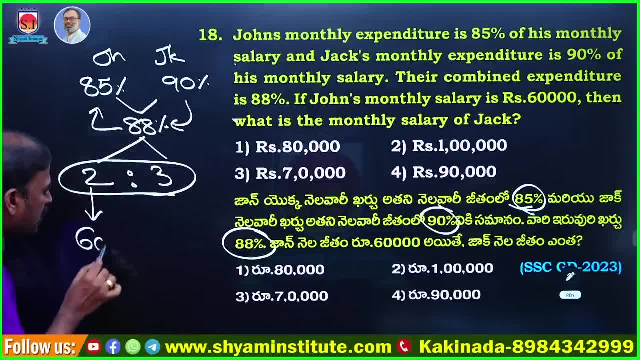 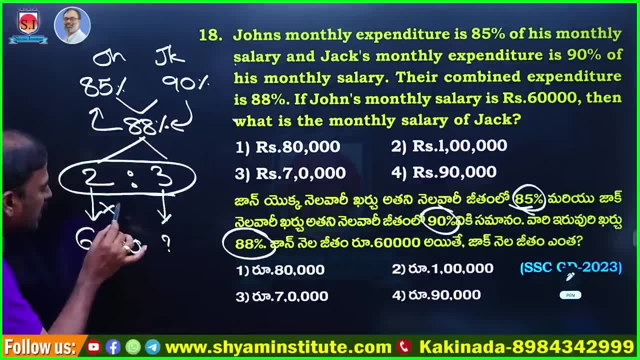 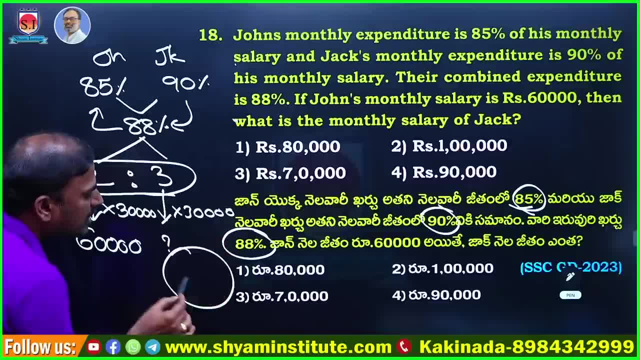 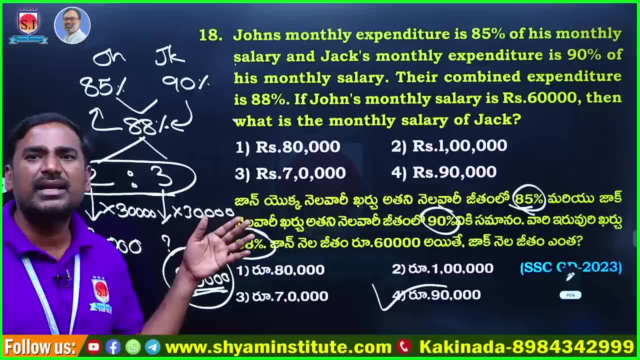 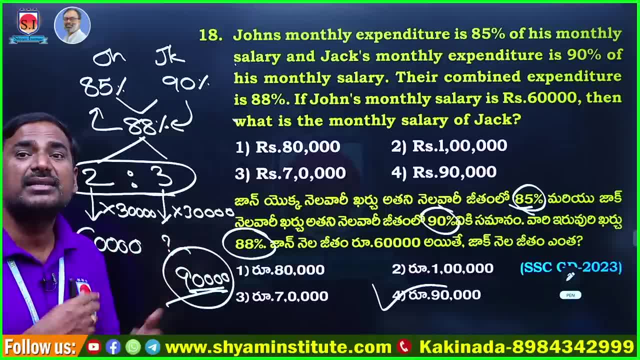 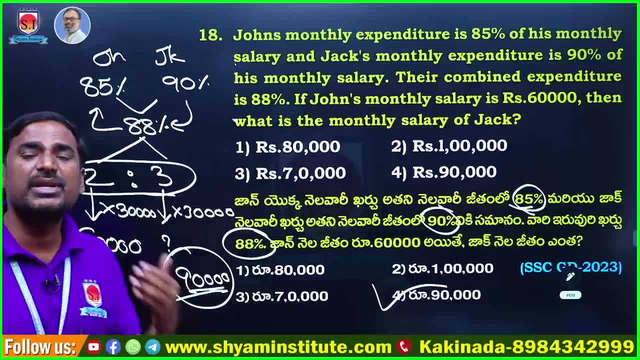 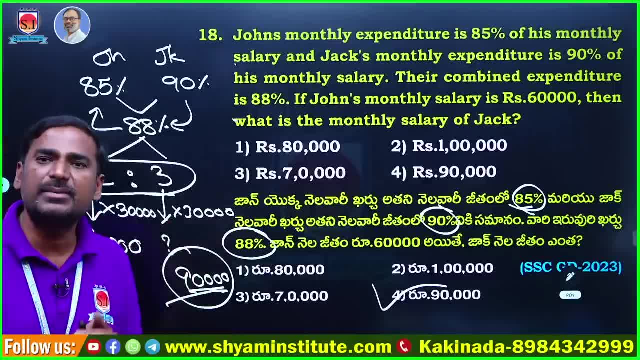 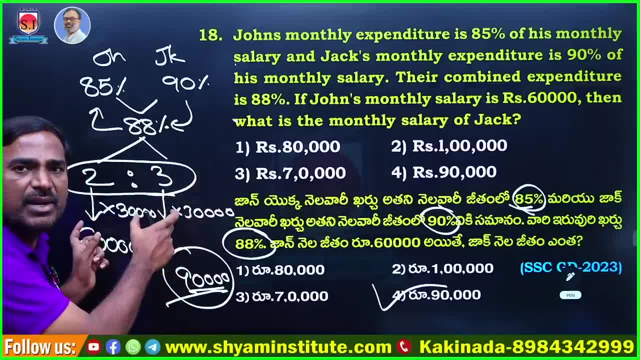 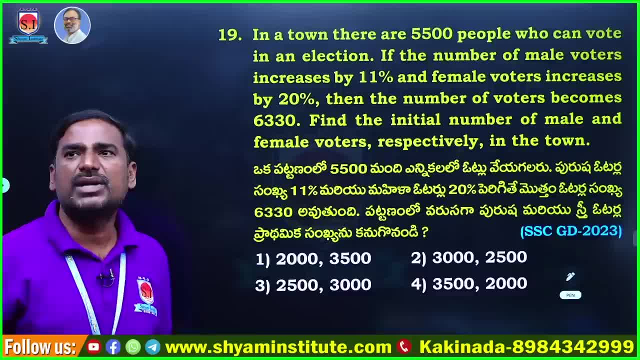 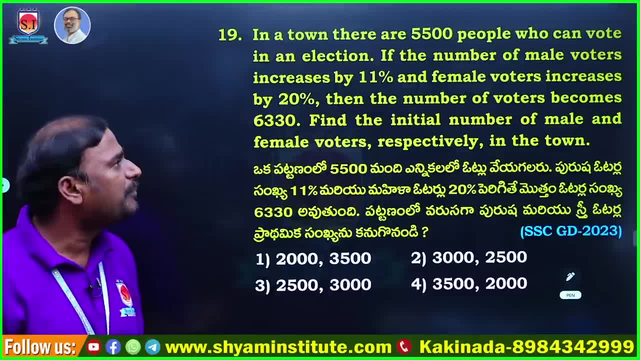 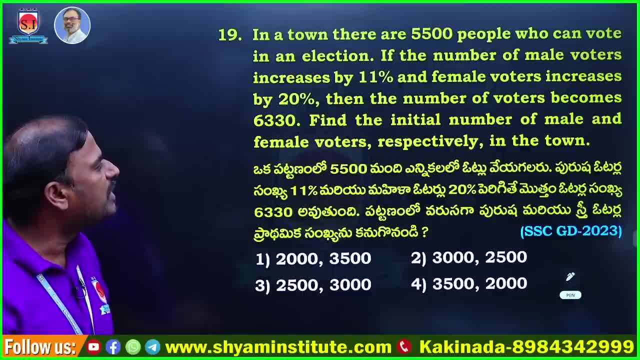 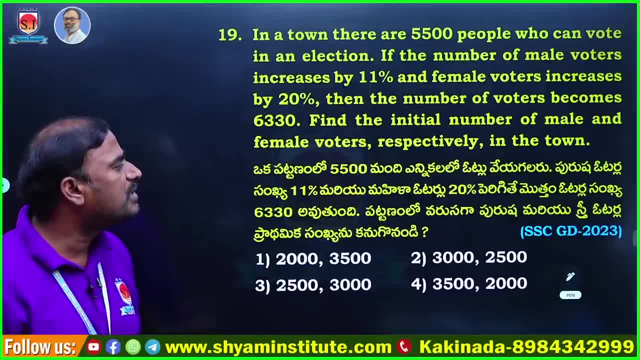 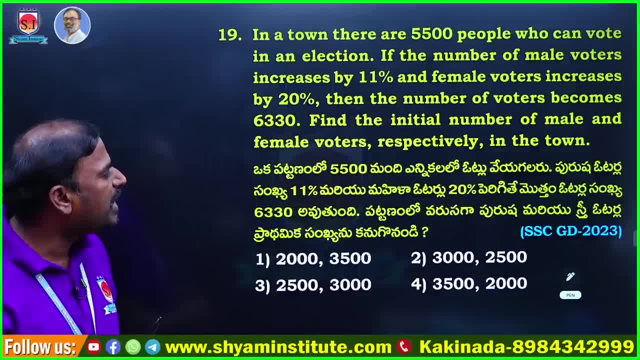 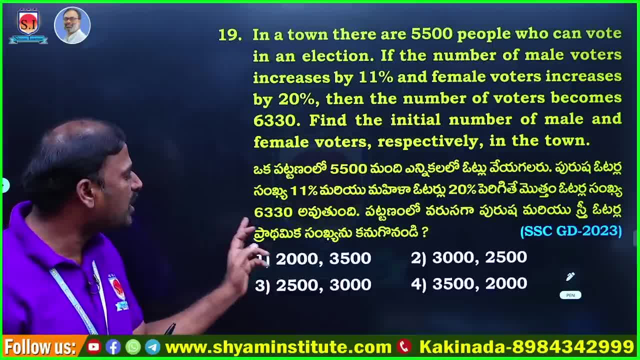 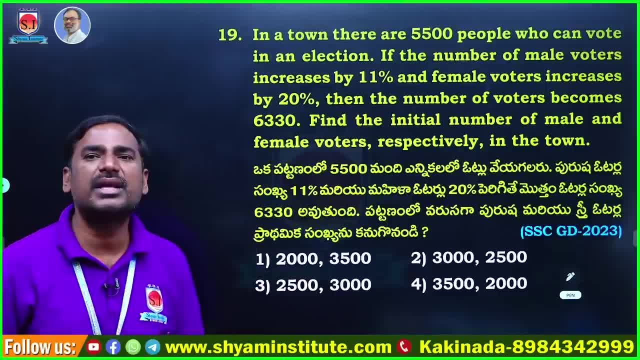 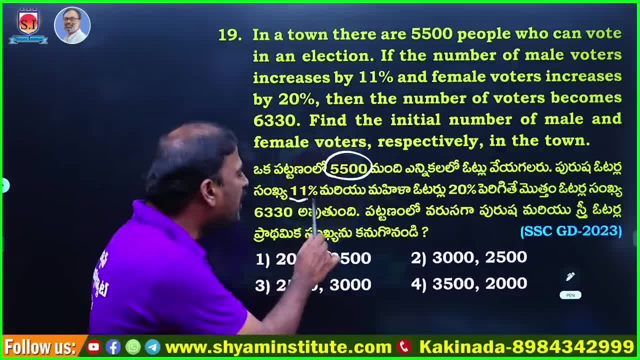 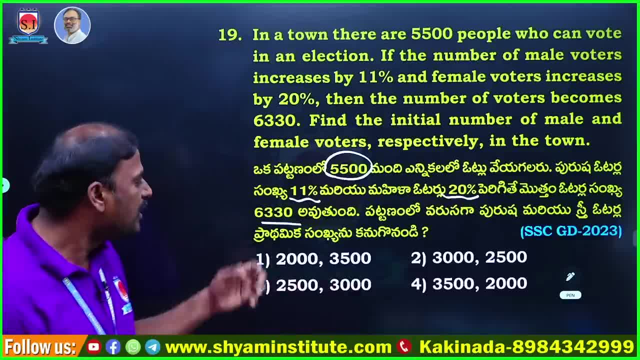 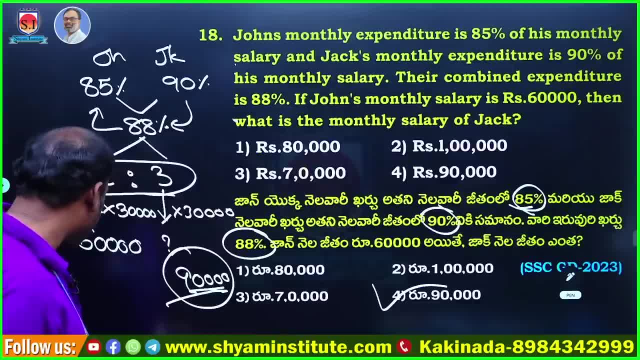 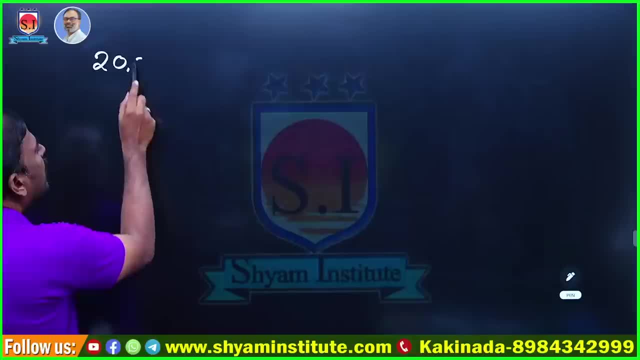 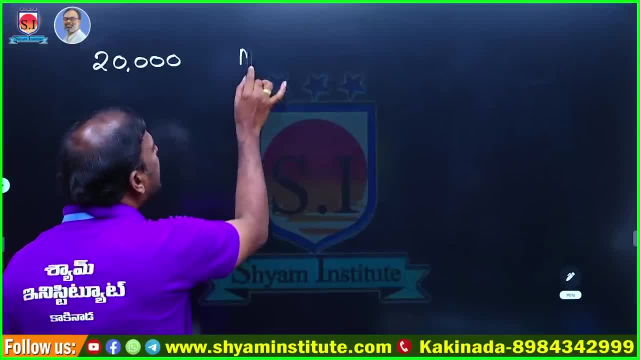 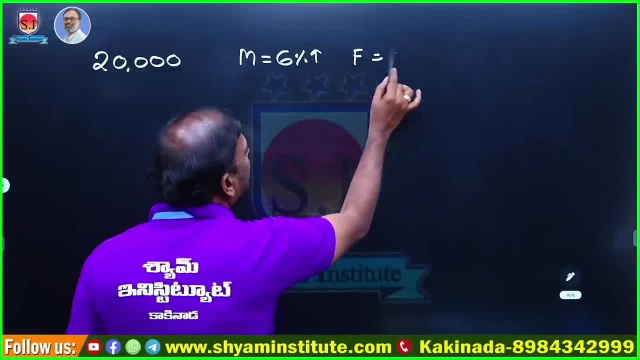 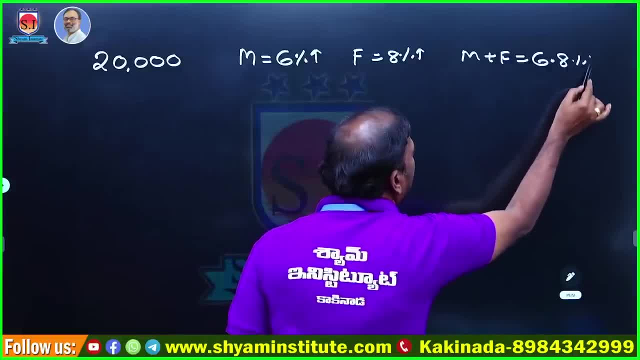 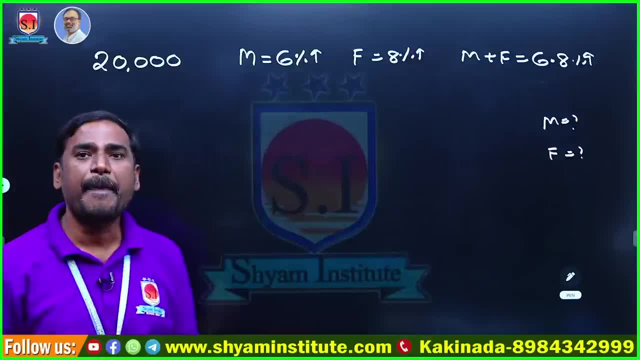 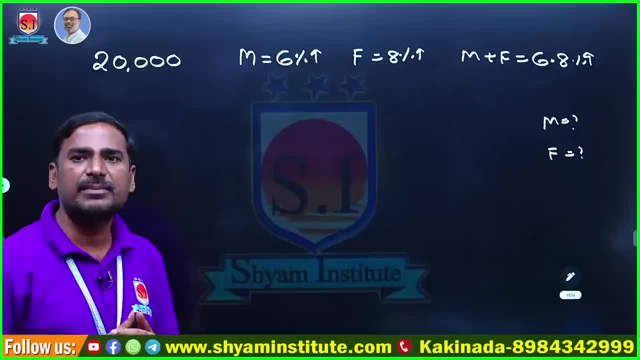 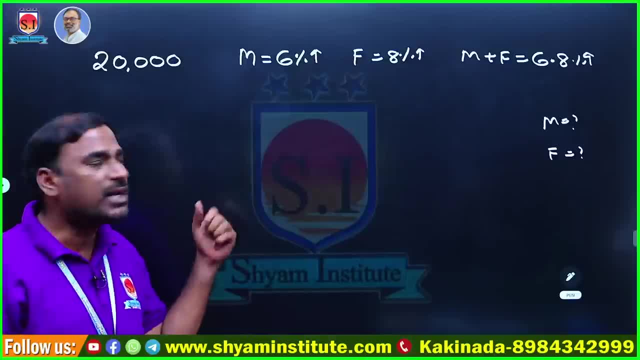 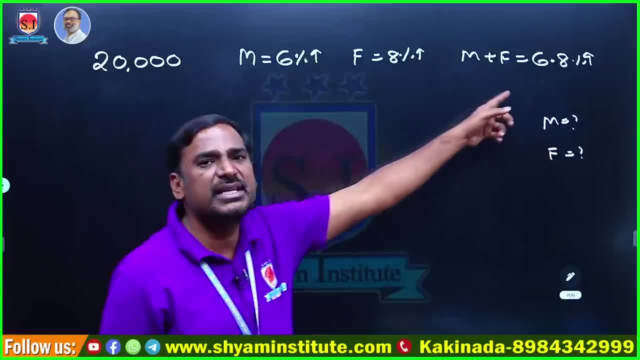 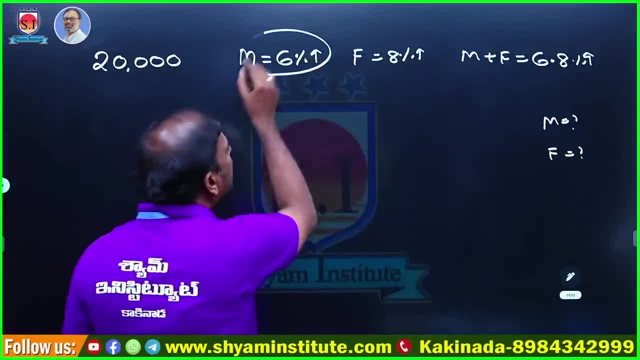 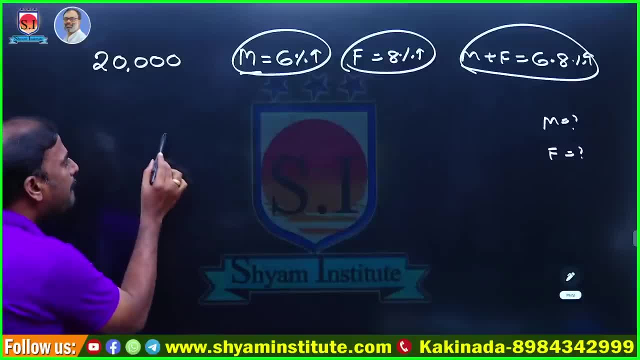 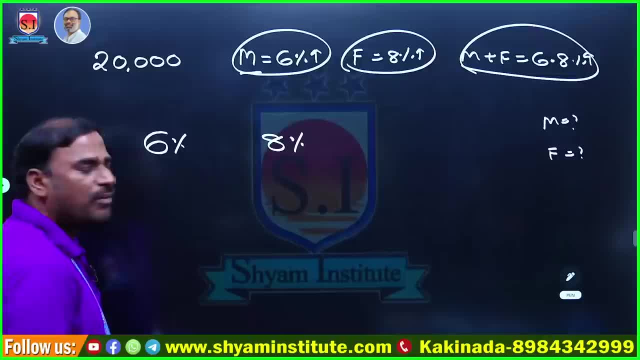 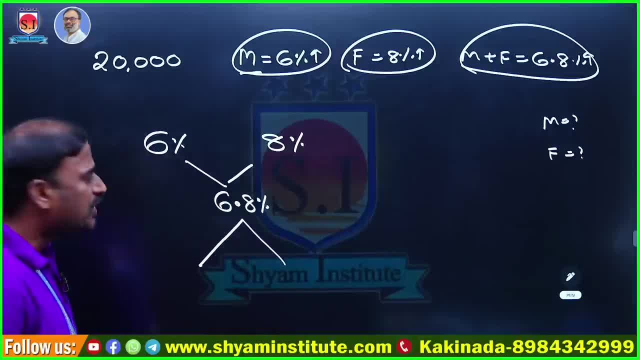 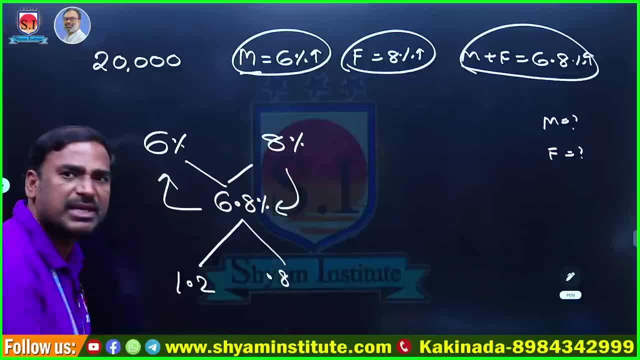 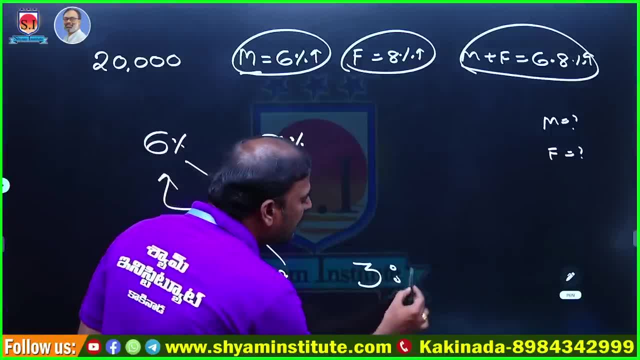 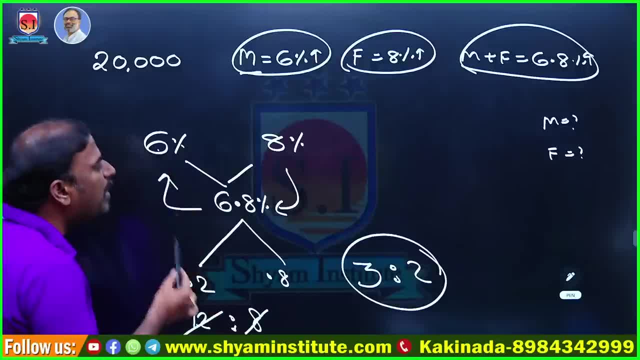 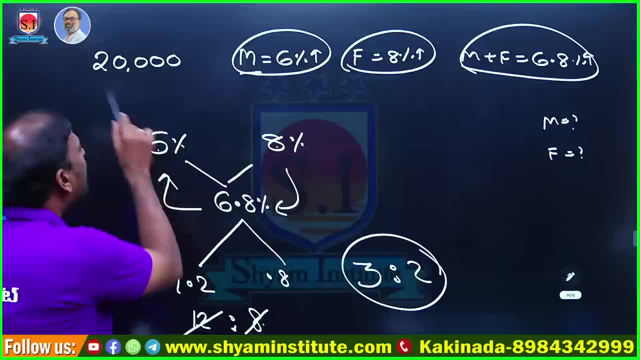 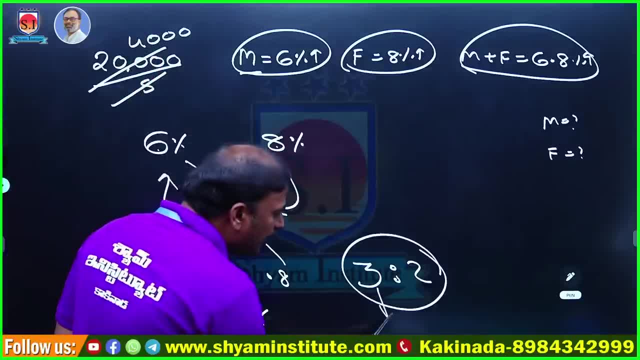 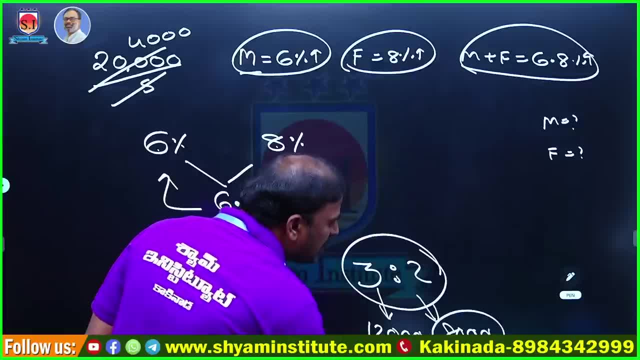 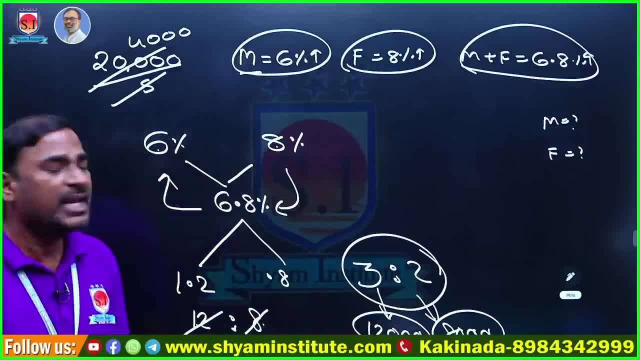 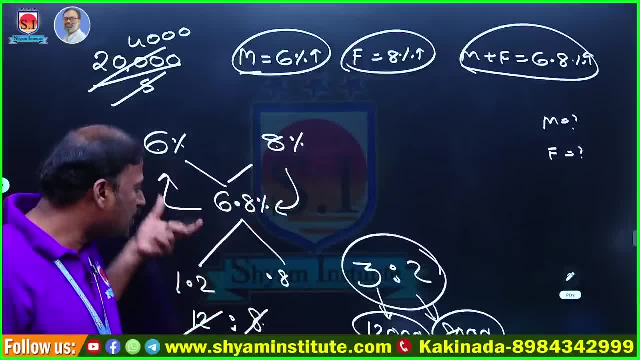 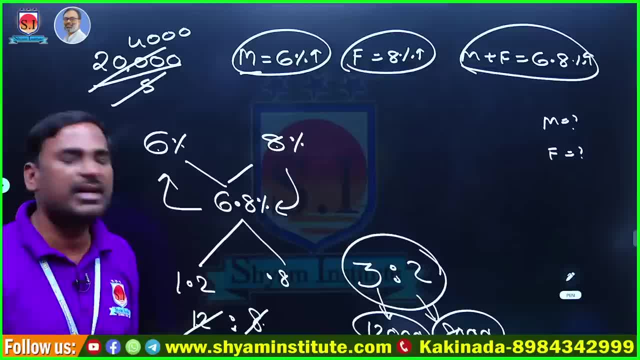 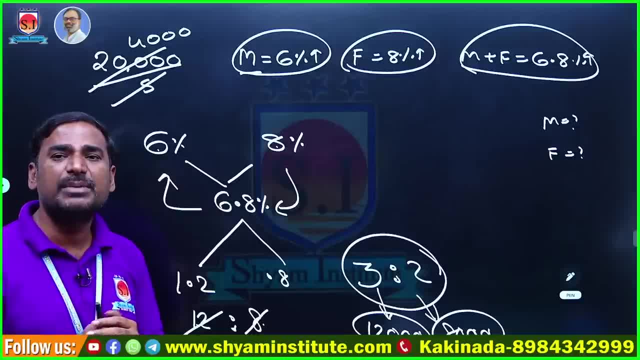 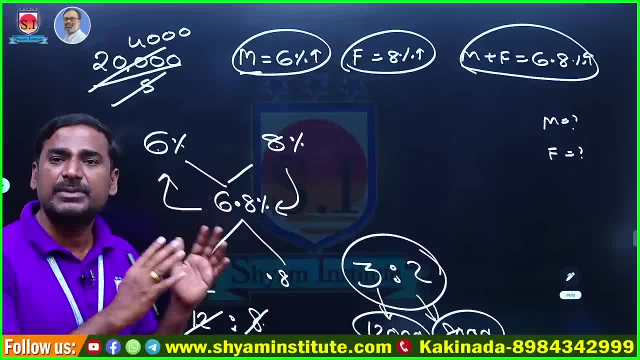 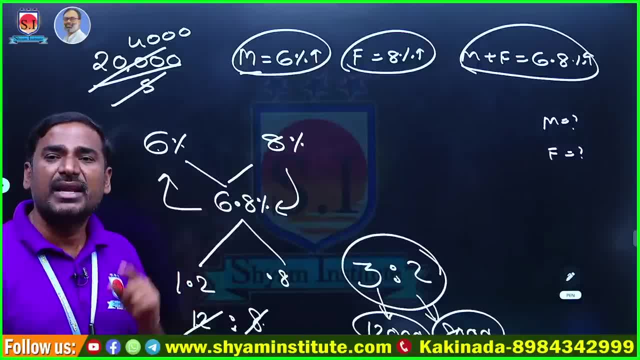 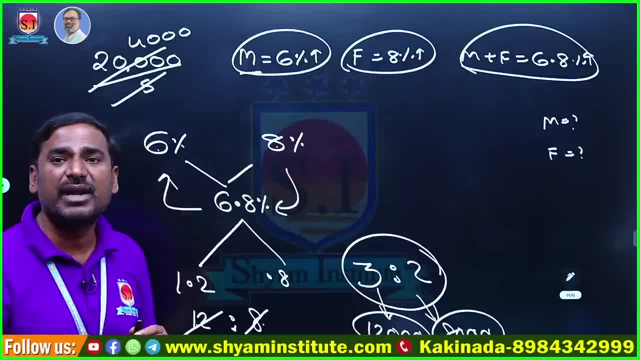 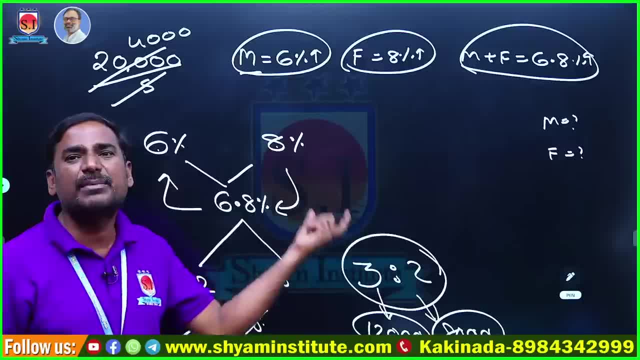 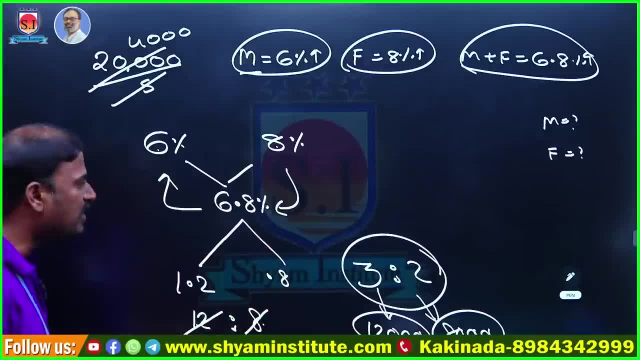 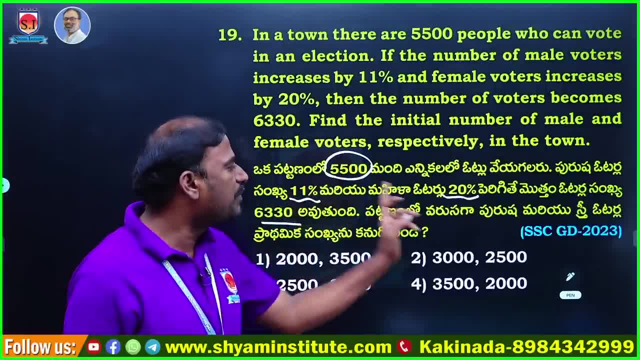 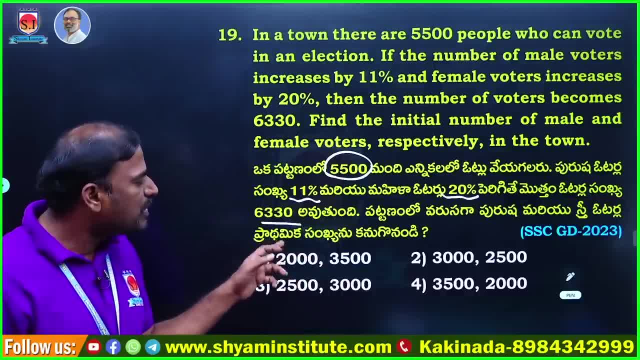 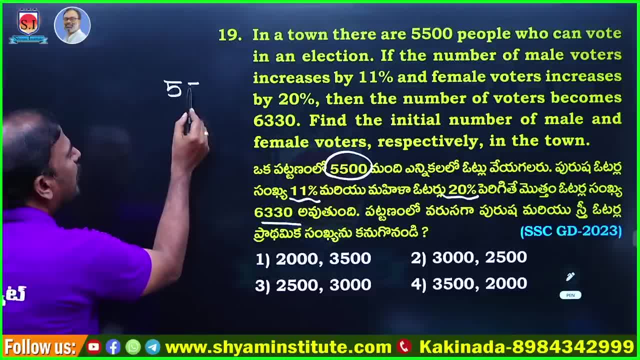 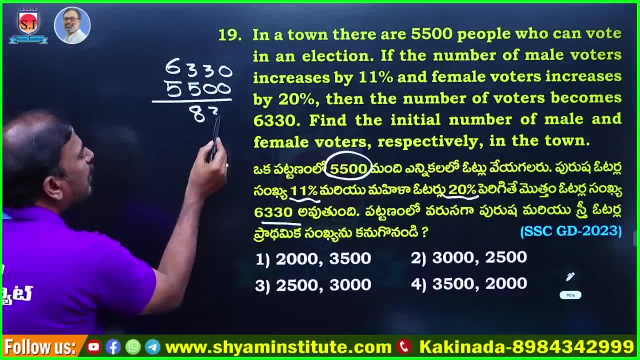 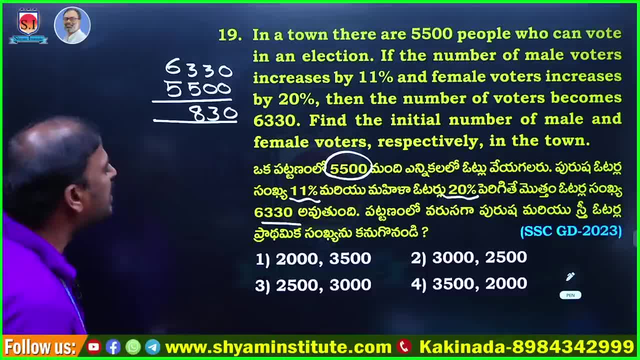 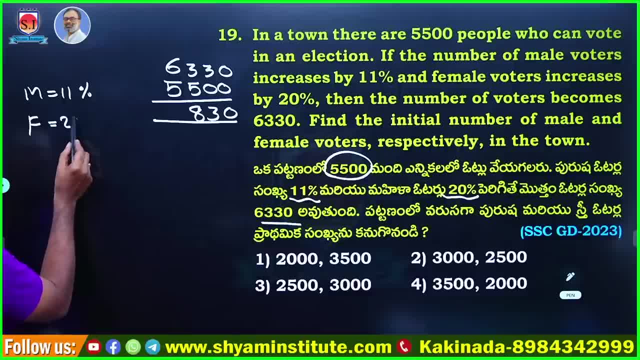 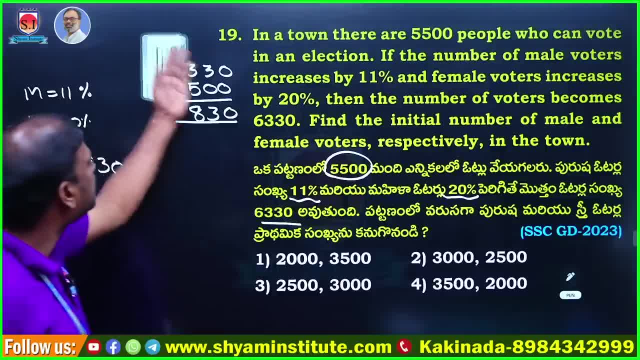 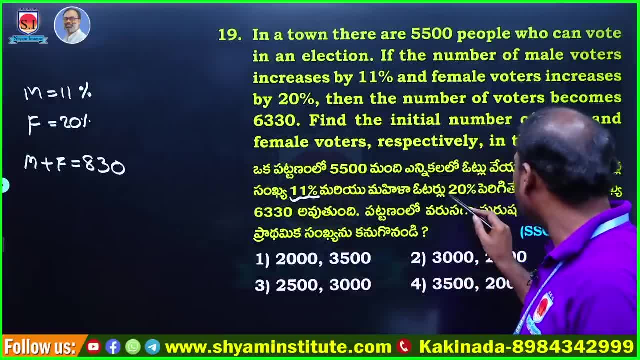 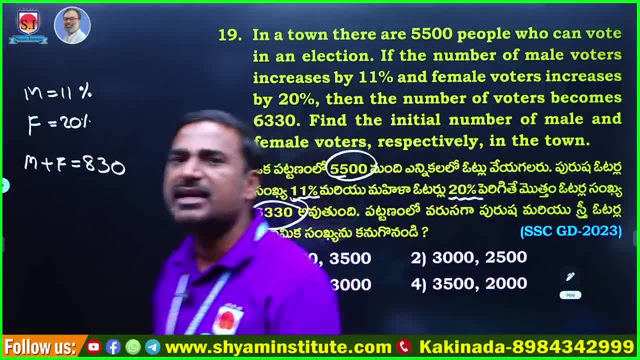 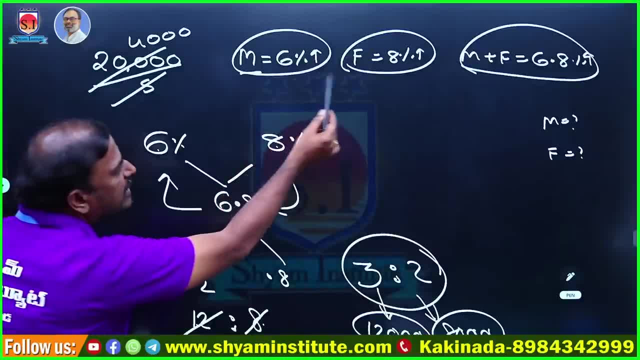 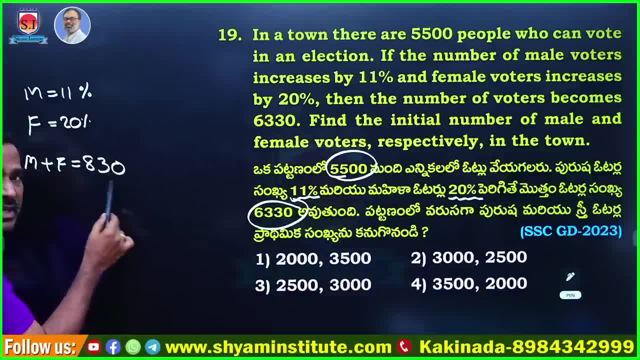 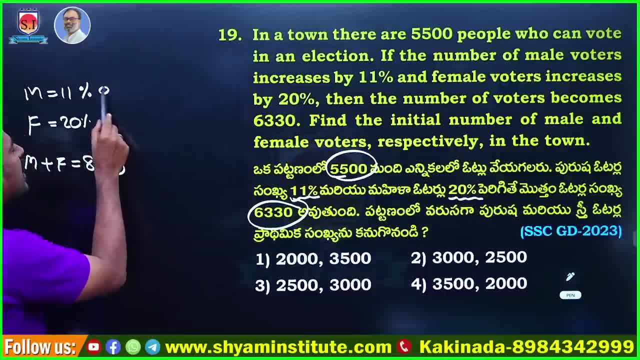 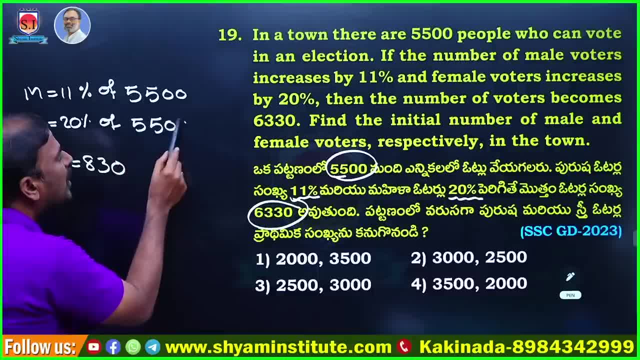 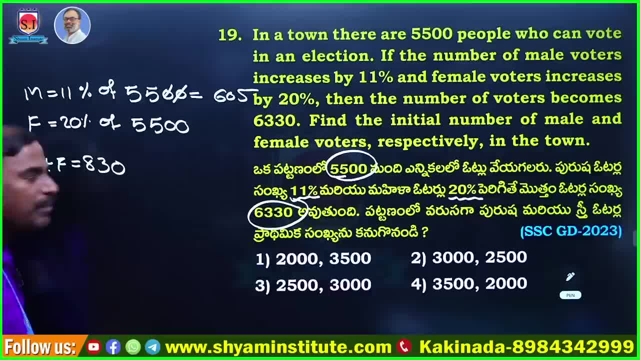 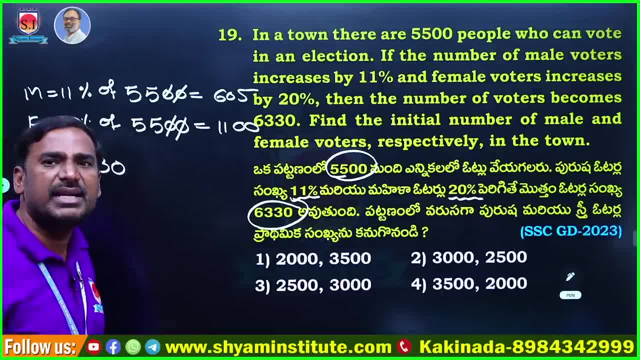 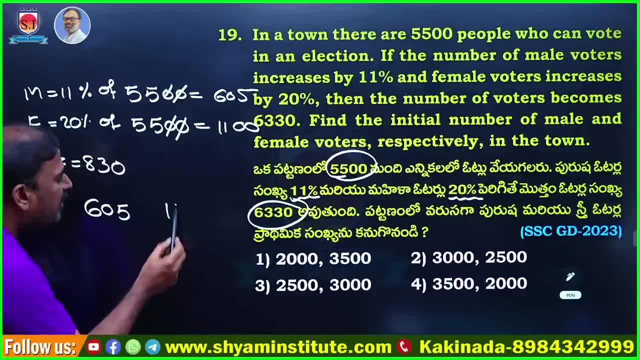 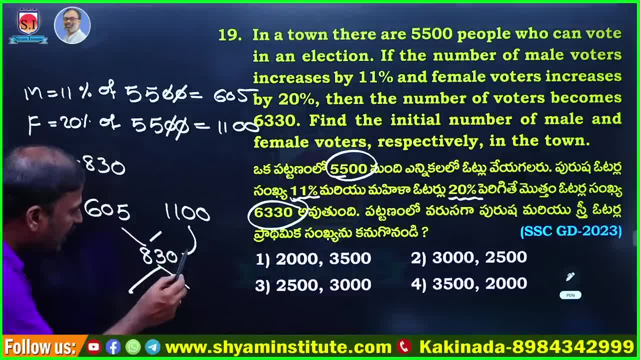 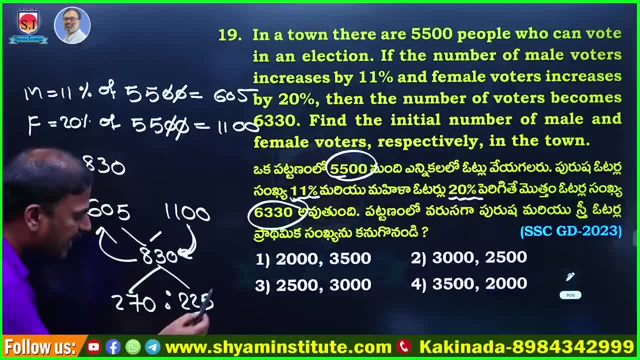 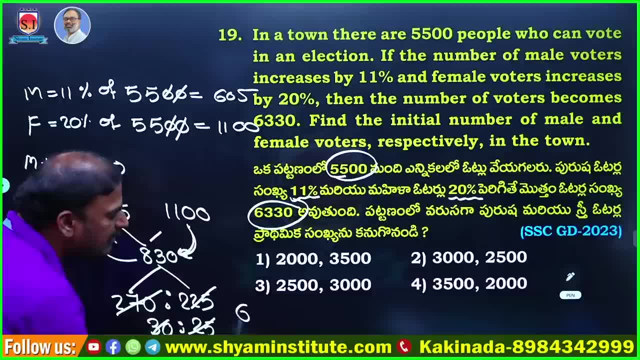 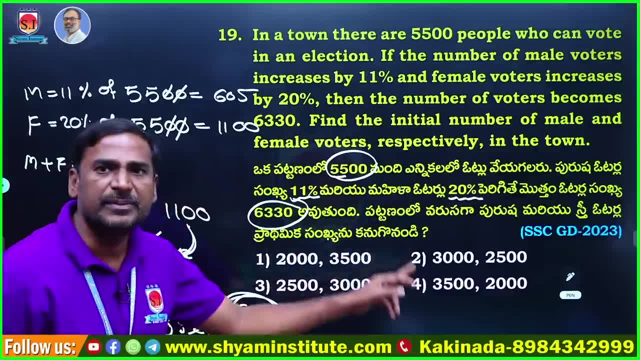 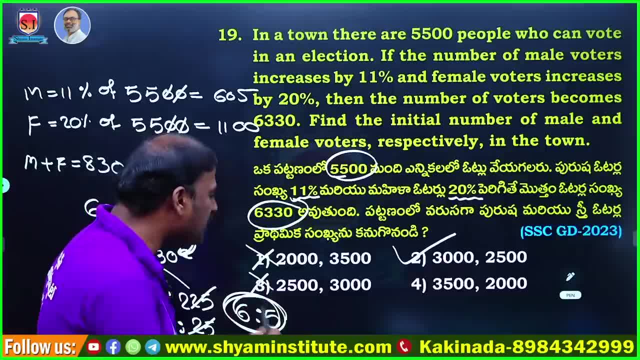 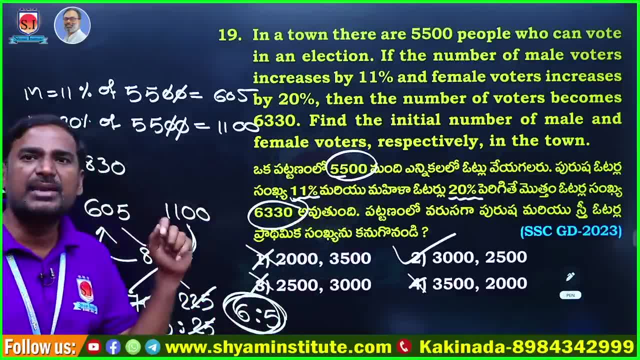 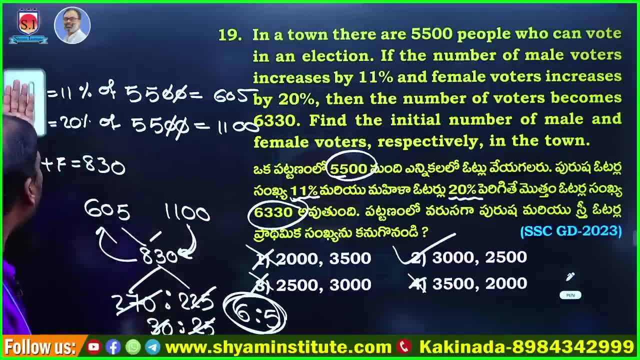 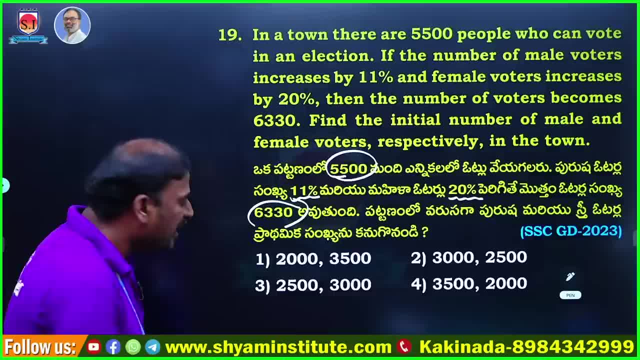 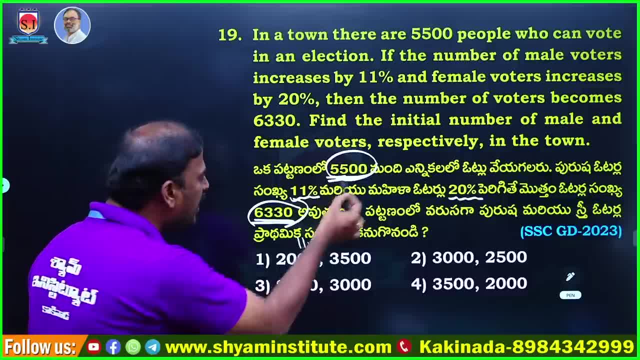 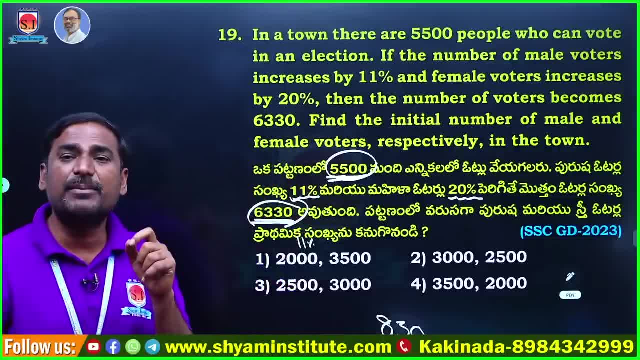 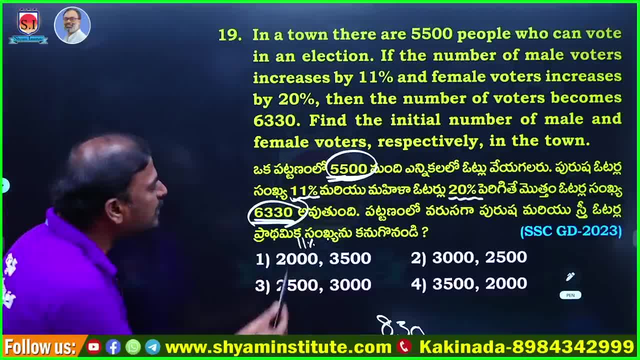 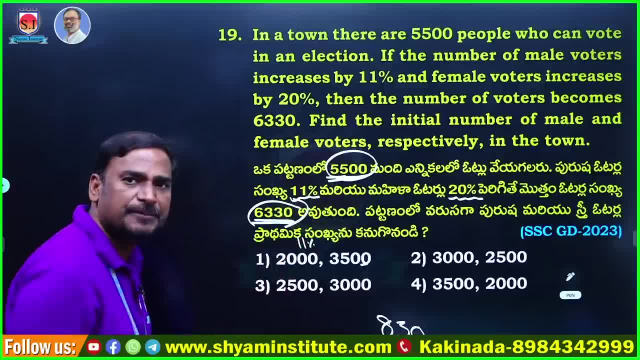 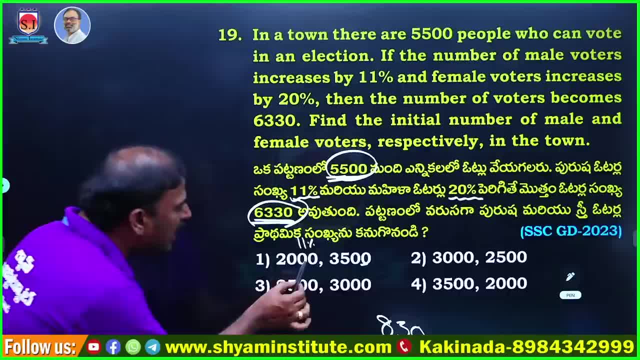 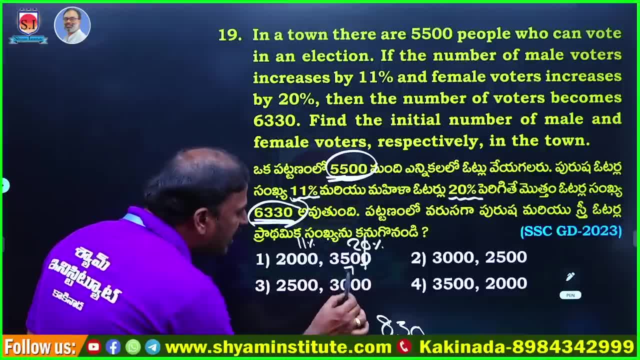 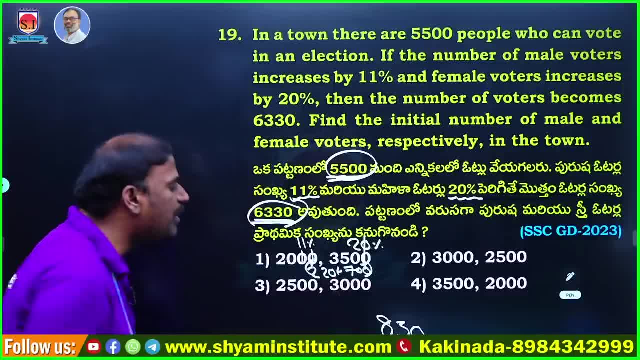 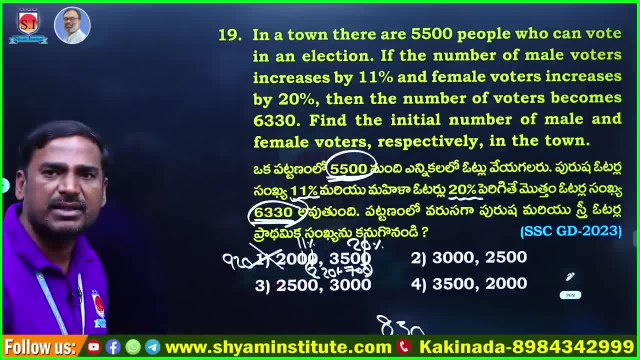 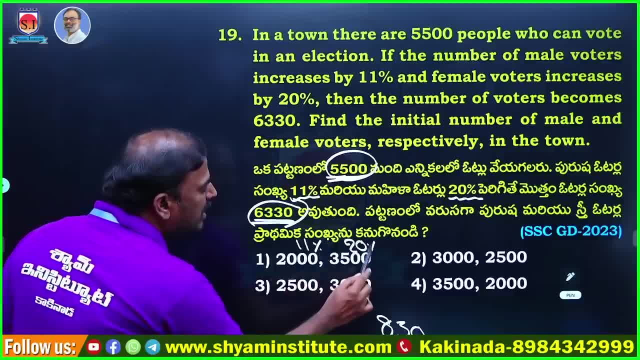 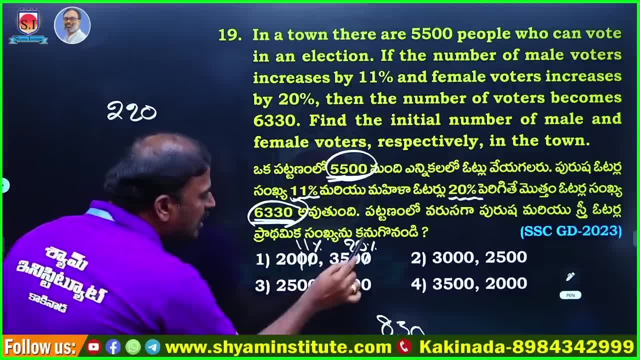 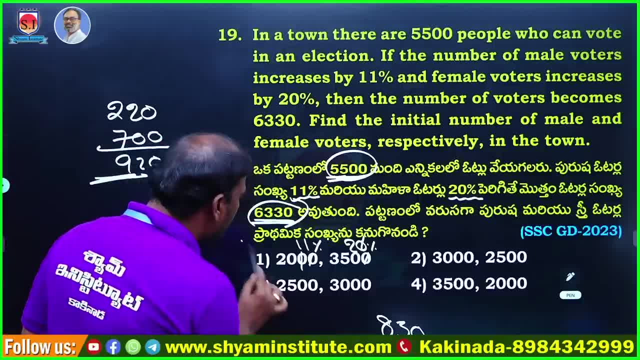 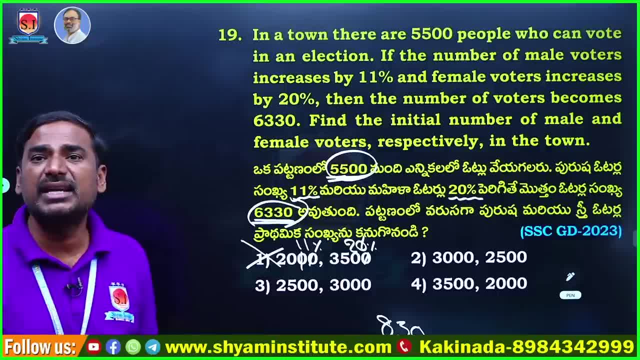 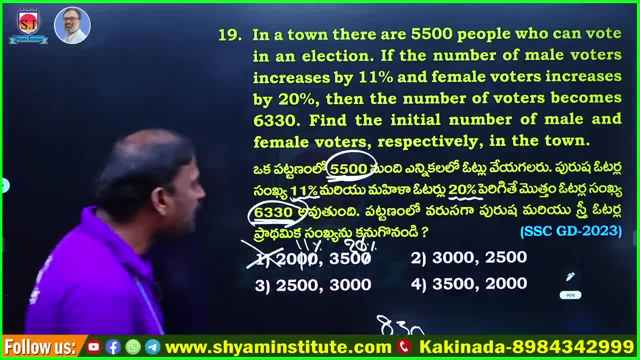 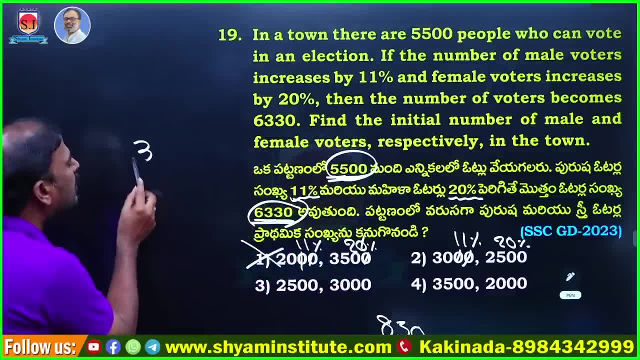 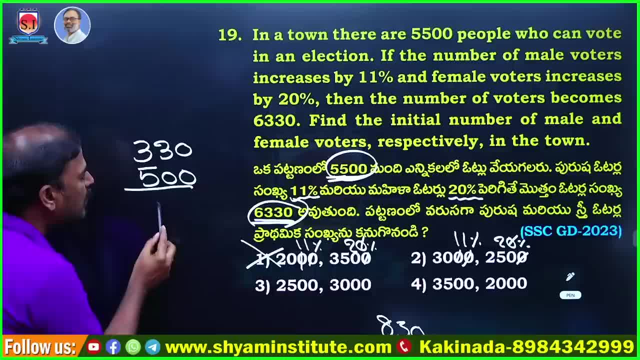 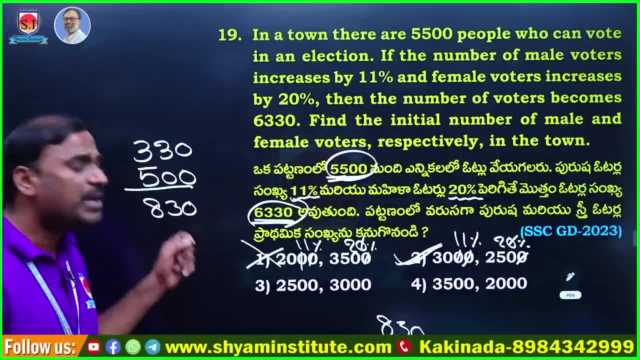 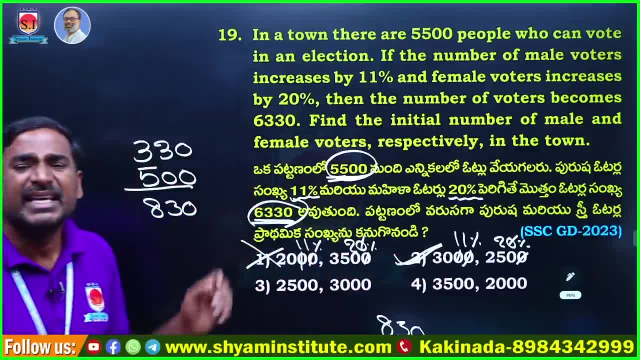 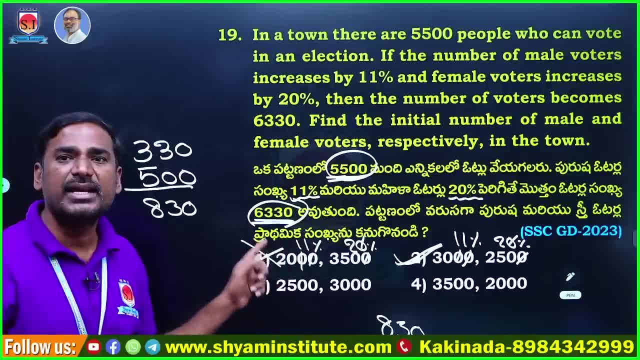 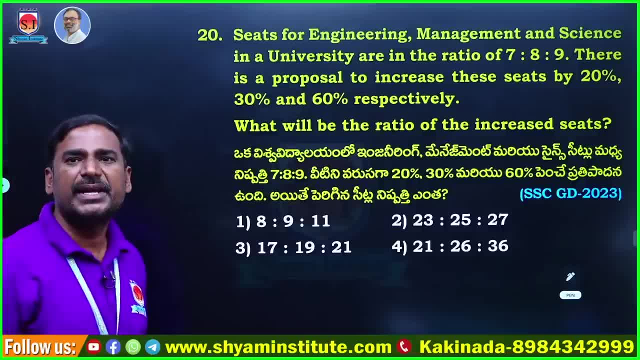 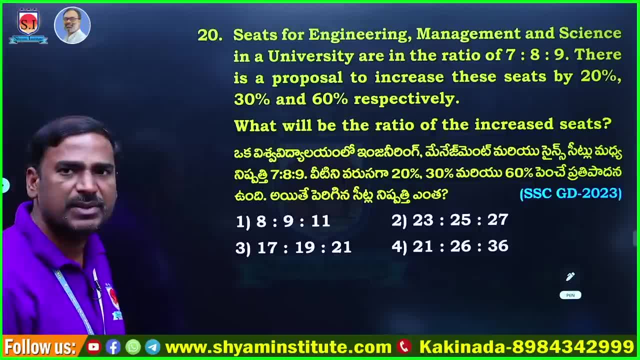 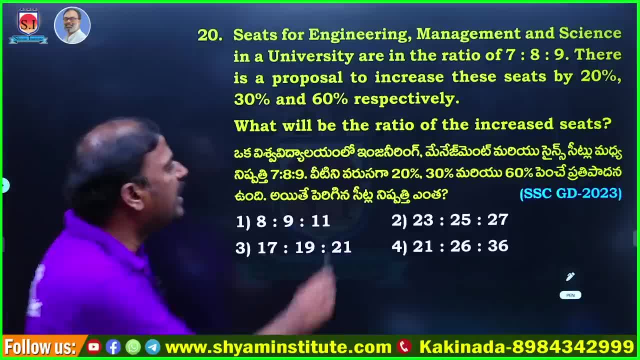 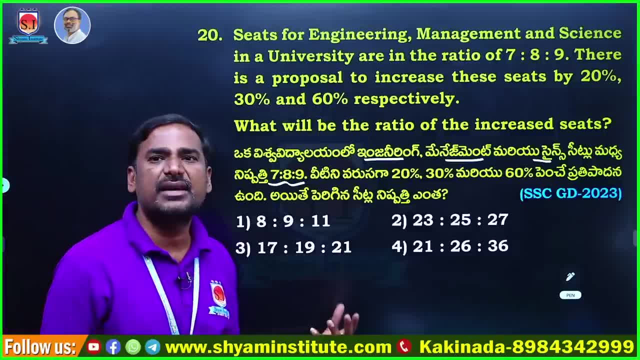 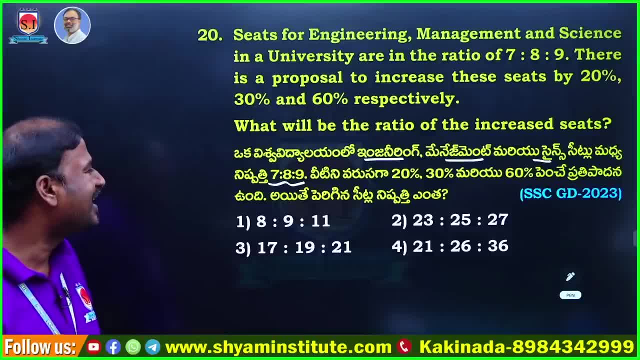 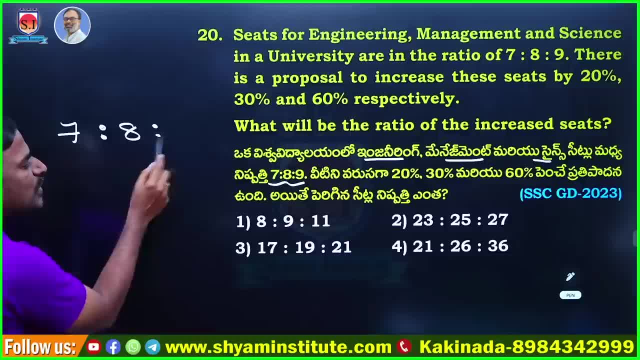 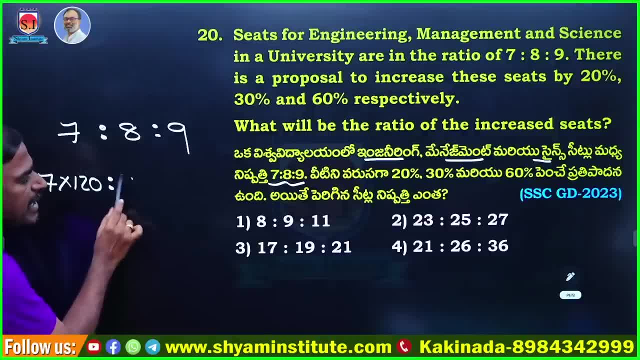 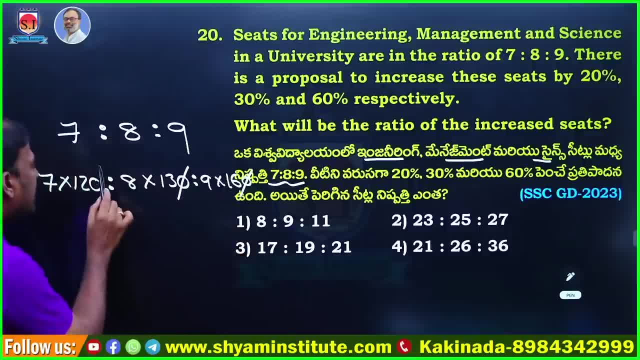 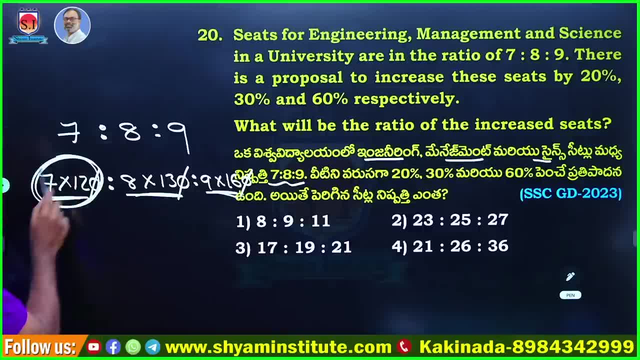 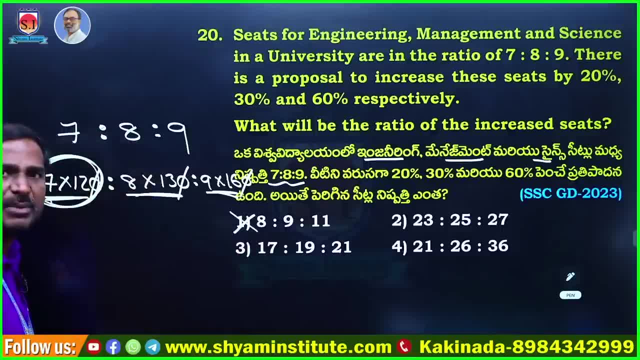 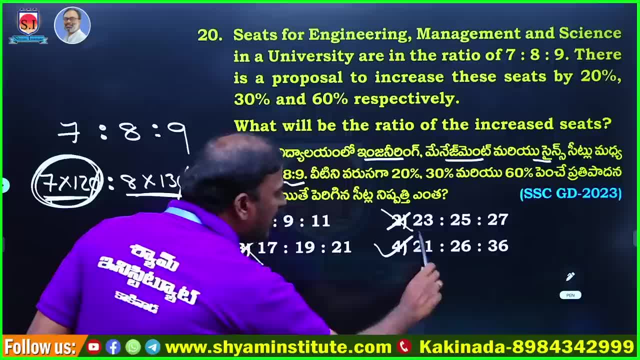 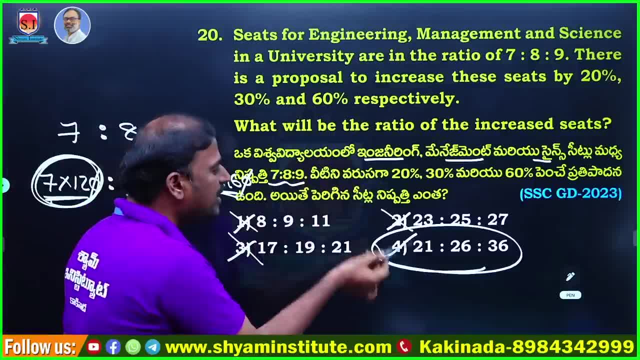 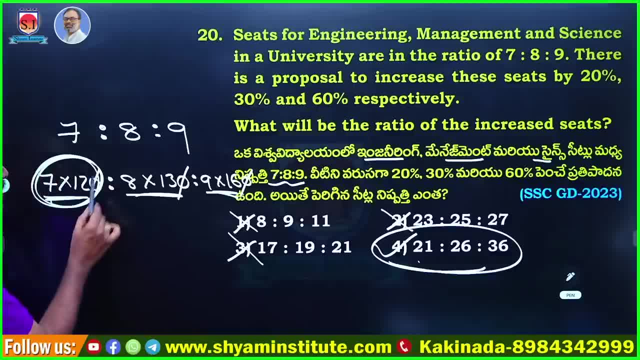 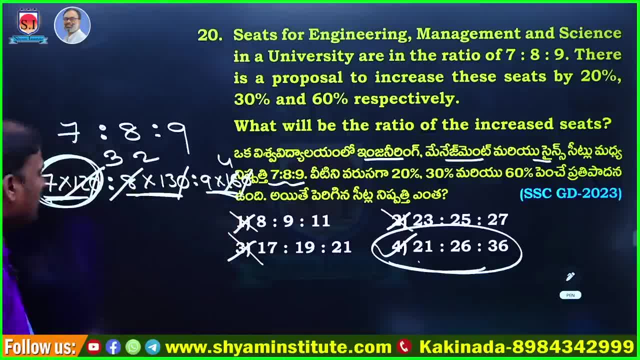 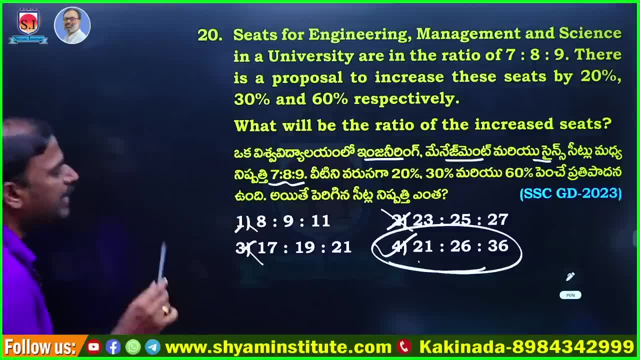 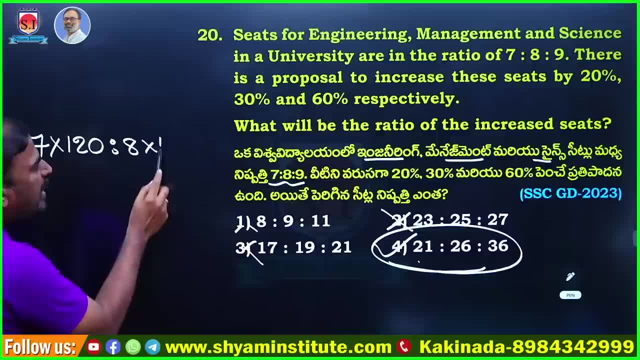 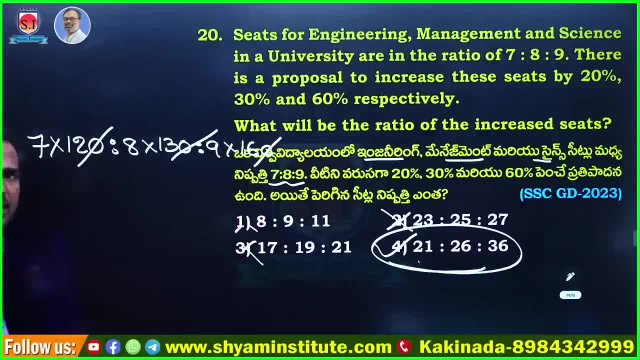 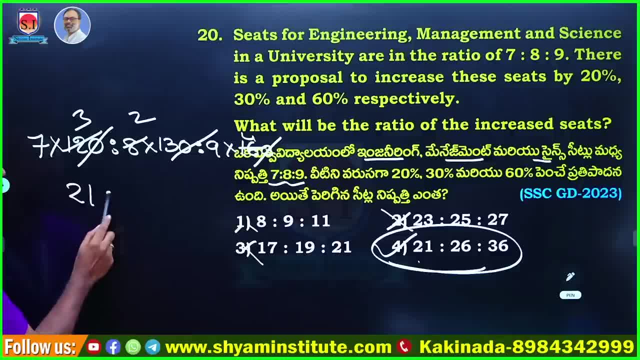 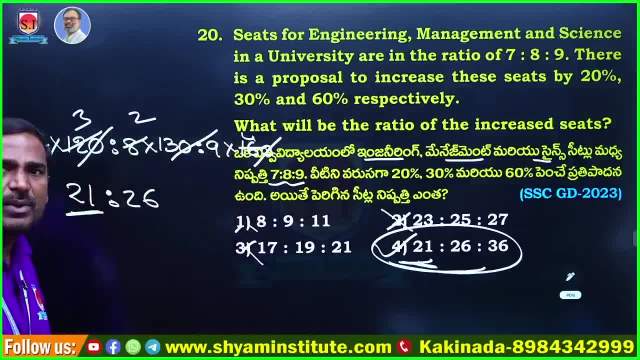 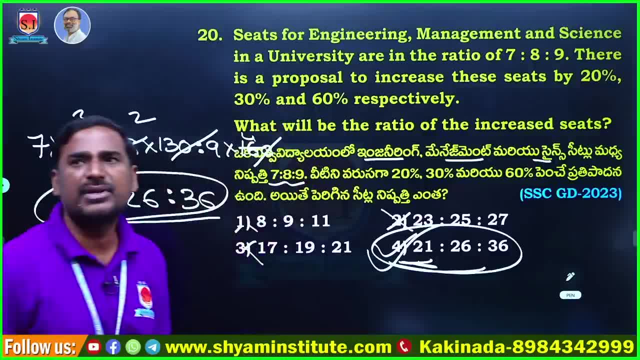 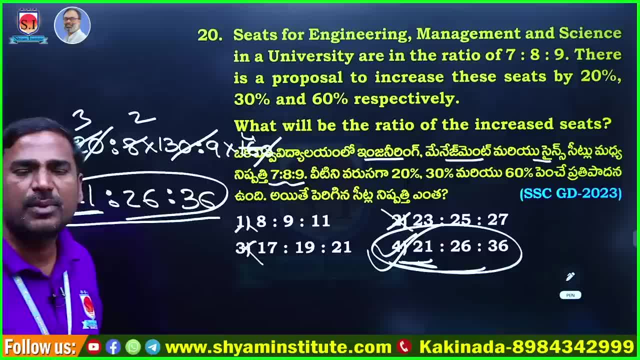 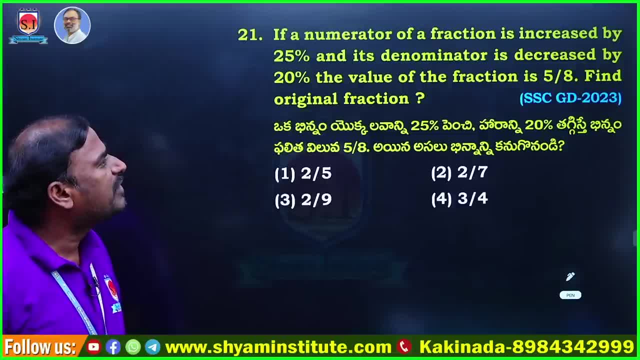 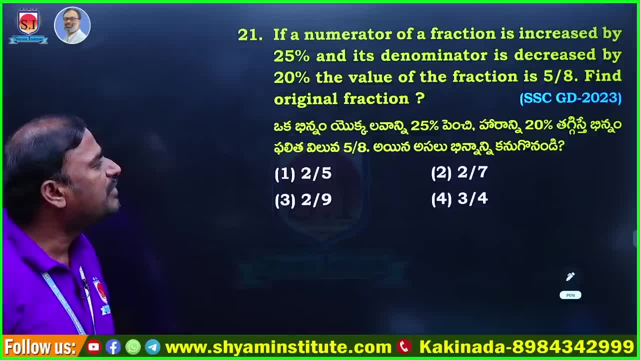 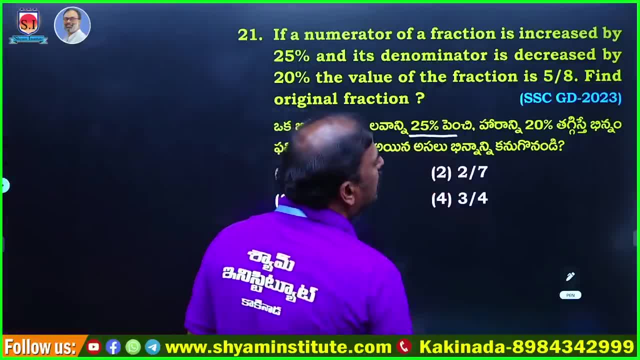 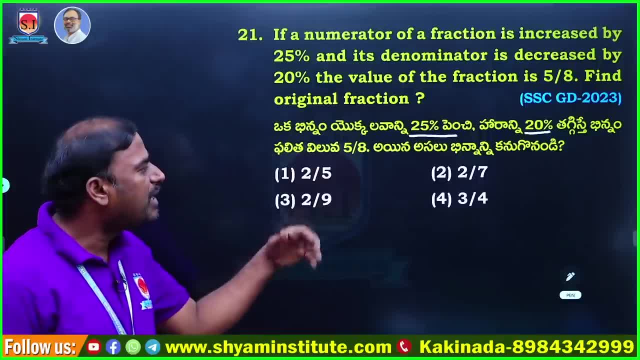 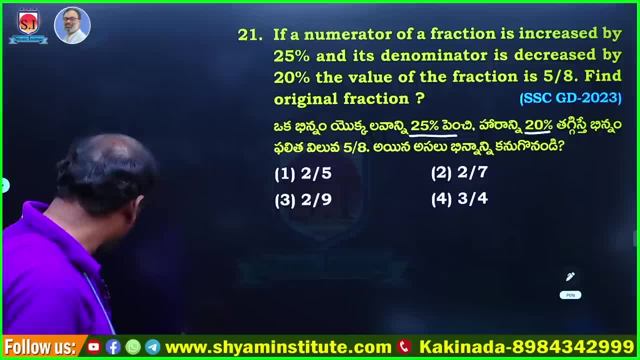 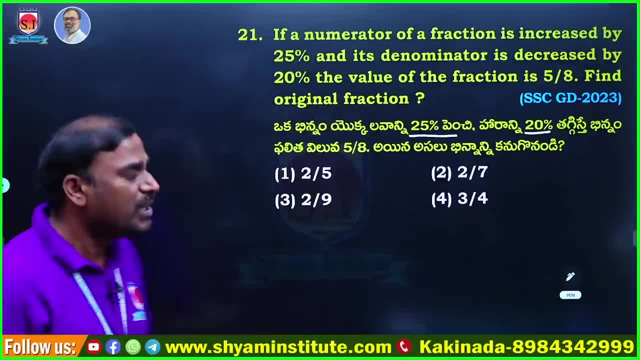 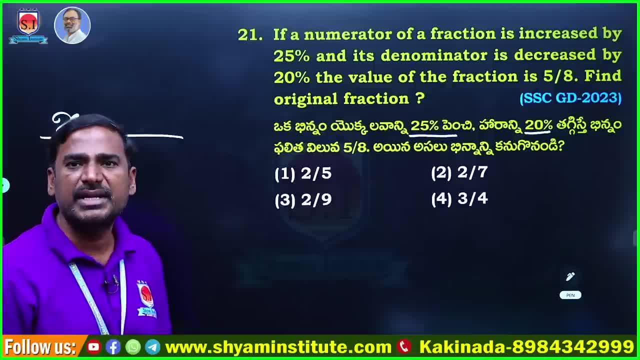 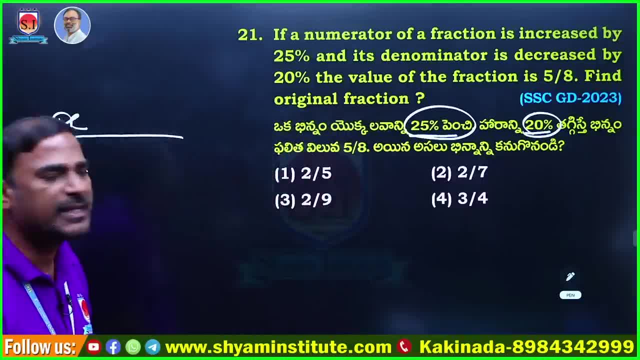 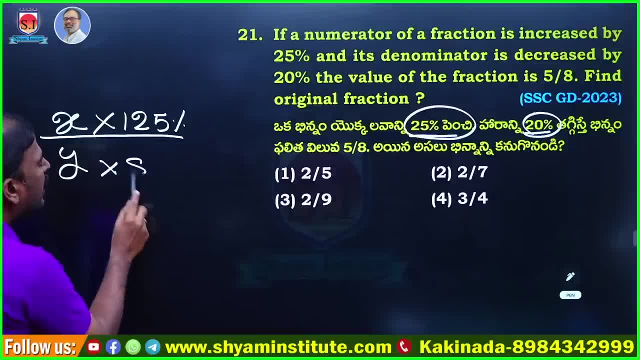 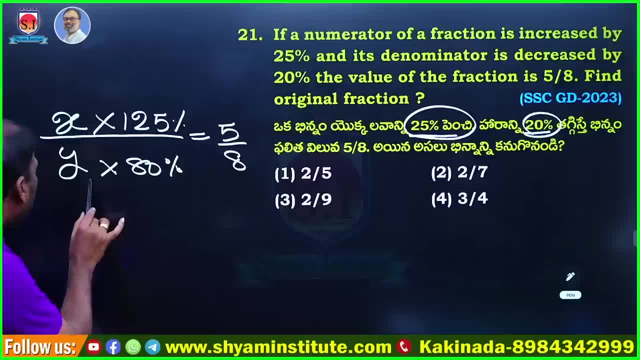 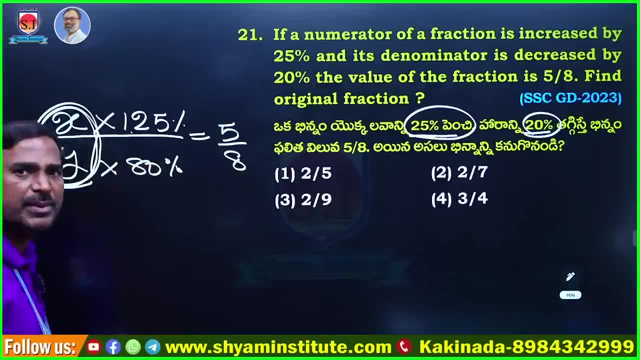 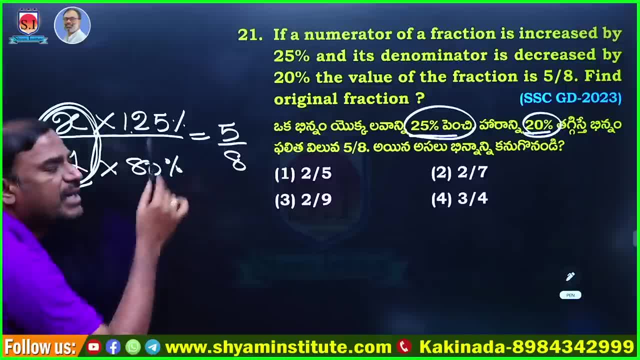 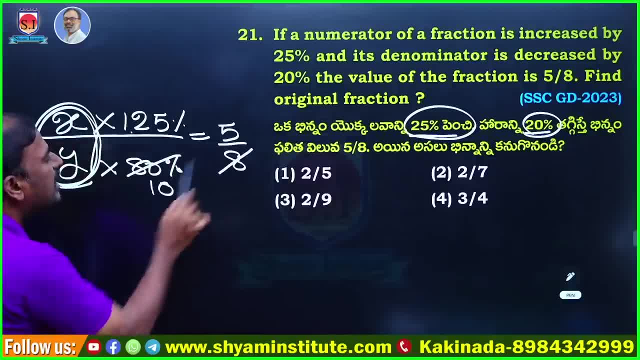 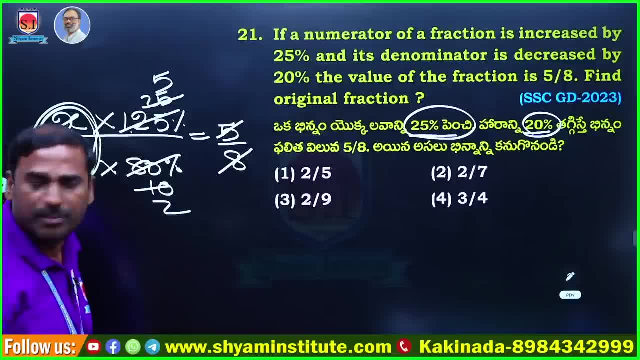 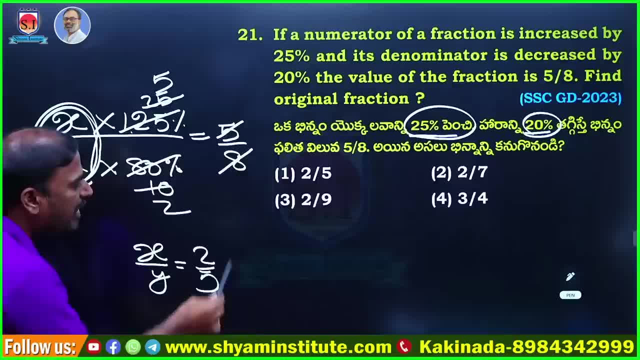 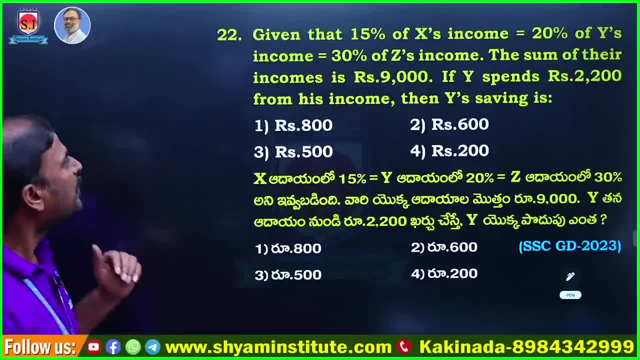 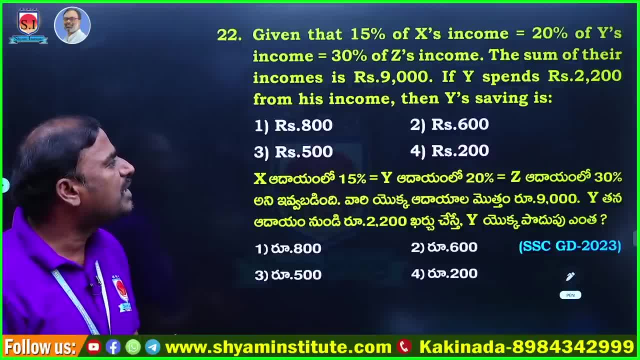 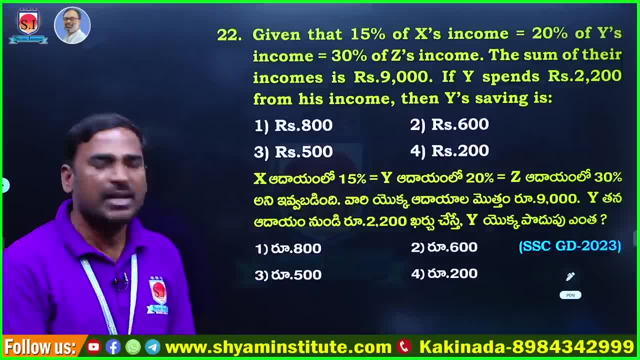 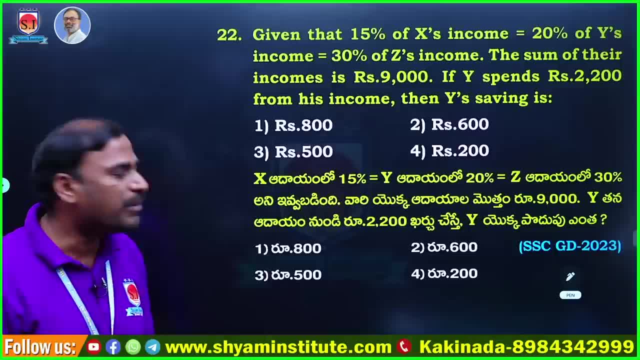 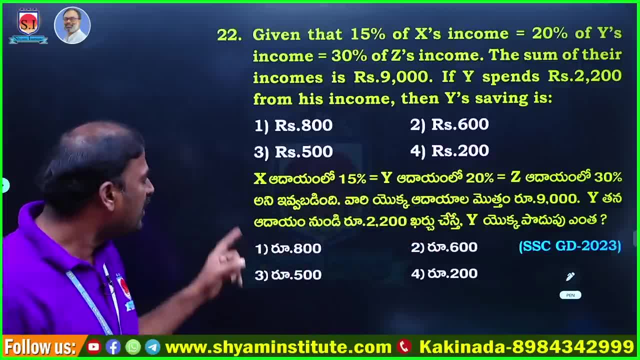 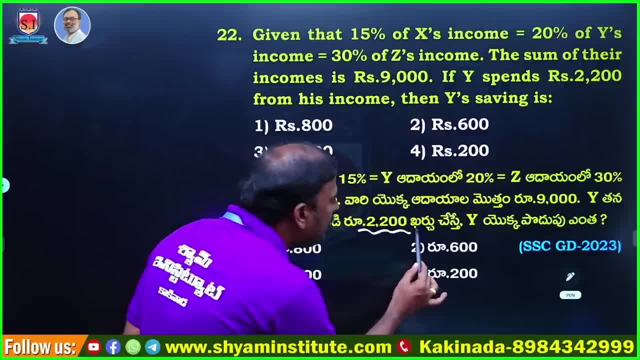 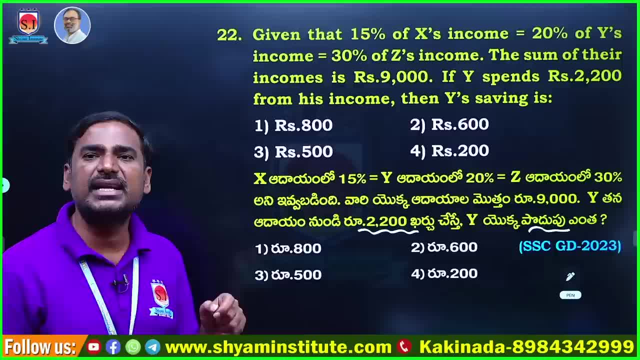 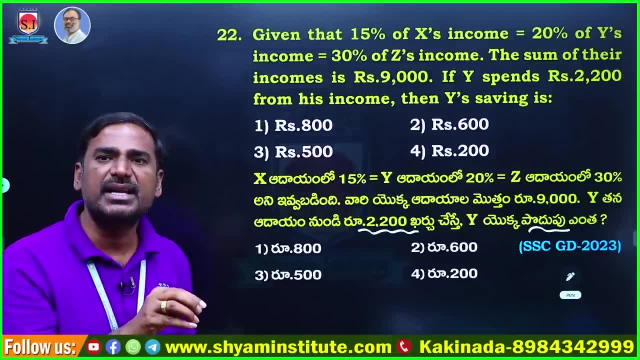 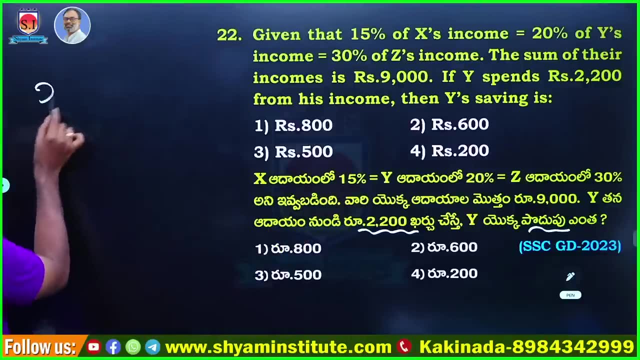 To find out the value of the compound that is required. we have to know the value of y. If we subtract y from the value, we get y. Now see what he gave. He said x is 15% in the compound. 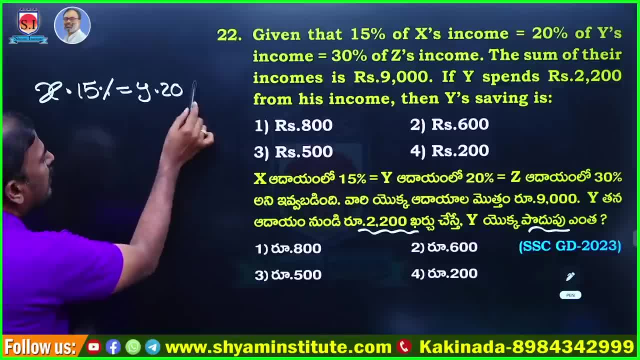 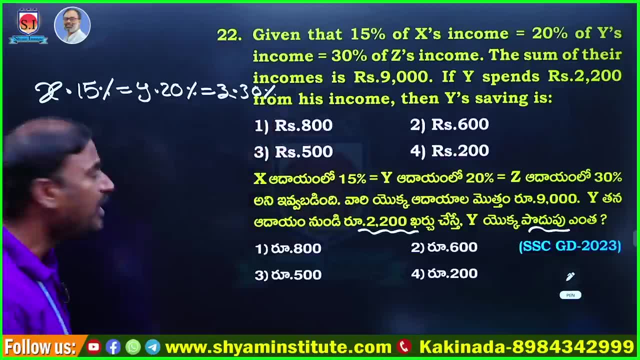 Also, y is 20%. in the compound, Z is equal to 30% of the half of X. All these are the same. The half of X is 15%, The half of Y is 20%, The half of Z is 30%. 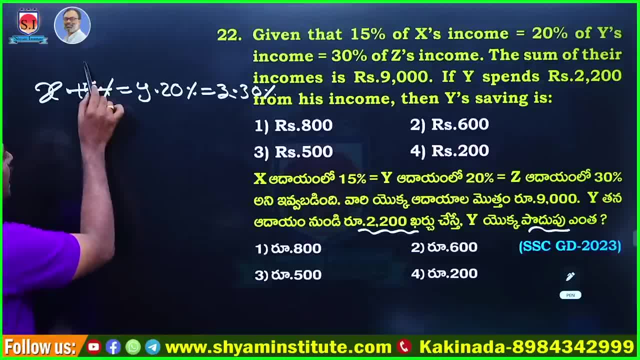 All these are the same. Think about it: 5 and 3 are cancelled, 5 and 4 are cancelled, 5 and 6 are cancelled. So the condition here is 3X is equal to, 4Y is equal to. 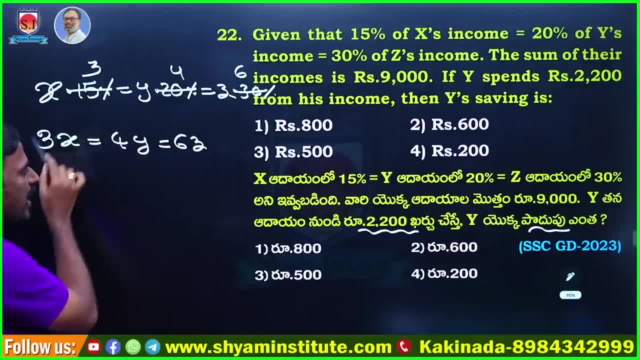 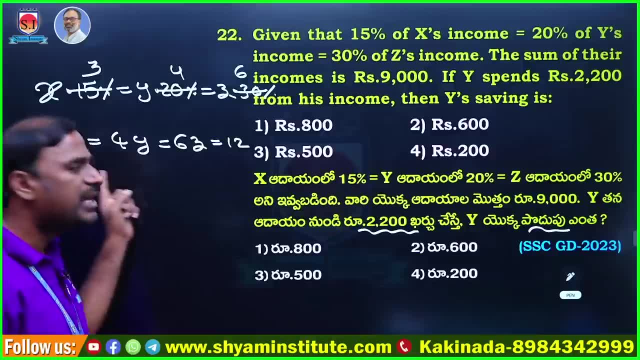 6Z. If you get mathematical condition like this, then take LCM. So if you get such equal condition like this, if you get such equal condition like this, if you get such equal condition like this, so in any concept or in any problem, 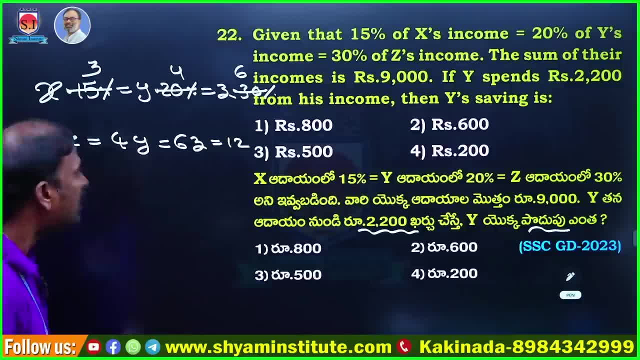 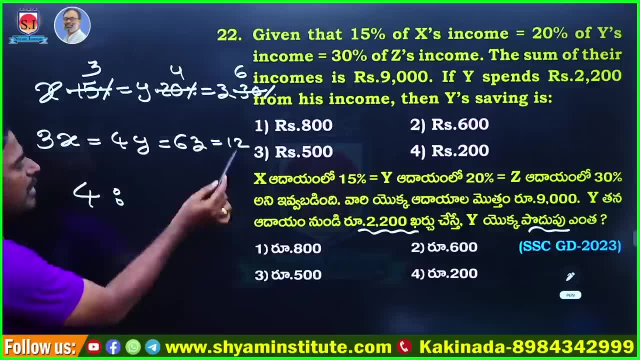 so directly you take LCM. So if 3X is 15%, then 1X is 3.4.. So how much is X? How much is X? 4.. So 4Y is 12.. 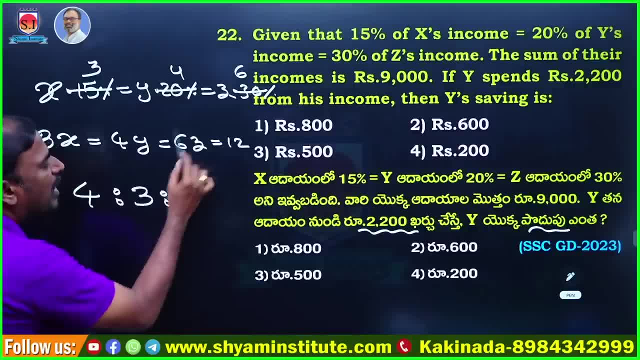 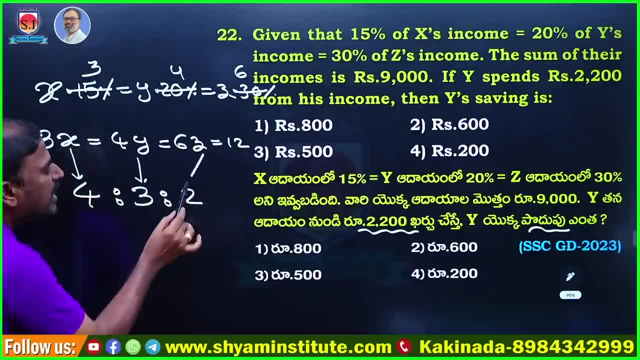 So how much is Y? 4 and 3 is equal to 12.. 6 and Z is equal to 12. So 6 and 2 is equal to 12.. This is X, and Y and Z are different halves. 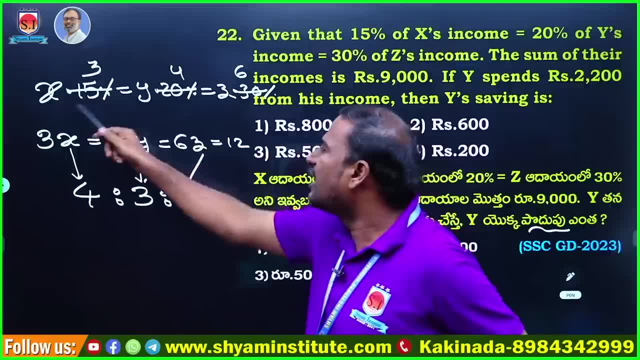 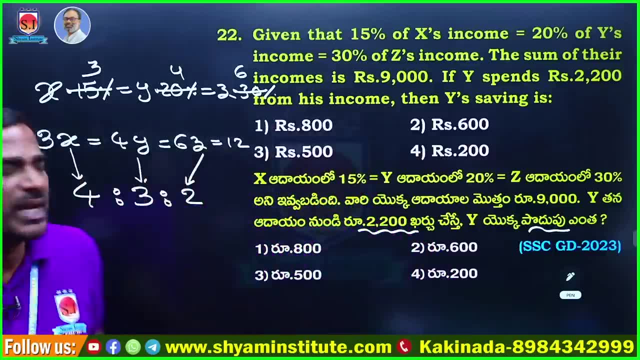 What I have taken here is: X is 15% of half, Y is 20% of half, Z is 30% of half. So they gave 9000 rupees to all halves. The other half was joined by Y. 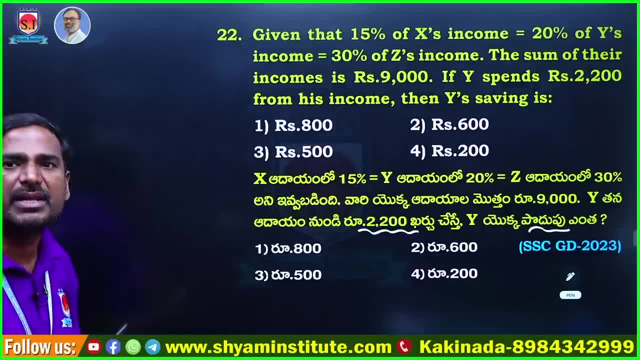 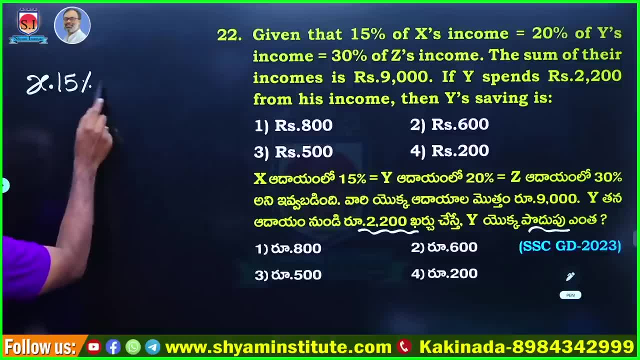 Y cover Y. If you spend Rs.2,200 from Rs.1,500, you will get Rs.10,000.. You can write like this Here: X is 15% in Rs.1,500.. Y is 20% in Rs.1,500. 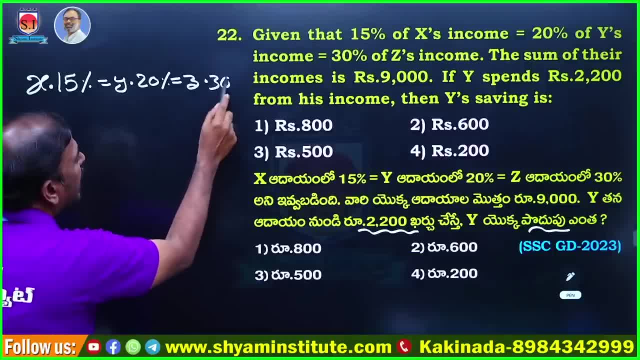 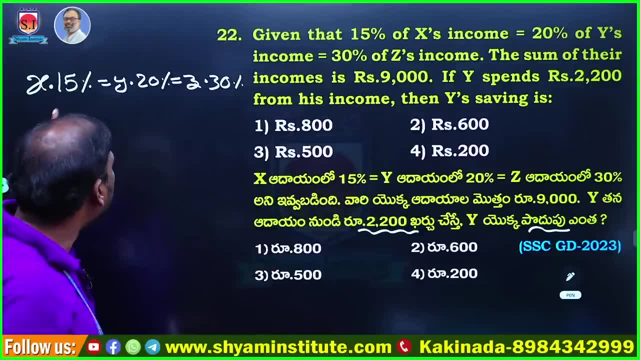 Z is 30% in Rs.1,500.. We have done the calculation with Rs.5,, right? You don't have to do the cancellation. You can do it directly. Since 15,, 20,, 30 is 60,, make it equal to 60. 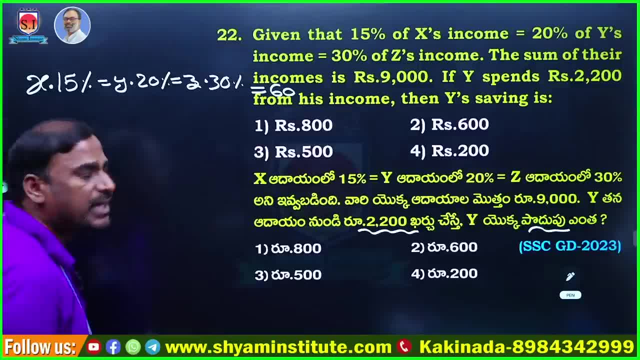 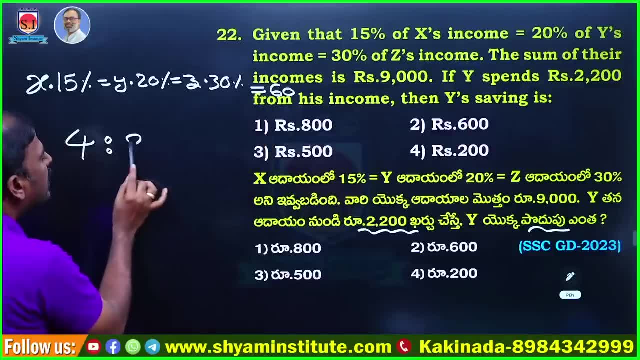 So what is X, Y and Z? 15 is 60.. X is 4.. So 23 is 60.. 32 is 60.. Now I need Y, 4, 3, 7, 7, 2, 9.. 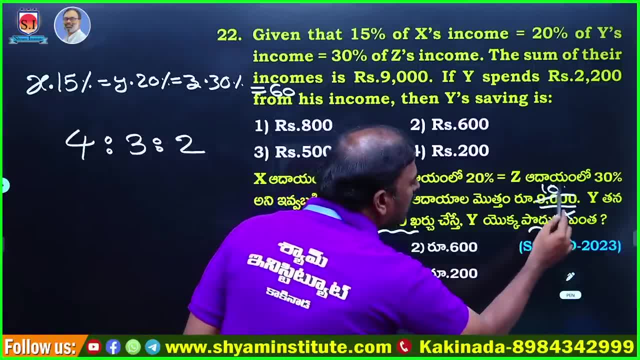 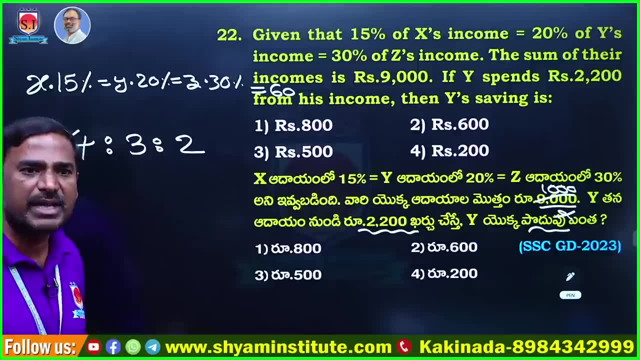 9 is 9,000.. 1 part is Rs.1,000.. So the total income of 3 people is Rs.9,000.. In which ratio we have: 4 is 2,, 3 is 2, 2.. 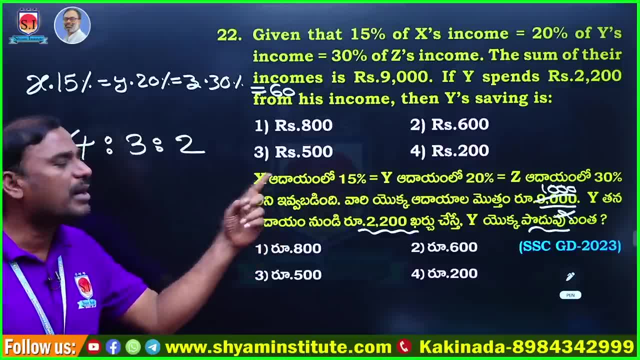 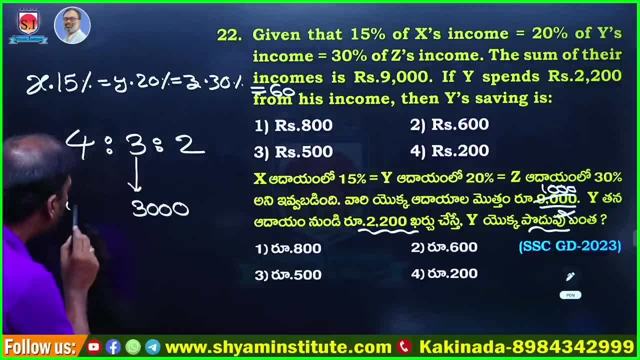 4,, 3, 7, 7,, 2, 9.. 9 parts are Rs.9,, 1 part is Rs.1,000.. So Y is Rs.3,000.. If Y is Rs.3,000,, 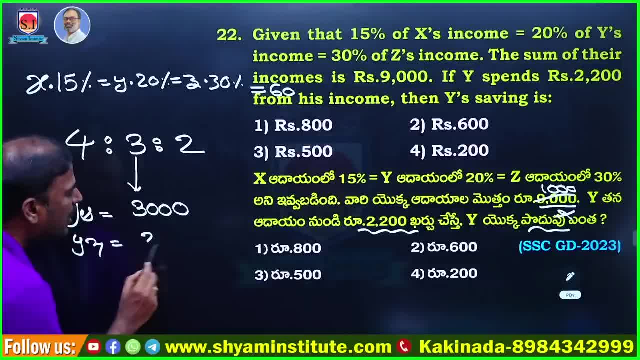 how much did he spend? Rs.2,200.. How much is Y? Rs.2,200, and Rs.3 is Rs.3,000.. How much did he spend for his life? Rs.2,200.. Here, the only difference is that, since it is Rs.800, the option 1 is the right answer. 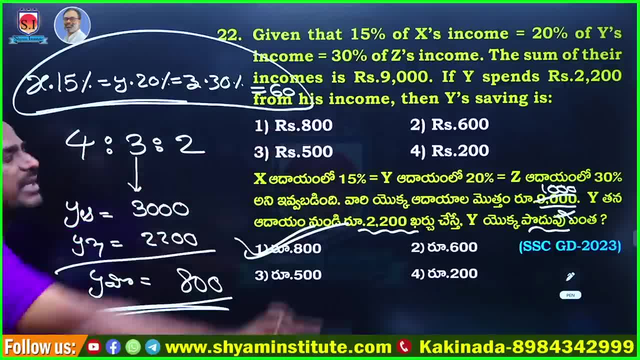 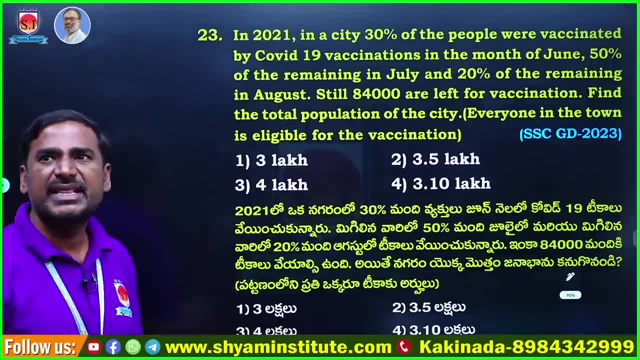 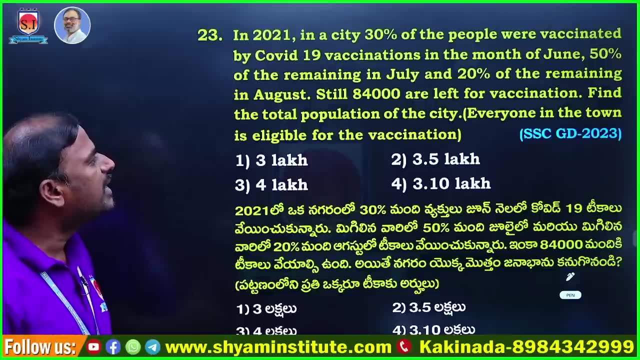 We can calculate LCN by memorizing it. We can calculate LCN by memorizing it. Next example: Look at the question number. It is the 23rd. The question is also very important. We ask this question repeatedly. So in 2021, in a city, 30% of the people were vaccinated by COVID19.. 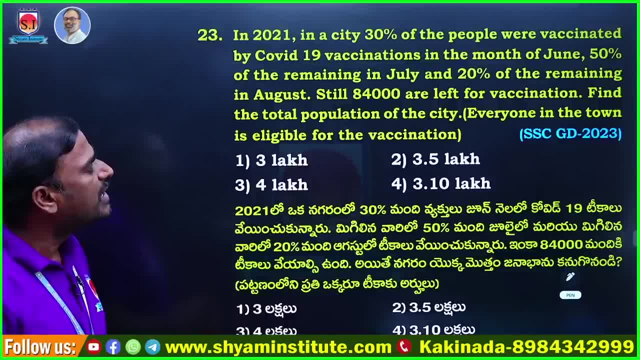 So in 2021, in a city, 30% of the people were vaccinated by COVID19. In the month of June, 50% of the remaining in July and 20% of the remaining in August. Still, 84,000 are left for vaccination. 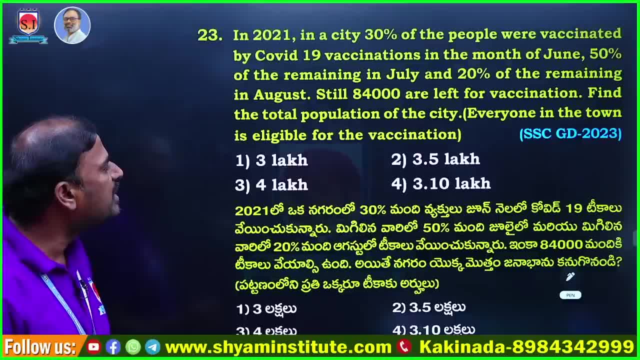 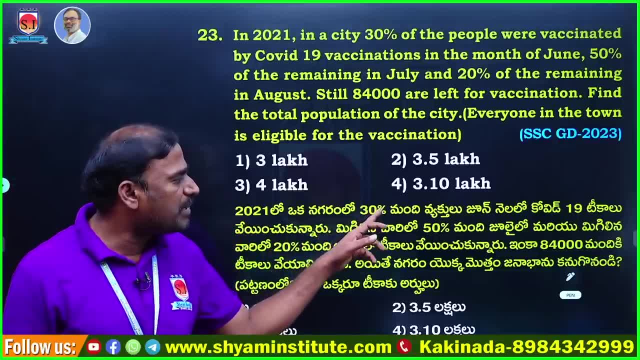 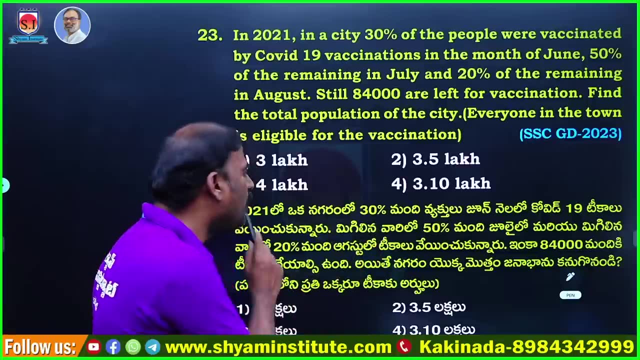 Find the total population of the city. Everyone in the town is eligible for the vaccination. See this question. In 2021, 30% of the people in a city suffered from COVID-19 in June. So in the month of June, 30% of the peopleaws COVID-19 vaccine are lettuce. 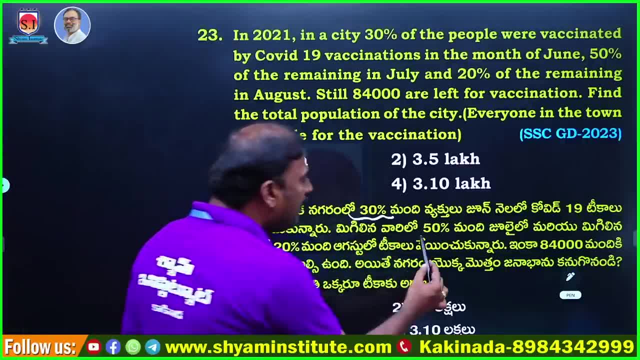 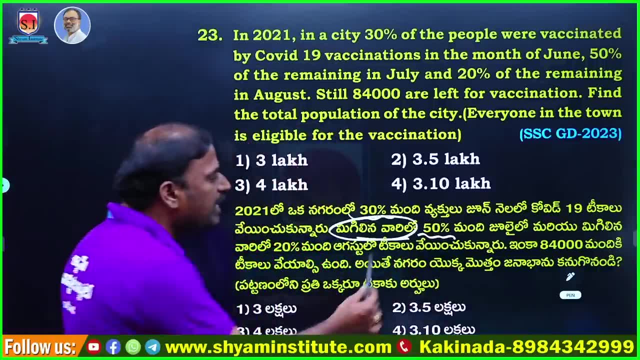 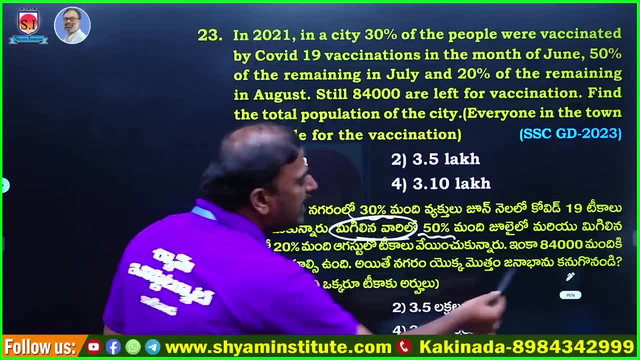 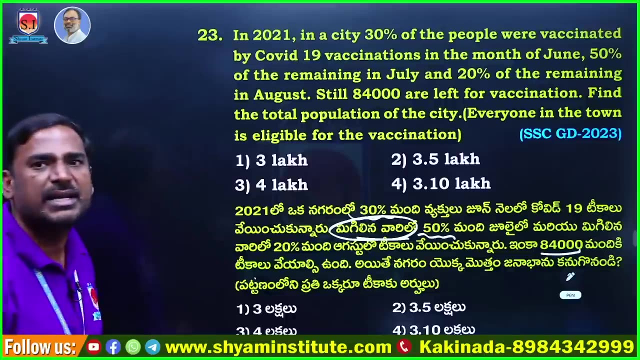 So this is a very important term that we used on July. So 50% said in July, 20% said in August. Still 84,000 have to be same amount of金. So It is not right to say that the entire population of that city is missing. 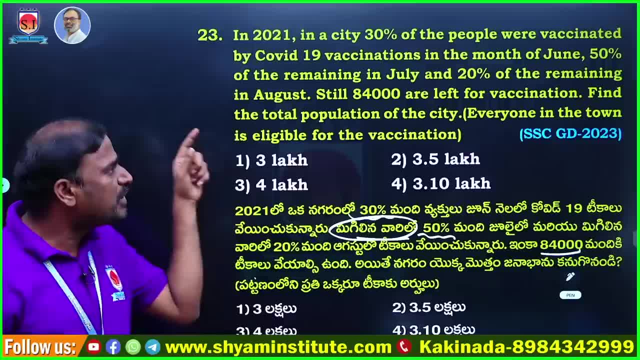 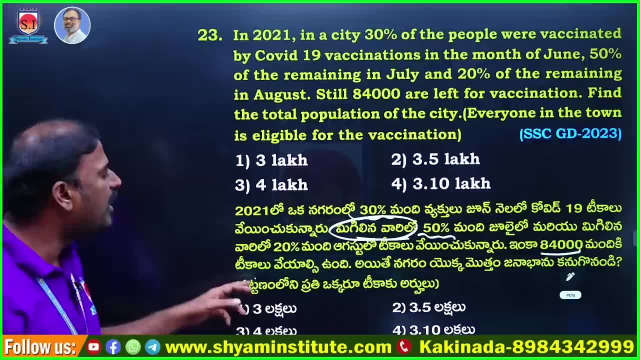 So if you are an English medium, what you have to see here is the concept of Inda Remaining, Inda Remaining, Inda Remaining. For Telugu people it is said to be in the remaining people, in the remaining people, in the remaining people. 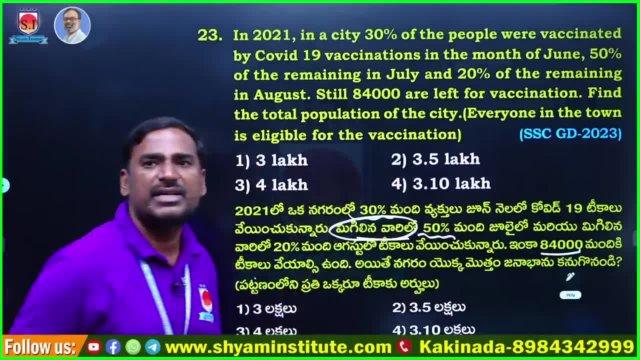 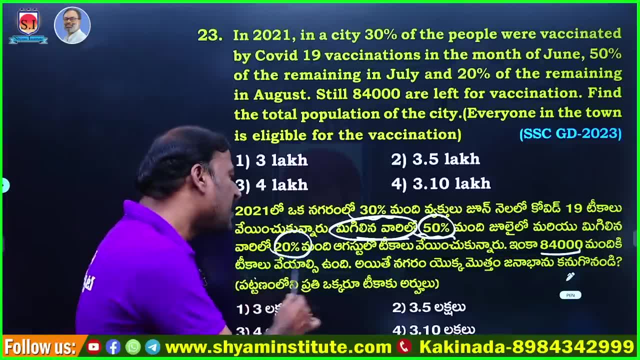 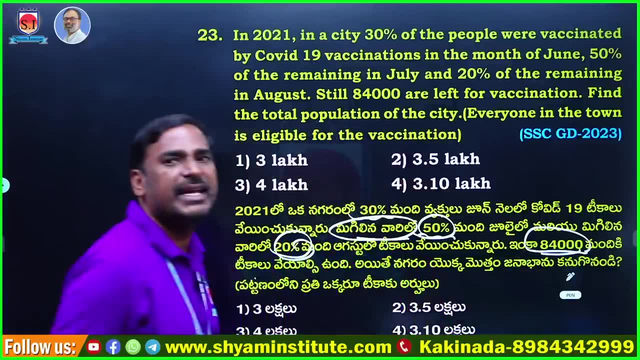 So in June, 30% of the Covid cases were reported. In the remaining people, 50% were reported in July. In the remaining people, 80% of the cases were reported in August. Finally, the number of people who have to be reported is 84.. 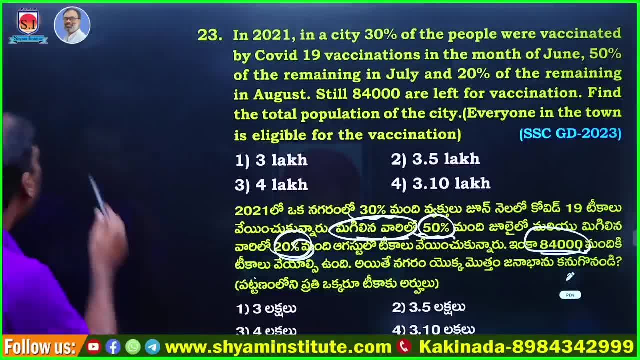 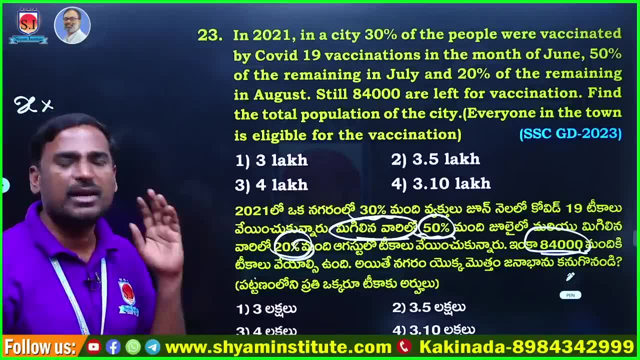 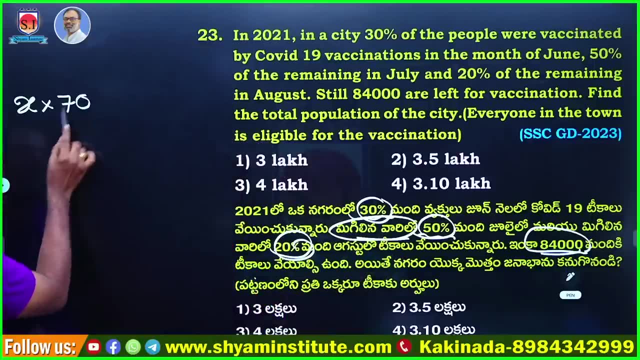 So what is the total population? So here I have taken the total population as X. We always have to remember one shortcut: In the remaining people, in the remaining people, the first 30% of cases were reported, So in the remaining people it is 70 by 100. 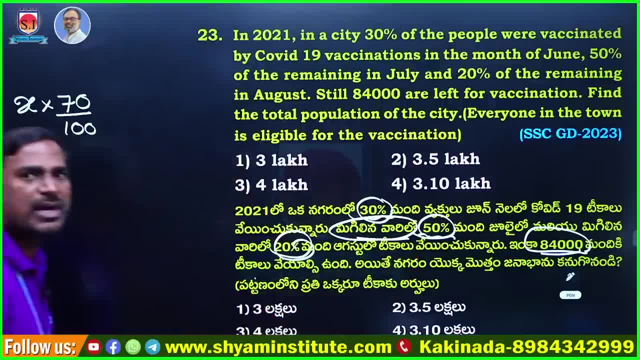 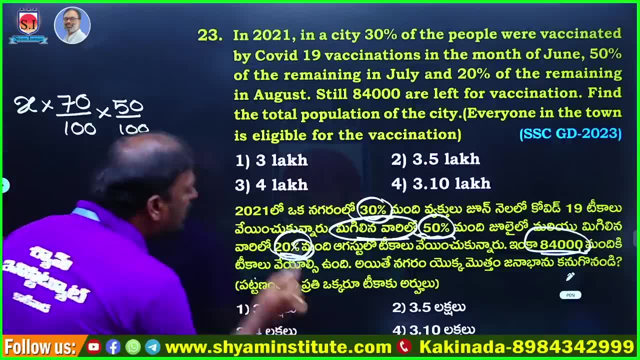 In the remaining people, 50% of the cases were reported in July, So in the remaining people it is 50 by 100.. In the remaining people, 20% of the cases were reported in August, So in the remaining people it is 80 by 100.. 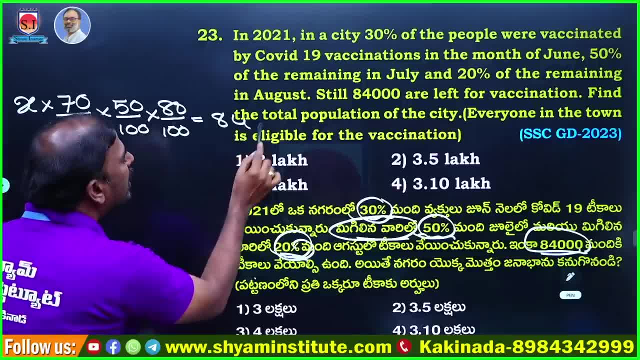 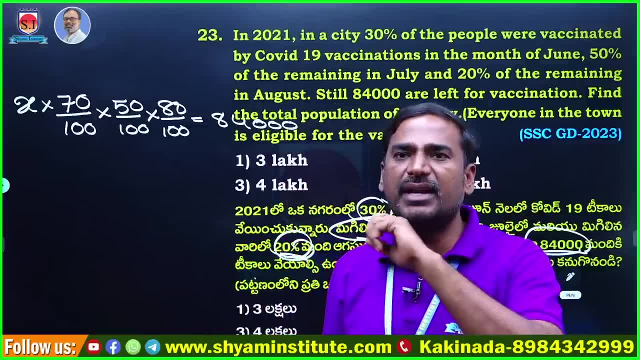 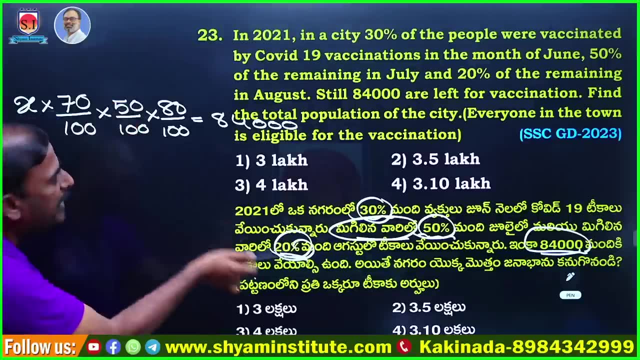 In the remaining people it is 84,000.. So this type of example: whenever you see an exam, you do not have to think about anything else. You can take this step directly. So the first 30% of cases were reported as 70 by 100. 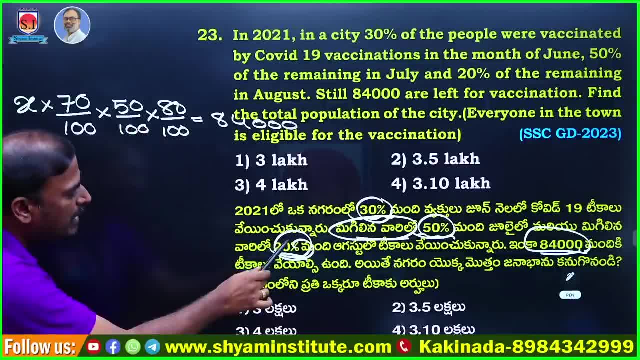 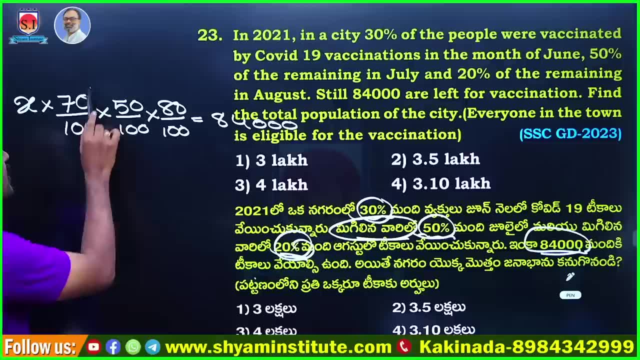 Then 50% of cases were reported as 50 by 100.. Then 20% of cases were reported as 80 by 100.. Finally, the remaining number is 80 by 4000.. Right, So 0, 0, 0, 3 zeros were taken. 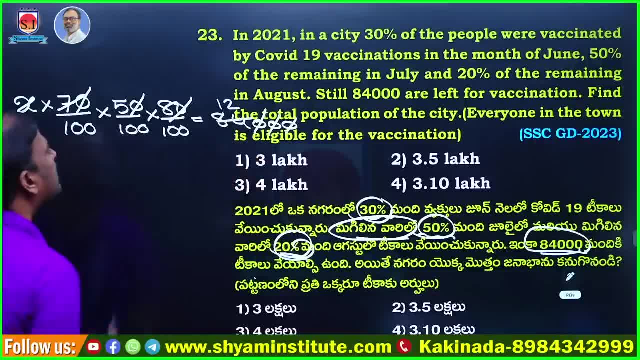 If we divide it by 7, it is canceled as 7 by 10.. It is canceled as 4 by 2.. It is canceled as 4 by 3.. If this becomes 10, it becomes 0.. If this becomes 9, it becomes 0. 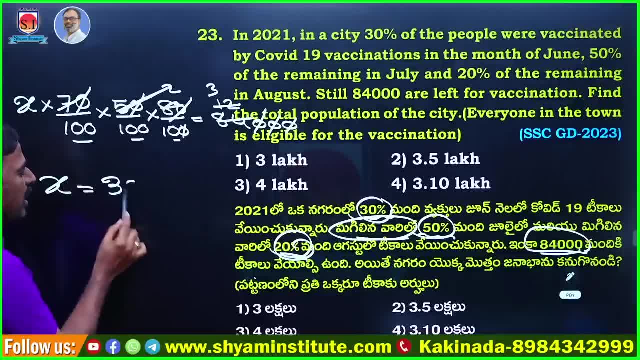 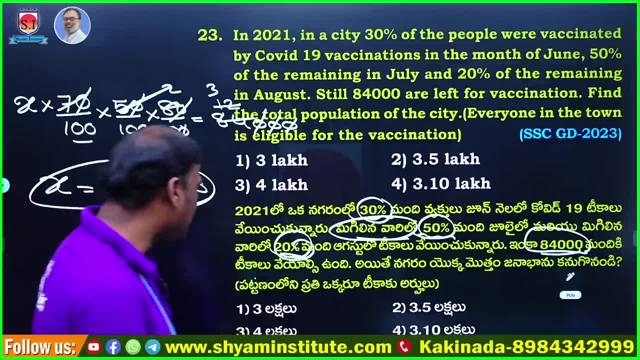 And if this becomes 7, it becomes 5 zeros. AX is equal to 5 zeros. If you have 5 zeros all over, We will count as 3 lakhs. The total number of those in that city, we will count as 3 lakhs. 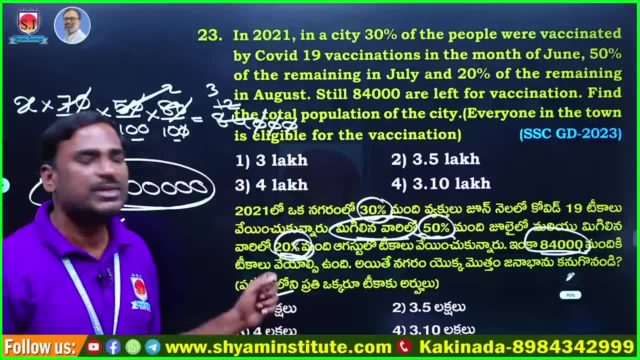 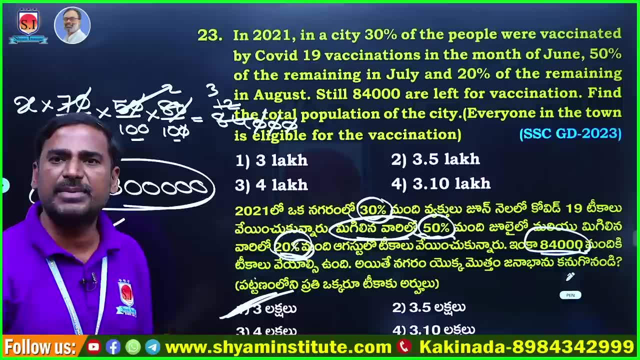 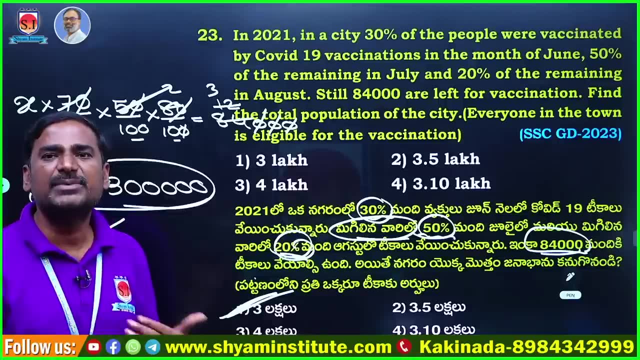 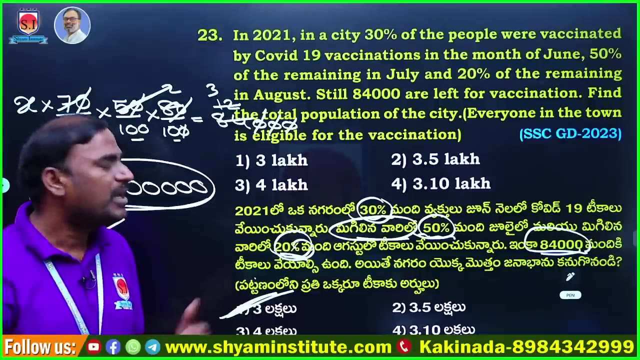 Option 1 is the right answer. So these are the repeated models. It is called Indah remaining or Indah remaining, Or. Telugu says in the remaining people, in the remaining people In the next class. we will discuss about Profit and Loss and Discount. 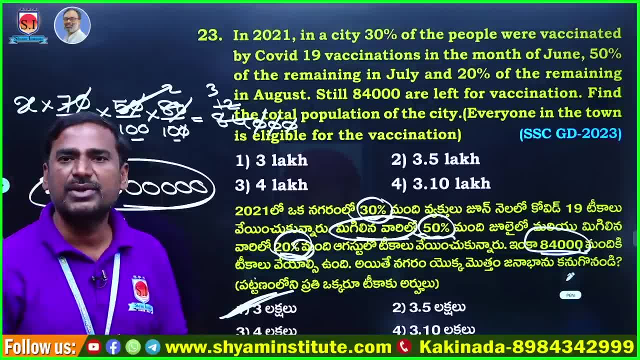 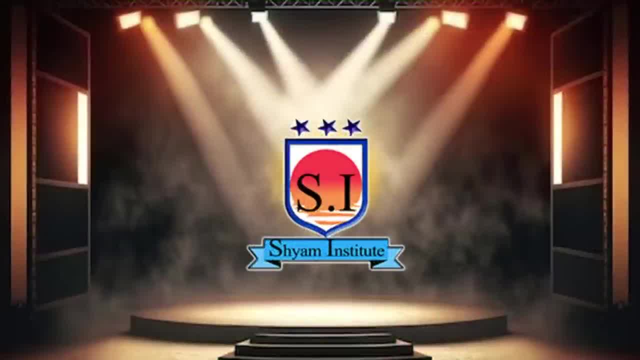 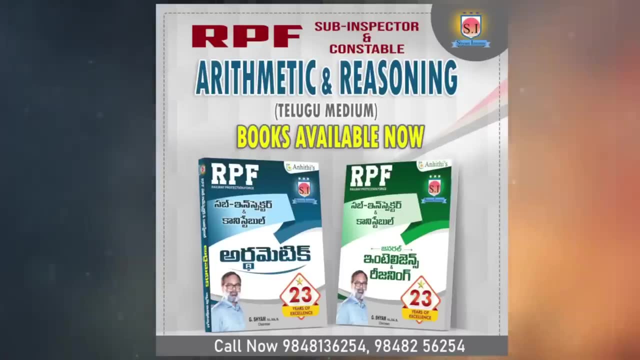 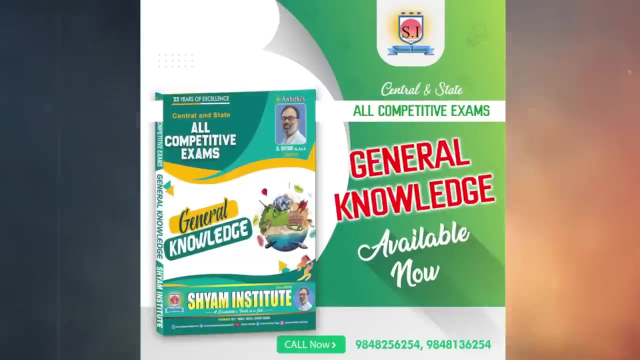 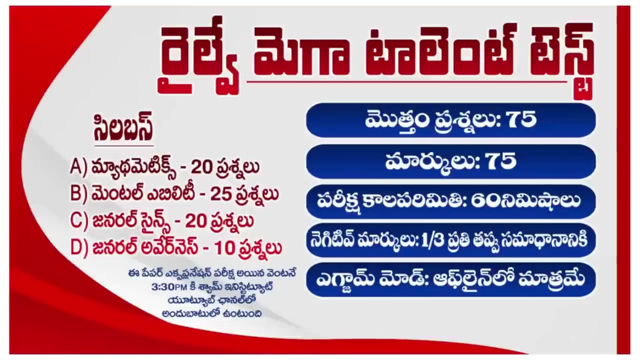 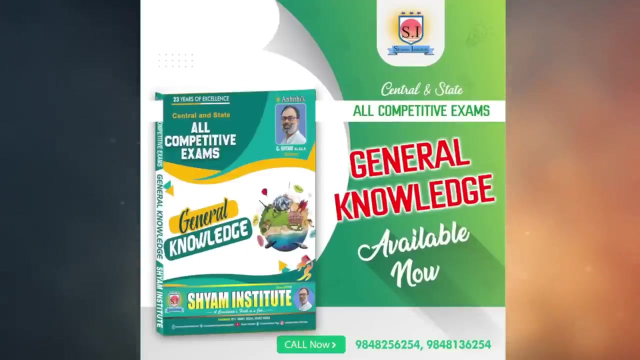 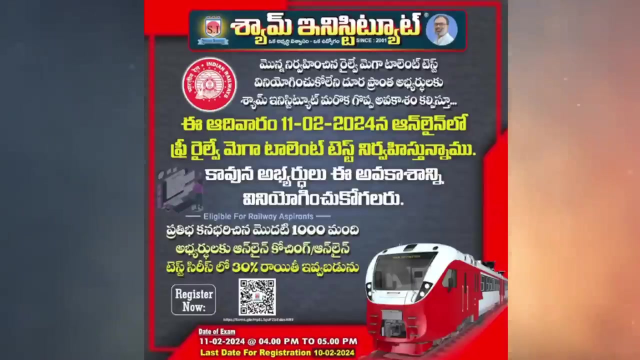 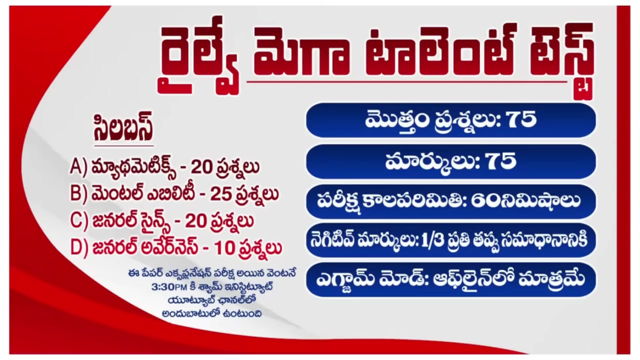 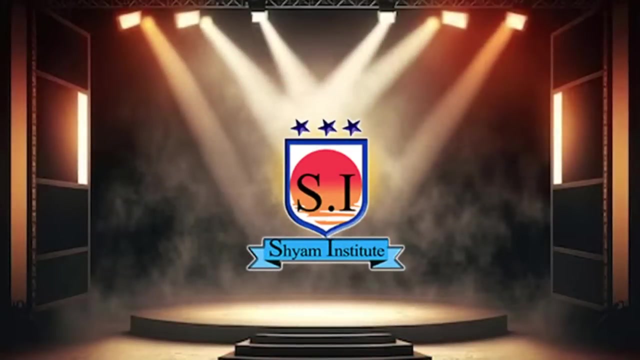 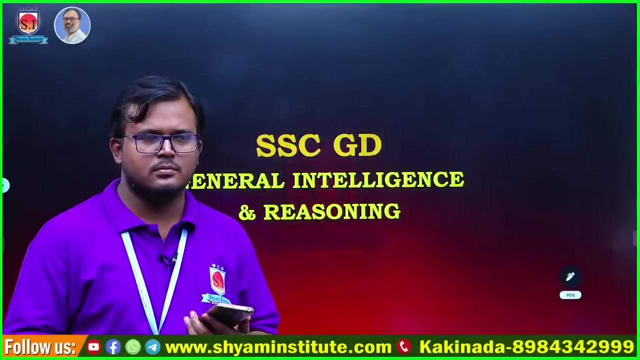 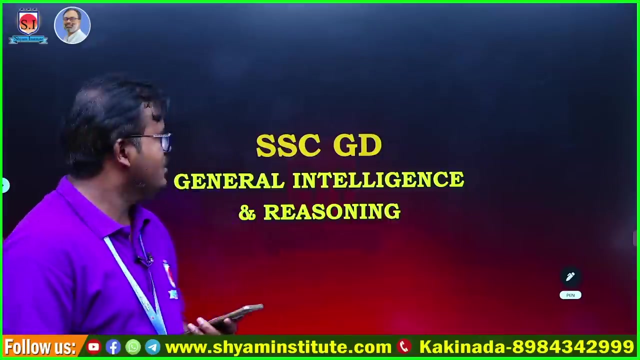 Thank you for watching. Have a nice day. Subtitles by the Amaraorg community. wwwamaraorg community. wwwyoutubecom. wwwyoutubecom. Good evening all of you. Welcome to our Siam Institute Youtube channel. Today is SSCGD: General Intelligence and Reasoning part- Live Session. 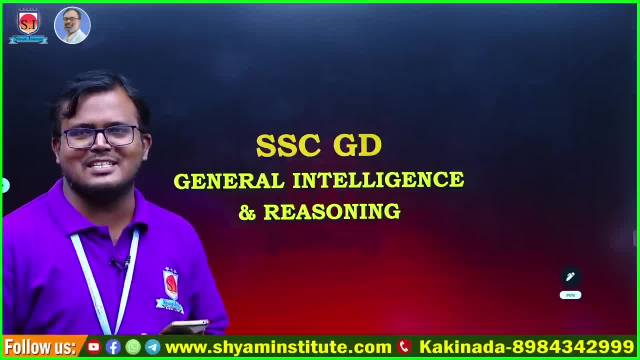 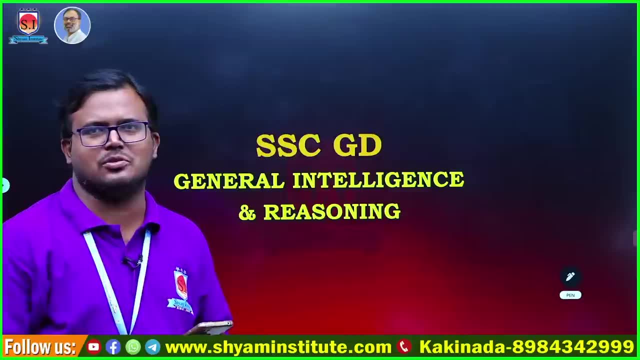 Today we are again going to discuss about SSCGD. Now we have academic exam point of view. Previous questions are like this. Next question will be like this. So from these questions we are getting a few questions based on the blueprints given to us. 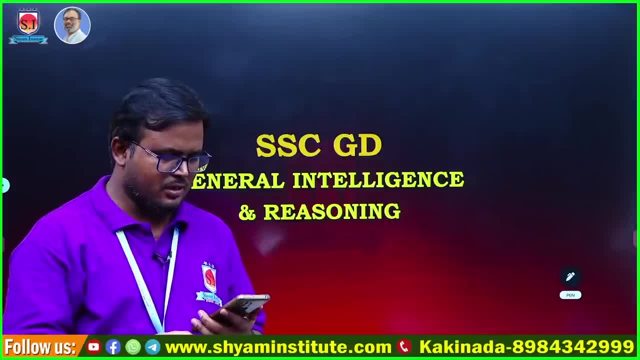 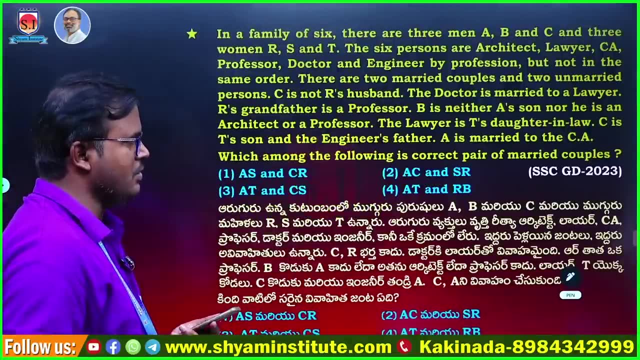 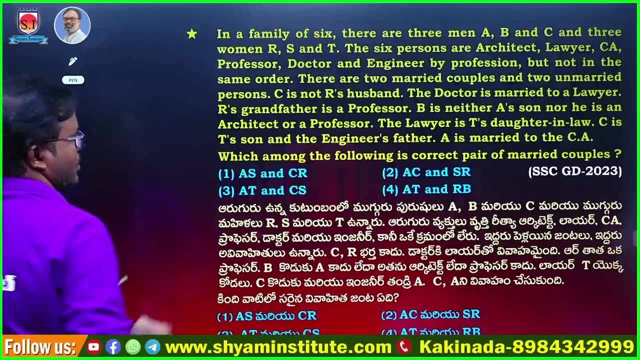 So let's see how these questions are being given to us. So the first question. So you have to guess the answer compulsorily when it comes in. So you have to guess the answer in the comment box. So you have to see the question. 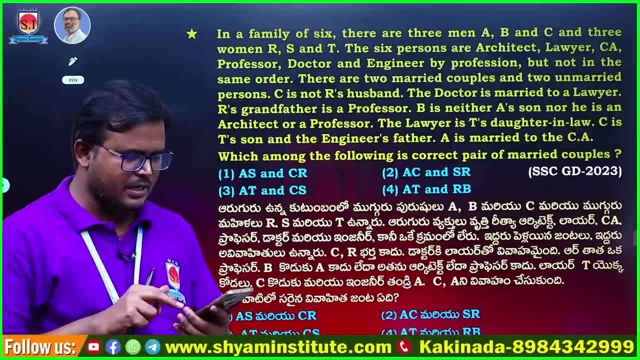 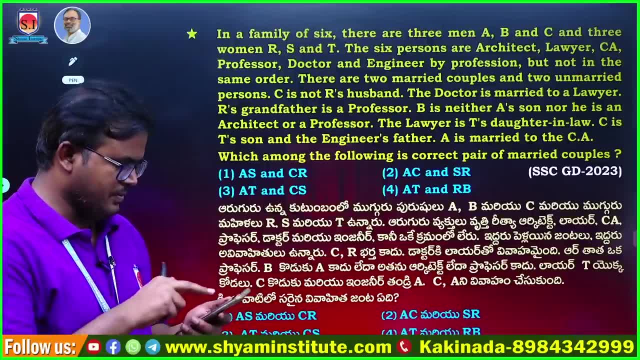 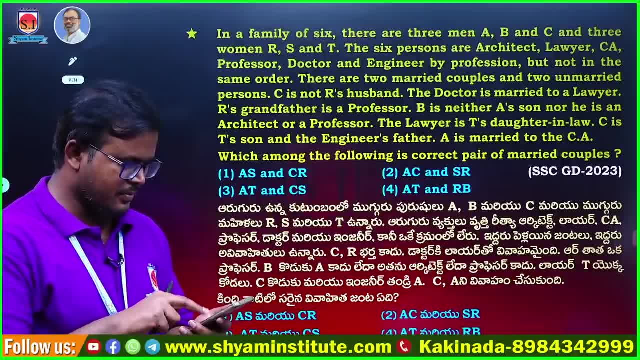 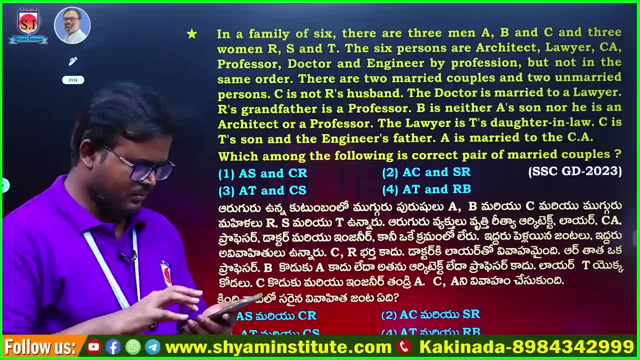 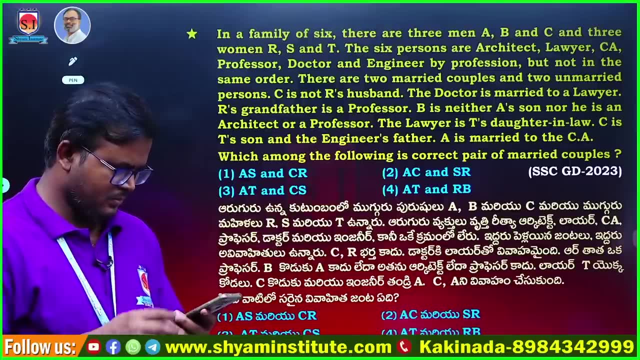 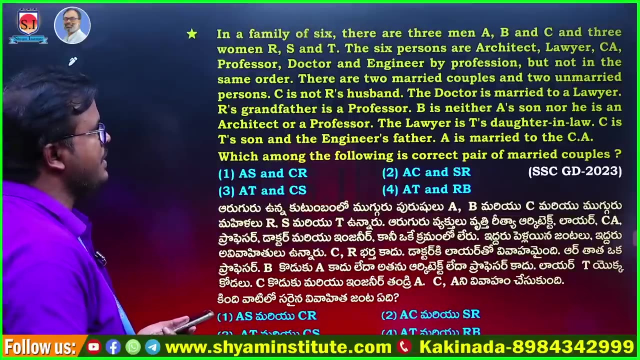 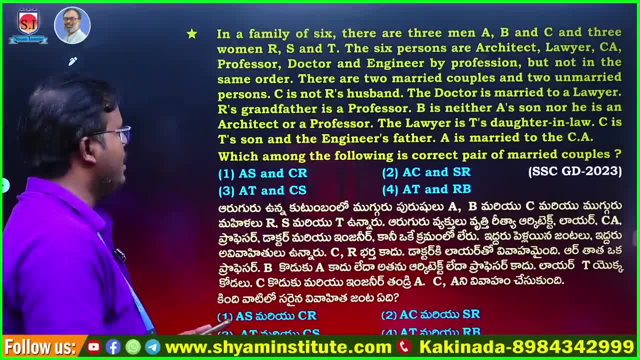 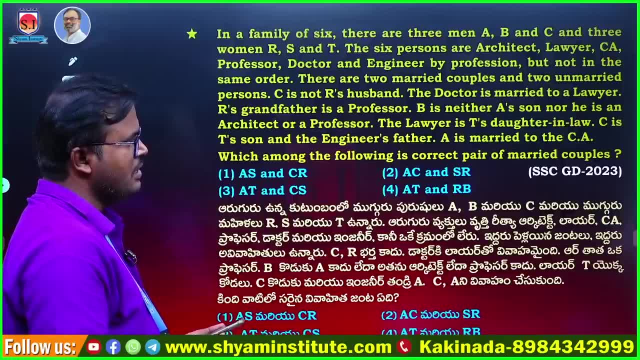 But not in the same order. as mentioned, There are 2 married couples and 2 unmarried persons. There are 2 married couples and 2 unmarried persons. B is neither A's son nor he is an architect or a professor. The lawyer is T's daughter-in-law. 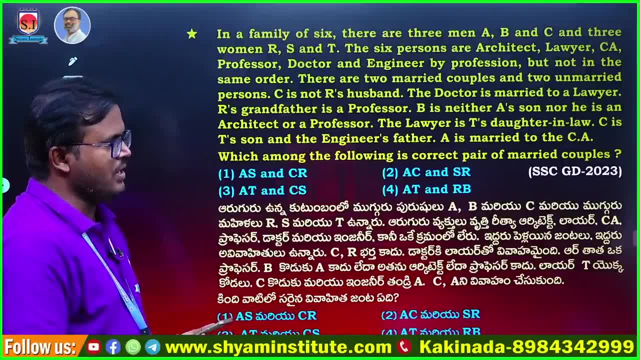 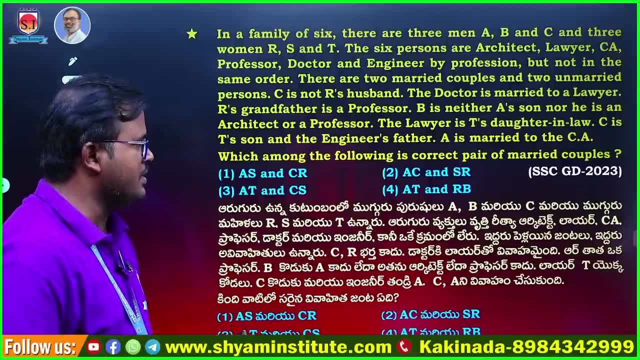 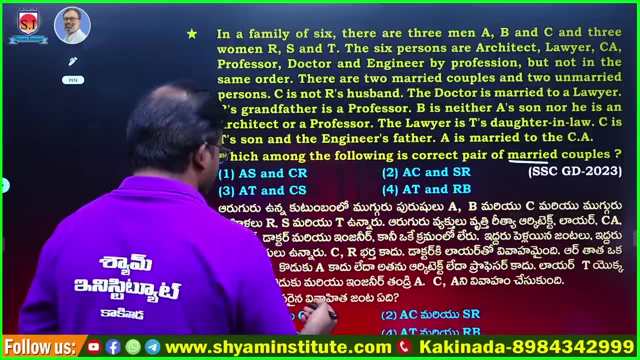 C is T's son and the engineer's father. A is married to the CA. So what did you ask in the final question? Which, among the following, is the correct pair of married couples? So who are the married couples And who is the married couple? 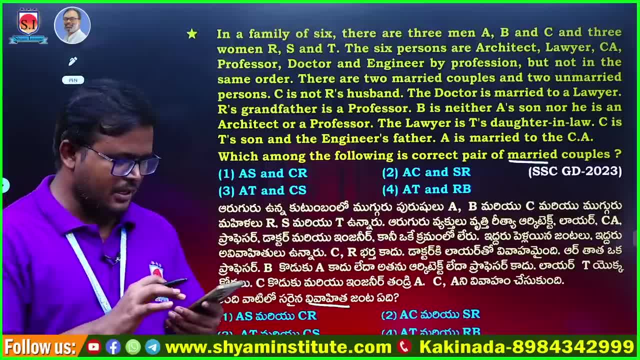 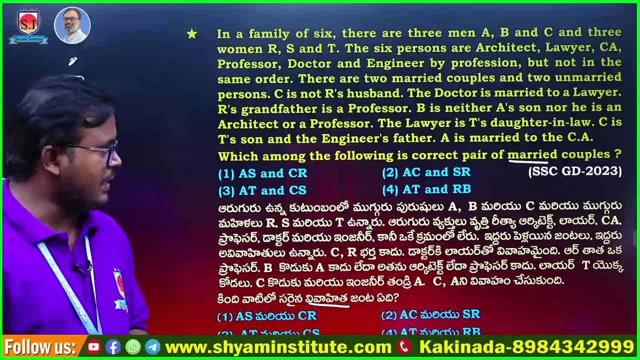 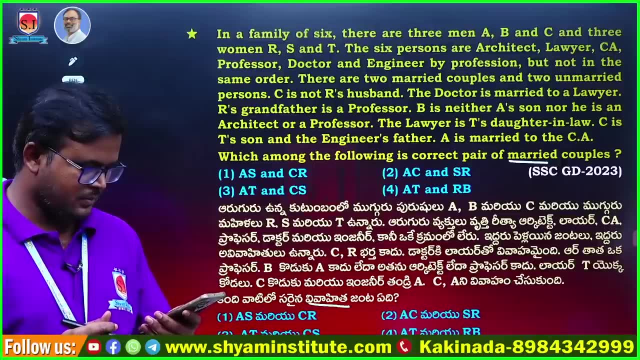 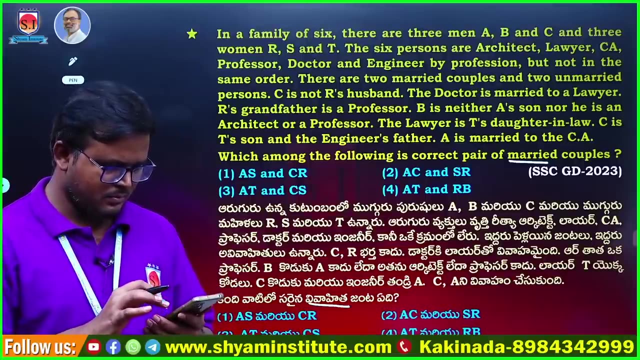 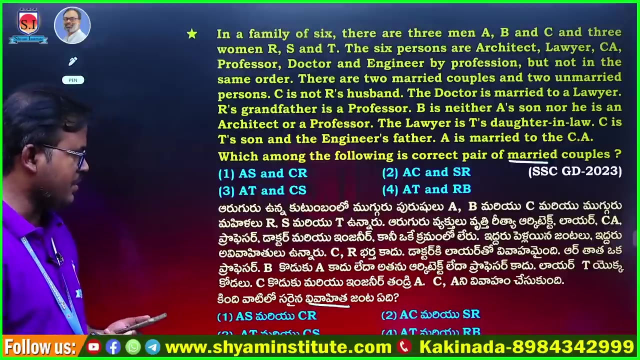 So which of the following options do you think is correct? So let us know in the comment box. Let us try it. So we have learnt the concept of Fuzzle Test. See, Are there any people who are coming as AS and CR. 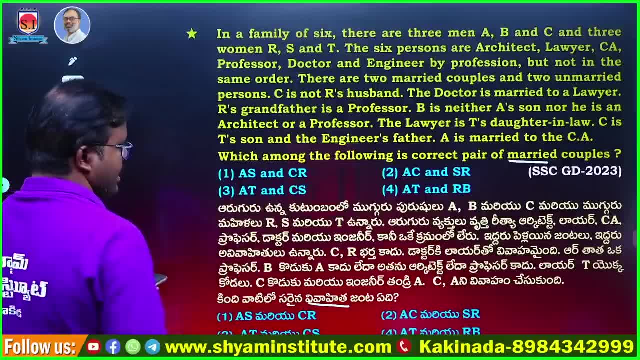 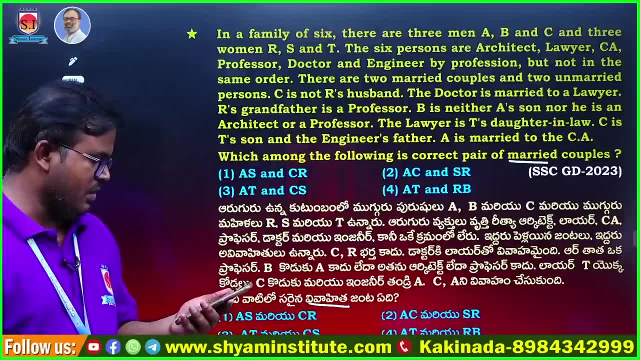 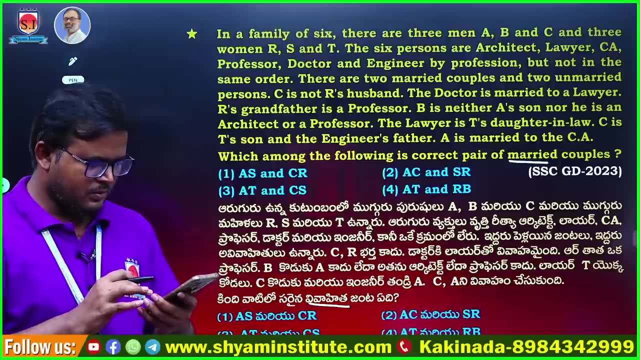 Or are there any people who are coming as AC and SR, AT and CS, Next AT and RB? So when we have married couples, we have two couples. So what are those two couples? If you think the answer is correct? 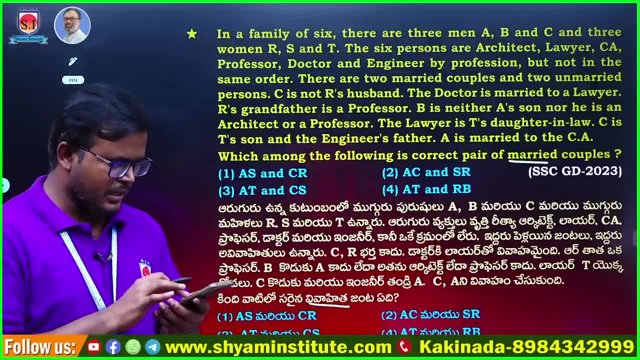 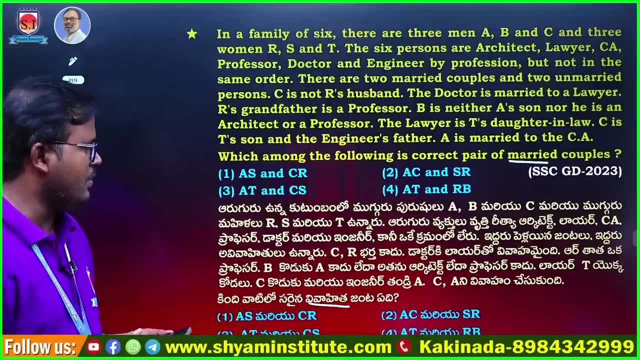 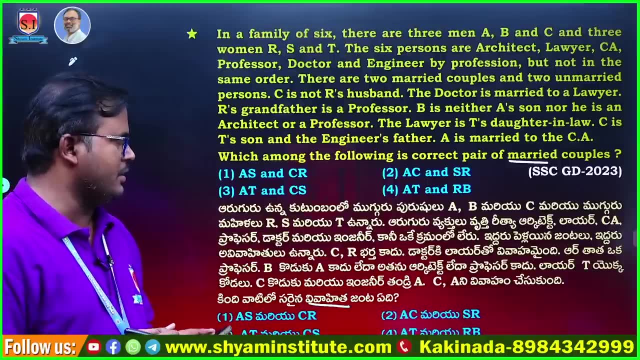 please let us know in the comment box, So in our live chat we will give you the answer. So let us start the problem. So let us start the problem. There are three men in the family of six. They are A, B, C. 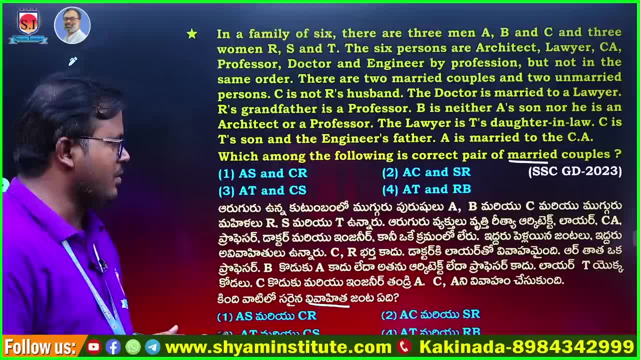 Next there are three women. They are R, S and T. The six women: one is an architect, Another one is a lawyer, CA is a professor, The doctor is an engineer, But they should not be in the same program. 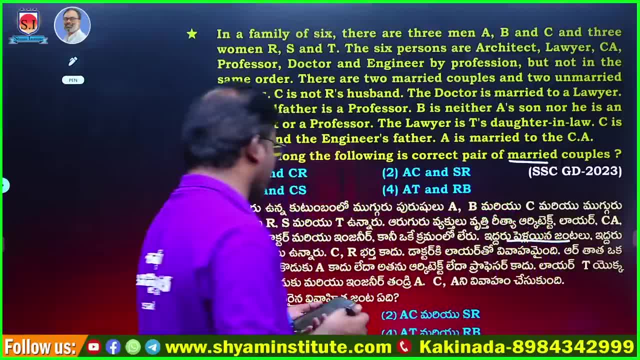 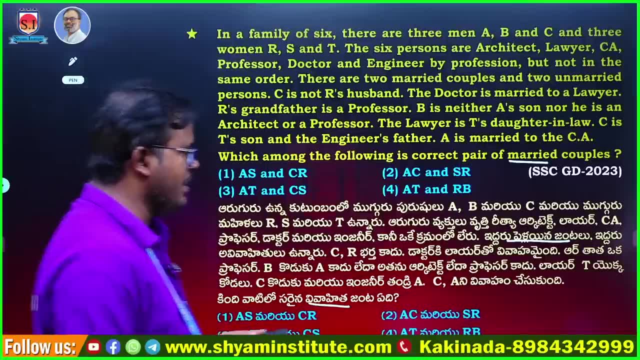 They are the two married couples. So they are the two married couples. Many of us are not husband and wife of CRE Doctor got married to a lawyer. So if you observe here, So the person named R is the grandfather. 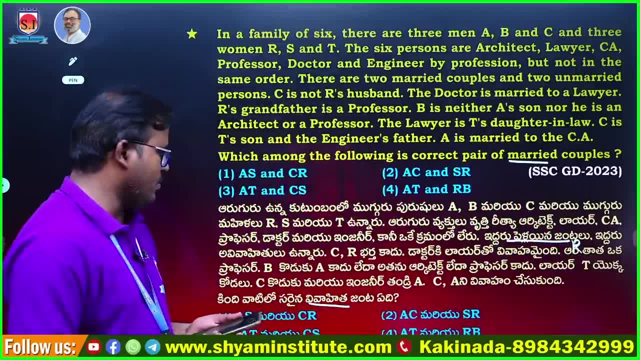 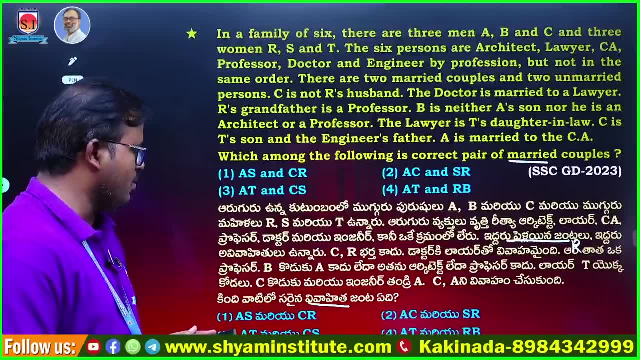 Okay, you are a professor. Next, when the son of B comes, it is not A, Or he is not an architect or a professor. Next, the lawyer is the daughter of T. The son of C is the father of engineer A. 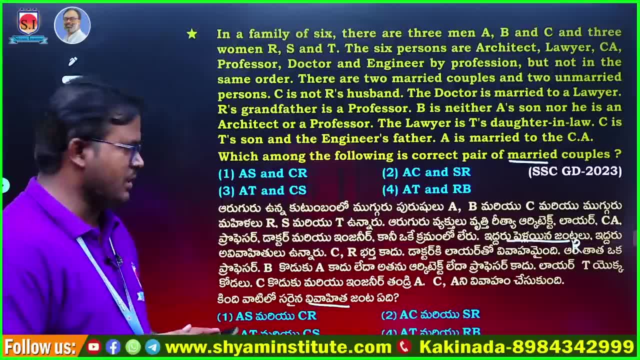 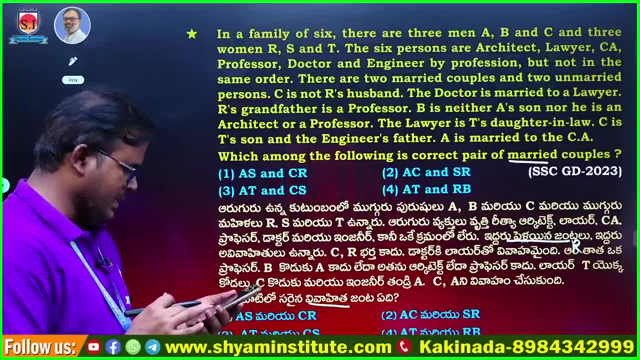 When C comes. A got married, So in the below he asked what is the gender of the married man? It should be AT and CS. It should be AT and CS. So Venkat Ramana gave the fourth option. 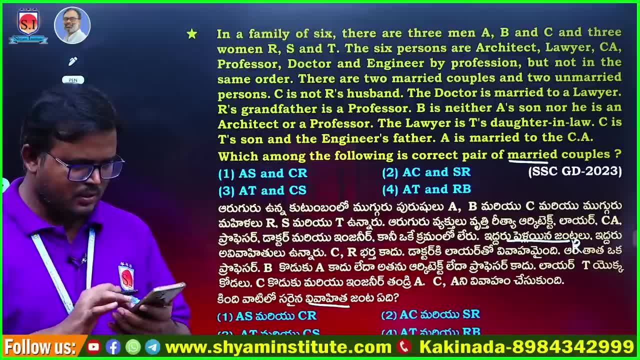 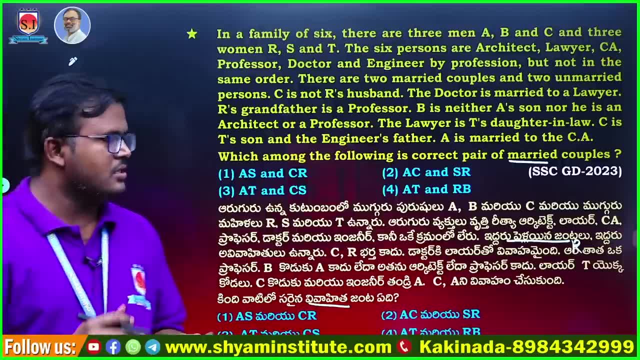 KV Ramana gave the fourth option. See, when we get the question of Fuzzle test in the exam point half they will give the data. So when it comes to the last, only one person will ask the question. 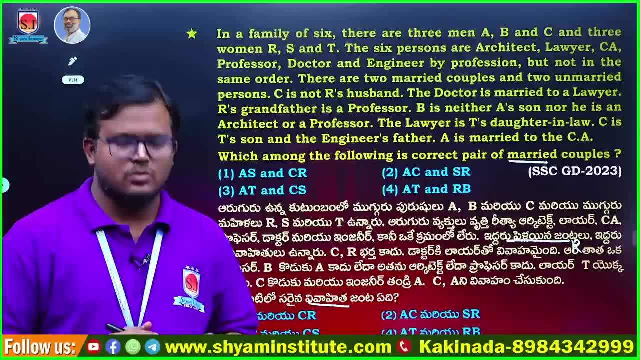 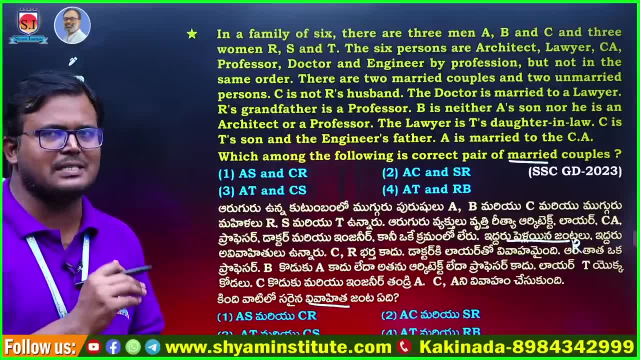 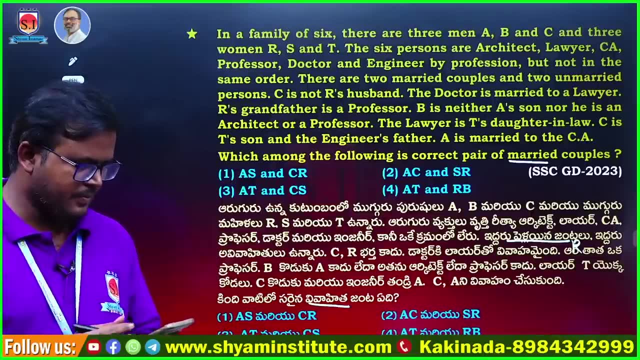 See what is the correct answer for this question, What is the answer that you think is correct. So once you try it, compulsorily Try it and give the answer that you think is correct. Tell it in the comment box. 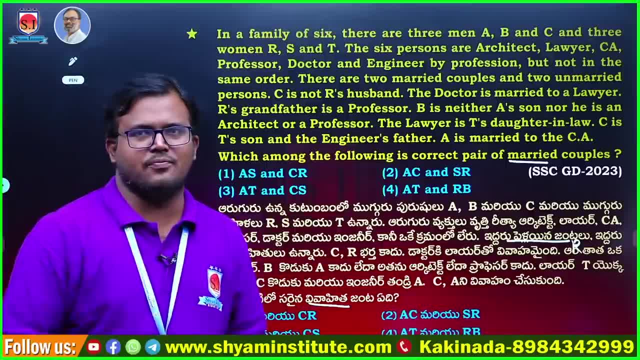 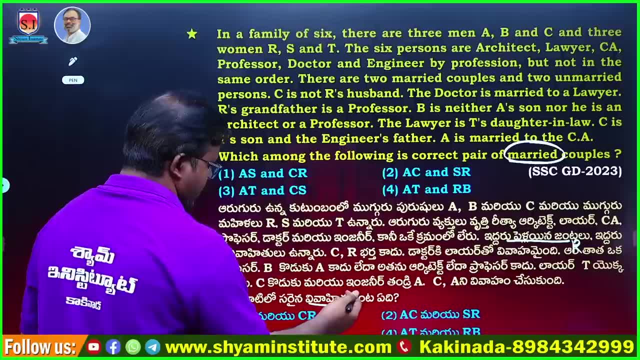 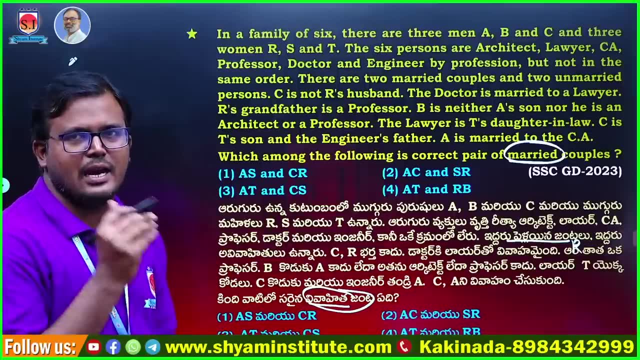 So in such questions, first, the question given is very important. So what is it Here? he said married couples. Okay, What happens here? What is the married couple? So when the married couple is asked, let us see how he explained about the couples here. 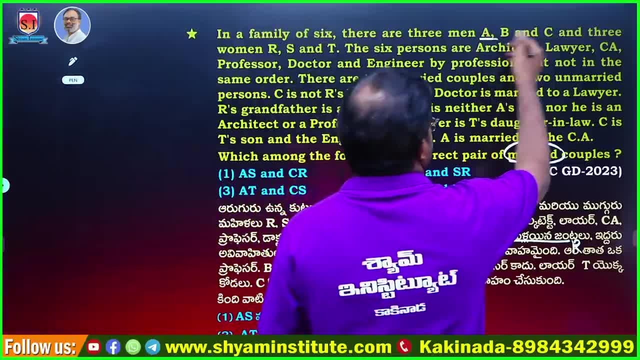 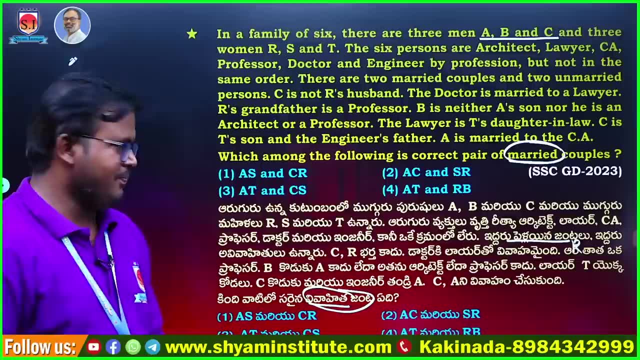 So what did they say? First, who are the people named ABC? So the person named ABC is a man. So when there is a man, we should take care of the guarantee in the option. What did he say when he came to the option? 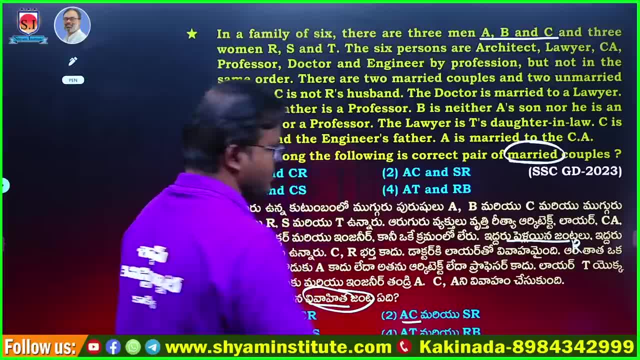 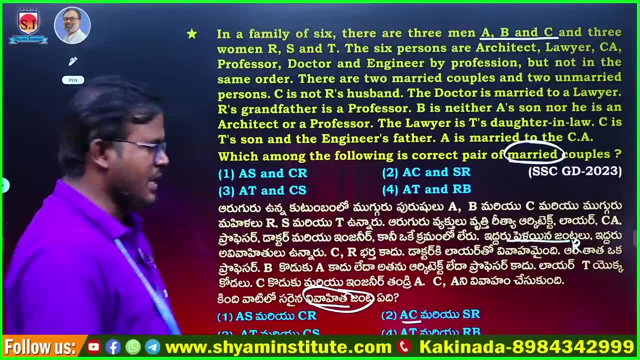 In ABC they gave the person named AC Who are the two people named A and B. They are the men, So they will be the married couple. So what is the guarantee? First take out the second option. 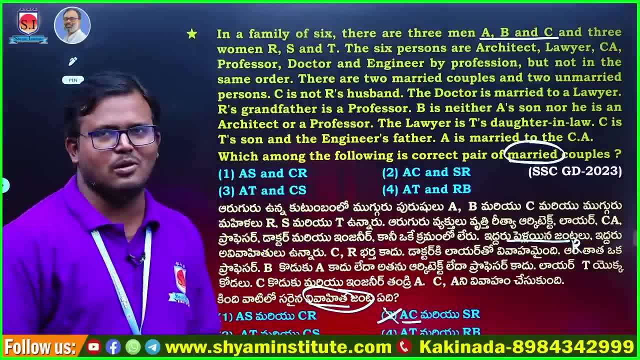 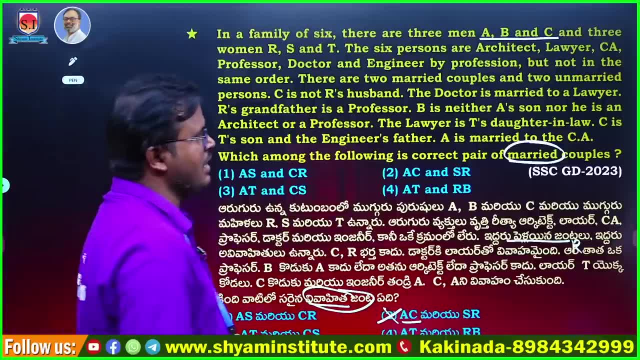 But the second option is not the answer. So we should read the question in that. And if you check the option on the verification method, it becomes easy. So what happens after that? Next, what is happening is…. So look at the data and see what else he will talk. 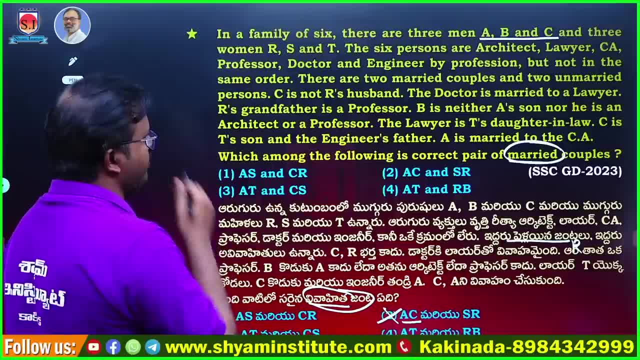 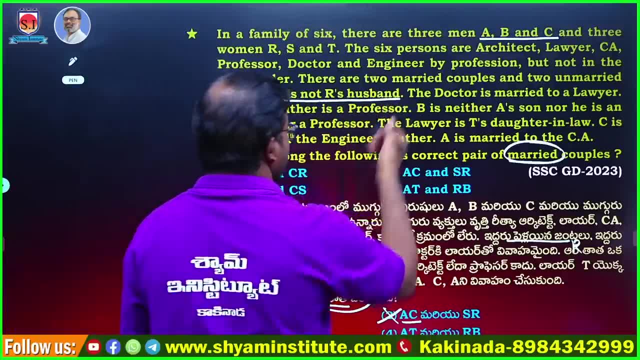 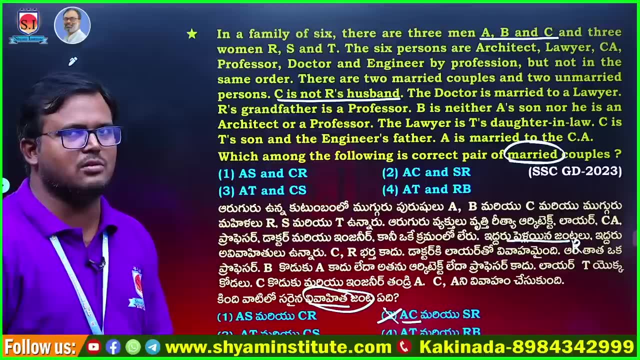 They spoke about a couple and the next person comes here. So there are two married couples and two unmarried persons are given. Okay, So the person named C is not our husband. Who is the person named C? He said that the CNA person and the RNA person did not get married. 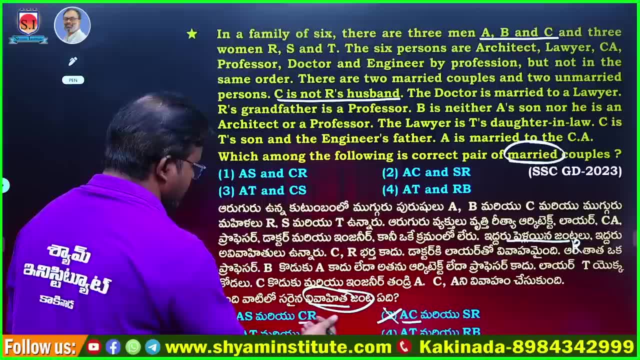 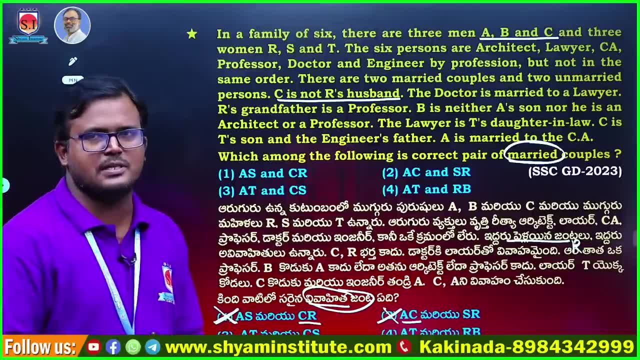 When you come here, the CNA person and the RNA person are in the first option, But this is not the answer. So what will happen If there are two options? we will eliminate them. After doing this, we have to study again. 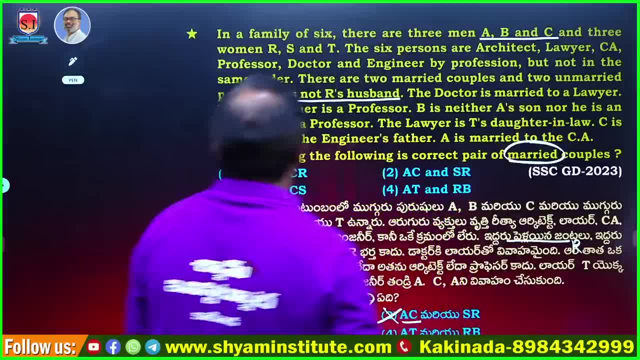 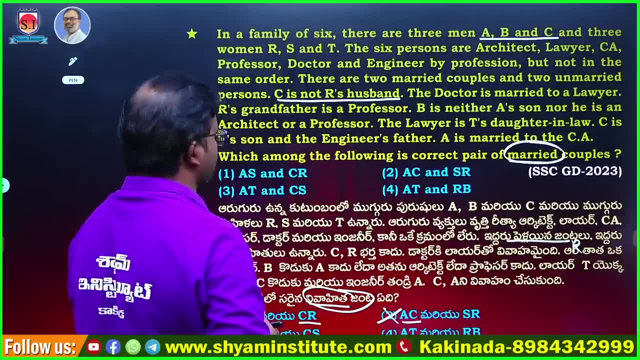 What did he say? He said that the daughter is married to a lawyer. When he came next, he said that the R's grandfather is a professor. B is neither A is son or he is an architect. Next, R is professor, So the lawyer is T's daughter-in-law. 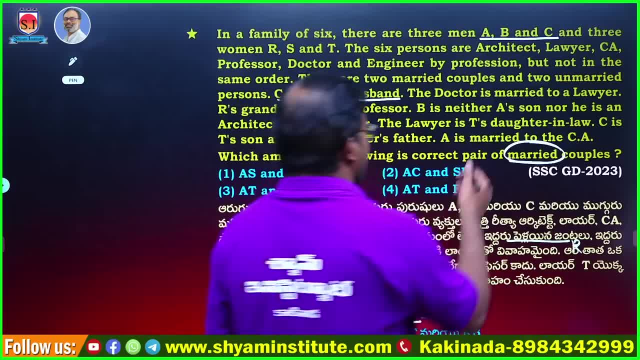 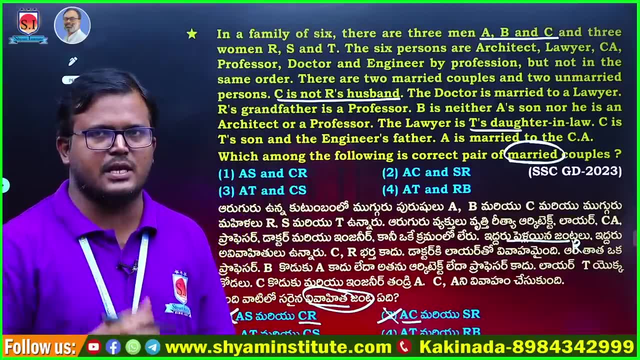 So you see here what is happening. He said that the TNA person has a daughter-in-law. What should be the daughter-in-law of the TNA person? First, what should be the guarantee for the TNA person? There should be a son. 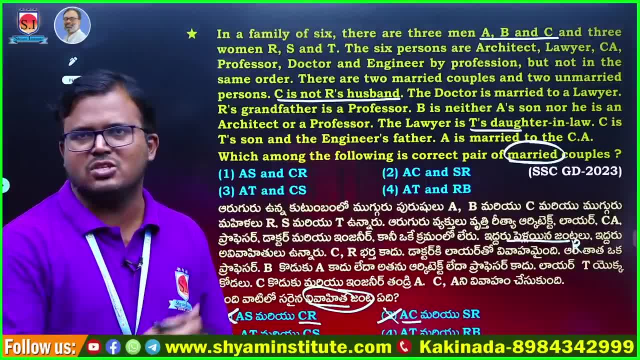 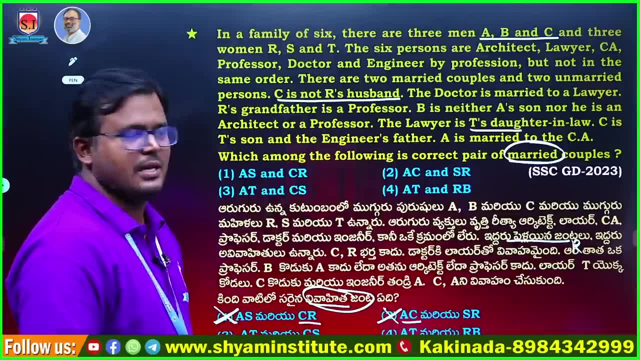 What is the responsibility of the son When we come here? he said that the daughter-in-law. He said that the daughter-in-law. Then what is the guarantee for the TNA person? So we have got a marriage here. What is the guarantee for the TNA person? 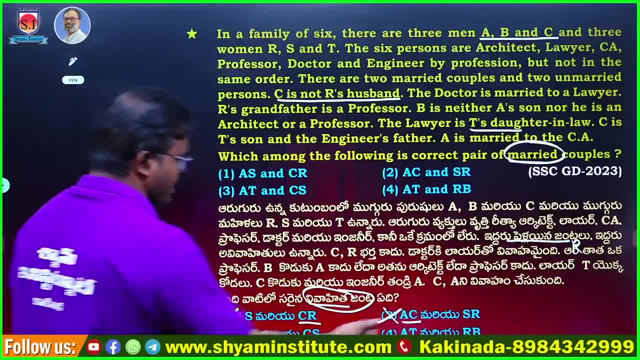 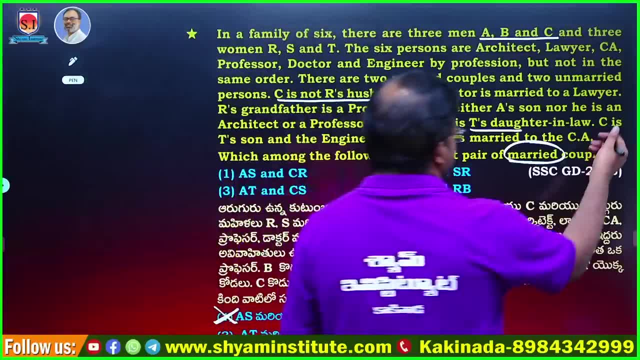 Like the marriage. So we have two letters in the R, Then what will you do next? He said that the C's and the T's are in agreement. Then who is the CNA person? If we observe the CNA person, The son is guaranteed for the TNA person. 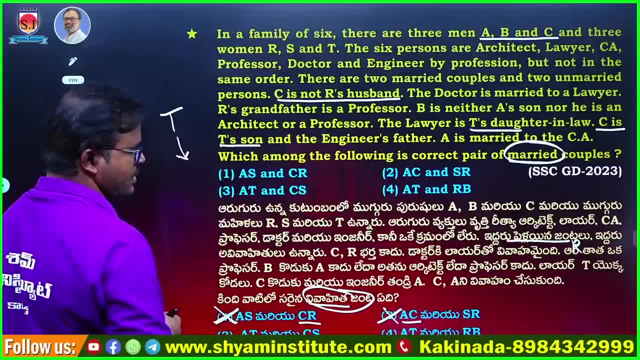 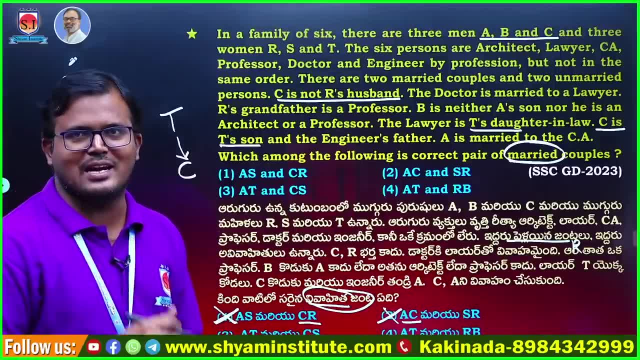 While we come here, the TNA person is a son. What is the guarantee for all these? When the girl is getting married, there should be an option to be a married woman. There should be a CNA letter as an option. Where is the CNA letter? It is here. 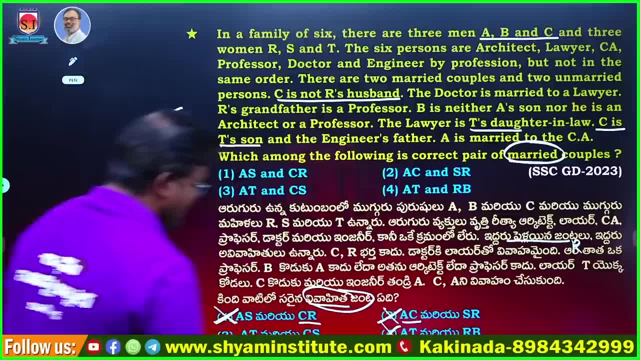 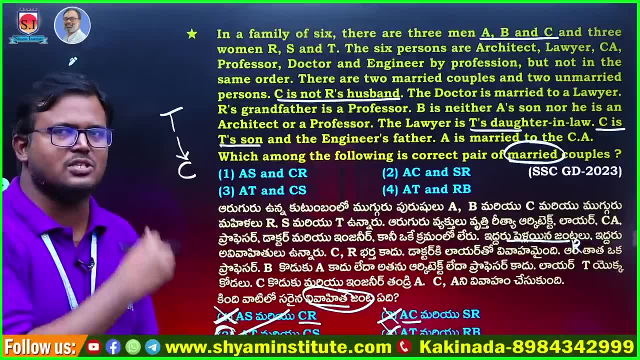 What is the answer here? It is RBN. This is not the answer. What is the answer to the CNA letter? This is the third option. When we look at the data given, we can check the options given here. Here is the option: verification method. 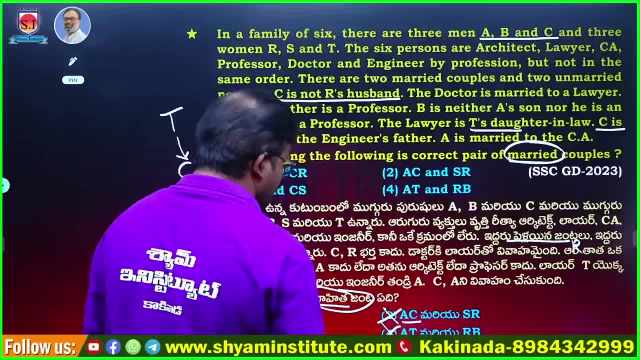 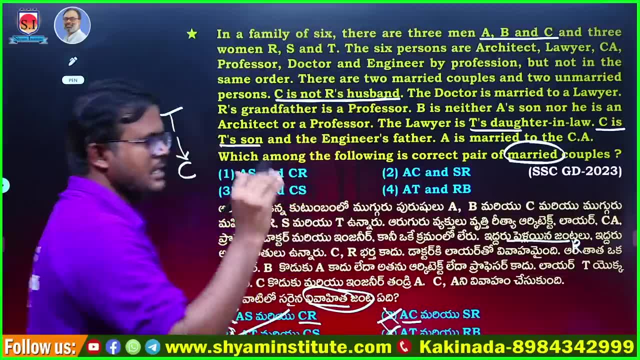 Here, no CNA person is a man, Because their marriage does not take place. Here. it is said that CNA persons are married. What did he say? CNA person and RNA person did not get married here, So this is also wrong. 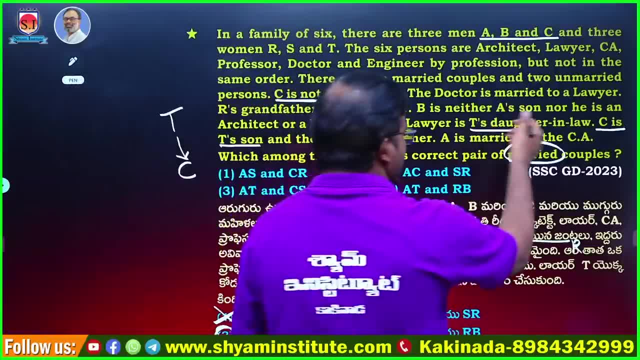 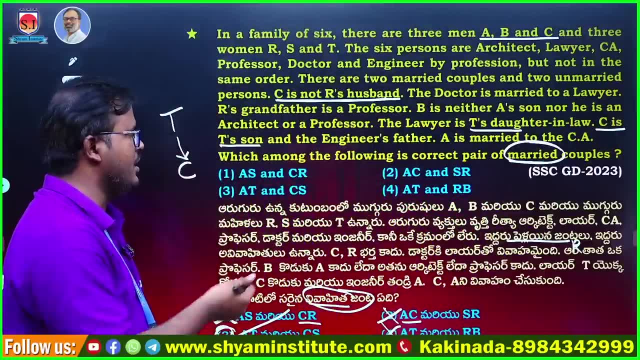 What happens to the rest? So the TNA person has a daughter. When there is a daughter CNA person is guaranteed here. So the TNA person has a son. So it is guaranteed that the TNA person should have a son. 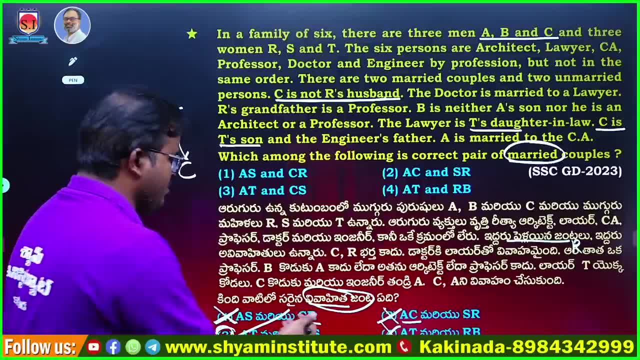 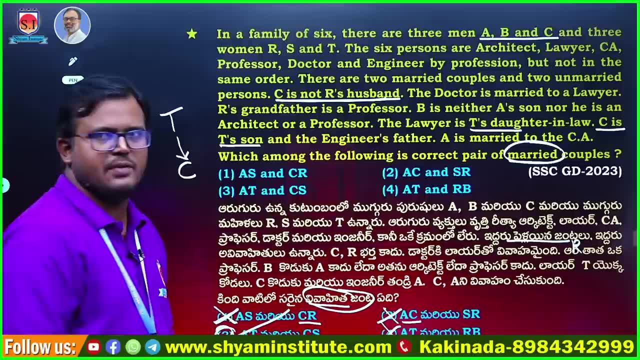 The wife who is related to that son. their wife is guaranteed to be a CNA person. So we have the option verification method. So what are the first, second and fourth options? They are guaranteed to be eliminated. So the third option is the correct answer. 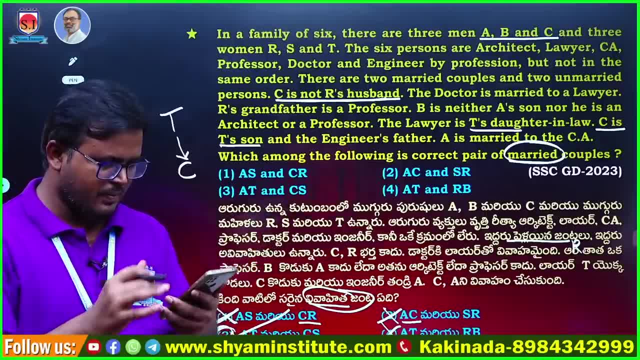 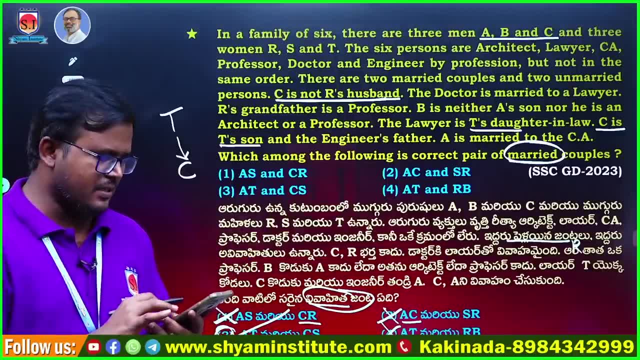 So everyone gave the third option. So very good, So very good. You are reacting very well. Look at us like this. So, in SACGD point of view, the option verification method works very well. We already got the first option. 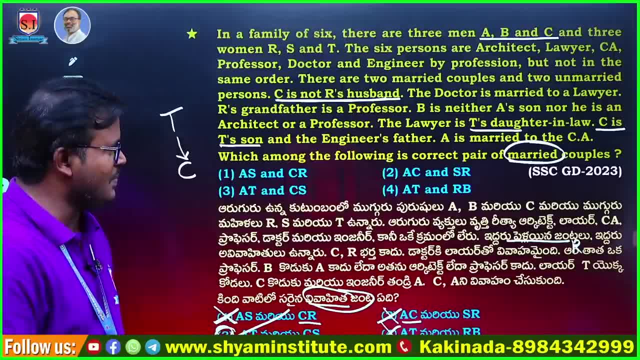 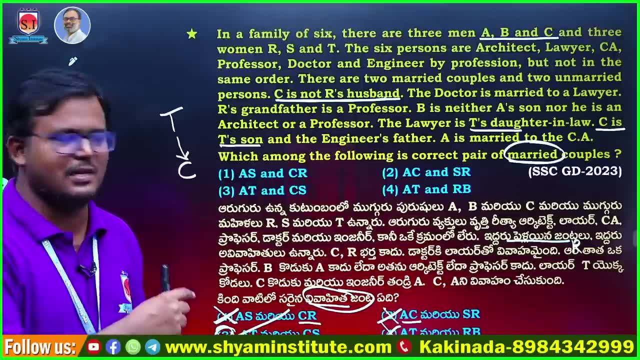 The question given in the previous exam. So the point we have to observe here is: we have to study this question first. What happens to you when you study this question In the elimination method? where the data is correct? what will you do with one option? 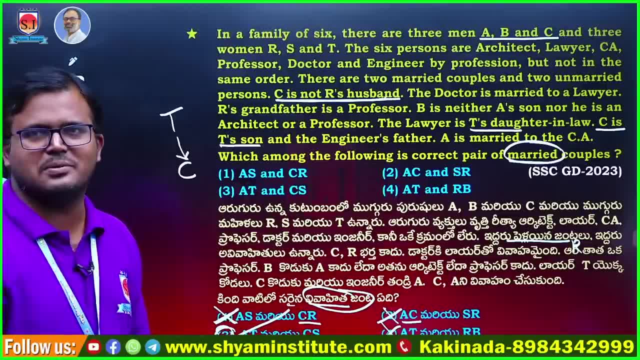 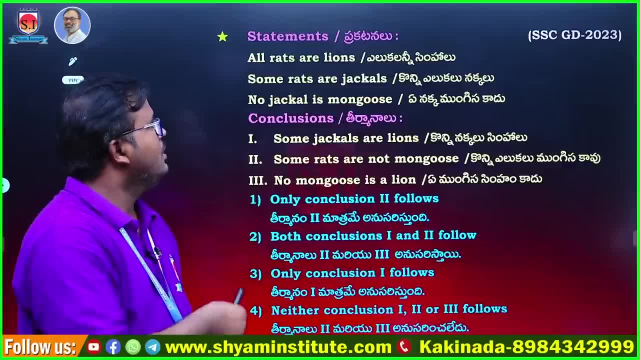 We will remove the option that is wrong and go. Only one option will be left. What is that? Here is the third option. Okay, next one. Then see, He said: all rats are lions. Next, some rats are jackals. 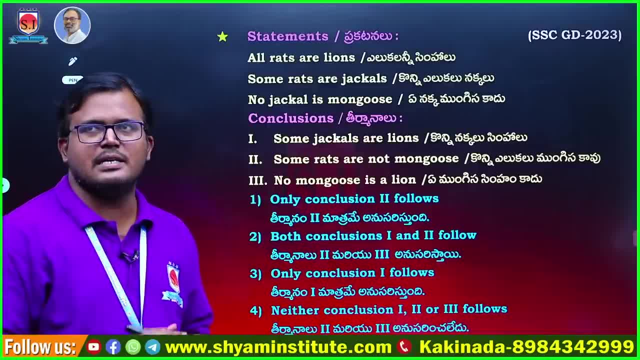 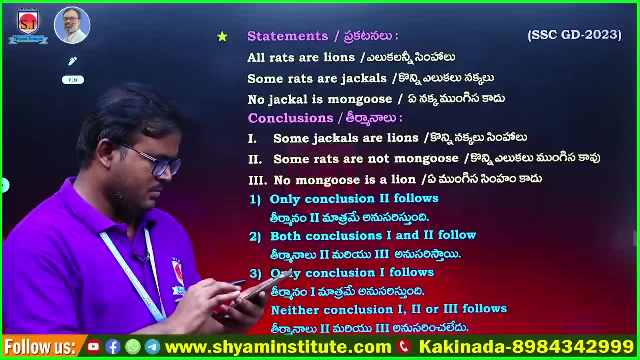 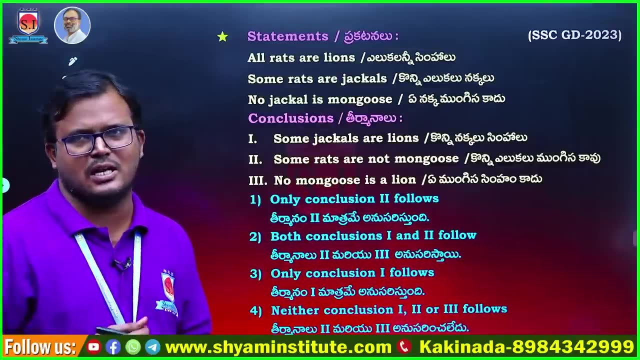 Next: no jackals and monkeys. So we got this from the concept of syllogism. I told you that we will be given questions like this when we come to the seating arrangement and facilitation, But we already have the questions given earlier. 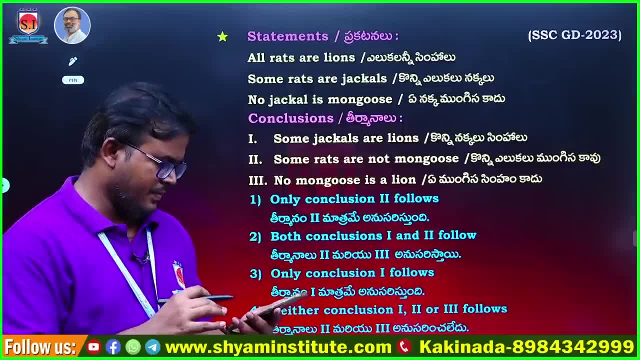 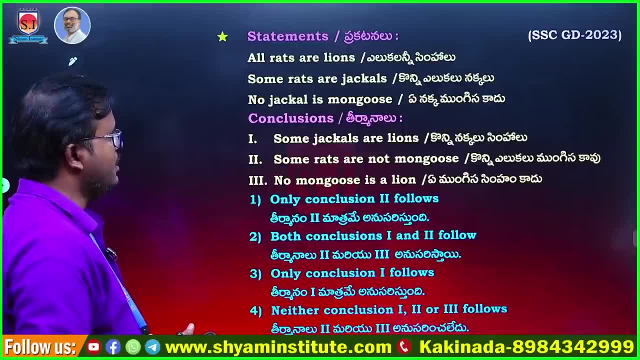 So these are the questions asked in the previous exam. Now I have to tell you what the answer is. First statement is: all rats are lions. Then some rats are jackals, No jackals and monkeys. Then, if you observe the conclusions, 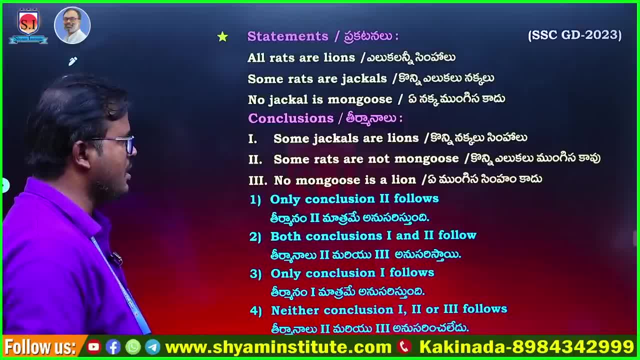 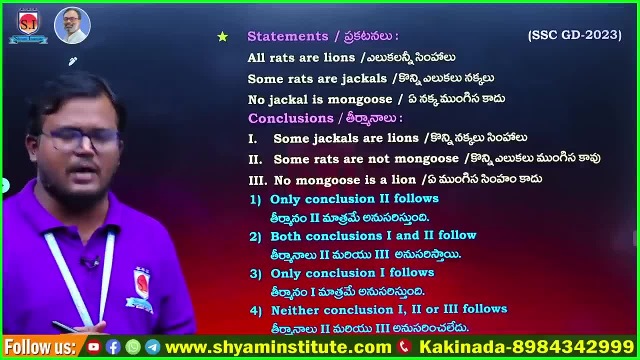 some jackals are lions, Some rats are not monkeys. No, monkeys is a lion. What will you do? First write down the answer. So you have to listen to the answer from that. So whatever you feel is correct, you can guarantee that. 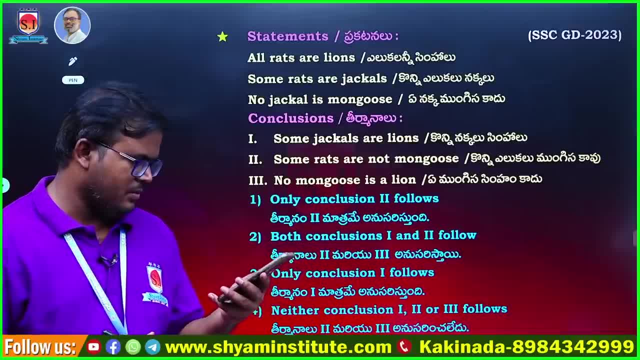 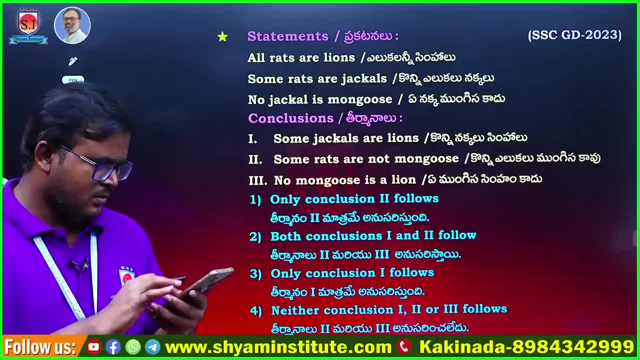 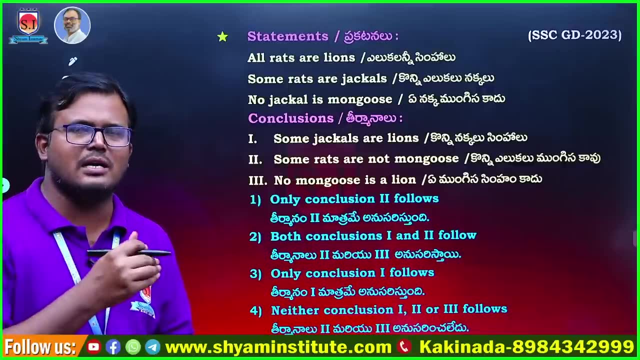 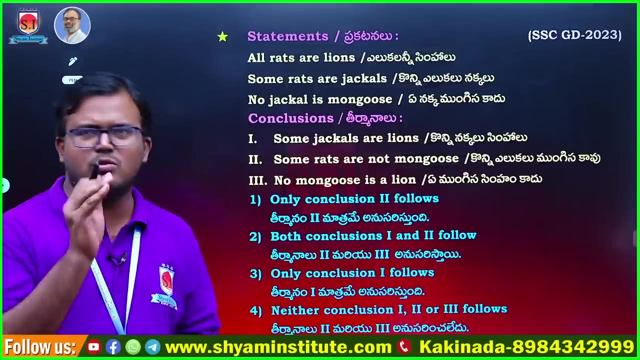 So you have to write down in the comment box. Next we have to see the answers. So what will you do? Is there any possibility that you can answer these questions without any difficulty? Then you have to make sure that you understand the answer. 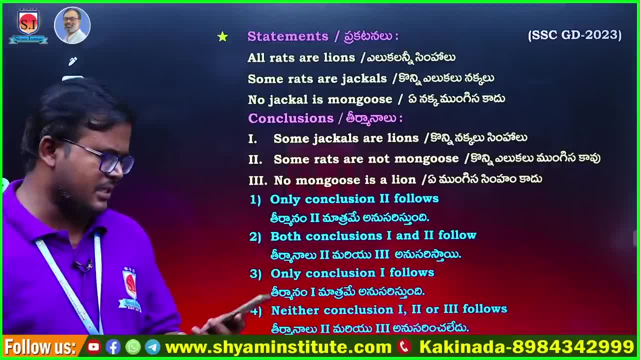 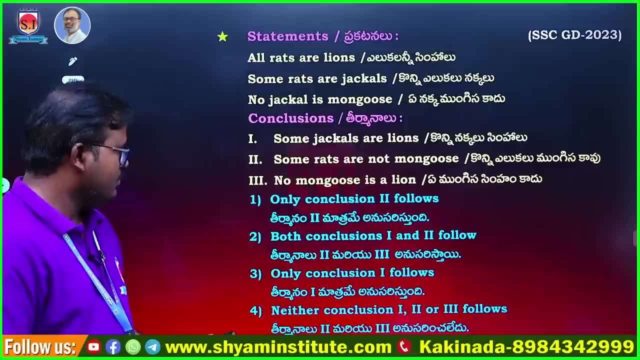 Let us see the answer. Let's see what is the answer to this question. Is only conclusion 2 followed Or both conclusion 102 followed? Is only conclusion 1 followed Or neither conclusion 1, 2 or 4 is followed? 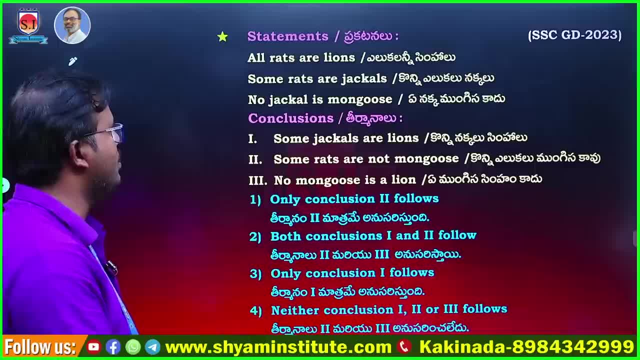 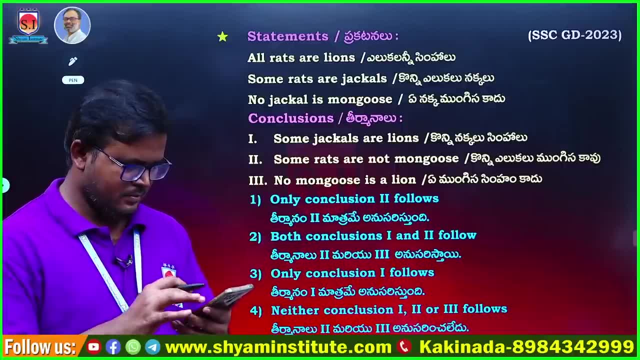 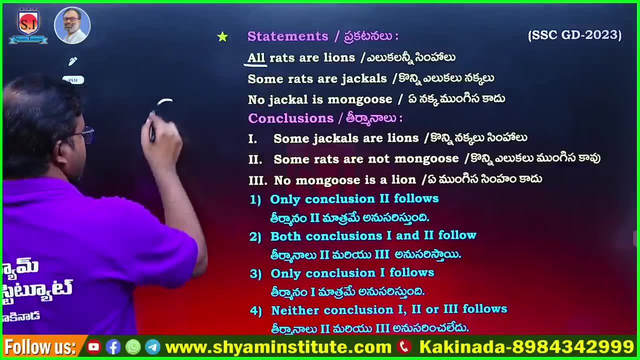 Let's check the correct answer. Let's see the first statement, Let's see the first diagram. Since all is the answer, we get the following: When all is the answer, what we do is: We don't have to worry about rats at all. 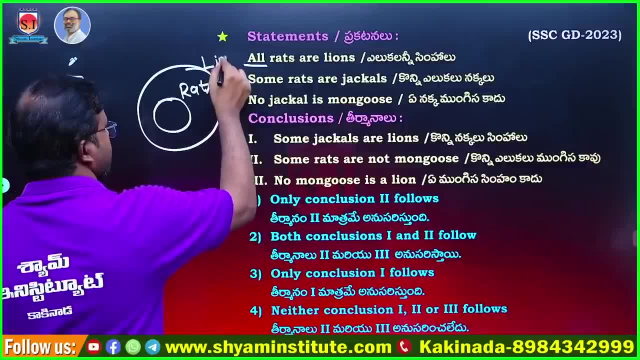 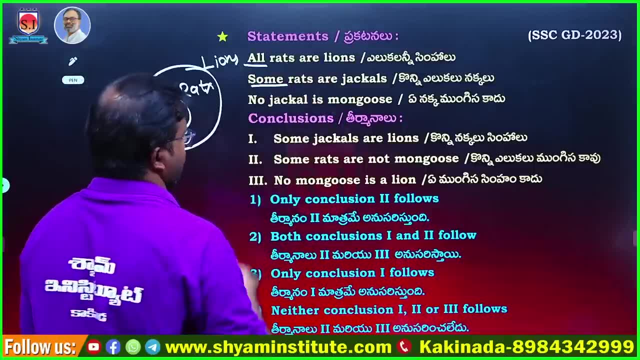 We get inside and outside are lines. Then what did he say? He said: some rats are jackals. After all, rats are lines. Some rats are jackals. So what do we have here? We have rats, So what do we do? 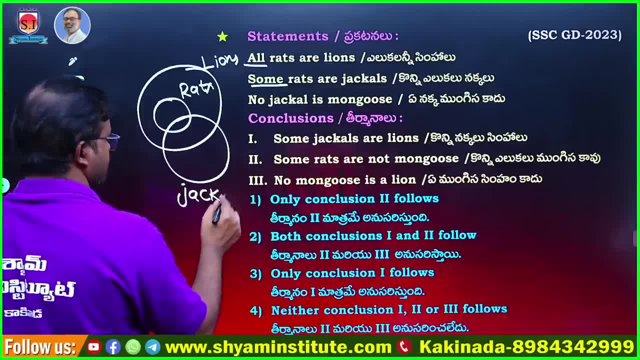 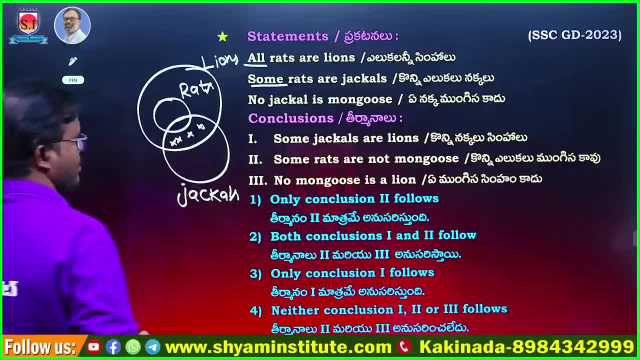 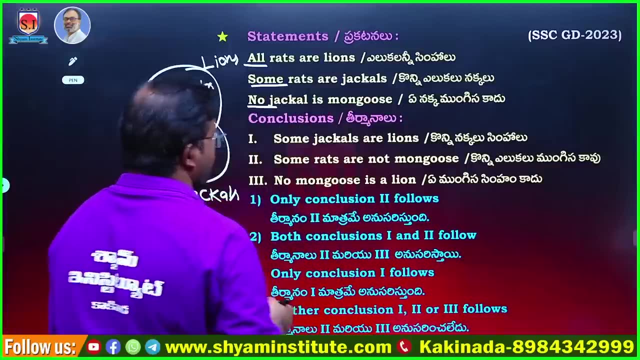 We take jackals. Now what is the condition between line and jackals? We get some condition, So remember this point. After this, what do we do next? So no, jackals is a mongoose. So what is jackals? It is not guaranteed. 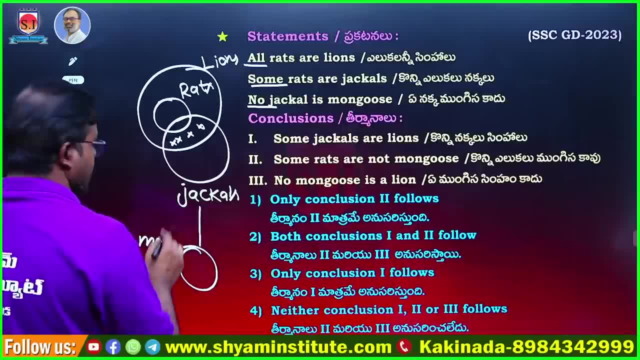 So he said it is not a mongoose. What do we write here? It is a mongoose To write. a mongoose write as mungee's. We don't have any articles about jackals. It is not a mongoose. So he said it is not a mongoese. 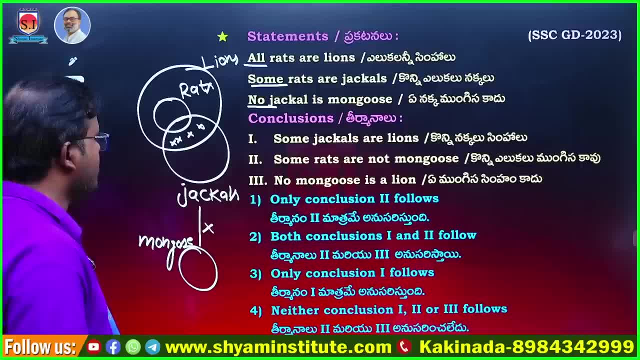 Now tell me when we come in what happens. So if you notice the conditions here, First he said all rats are lines. Next, when we come in, he said some rats are jackals. So it is like some rats are jackals. 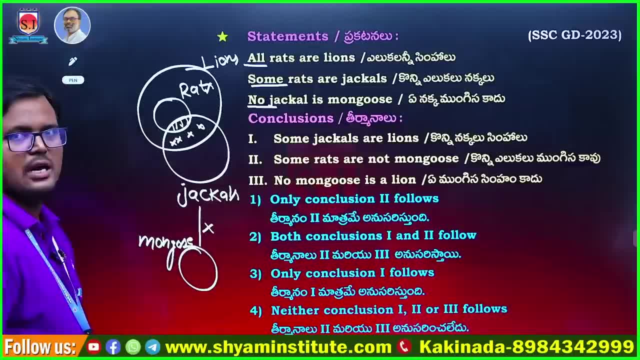 Then he said: no, jackals is a mongoose. He said: jackals are not mongooses. The first question is: some jackals or lions See the relationship between jackals and lions. Jackals are here and lions are here. What condition? will we get Some condition? 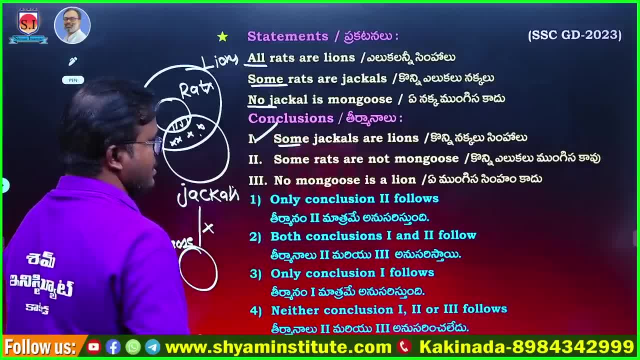 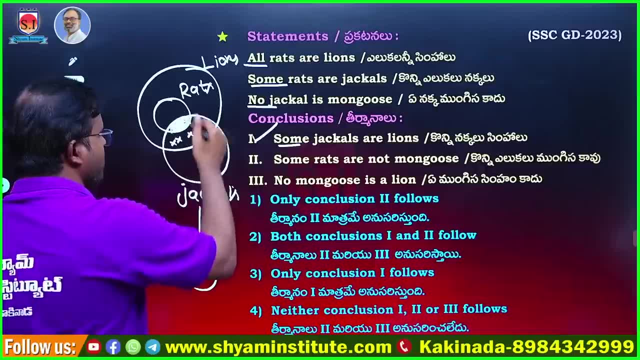 That's why it's correct. Next one is some rats or not mongoose. As you can see here, there are some rats in this. What does this mean by rats? What does it mean by not mongoose? It means that they are not mongoose. 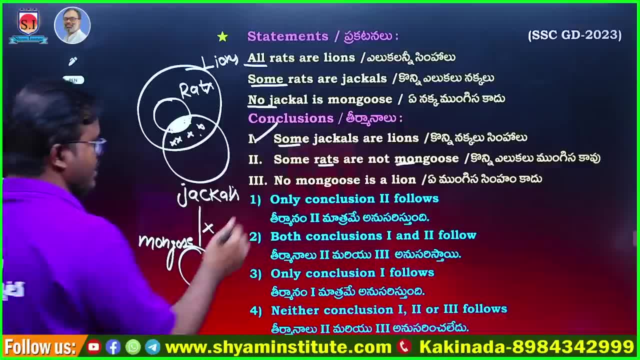 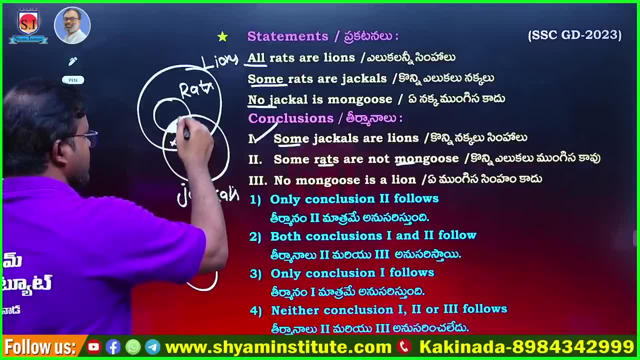 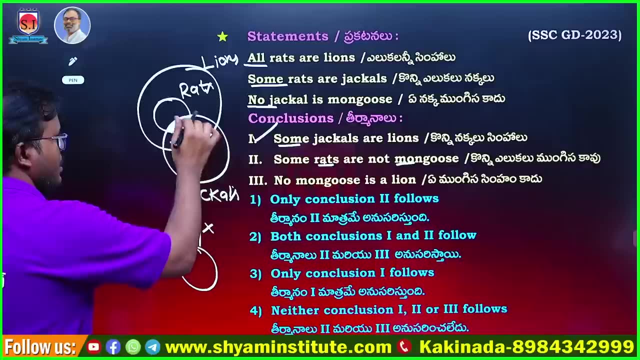 Let's see the situation As we are talking about rats. where are these rats? They are in the jackals. What is this small part in the jackals? It is called not mongoose. It has nothing to do with mongoose. What is this small part? 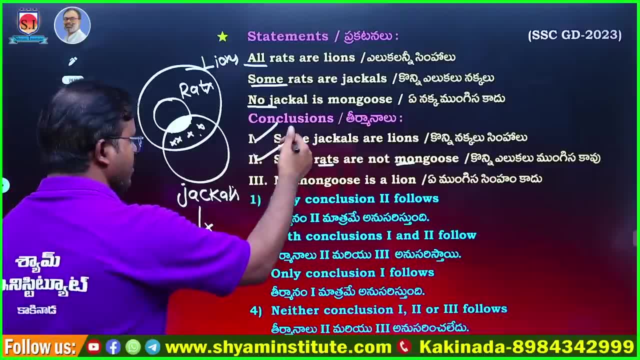 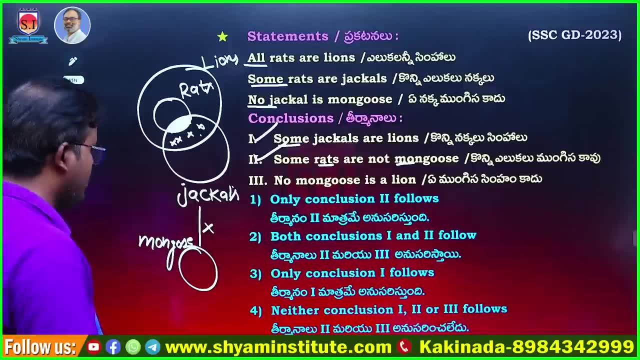 It has nothing to do with mongoose. It is correct that it is not mongoose. Next one is when we come here. no, mongoose is a lion. So mongoose is here and so is the lion. He said that mongoose is not a lion. 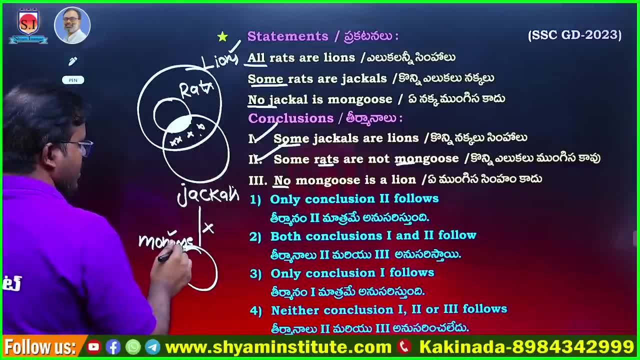 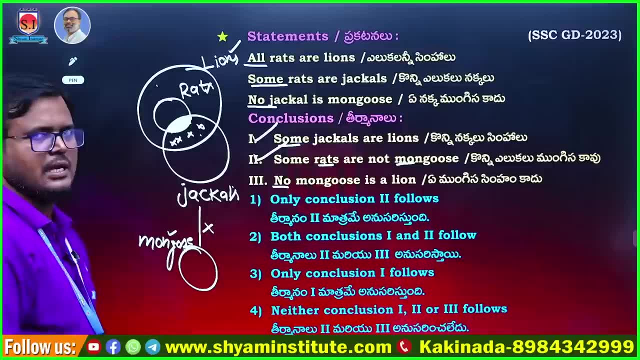 We should not say that mongoose is not a lion, Because when we say that mongoose is not a jackal, if this mongoose came here as a giant, there are chances that it will come to us, But this is not a one-sided statement. 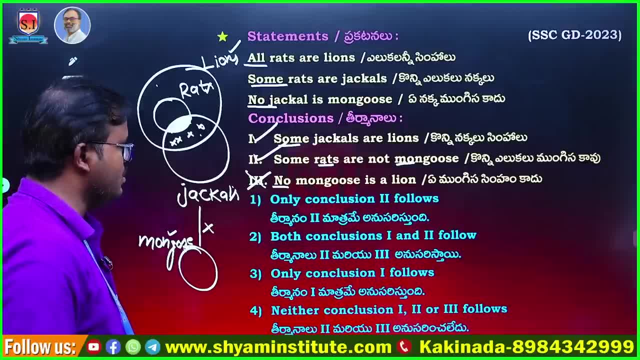 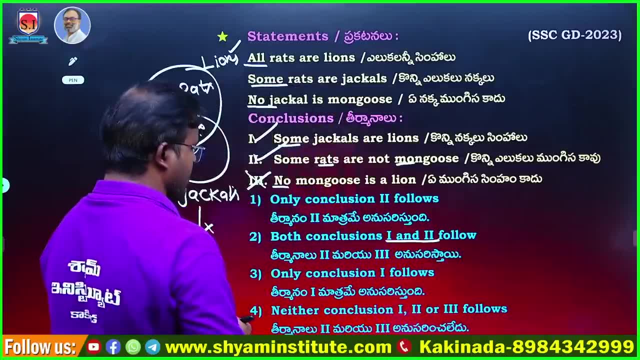 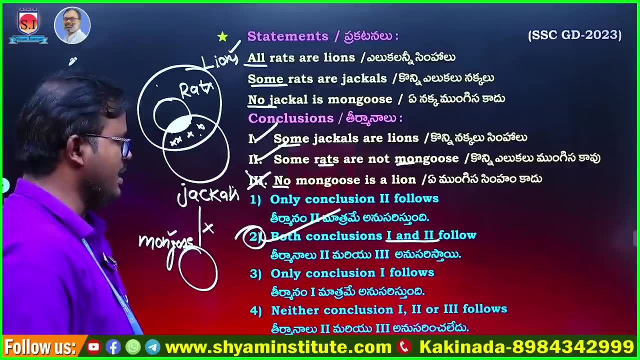 So what happens to the giant is wrong. So only conclusions 102 follows. If you observe, both conclusions 102 follows. So where are the options? Both conclusions 102 follows. So option number 2 is the correct answer. So what happens is: 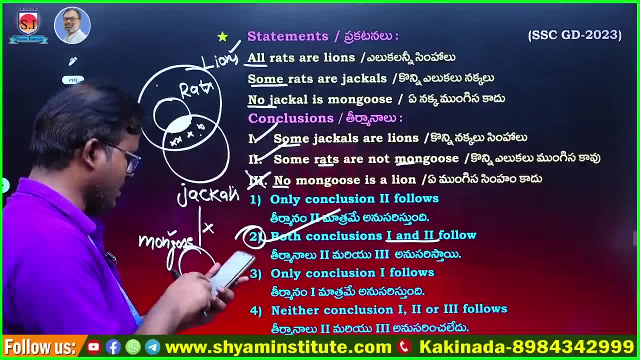 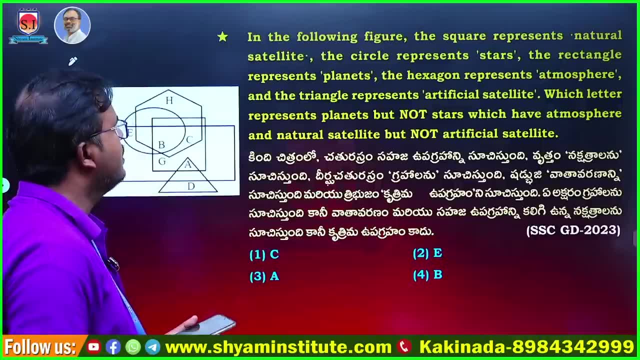 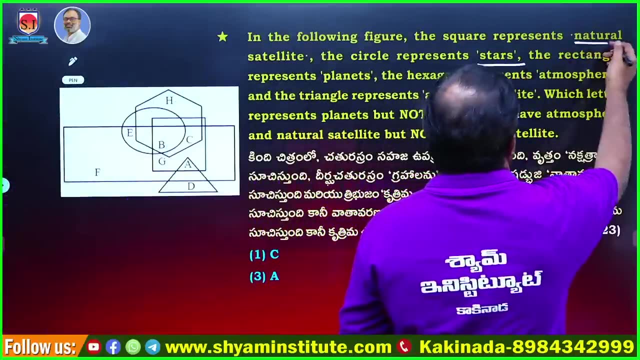 both the conclusions are correct, So the second option is the correct answer. Next problem: In the following figure the square represents the natural satellite, The circle represents the stars. So we have to observe once What are the natural satellites. So the circle represents the stars. 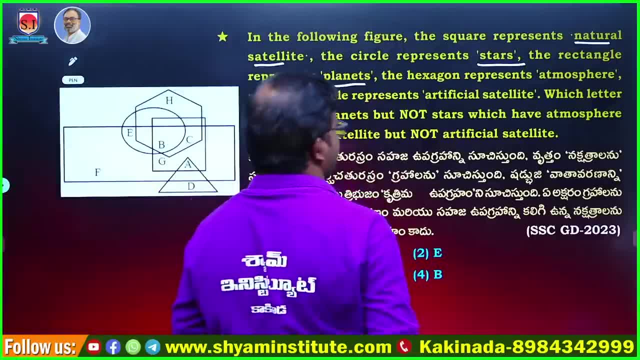 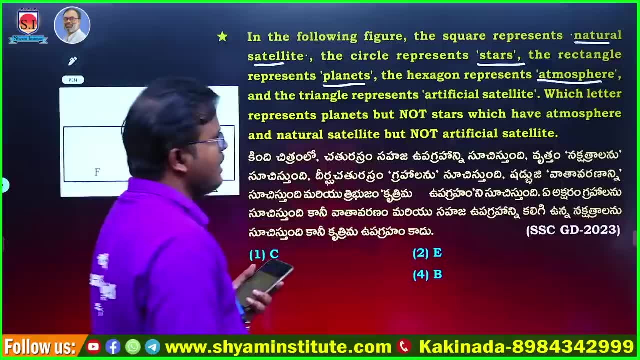 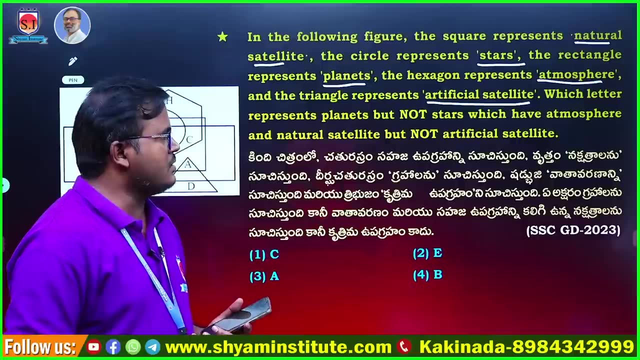 The next rectangle represents the planets, The next hexagon represents the atmosphere, The next triangle represents the artificial satellite. So what did he ask The vigilator? represents the plants, but not the stars, which are the atmosphere, and the natural satellite, But not the artificial satellite. 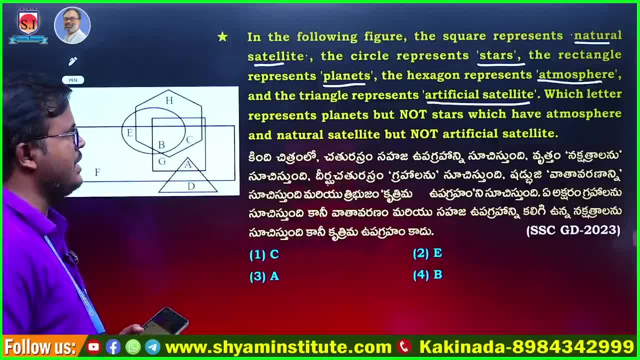 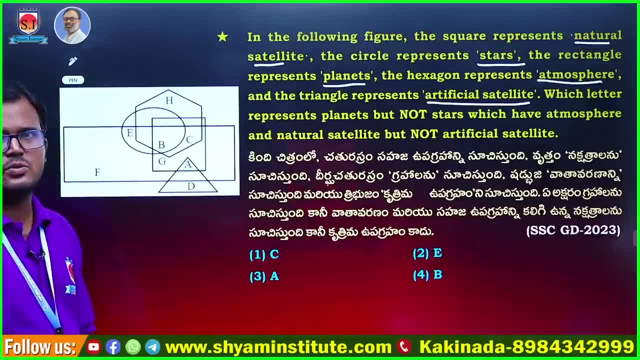 He said it is the natural satellite. So what you have to do from this diagram is you have to tell us the correct information about the information given by him. So tell us the answer by looking at this diagram. You have to tell us the answer in the comment box once. 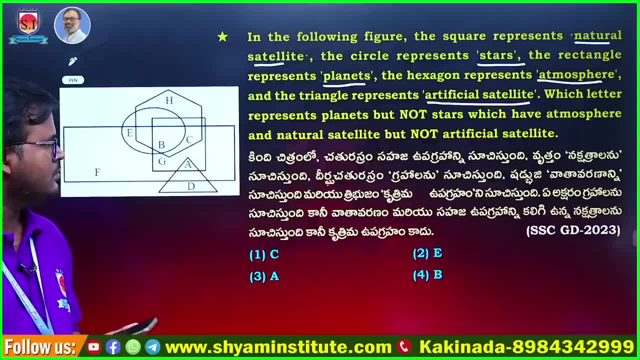 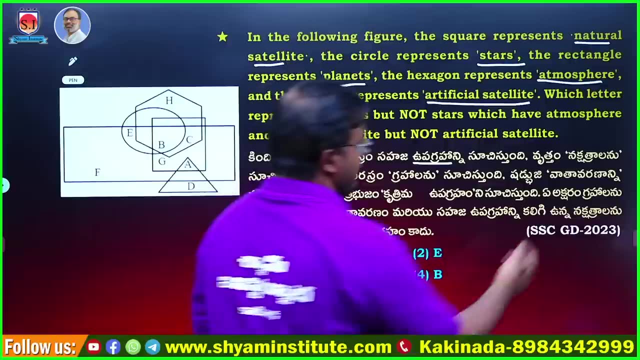 See what are the diagrams given here. So, according to this diagram, we have to see which is correct when it comes to it Here. what he said is: the circle represents the natural planets, The circle represents the stars, The square represents the planets. 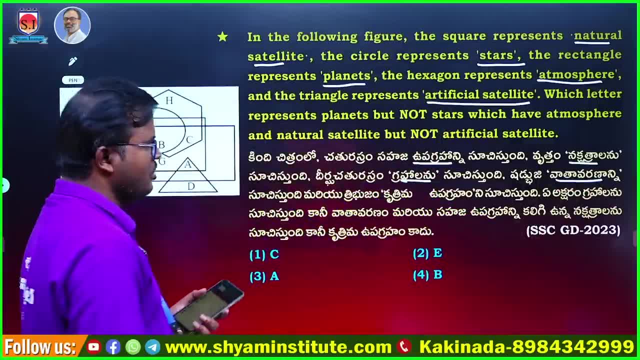 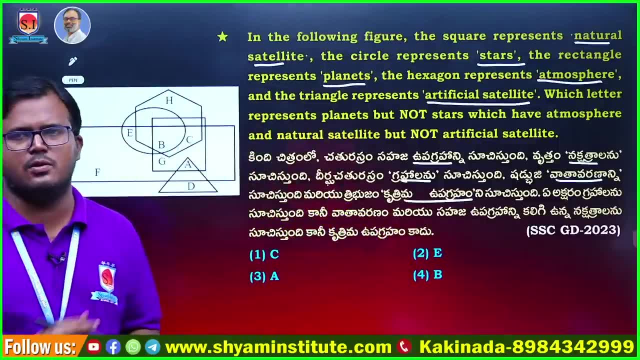 The circle represents the atmosphere. When the triangle comes, we are told about the natural satellite. So what do you do? So what do you do When you take this diagram? what is the diagram given to us? What is the question given to us? 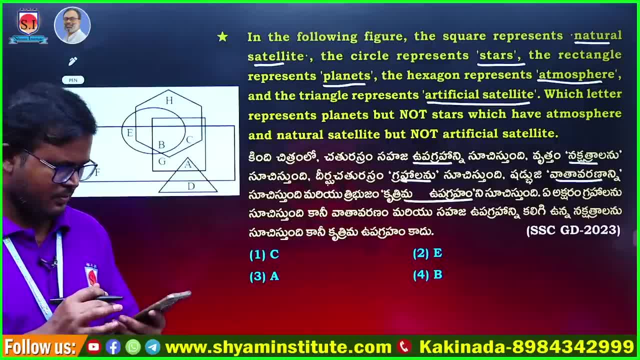 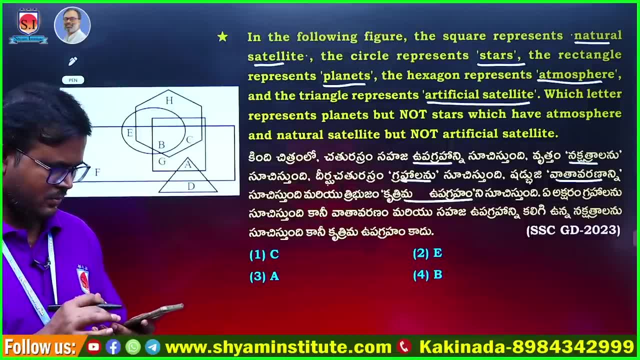 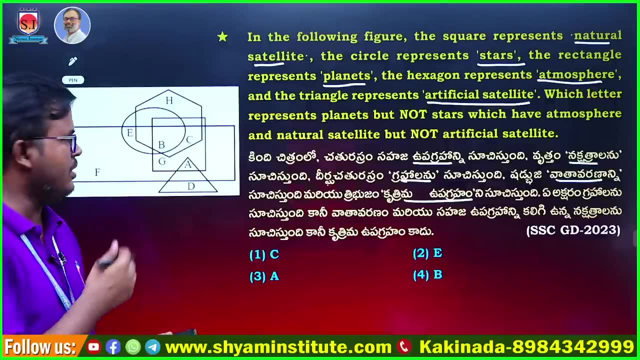 that is given to us through that diagram. Read it once. You have to tell us. You have to tell us which answer is correct. What is the answer given to us through this diagram? So what is the answer given to us through this diagram? 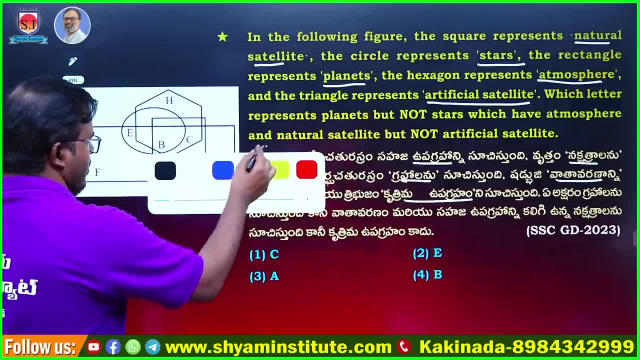 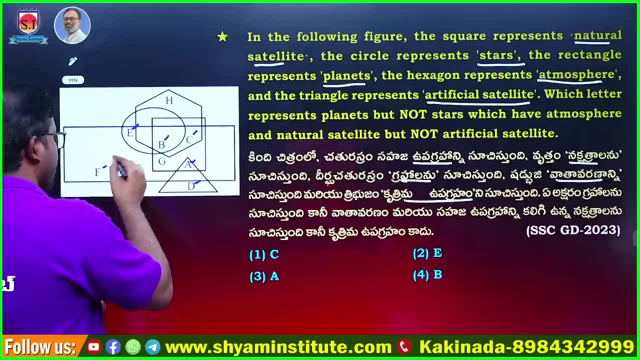 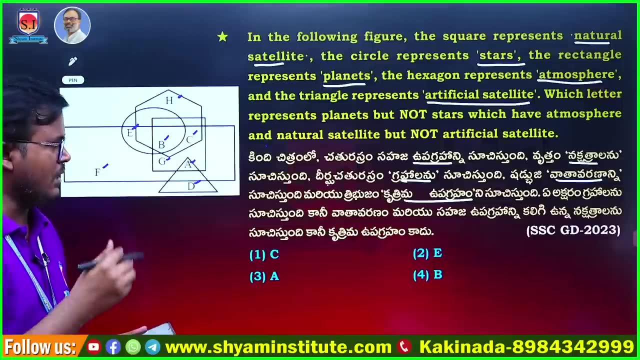 They gave us letters here, First letter A, then letter B, then letter C, then letter D, then letter E, then letter F, then letter G and finally letter H. They gave us letters from letter A to letter H. There is a letter in those letters. 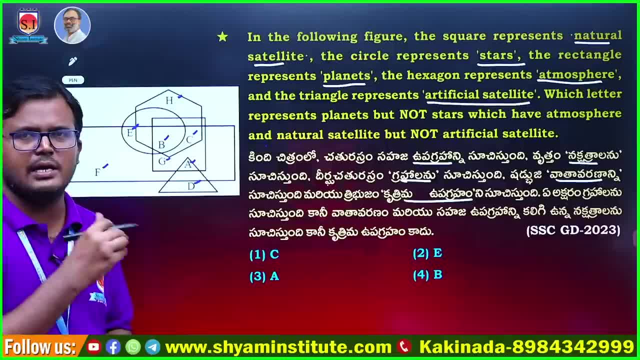 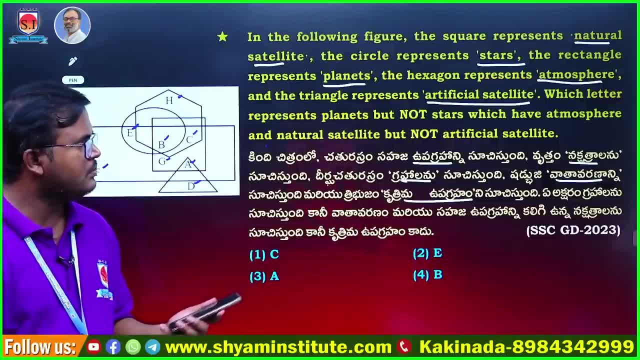 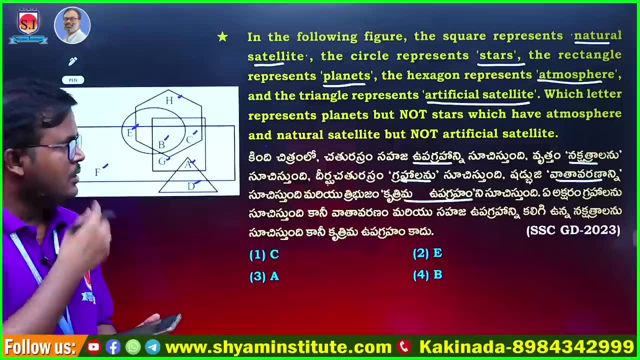 The quality of those letters is the same as the quality of those letters. You have to tell us what is the letter in the options, Tell us what is correct in the options given here in the comment box. So what will you do when given like this: 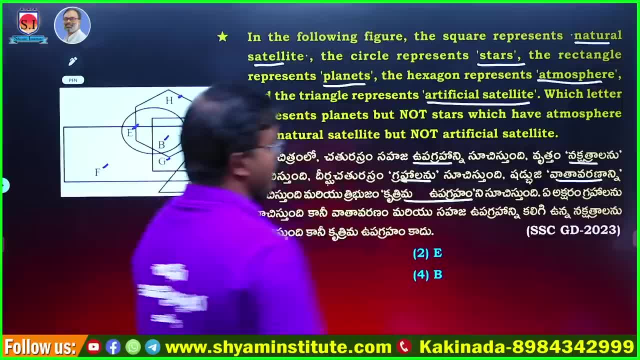 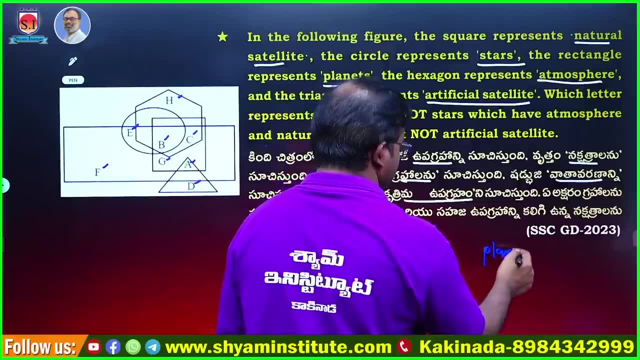 You have to remember one thing First, the question should be clear. So what did he say? Which letter represents planets? What should be guaranteed? It should be planets. So what do you write first? It should be planets. What did he say? 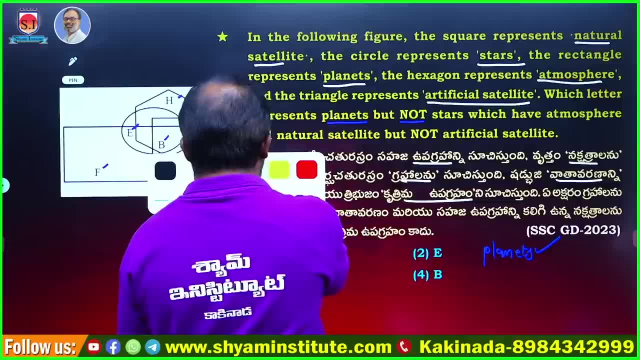 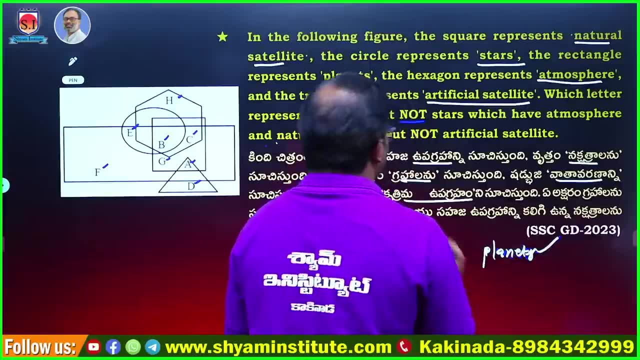 But not stars. There should be no stars here. So when it comes first, what should be guaranteed? It should be planets. Then what did he say? when it comes next, Stars. So the stars should not be anything like that. 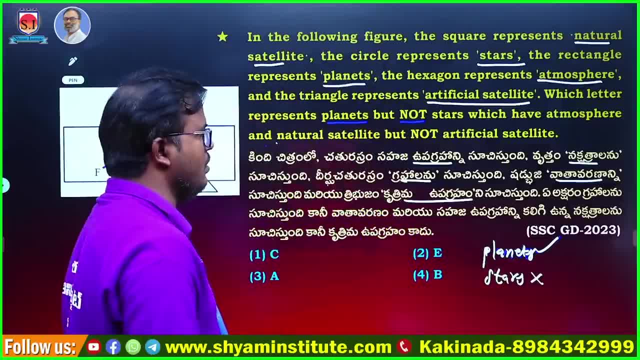 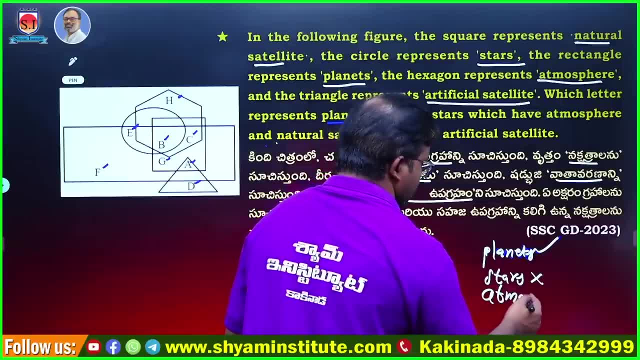 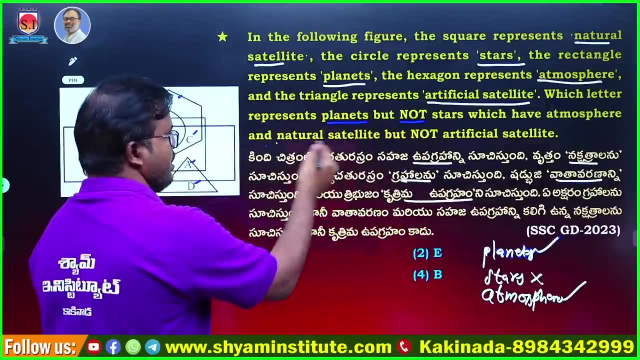 What he is saying next is: It should be an atmosphere. What does it guarantee It should be an atmosphere. When it comes next, the atmosphere should be coherent. Another thing is it is not allowed to mention natural satellites. The one that is included in this question should be a natural satellite. 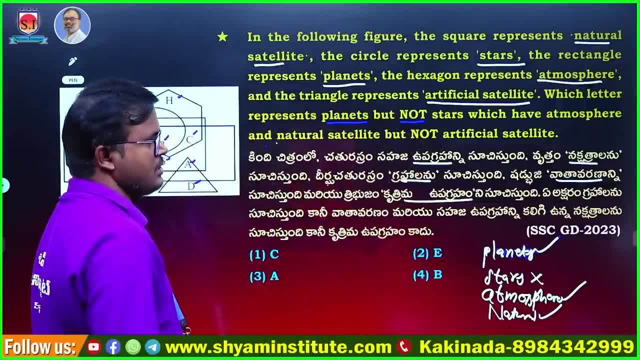 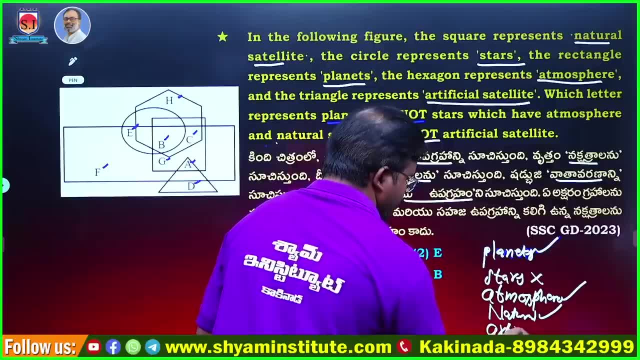 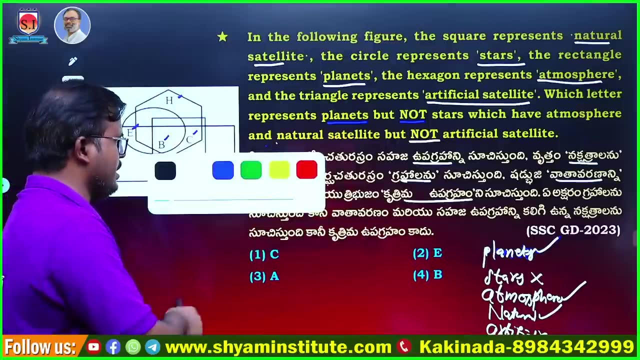 It should be a natural satellite. The next one is not artificial satellites, But it is a guarantee that it is artificial. If it is an artificial satellite, it should not be a satellite. To answer this question, we have to pay attention to the time, as it is a guarantee for us when we answer the question. 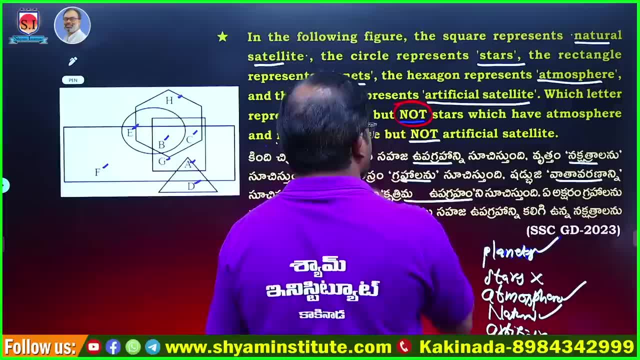 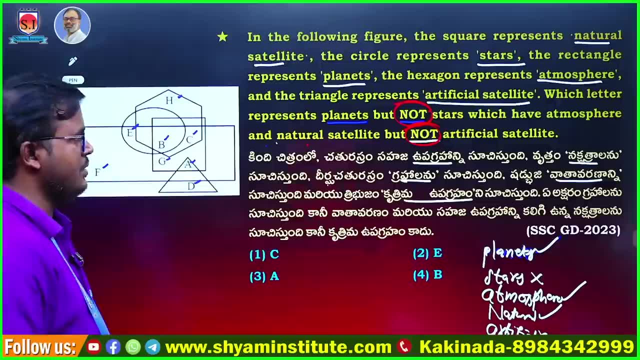 So what you have to do in such questions is first tell us what is here. He said not stars. Next, he said not artificial satellites. Then observe stars. So if we observe stars, tell us what is here. So where should stars be? 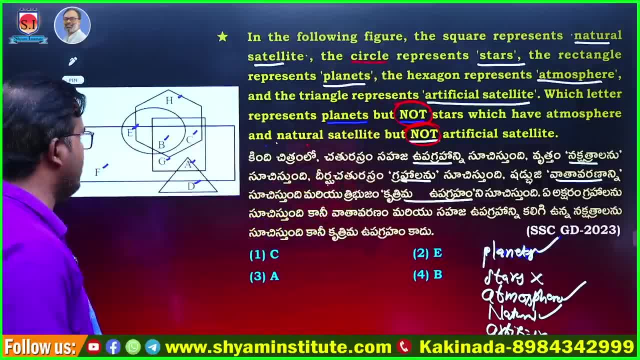 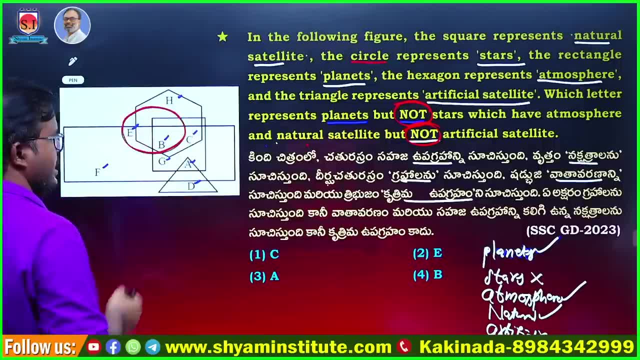 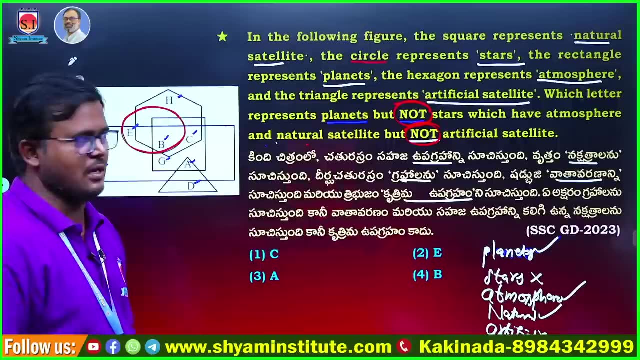 They are in this circle. So see what is a circle, If you observe this circle. there is a letter B and a letter E here, But when we come to the place where it is a guarantee, it is said: not stars. Since it is not stars, what happens to us as a guarantee? 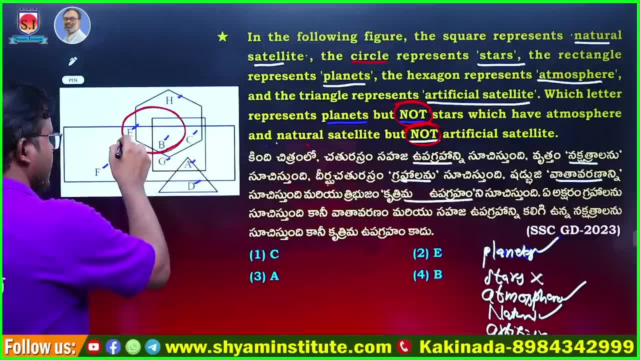 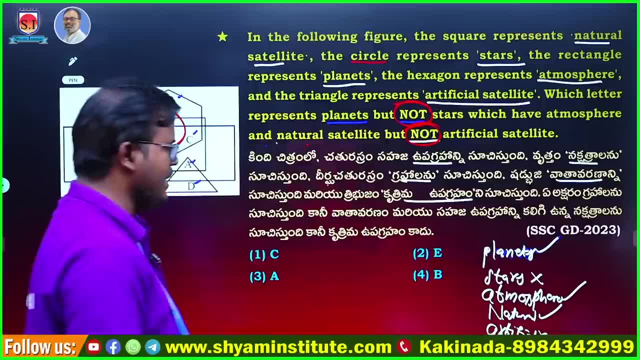 So if we get a letter B and a letter E as answers, it will not happen. If we come to that place, what happens to us? as a guarantee, They will become stars. But since it is not stars, what will they do? completely? 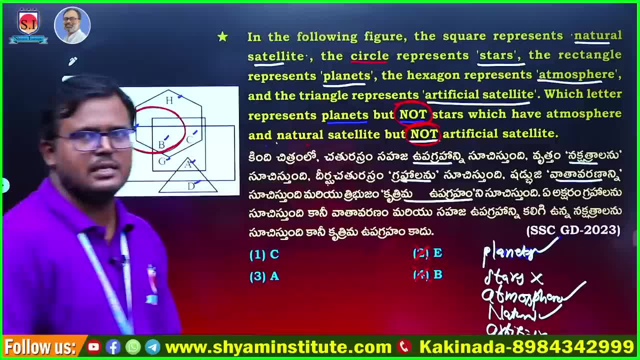 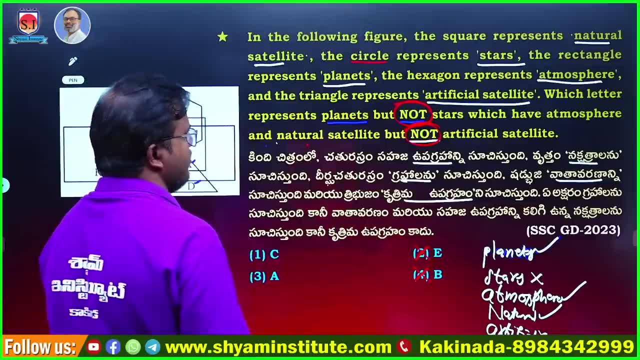 So first cancel the letter B and the letter E. These are not answers. Next, where is the word not? It is artificial satellite. Then where is the word artificial satellite? It is a triangle. Then come to the triangle. 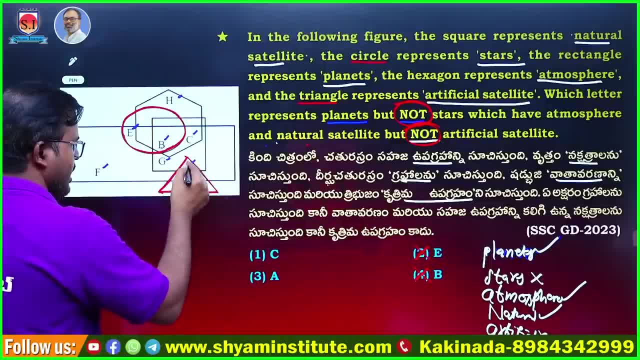 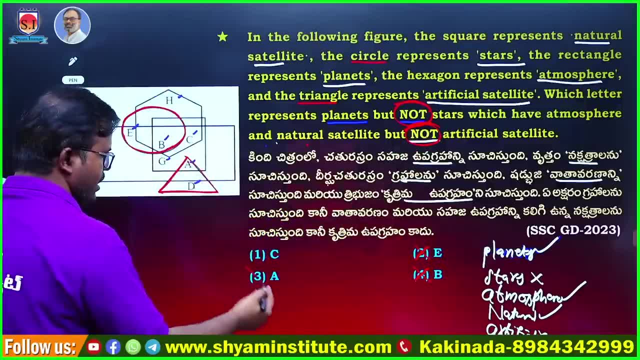 So tell us what letter is there in the triangle? There are E and D letters in the triangle, But since it is not stars, we should not come to the option. But since it is E, there is no answer to this. So we will get the correct answer as a guarantee. 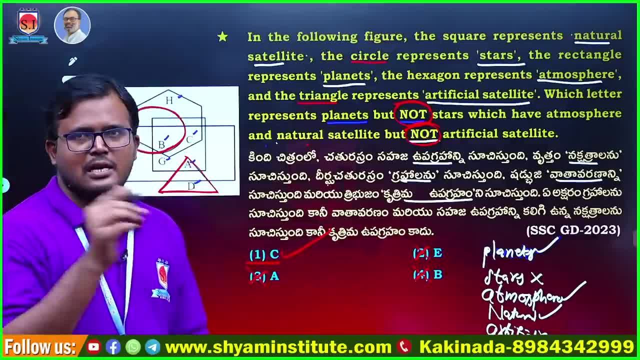 So what is the option? We will get the first option here. If we take it as a letter, we will get the letter C. So when we are given a question like this, if we do it according to the points here, 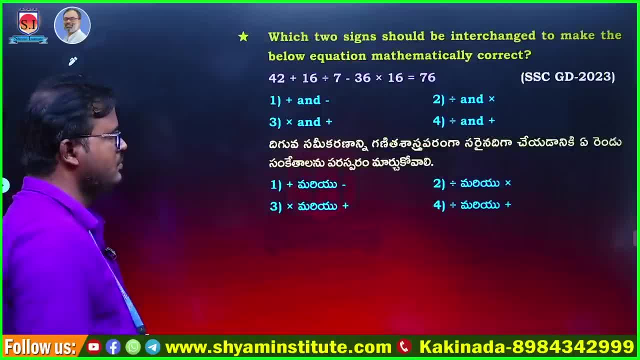 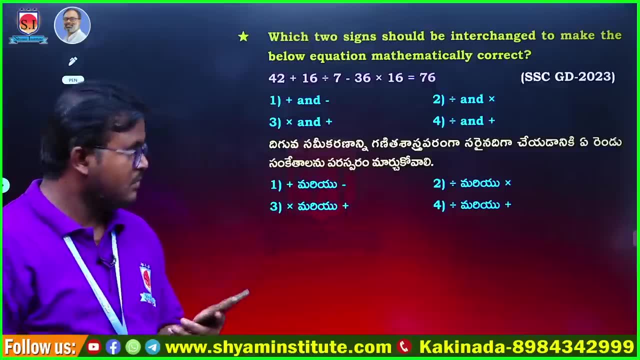 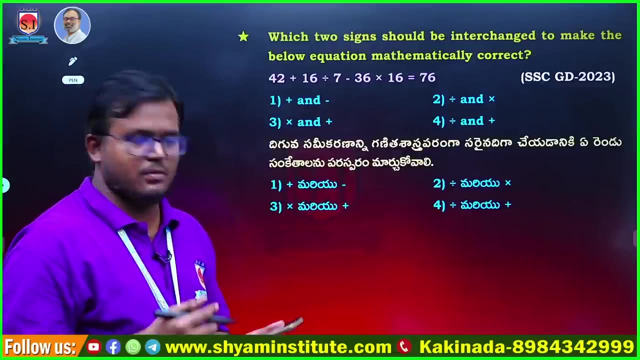 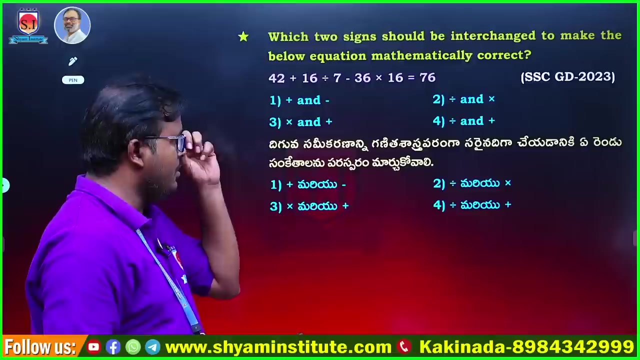 we will get the answer soon. Okay, next problem. So which two signs should be interchanged to make the given equation mathematically correct? So if we take it mathematically, this equation that I gave here, when we have to come to the correct answer, 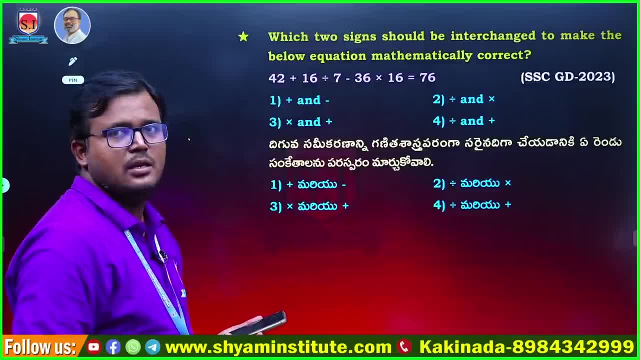 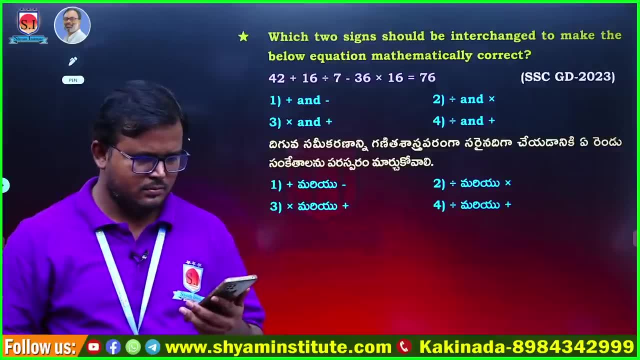 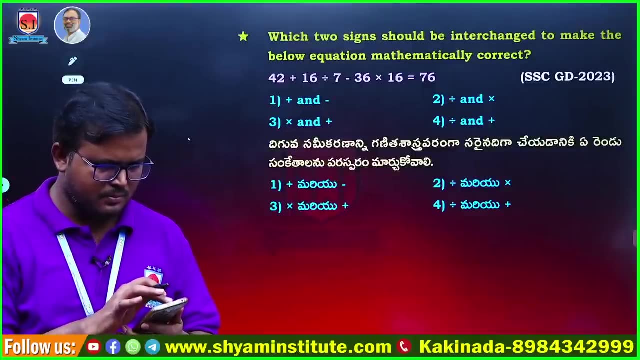 we should change the two signs compulsorily. He asked: what are the signs that we should change? So tell me what is the answer to this. So tell me what is the answer to this. So what is the answer to this? 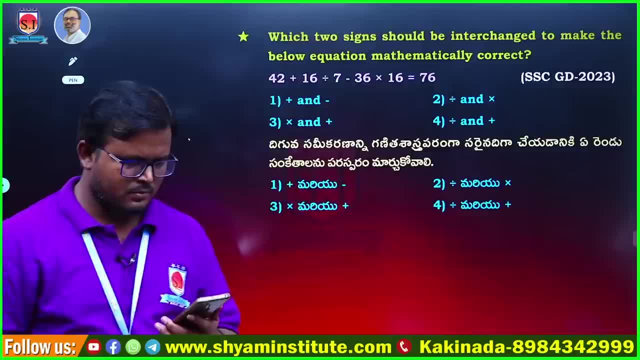 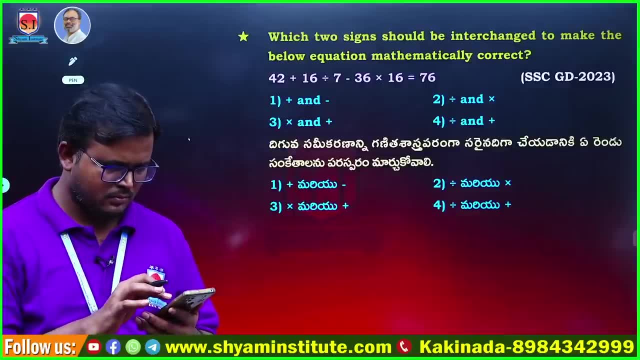 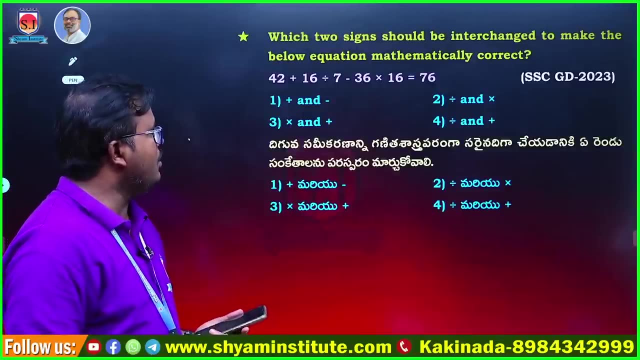 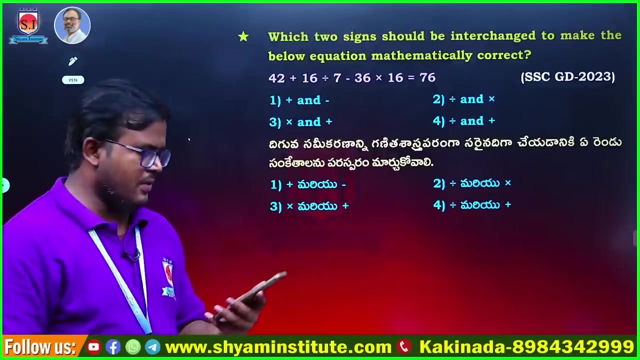 So what is the answer to this? So once you have to write in the comment box 42 plus 16, divided by 7 minus 36 into 16, that is equal to 76, and the answer should be so here you are saying that if there are two. 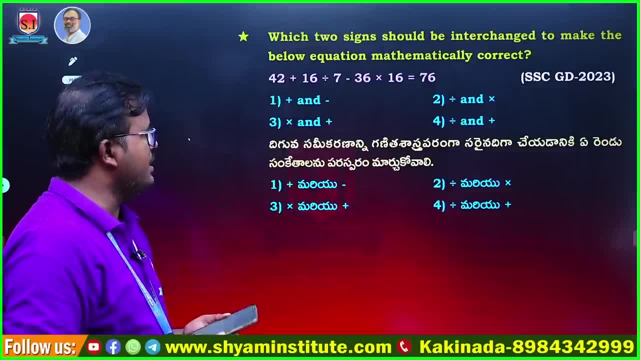 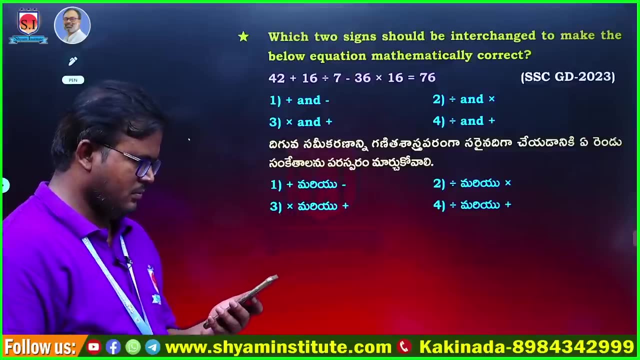 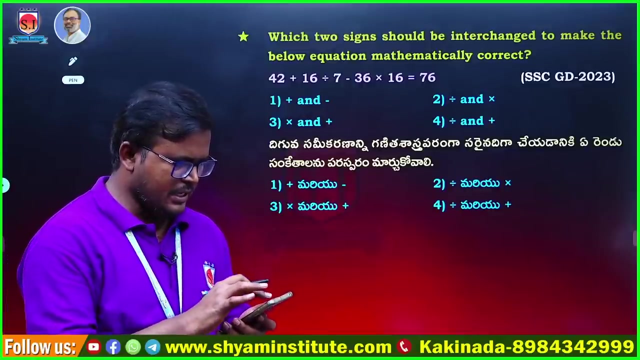 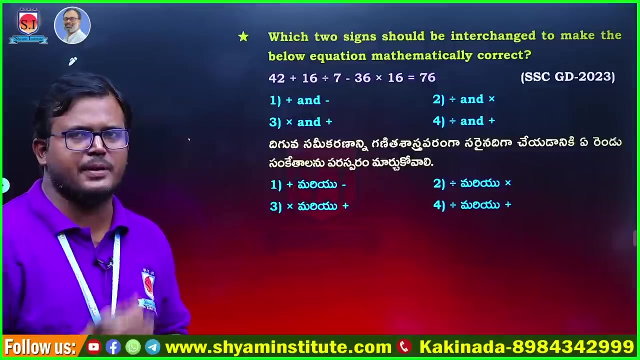 symbols, then you should change it. then what are those symbols? if you change the symbols you will get the answer. Tell me in the comment box once which answer is correct for this, because we have SACGD point of view from the concept of mathematical operation. so there are two questions in the 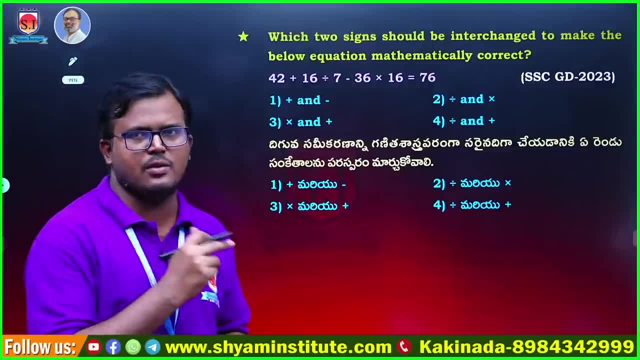 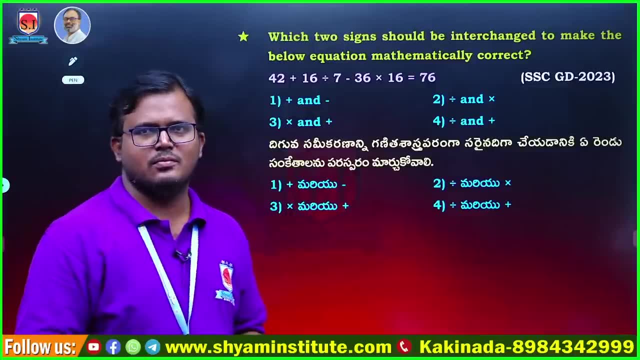 exam point of view from the first question. this model question will be guaranteed. If you look at the question paper you can see that we have given it in every ship. So you have to tell me in the comment box once which answer is correct for this. 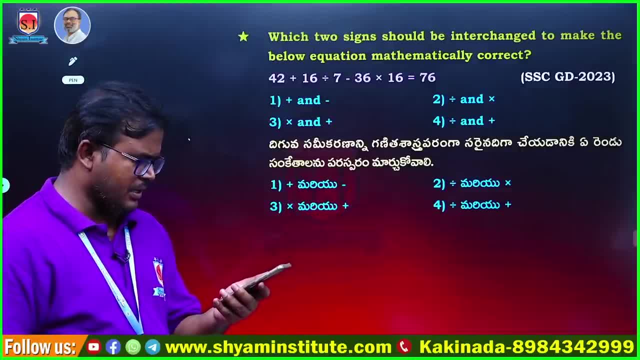 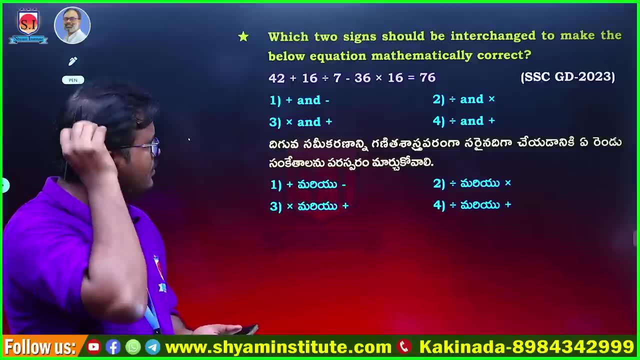 So, as you can see here, you gave the fourth option, some gave the third option. So let's see if the third option will come or the fourth option will come. So what should you do for a number 706? You said that there should be a number. 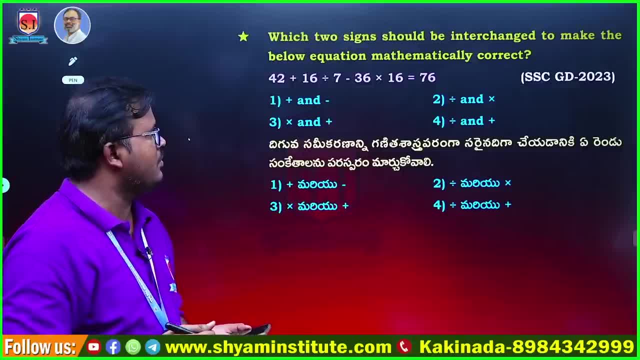 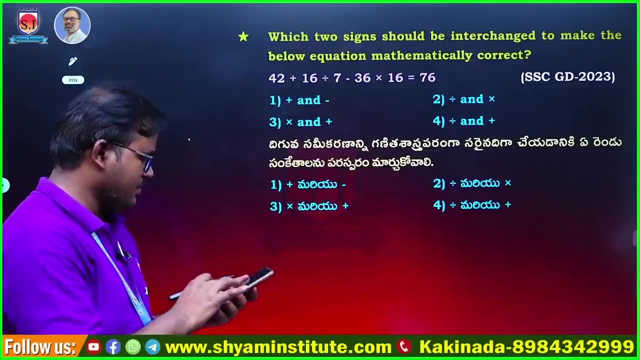 So a number called 706 should come. so what should we say for that number? you should see what option comes from it once. So when you are like this, what will you do? so the number on the right side, but 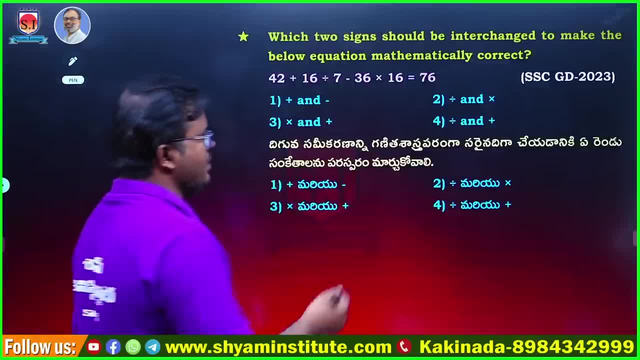 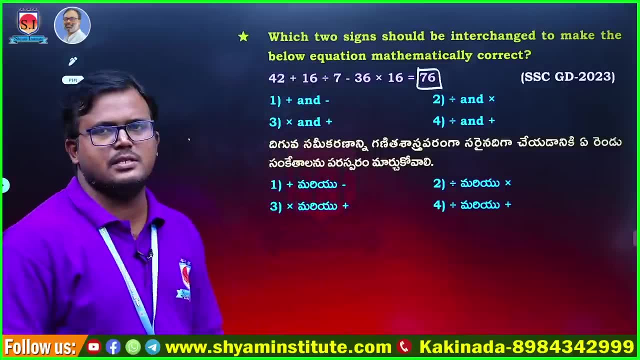 this number is not there. this number is 70, so you should first observe the number and make an answer to this number. So what can we do when you have a number? and in case you have the answer, what should we do here? 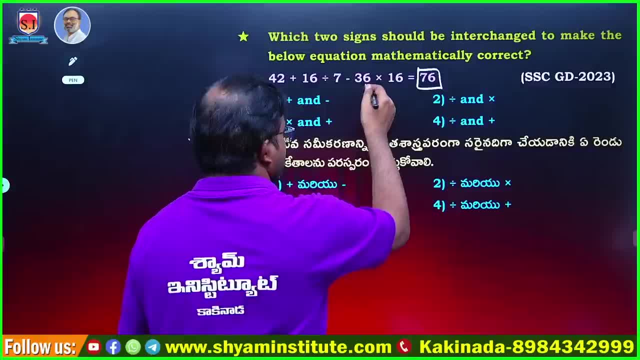 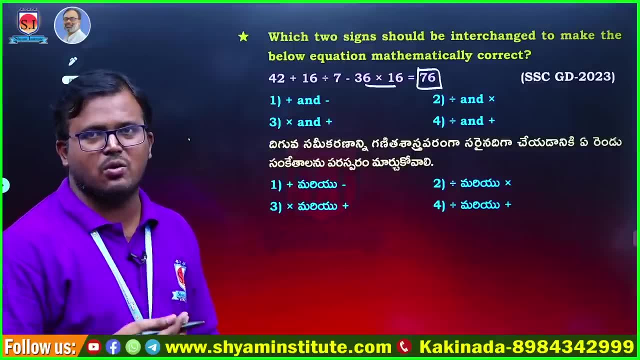 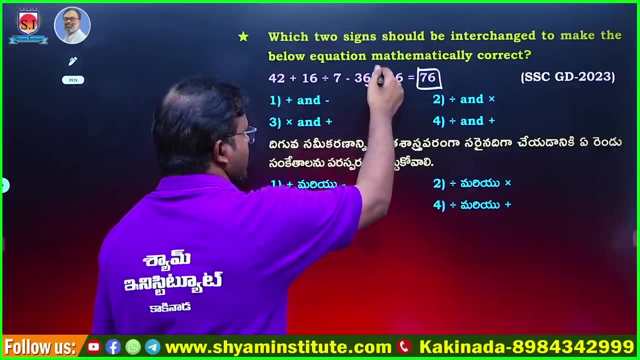 So then the first option is questioned, which is 786.. If you multiply 36 by 16, the value will increase. If the value increases, there will be a minus sign in front. If you want to change the symbol, you have to be in the option. 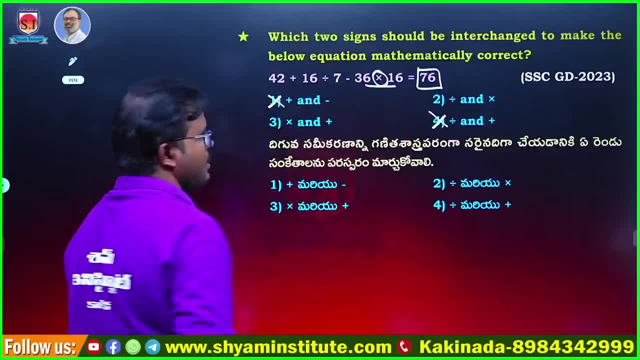 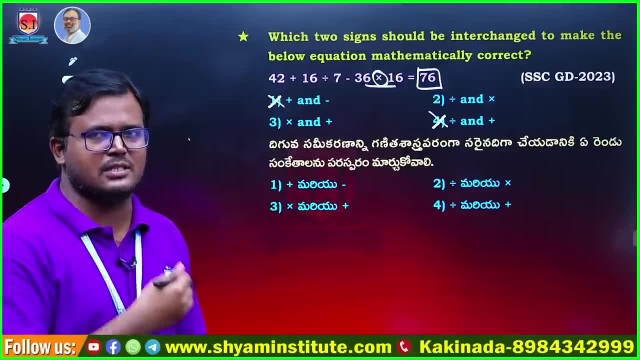 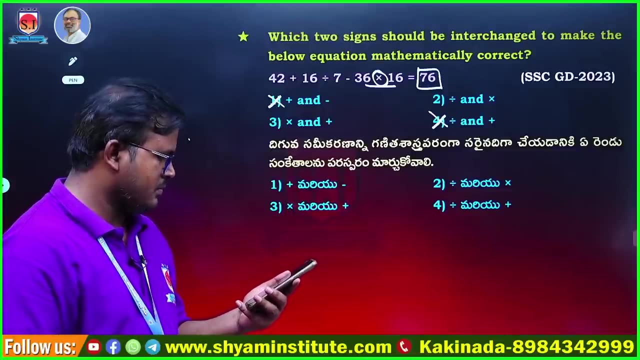 But there is no option in the fourth option. If these two options are guaranteed, we will be wrong. There are only two options. Check one of them and you will get the answer. You have to do it quickly. If you follow this technique, you will get the answer. 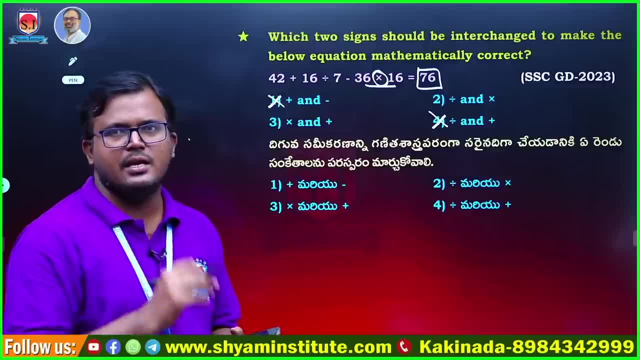 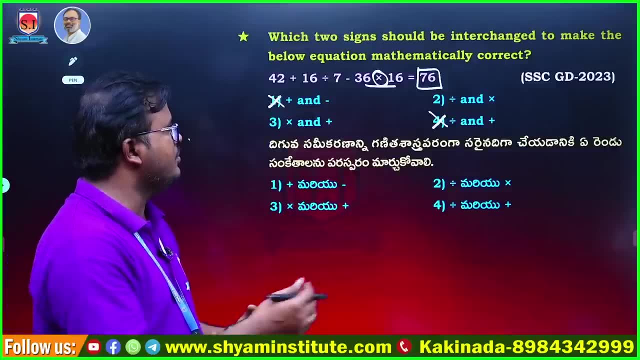 Here we have two options, second and third. If you try one of these options, you will get the answer. If you try one of these options, you will get the answer. Here we have two options, second and third. Then what will be the answer? 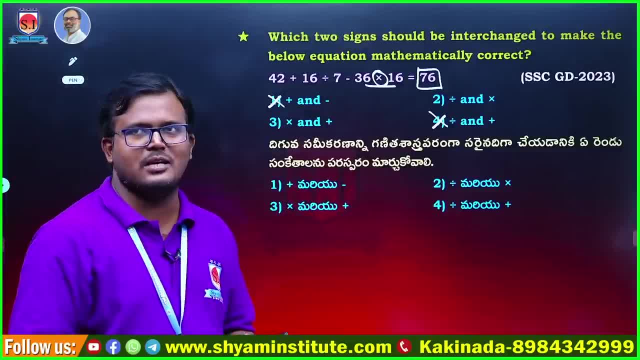 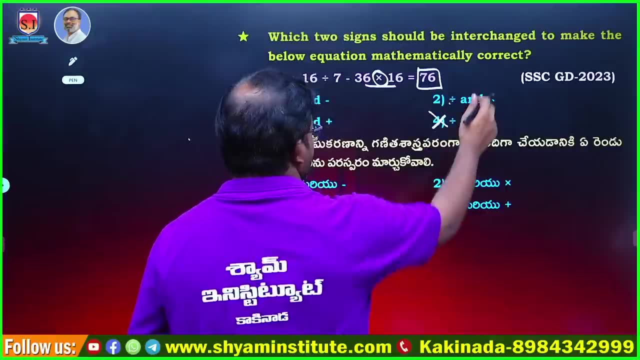 What will happen if you choose the second option? Let's think about the second option first. So what do you have to do according to the second option? Here there is a divided by, and here an into, Because we have to change the two options, and so 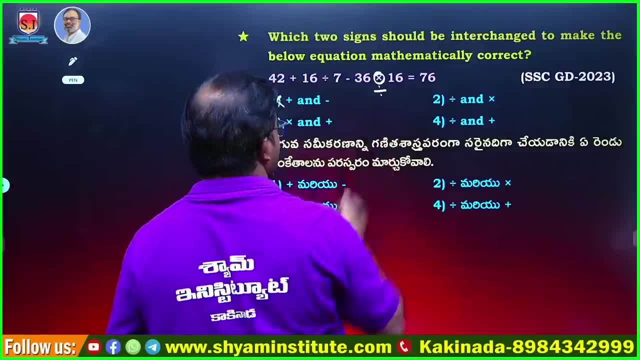 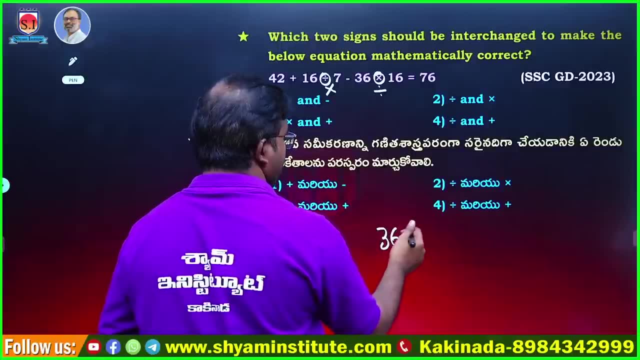 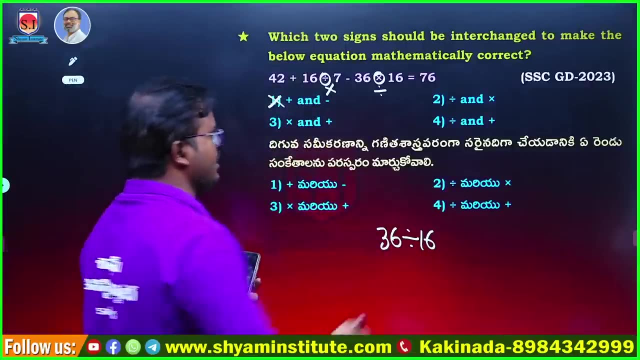 what did I do First? I wrote dies by at intu. Now give me the position on 36.. If you divide 36 by 16, will you get the 36th number in the 16th table? If you don't get it, what is the guarantee that you will get the answer? 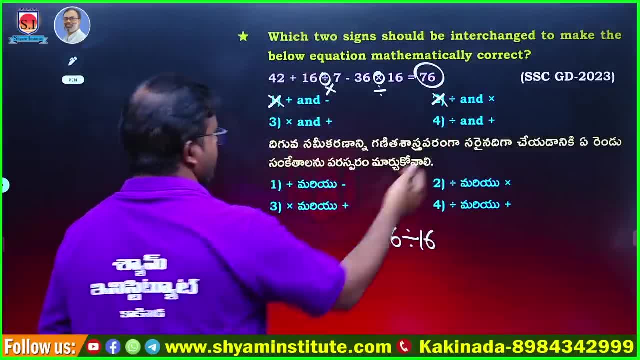 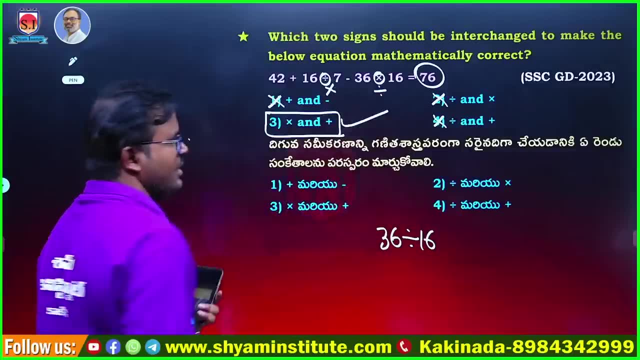 Because we need to get the number 76. Now tell me what is the guarantee that we will get the answer? What is the remaining option? Third option: You don't have to answer, Just look at the options and cancel the first one. 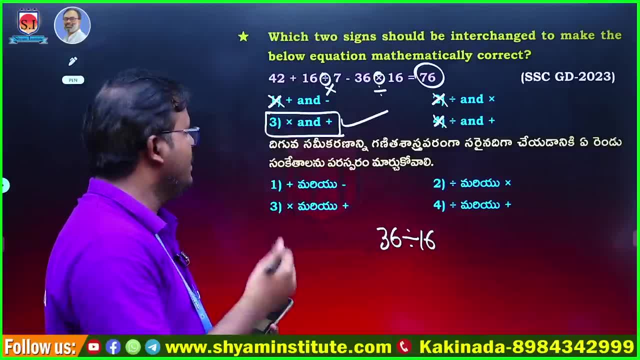 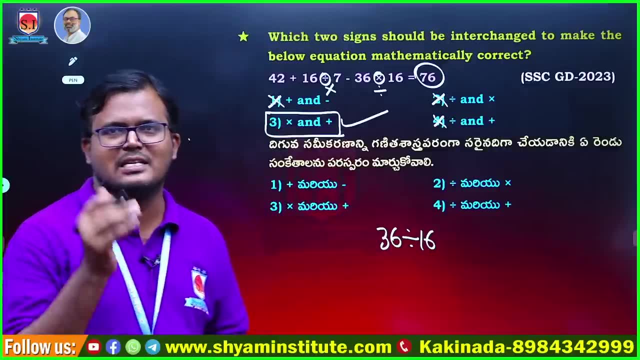 Cancel and answer the remaining one. What is the answer? Third option, As we said, what is the compulsory answer? We can do the calculations easily. We just need to observe the equation. We need to divide it according to the Badma's rule. 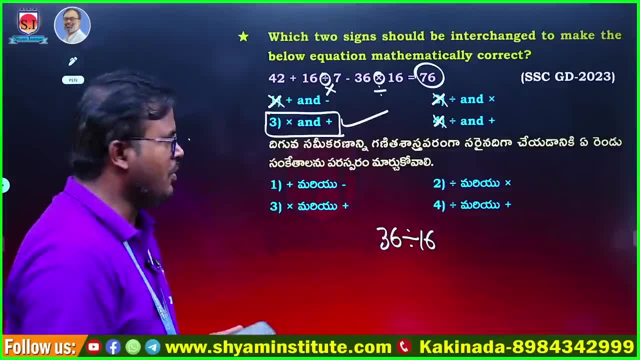 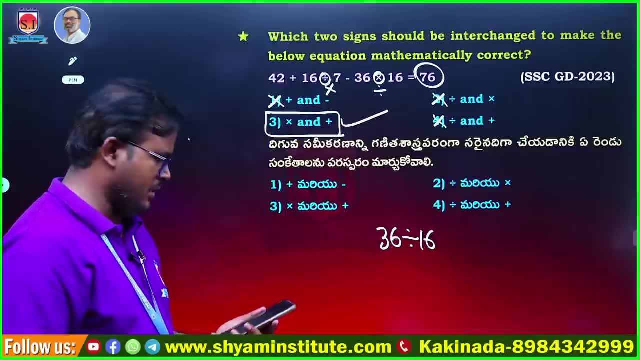 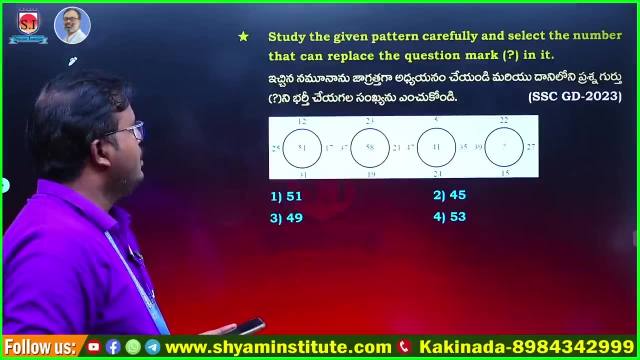 Dividing is not divided by 4.. What is the guarantee that we will get the number 76?? What is the guarantee that we will get the answer? Third option: What is the correct answer When? let us look at this question mark and take a look at it again. 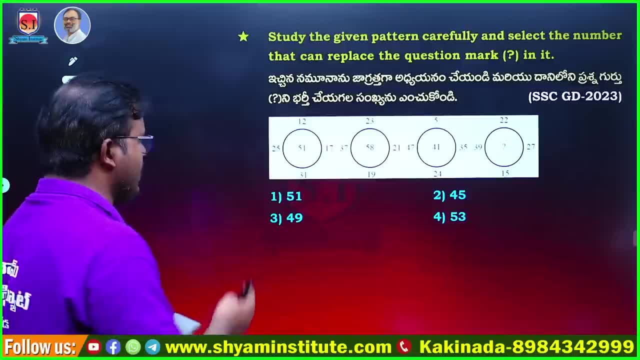 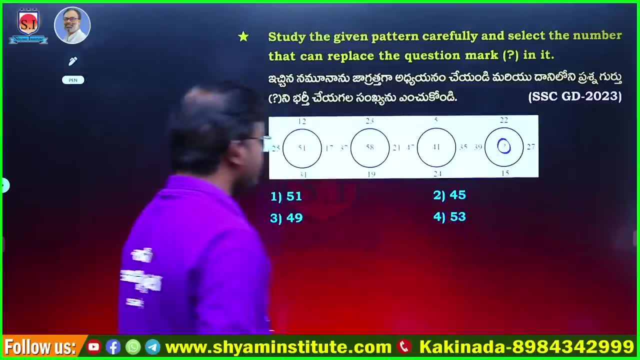 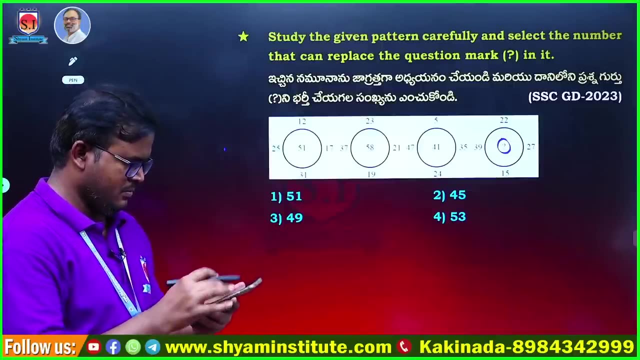 if there is no short form, what number can we get for this question mark? Question mark must be in this fact: Leanckرت. Question mark must be in this fact: Leanckrecht. Question mark must be in this fact: Leanckół. Question mark must be in this fact: Leanckatsu. 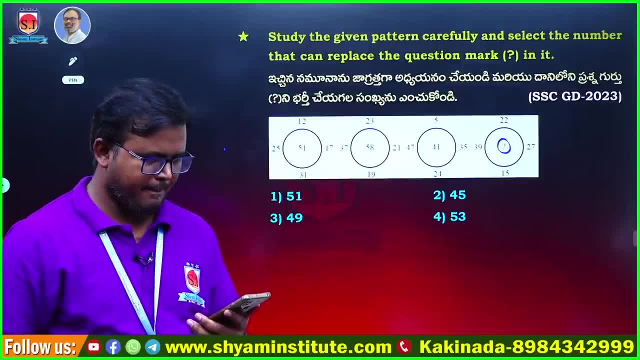 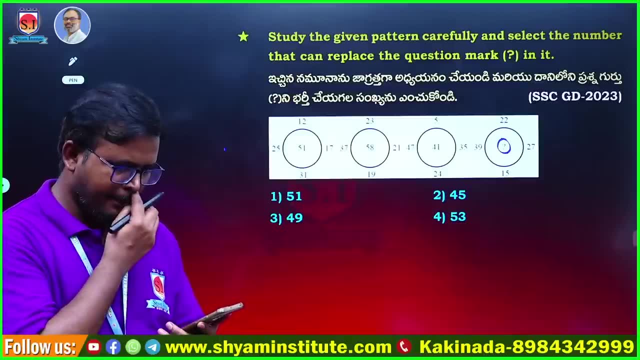 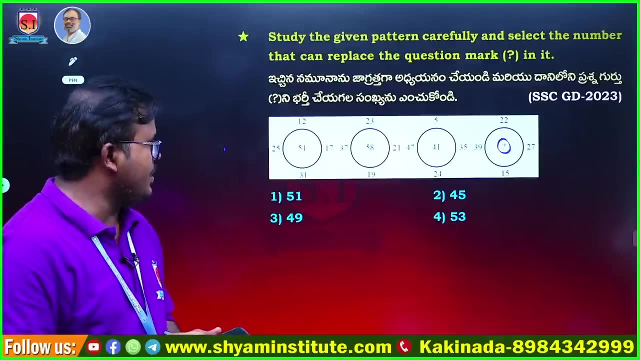 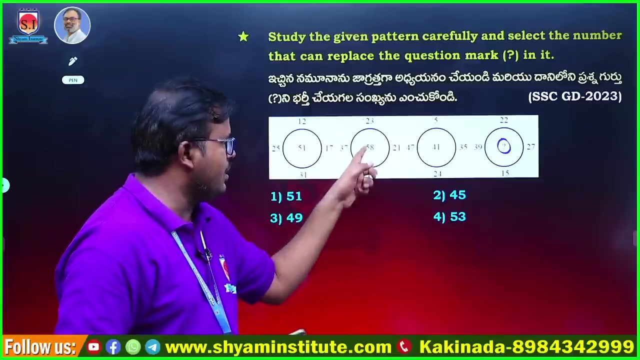 Question mark must be in this fact: Leanck으. Let's see the numbers here: 25,, 17,, 12,, 31 and 51.. Let's see the numbers. How do we get 51 from the numbers around us? How do we get 58 from the 4 numbers around us? 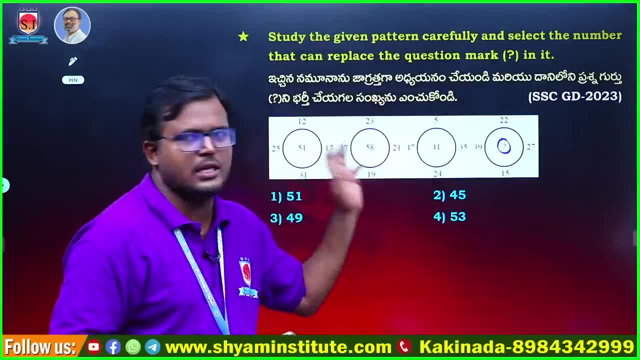 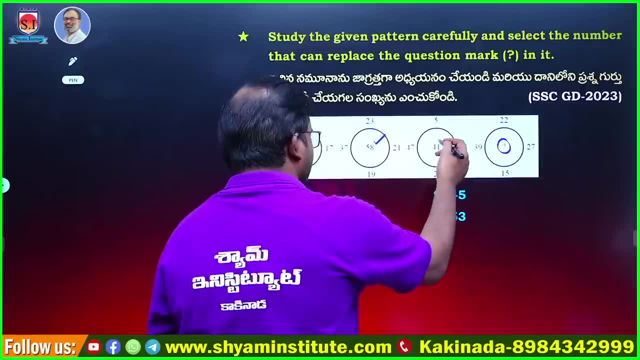 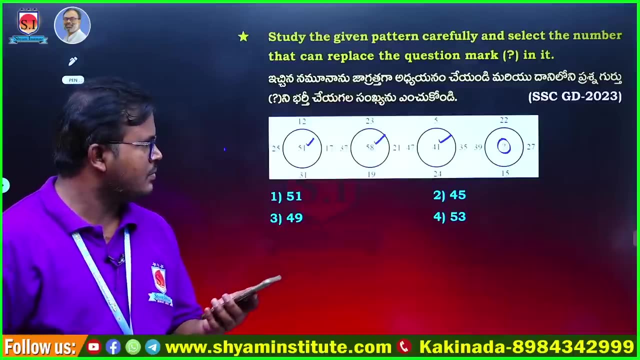 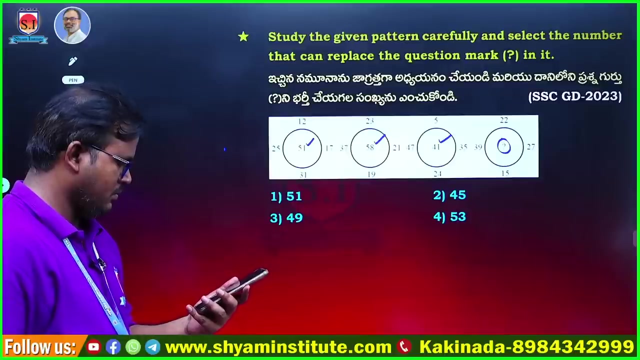 How do we get 41 from the numbers next to us? We can easily answer these questions. First, let's see how do we get 51,, 58 and 41.. Let's do it fast. Let's see how to get 51 from the numbers around us. 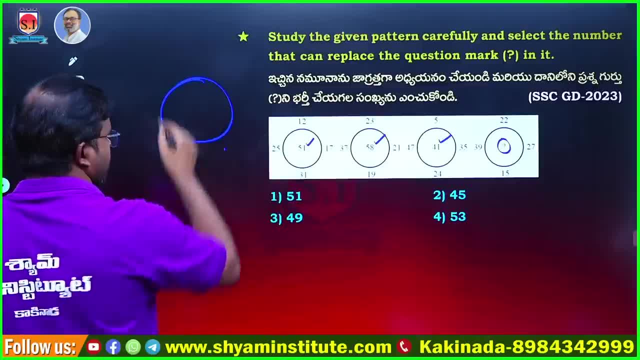 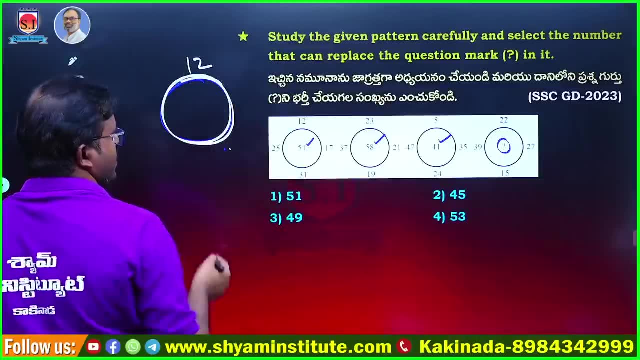 Here, when we get 51, we get a circle like this: If we take the numbers around this circle, we will get a circle around this circle and the number around the circle will be 12.. What will we get from here? 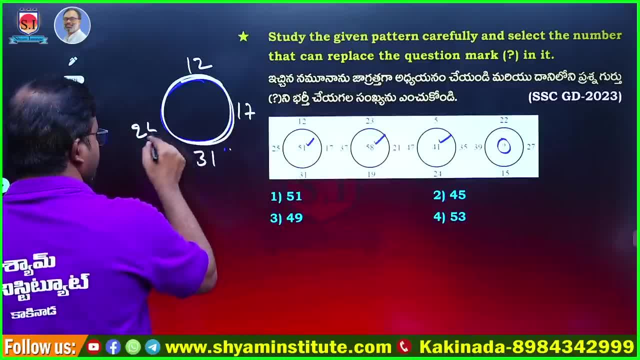 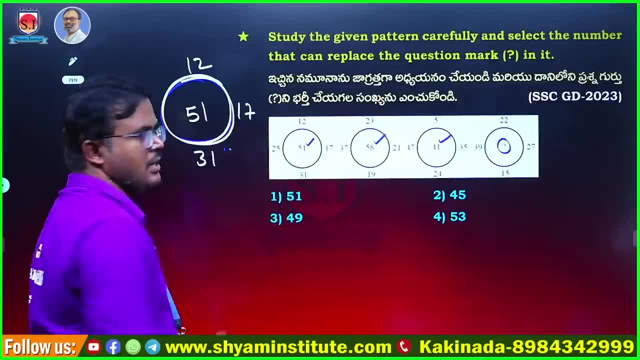 17,, next is 31,, next is 25.. In the middle they gave us 51 number. From these numbers we have to check how 51 number comes. Next one, as you can see how many numbers does it give us. 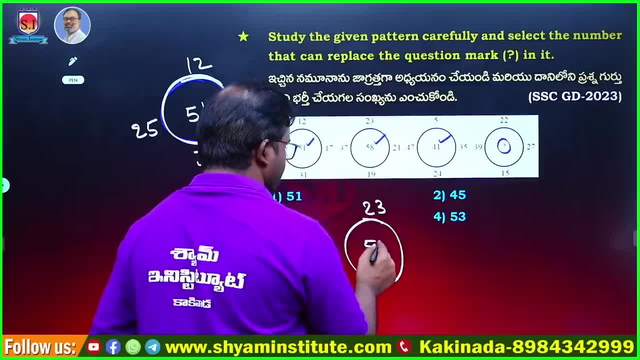 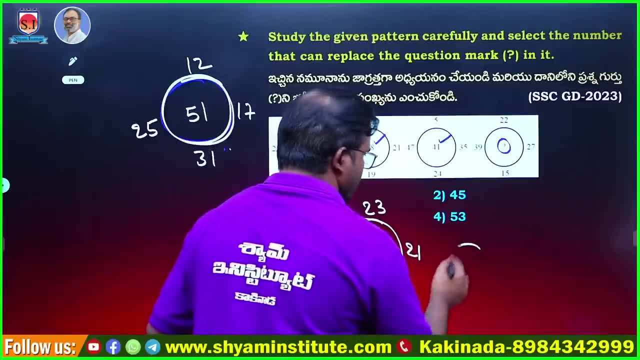 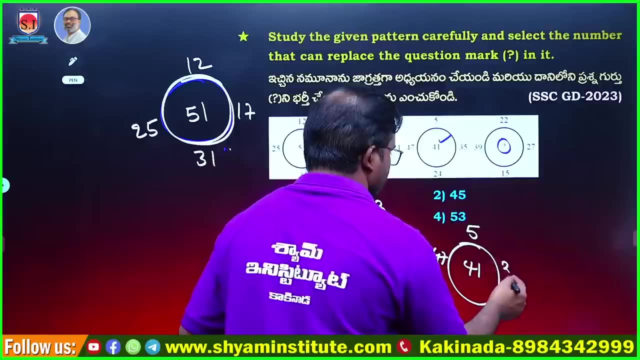 If you see the numbers: this is 23,, this is 58,, next one is 37,, next is 21,. this is 19.. Next see the numbers here. Here number 5 comes. this is 47,, next is 41,, next is 35,, this is 24.. 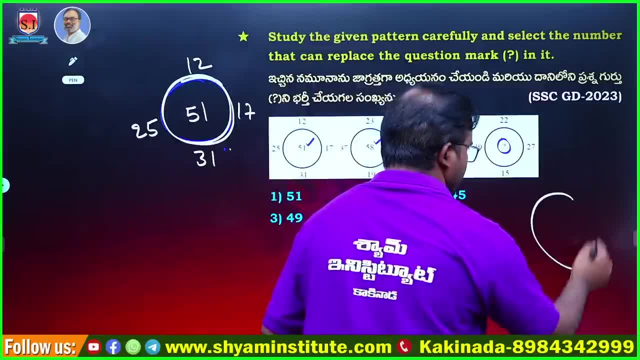 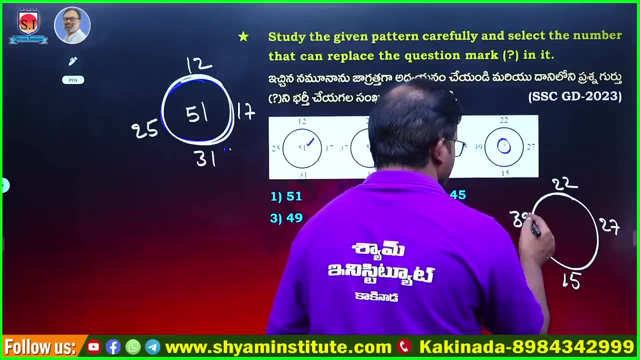 Last one. see the numbers here Here. how many circles does it give? This is 22,, this is 15,. next is 27,, this is 39.. Here it gives question mark. In this question mark place it is asking you to type the number. 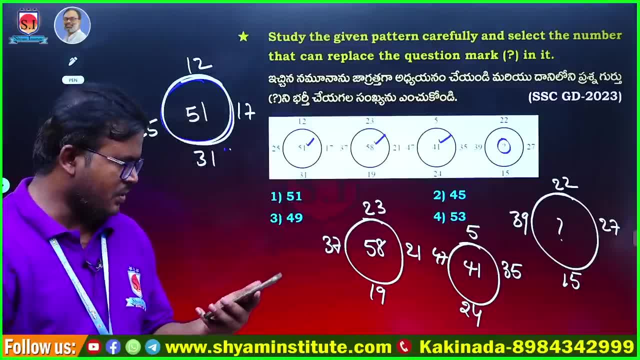 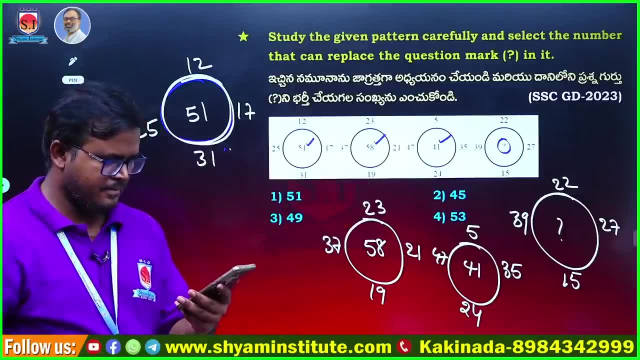 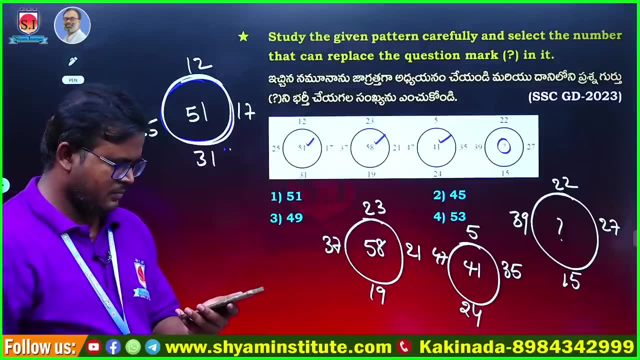 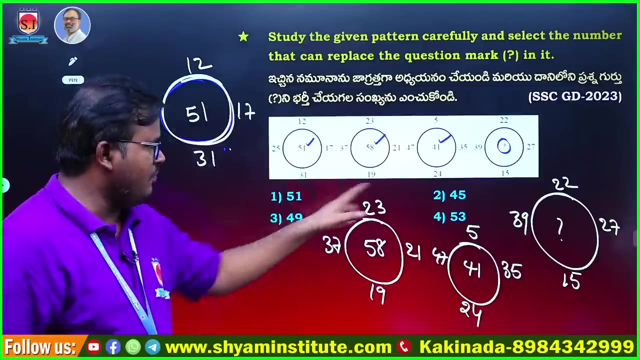 It is asking you to type the number: See, see, see, see. Here it is asking you to type the number. Here it is asking you to type the number 51,, 45,, 49,, 53.. 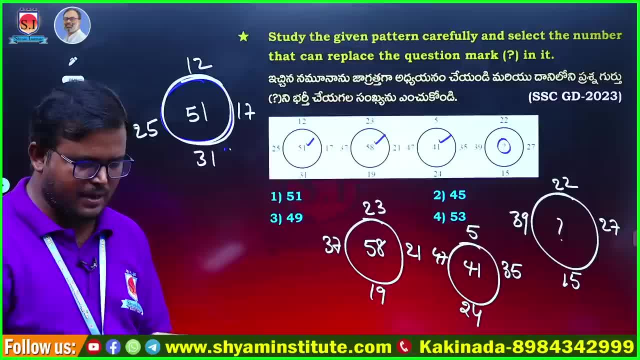 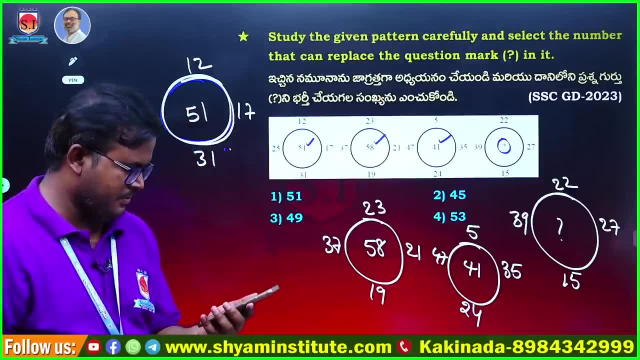 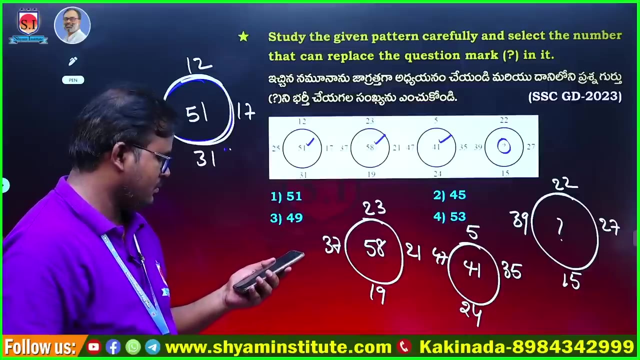 Which one is the correct answer in this question mark place. So let us know. in the comment box, Ramana sir has given the third option. So first let us see how 51 comes in front. So first let us see how 51 comes in front. 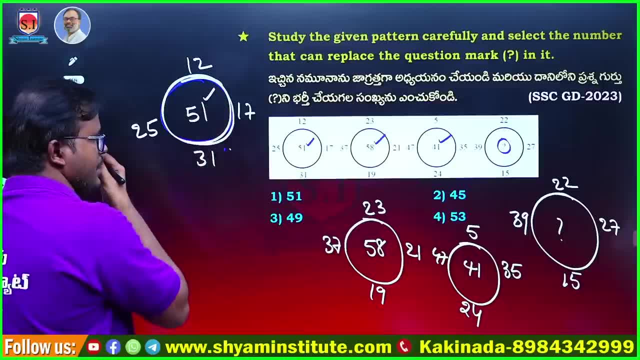 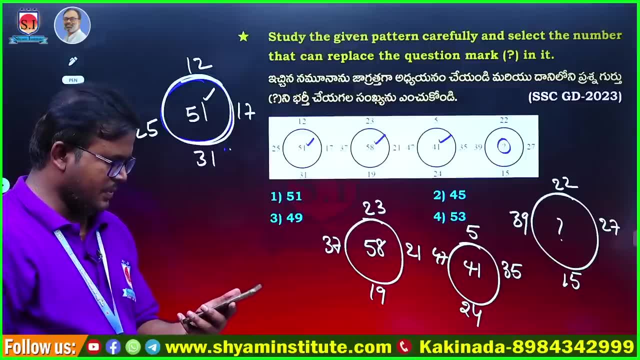 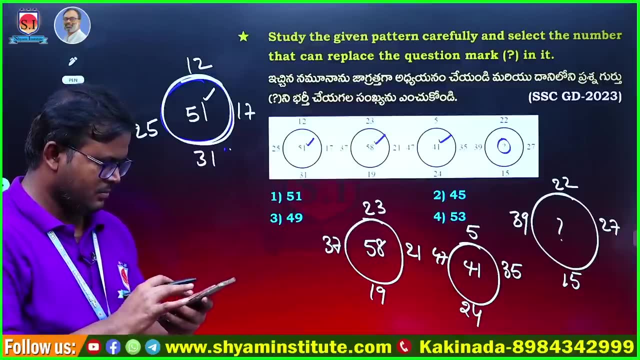 So first let us see how 51 comes in front. If we know how to get 51, we can answer it accordingly. We have to tell the answer. 45 is the second option. What else? What is the reason for this? 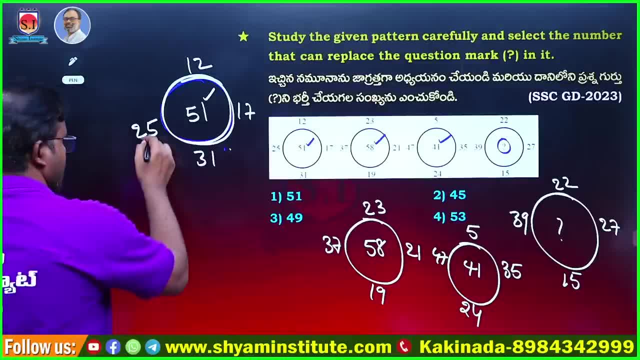 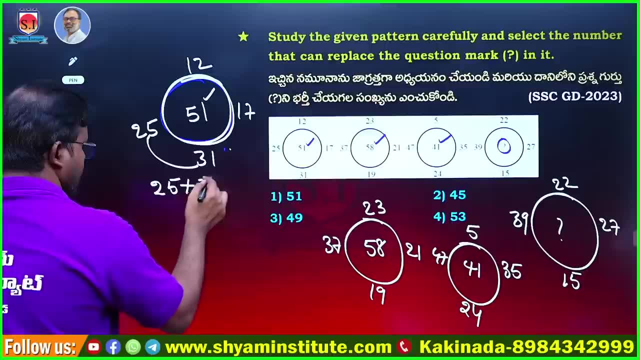 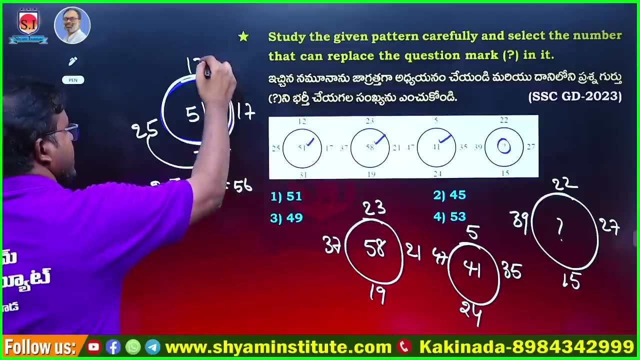 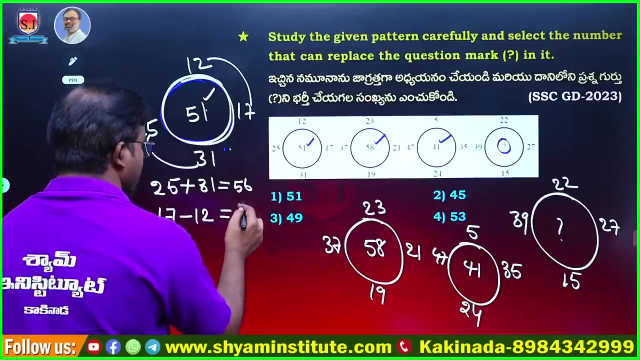 First, add these two numbers here: 25 plus 31. If we add these two, we get 56.. Since 51 is here, subtract these two numbers, 17 minus 12. Subtract What is this? We get 51.. 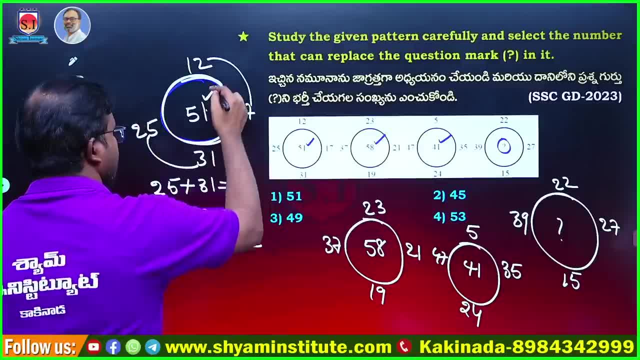 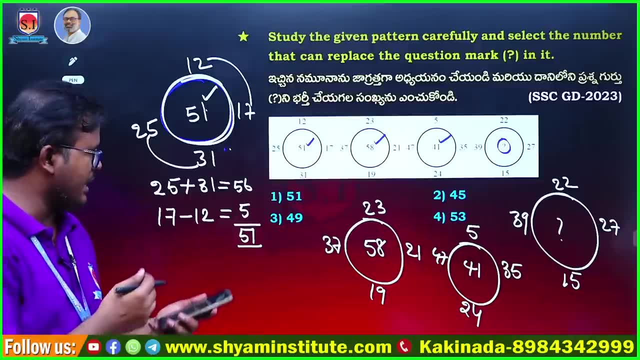 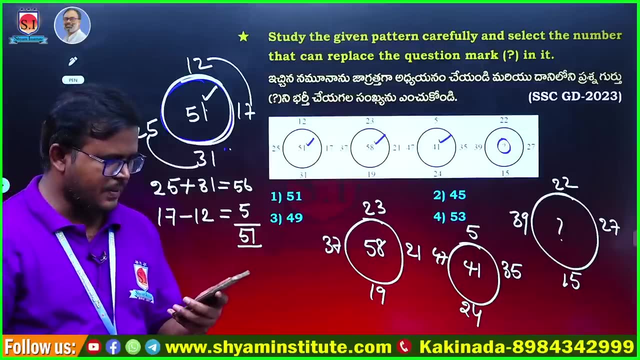 What is the difference? We get 51.. What is the reason for this? We get 51.. Now tell us the answer. according to this, I have already told you the clue, So apply it once. Mr Durga Prasad, you gave the third option here. 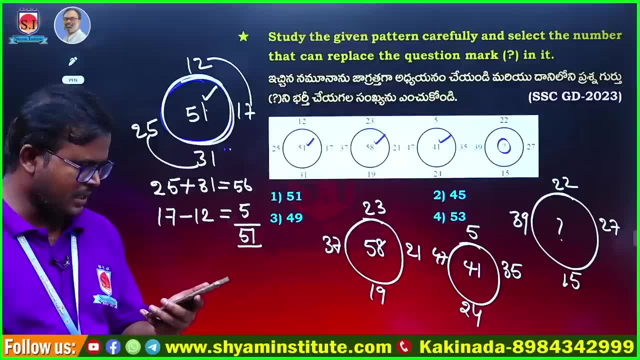 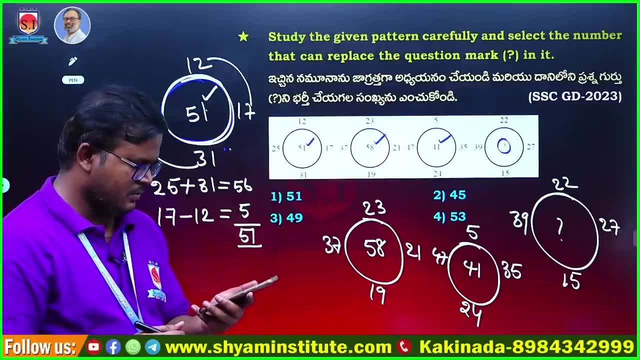 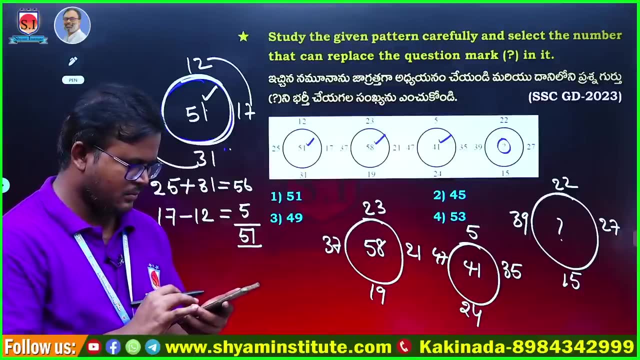 Mr Bharati is 49.. Mr Kusumant is 49.. Third option: Third option: Fourth option. Fourth option. Fourth option: Third option: Fourth option: Alright, Okay, who knows which is right? My answer seems partially correct. 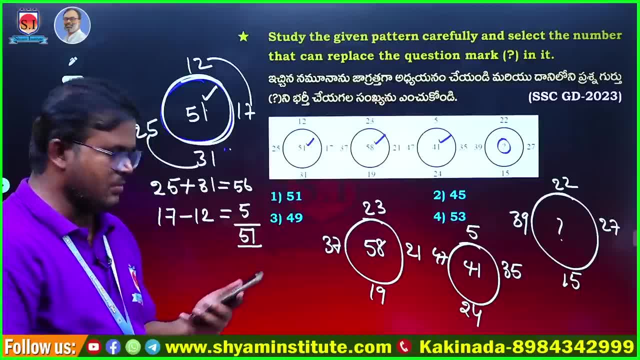 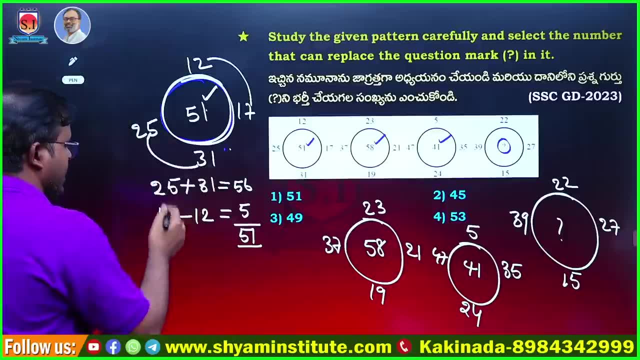 Good, Many of you are saying that not. my answer seems right. All the three are now correct. You are the Double Piece. Yes, In this slip that new Gift. I am forgetting about a simple fraction right now. Yes, You are right. 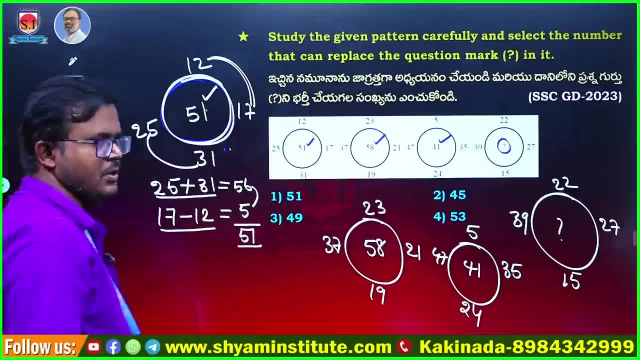 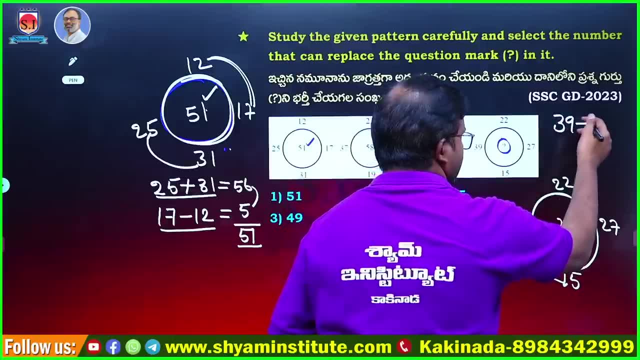 So keep taking. So how much will we get? We will get 51.. Now let's come directly here. First add these two numbers, That is, add 39 plus 15.. Add these two numbers. So how much will we get as we add these two? 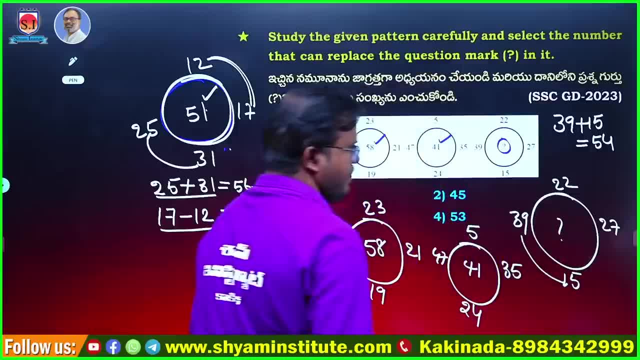 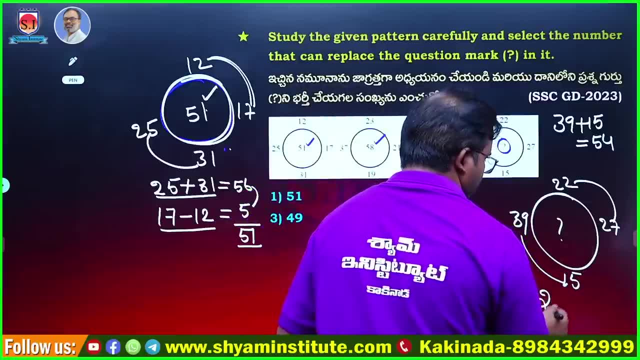 We will get 54. So we got 54.. Next we need to make a difference between these two. So make 27 minus 22. So we will get a number called 5.. Here it is 54 and here it is 5.. 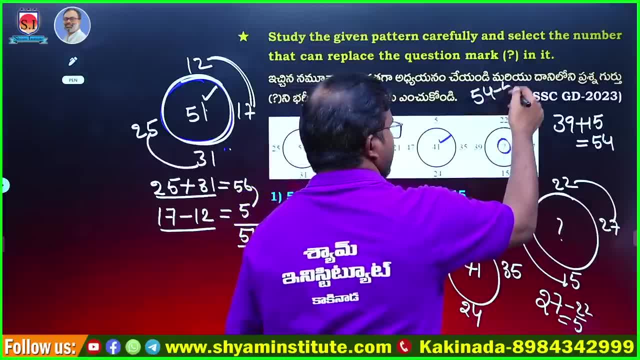 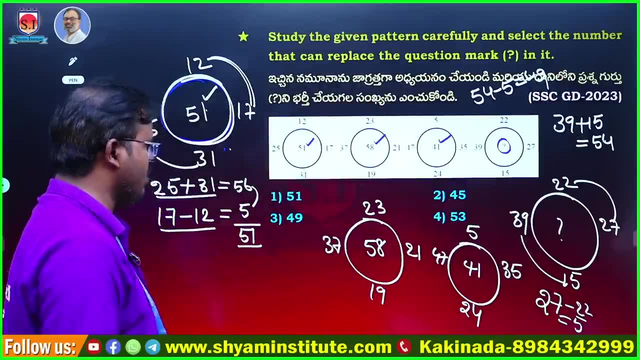 So the answer we will get is 54 minus 5.. How much will we get? 49.. Now, what is 49?? We need to check the option given to us. Where is it? It is in the third option. 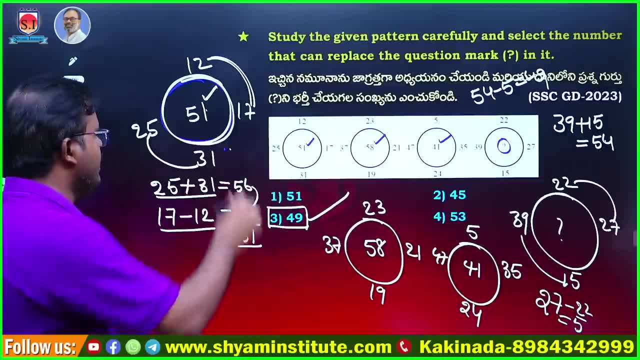 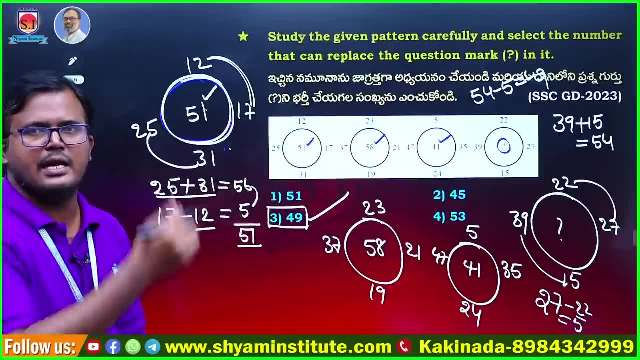 So the third option is the correct answer. If you observe the first diagram correctly, we will have the same pattern in the second and third. Now what will we do? directly, We will go to the last diagram For the third diagram. 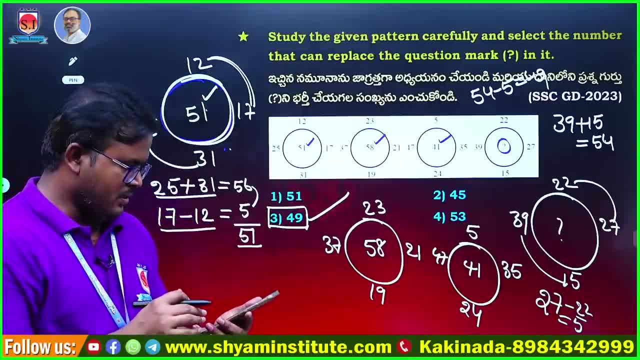 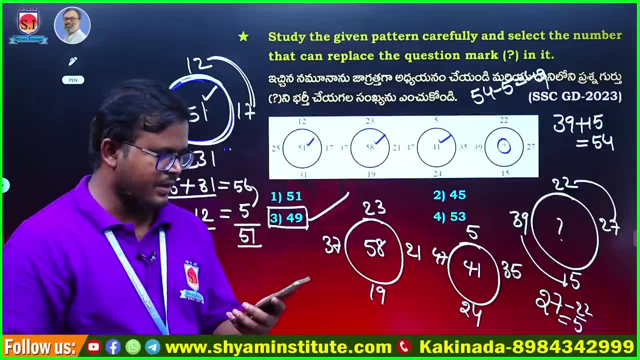 what will be the answer here? We will get 49 here, So very good. So you are doing very well. Some of you have typed here without any reason, So very good. What I am telling is, if the practice is not correct, 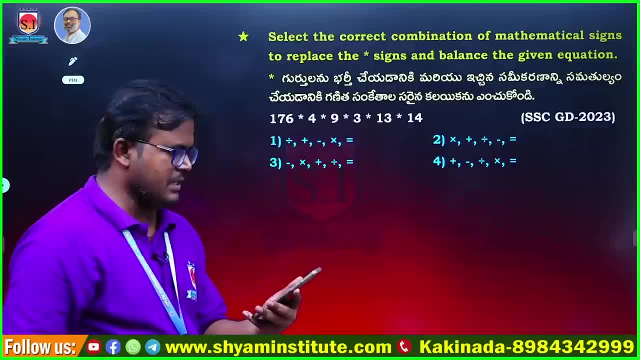 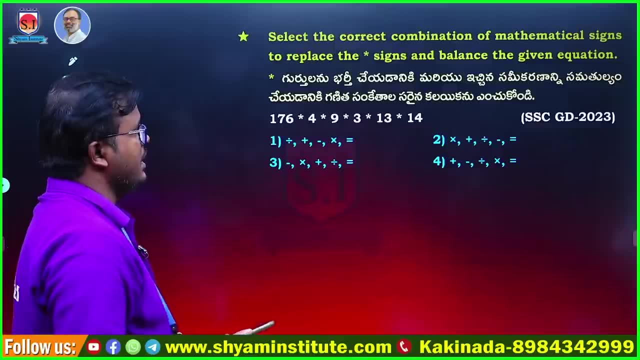 it is not that difficult to get a job in SSCGD. Now look at this problem. Select the correct combination of mathematical signs to replace the star sign and balance the given equation, The formula given forν, to get the star symbol as the right combination. 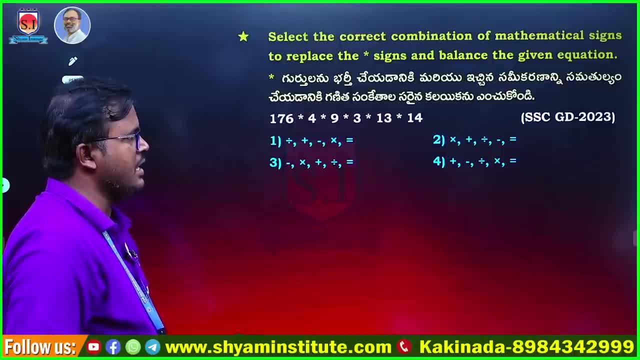 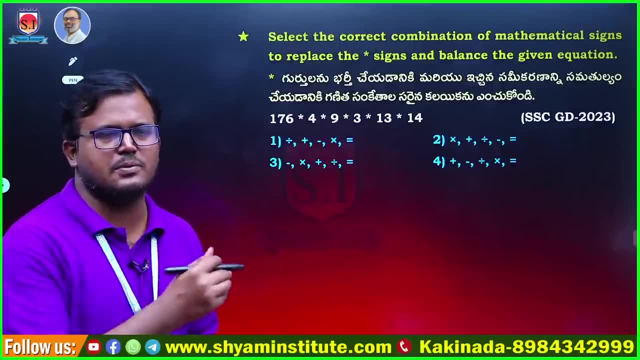 and for the mechanism to get the right combination is given according to the mathematical signs. And here, in case you get the right combination, what we have given here is that in the options given to us, which is a set of symbols, they will get set correctly to us. 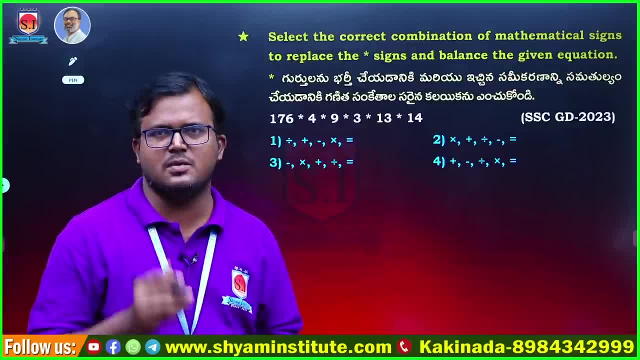 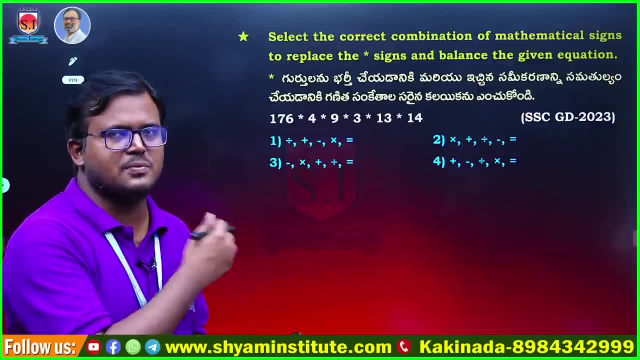 What do we need to check about that? Whatever we have said so far In the concept of mathematical operation, we have given the problem on the interchanging model. What is this? This is a substitutional model. If we substitute an option, the answer will be correct. 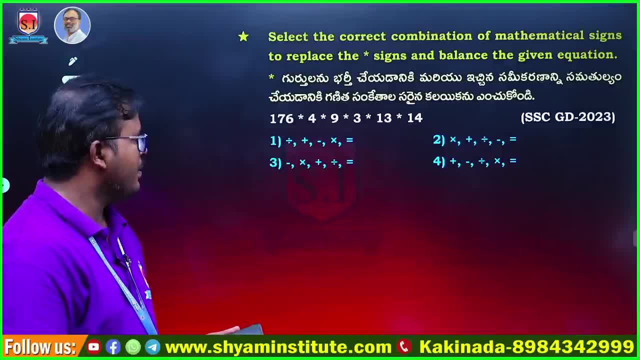 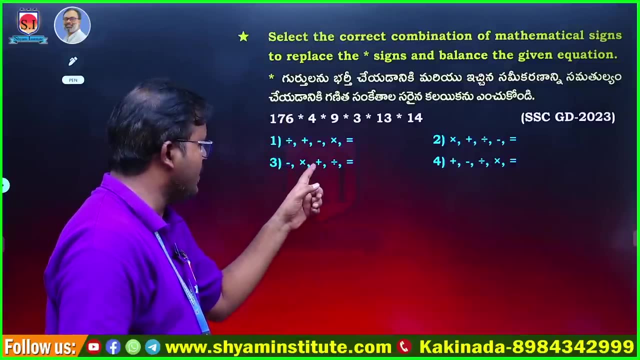 What is that option? Tell me the answer. The first option is divided by plus or minus, or into is equal to. The second option is into plus or divided by minus or is equal to. The third option is minus or into plus or divided by is equal to. 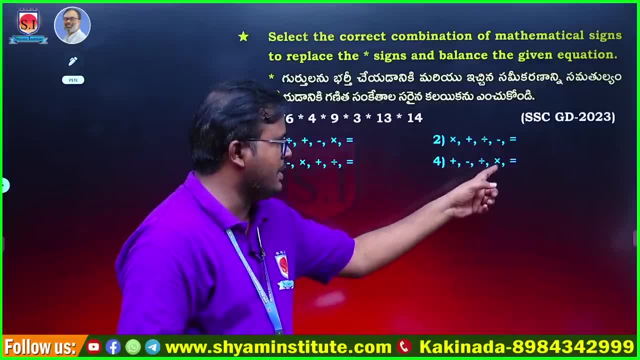 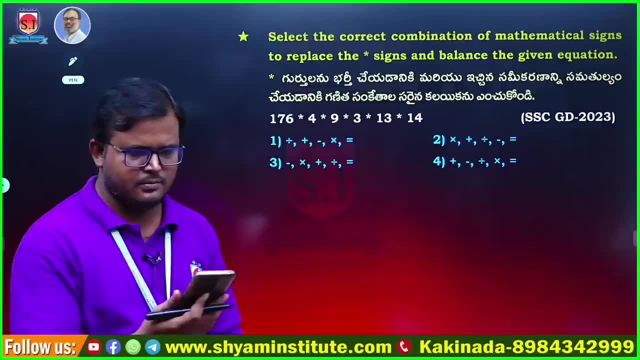 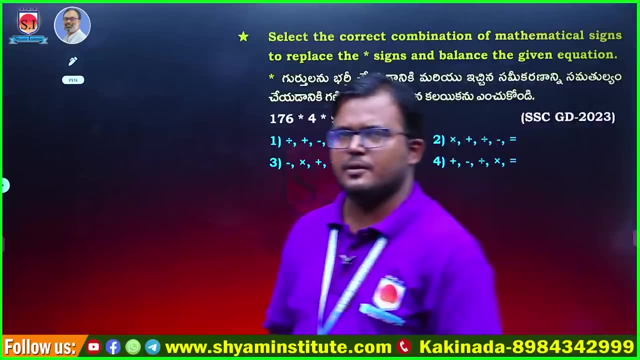 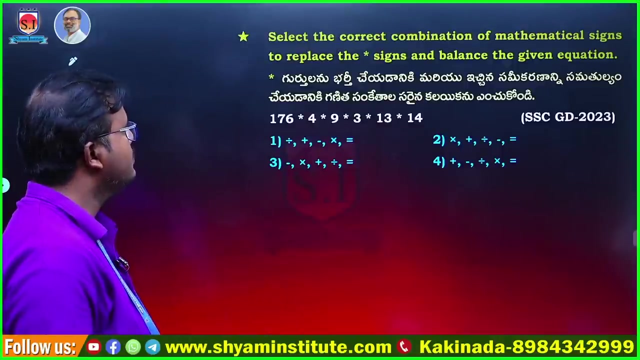 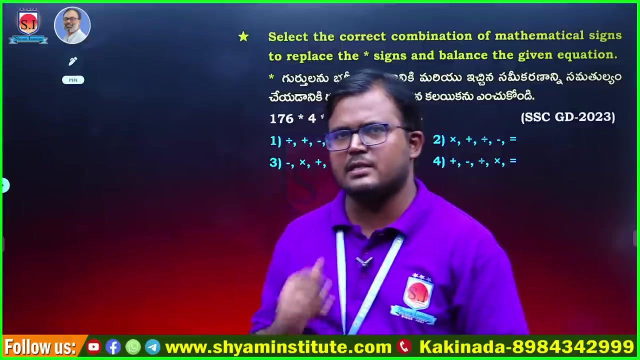 The last option is plus or minus or divided by into is equal to. Which option will give the answer? Write in the comment box. Tell me the answer in the comment box. The answer is correct. The correct combination of mathematical science. The correct combination of mathematical science. 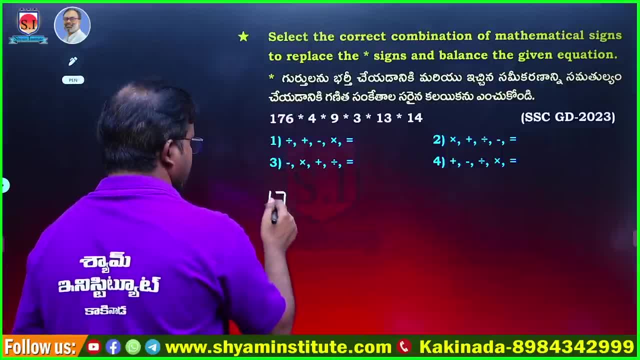 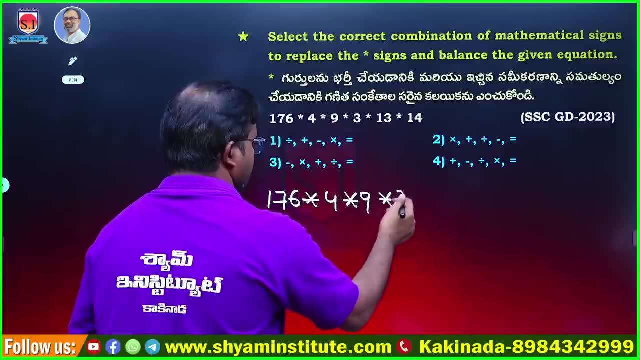 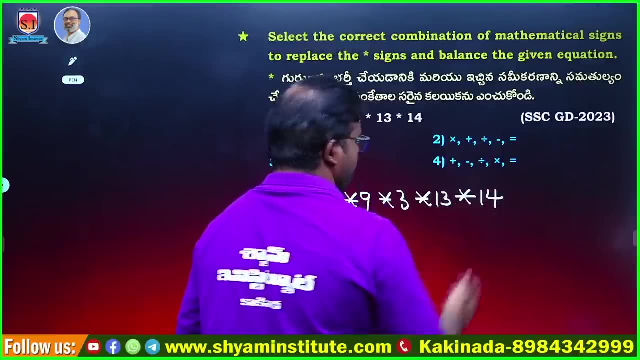 The first one is 176.. Then the star symbol is 4.. Again, the star number is 9.. Again, the star number is 3.. Again, the star number is 13.. The last one is 14.. What is the equation? 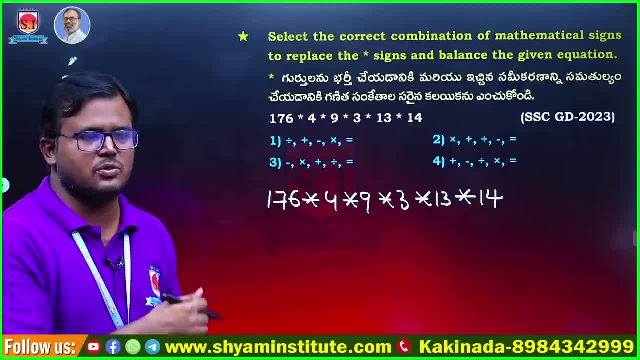 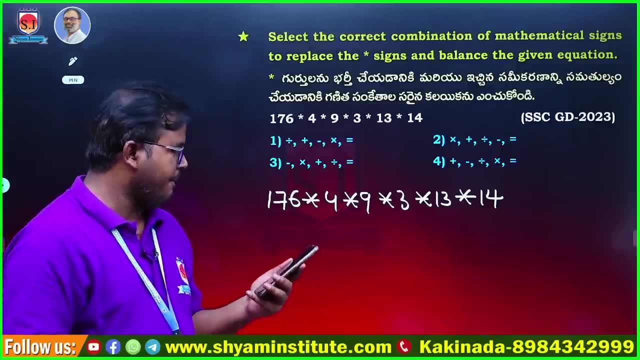 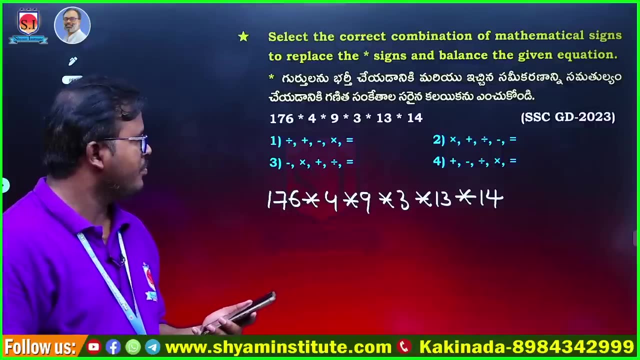 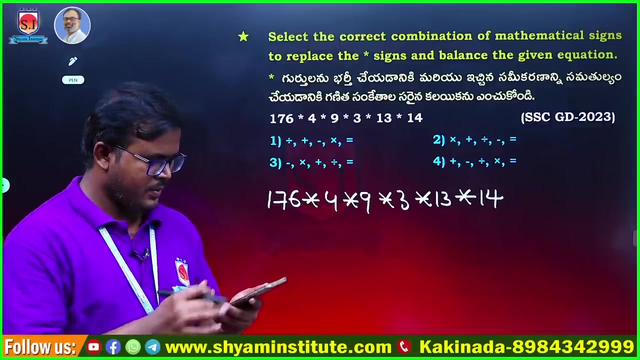 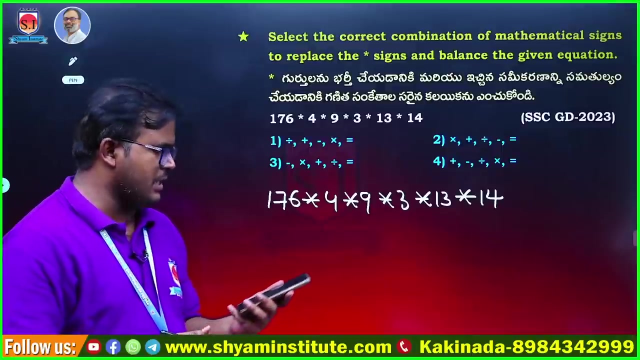 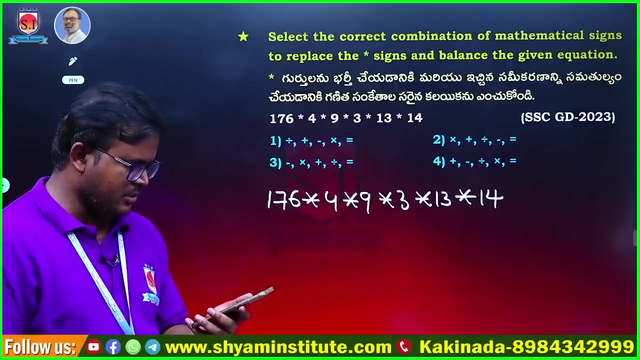 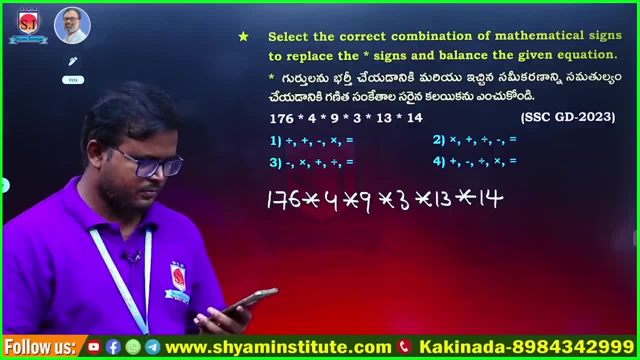 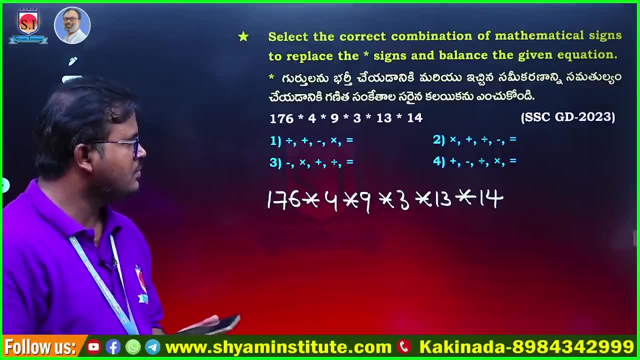 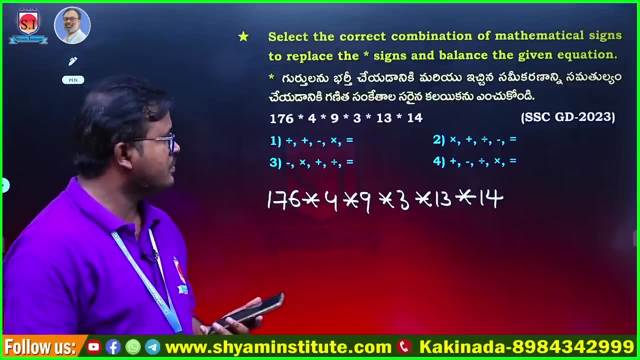 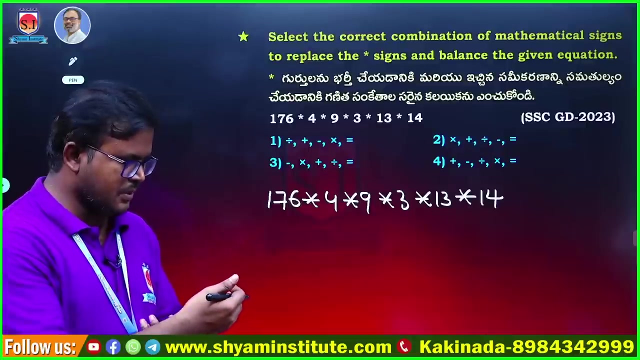 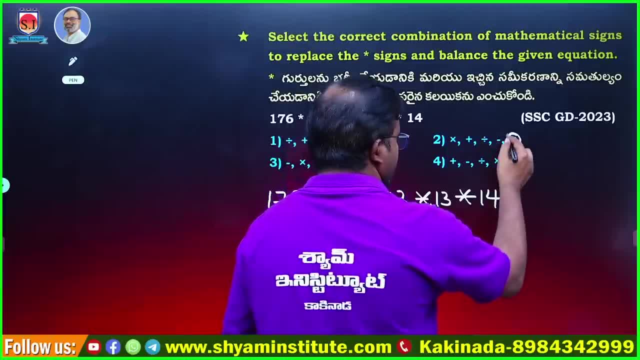 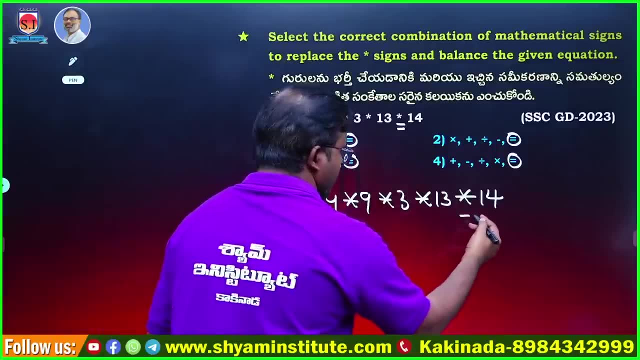 In the last, there is a symbol called Easy Equal. What you have to do is You have to notice the symbol Easy Equal. Let us see what is coming here. Easy Equal should be 14.. To get the number Easy Equal 14,: 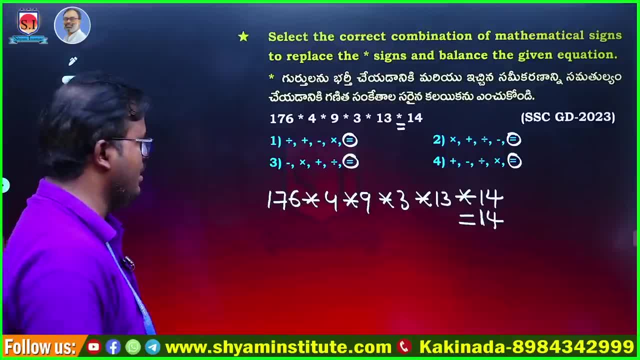 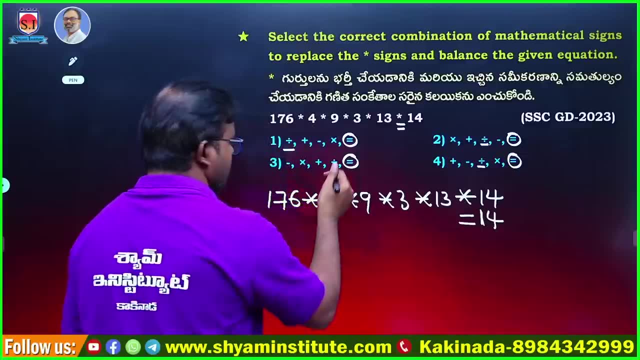 You have to go to the symbol Divided By. The symbol Divided By is here. What is happening here is: it is in the third position. What is happening here is: it is in the fourth position. What is the fourth position? 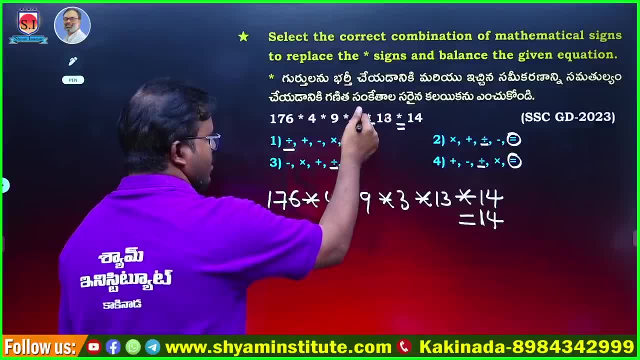 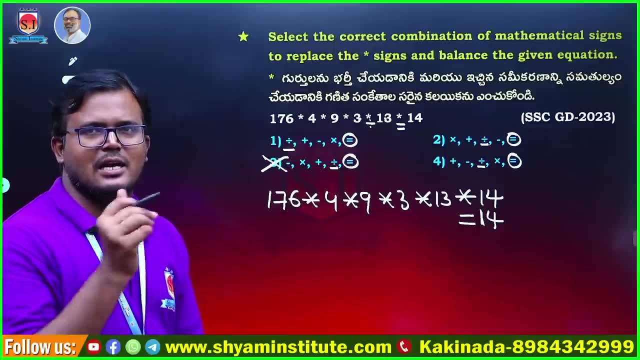 If you take Divided By here, 3 divided by 13 means The number 3 here is going to be 13.. For that, this is not the answer. Don't remember the first. What we have to do first is: 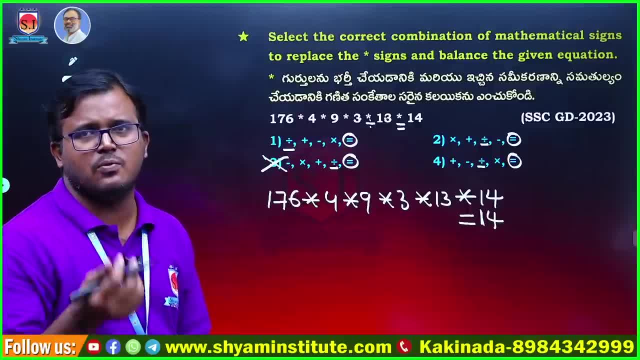 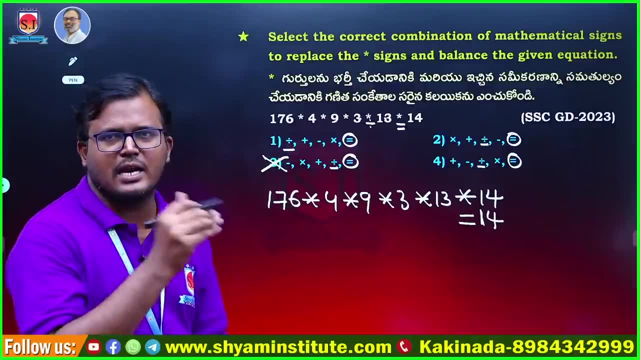 Option Verification. If you are given the first option, we will do it immediately. If you are in the fourth option, what is the situation? We have to check that too. What we have to do is We have to do an observation like this: 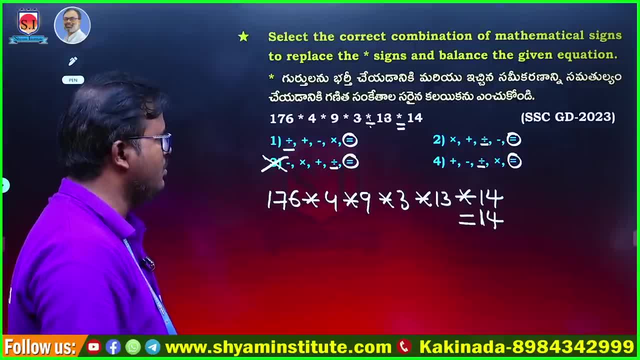 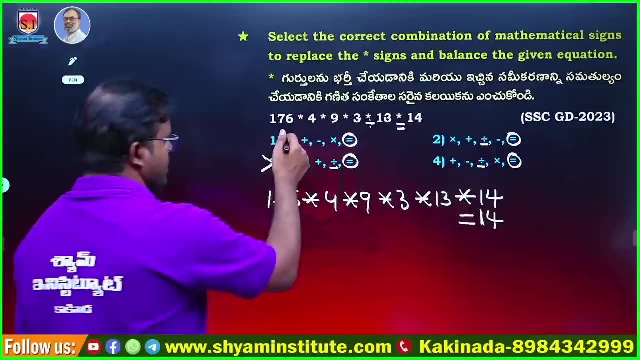 So we know where to stop the problem. What is happening here is: The third option is not the answer. What will they do next If we see the symbol Divided By here? What is happening here? We are in the first position. 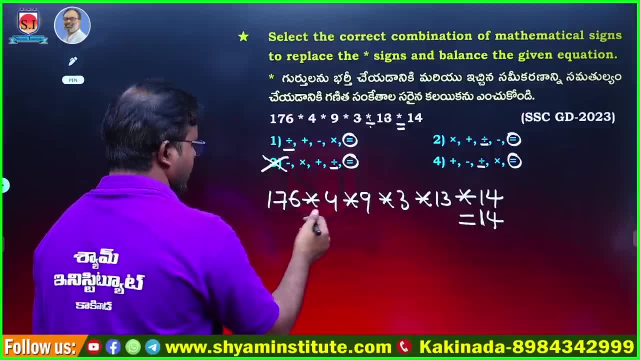 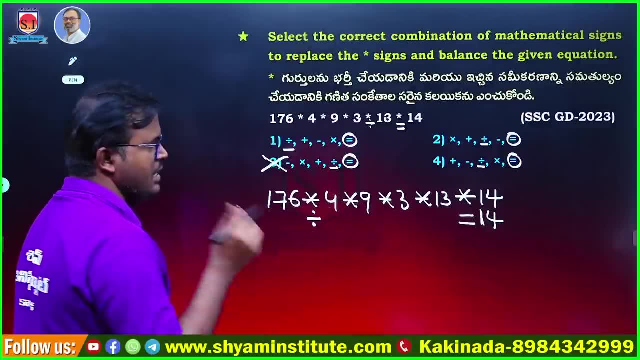 What is happening here is: The third position is here. So what is happening here? Let us take Divided By here. If we take Divided By here, 170, 670 number, What will we do If we do Divided By 4,? 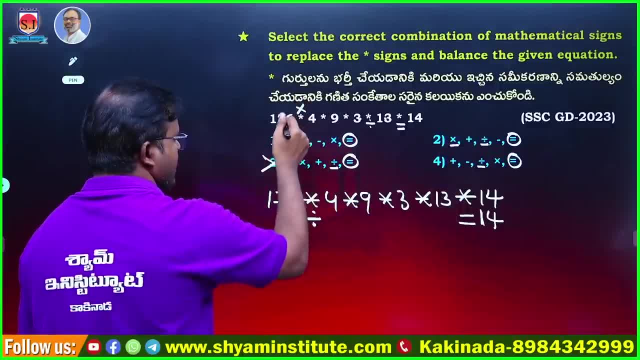 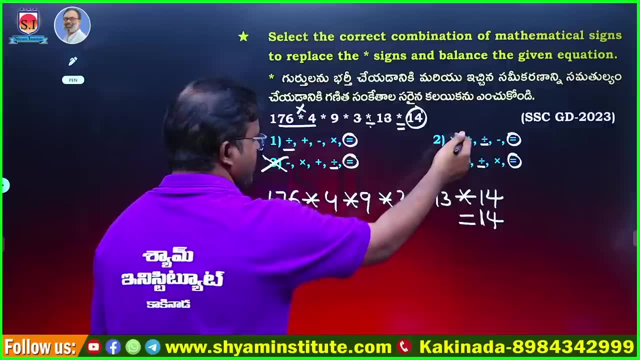 The fourth option will be cancelled. I think we should see the other twist here. See, here there is a symbol Intu, But the answer should be 14.. So there is no such thing as a divided by. This is not the answer. 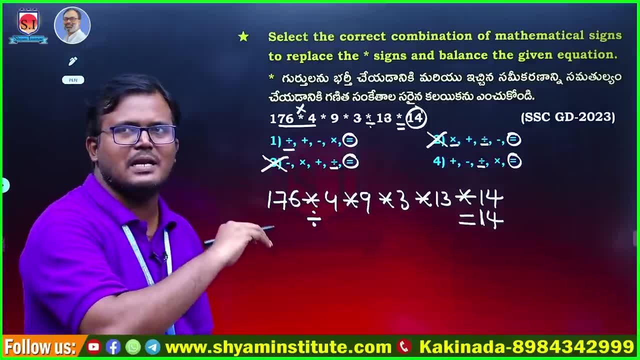 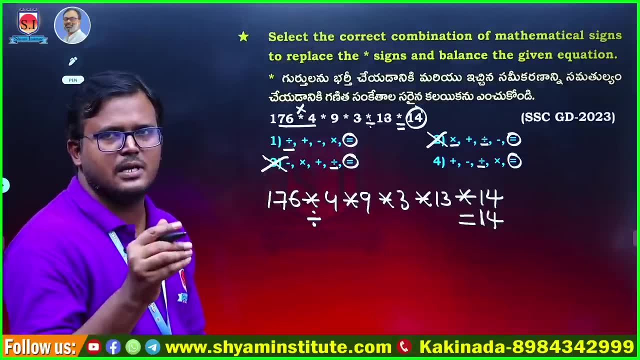 If you take the symbol into as a guarantee, you will get an idea that if you multiply, the value will increase. But that is not the answer. What are the options here? 1st option or 4th option? If the answer is 1st option, it is the same. 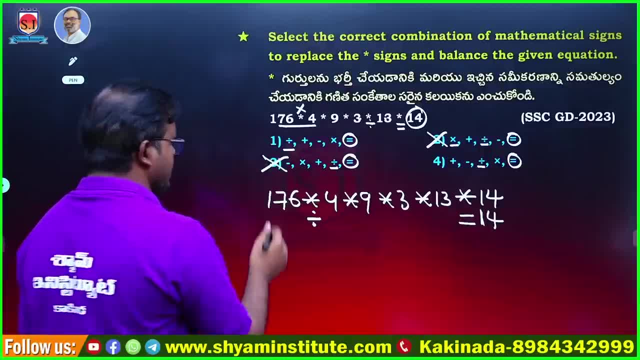 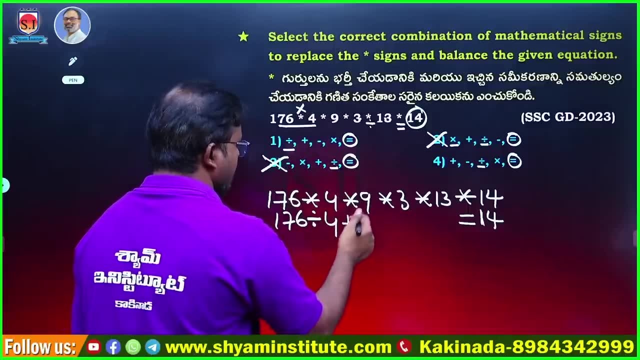 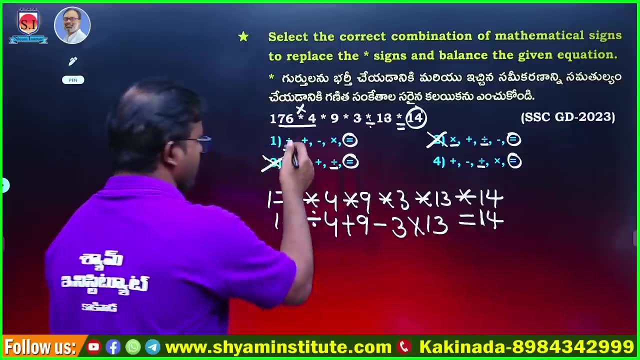 If it is not, it is 4th option. So go to the first option. 176 divided by 4.. Then what symbol is there? Plus, Then there is 9.. Then there is minus, Then there is 3.. Then there is 13.. 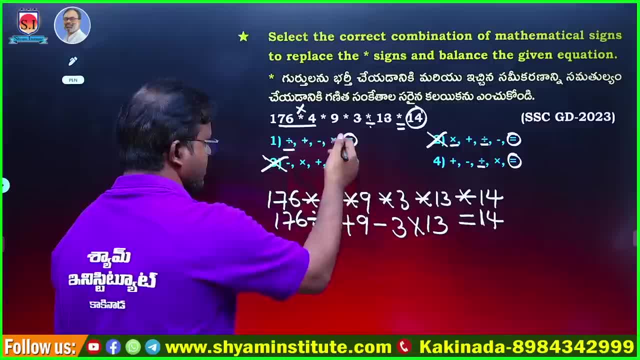 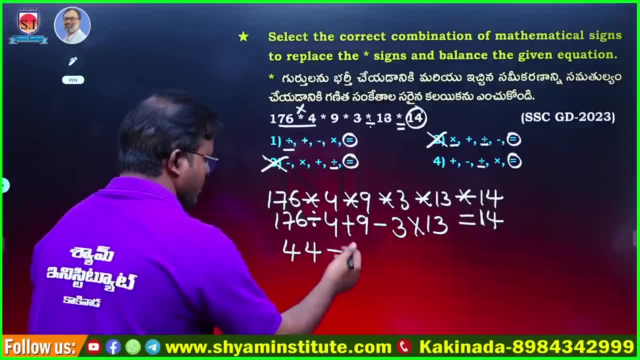 So first is divided by, Then there is plus, Then there is minus, Then there is into. Now, if we cancel with 4, then there is 4, 4s, Then there is 4, 4s. 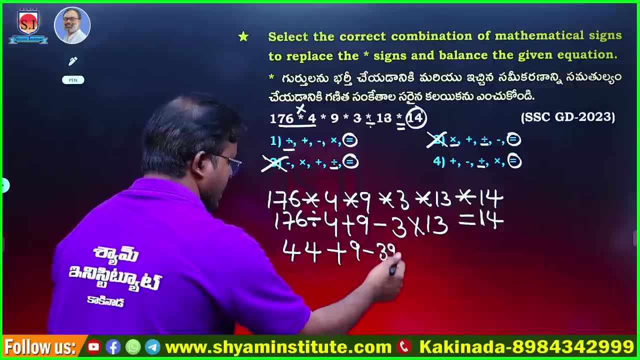 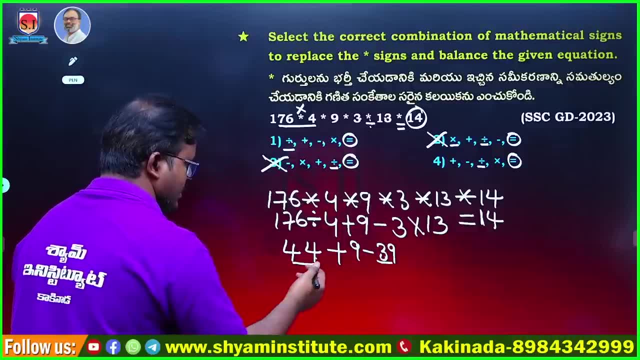 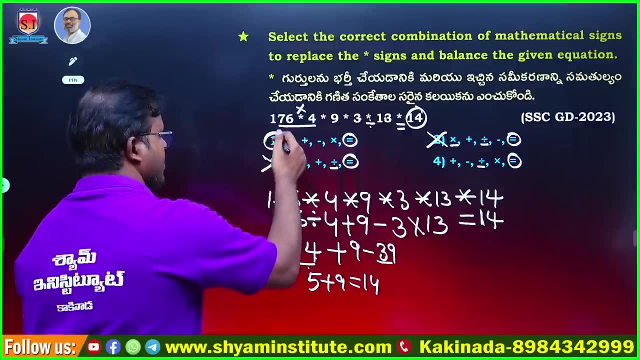 Plus 9, minus 13, into 3. Then there is 39. Then what will you do for these two? Make a difference. If you make a difference for these two, how much will be the answer? So 5 will be the number. 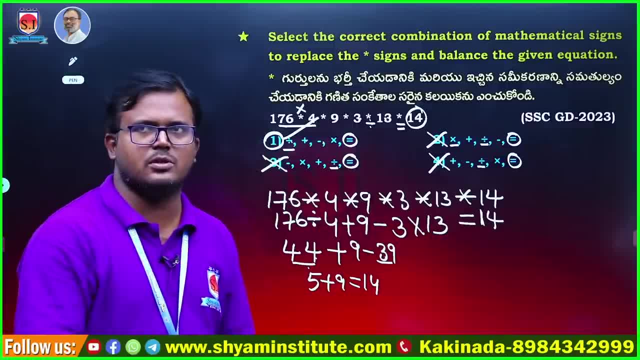 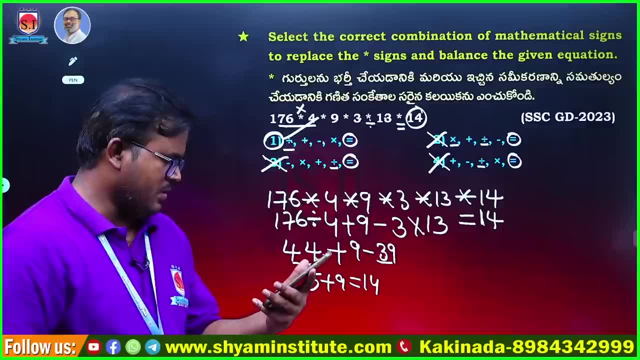 So 5 plus 9 will be 14.. Because option number 1 is correct, option number 4 will be wrong, as a guarantee. So since we got it in the first option, it will end soon. So you are doing very well. 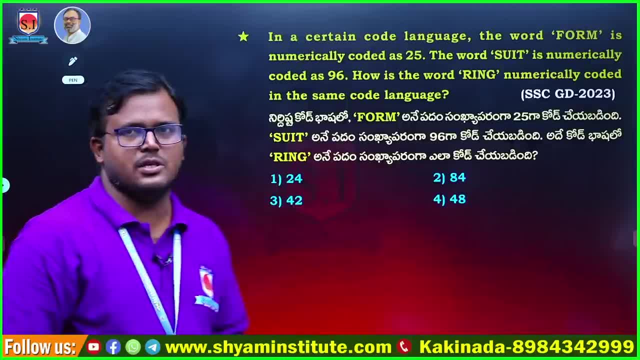 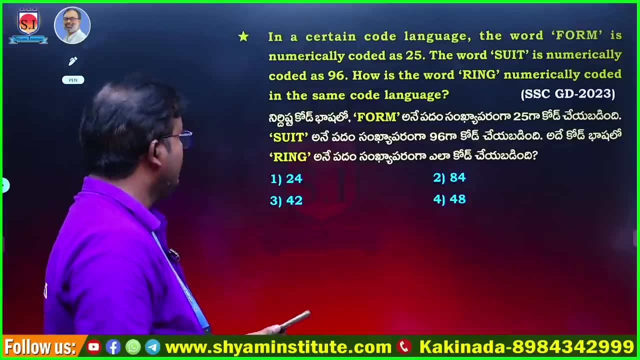 Next problem is about coding and decoding. So what is the answer to this? So quickly tell us in the comment box. See, in a certain code language the word form is numerically coded as 25.. The word suit is numerically coded as 96.. 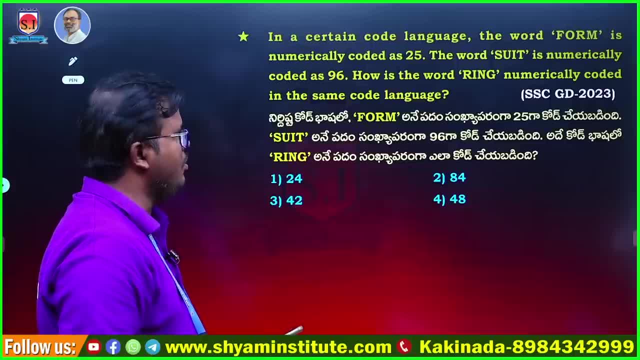 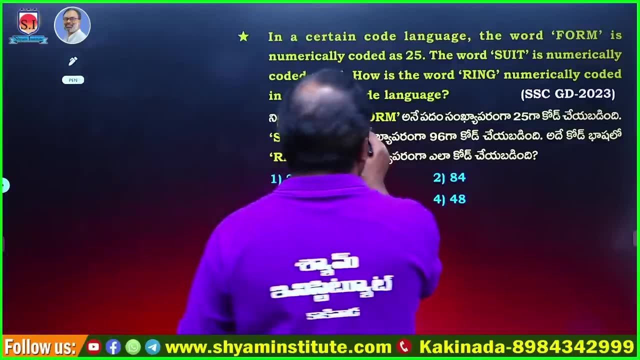 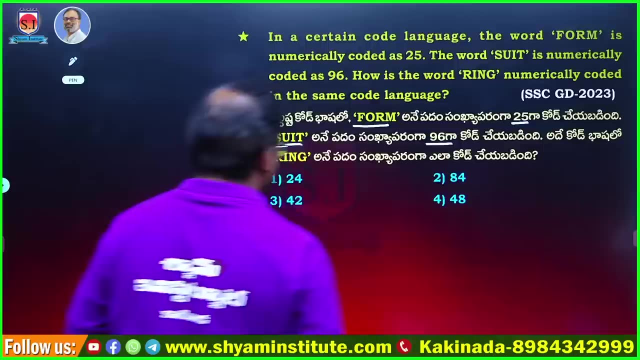 How is the word ring in a numerically coded in the same code language? What we have to notice here is that the word form is numerically coded as 25.. The word suit is numerically coded as 96. So what is the answer to the word ring? 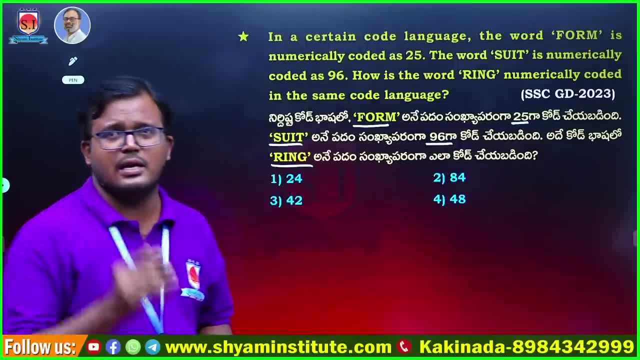 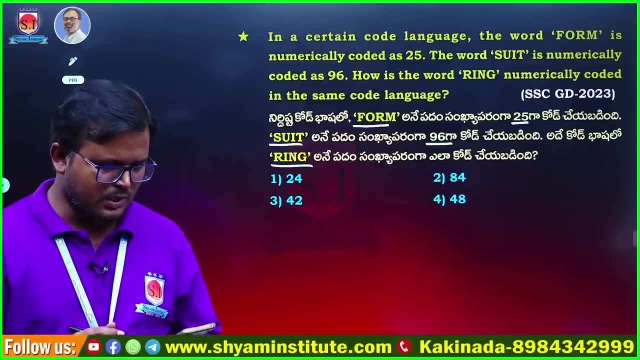 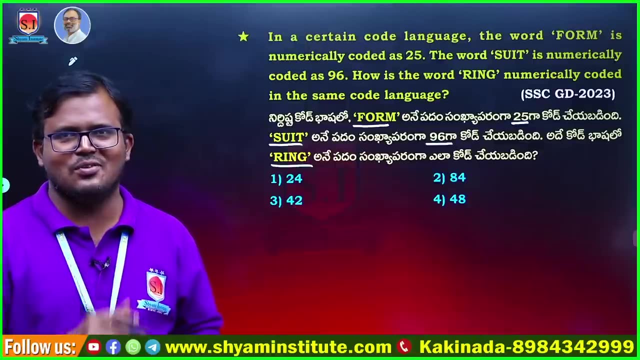 What is the answer to the word ring? What is the answer to the word ring? Tell us what is the answer to the word ring. Tell us in the comment box. Try it out. Try it out with pen and paper. You will find the answer to this. 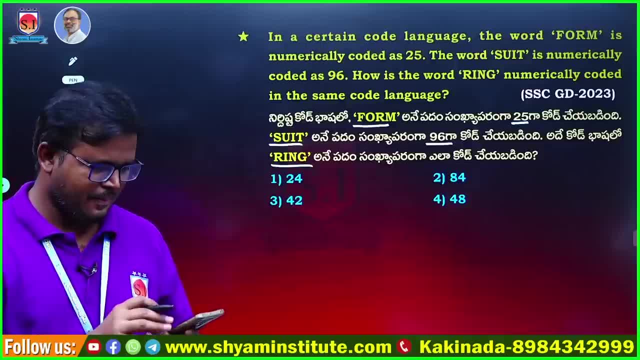 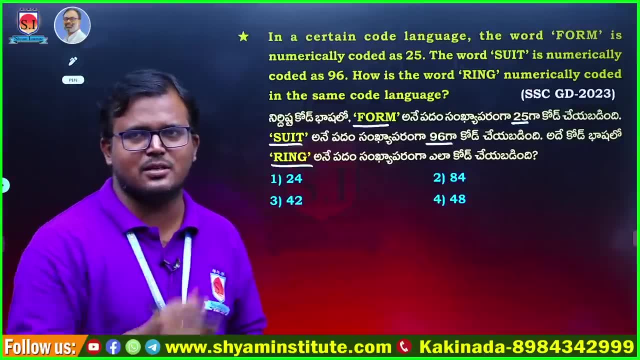 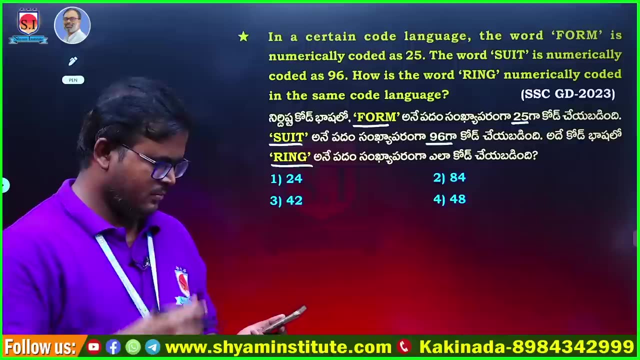 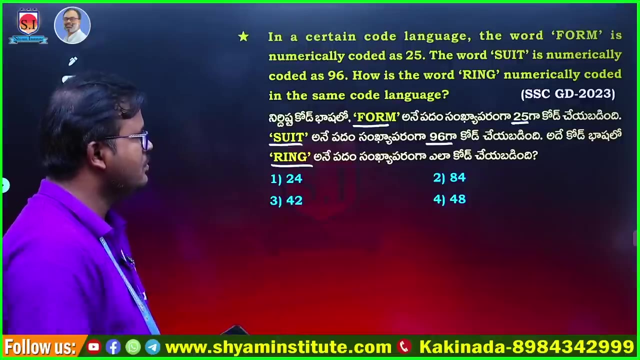 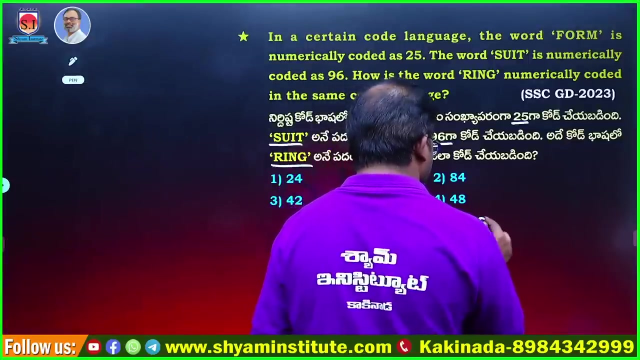 Live in the comment box. Try this out. Coding and decoding. We said that the letter is two numbers. You should know the numbers With the numbers. check what you did First. what is the spelling given to us? F-O-R-M. 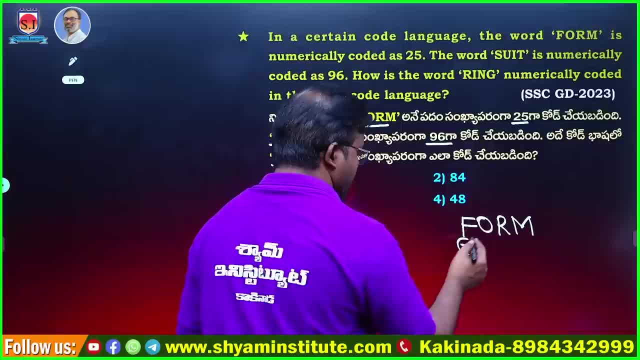 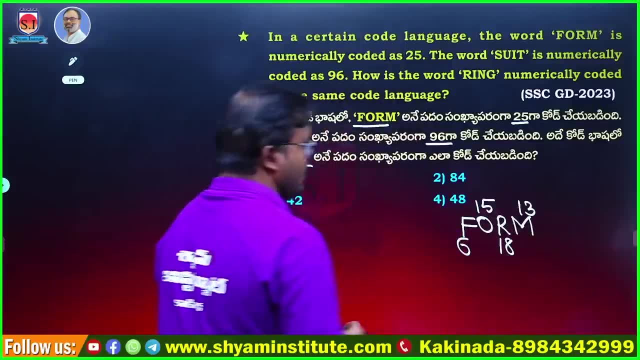 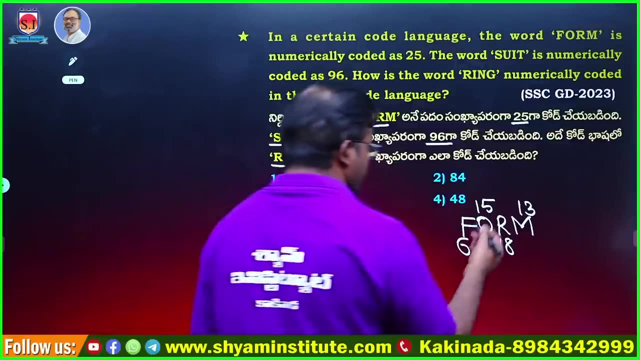 F-O-R-M, O-15, R-18, M-13. Now what will you do? First, check whether we get answers based on these numbers. What will you do with all these numbers? First, combine them. So what will happen here? 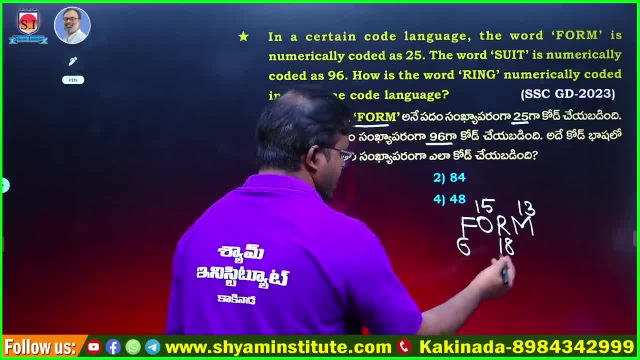 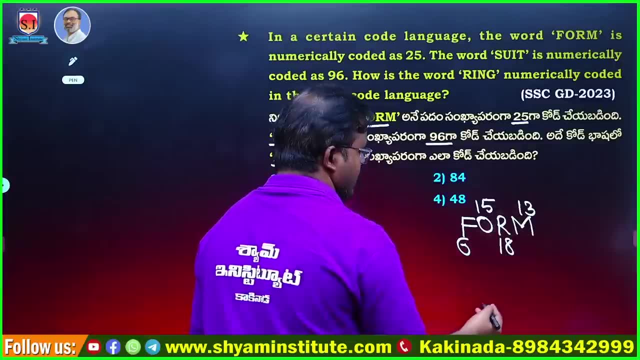 15 plus 6. This is 21.. Next, this is 29.. This is 39.. This is 39.. Next, how much will we get? 39 plus 13? So the total is 6 plus 15 plus 18. 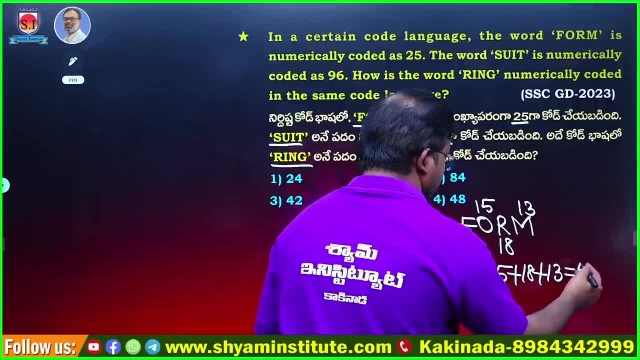 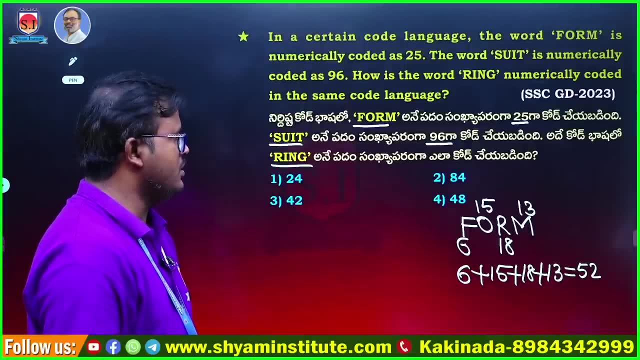 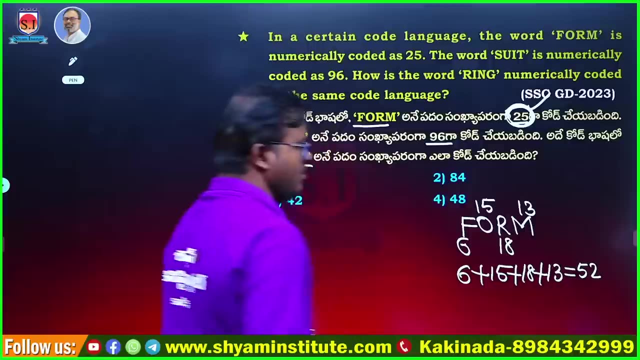 plus 13. What is the answer here? We got 52.. We got 52.. If we get 52, we didn't get 52 here, right? What number did we get? here? We got 25.. If we get 25, what can we do? 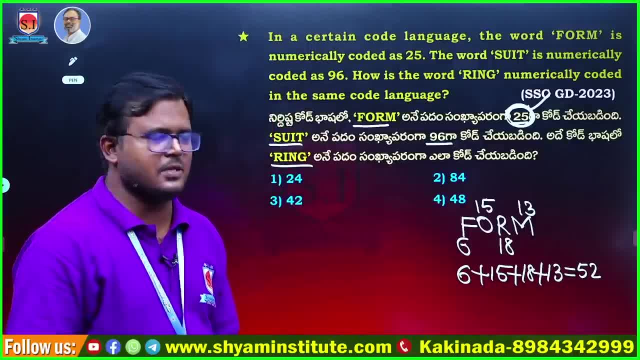 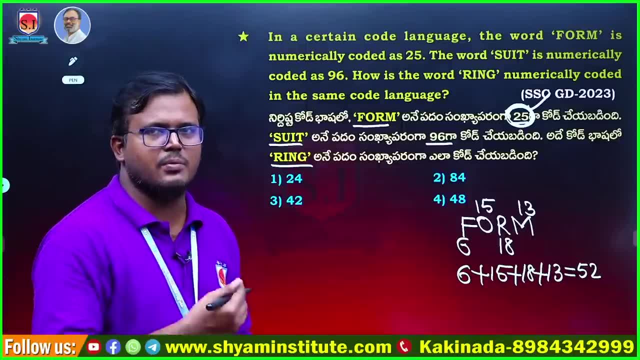 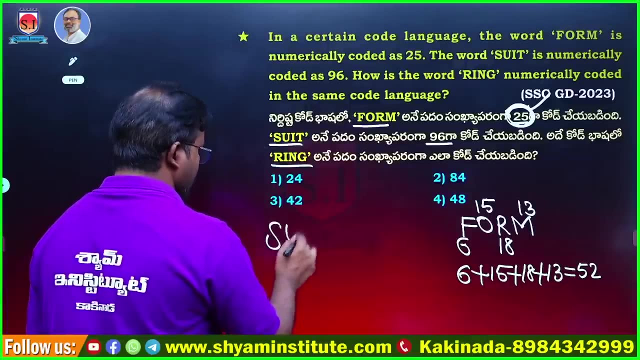 We have to think about it. What do we do to get it right? We have to check the spelling here. If we know the spelling of that number, we will get clarity. If we take the spelling here: S means 19,. U means 21,. 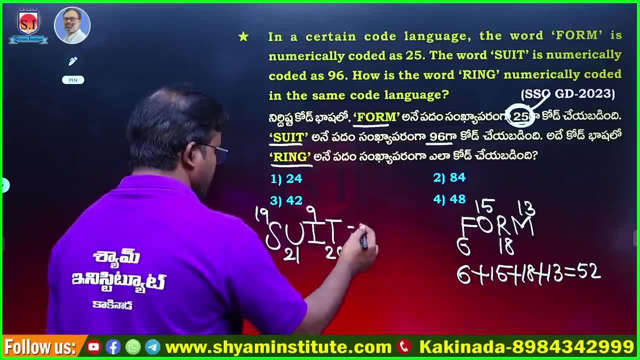 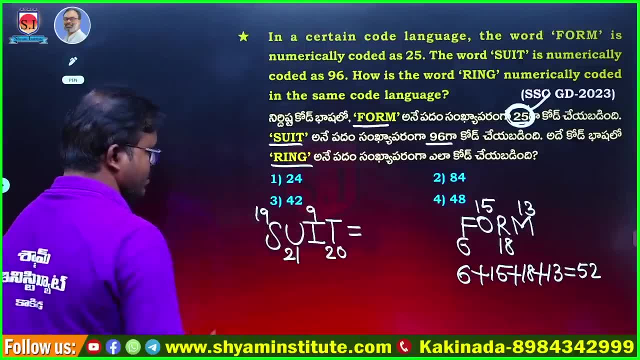 I means 9, T means 20.. So these numbers are total. 20 plus here is 50.. 20 plus this is 30 is 50.. 50 plus this is 19.. So the total number is 69.. But what did he write 69 here? He wrote 96. 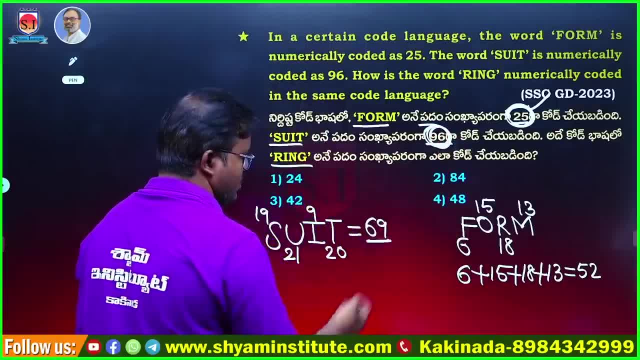 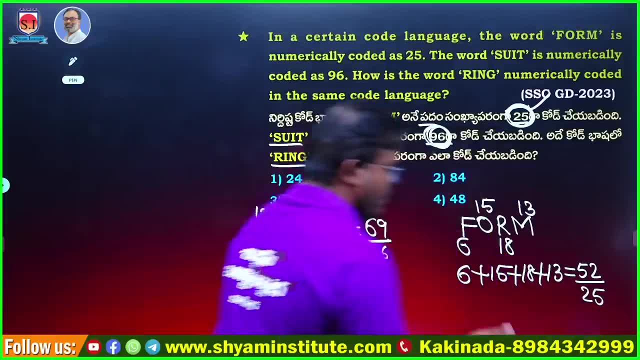 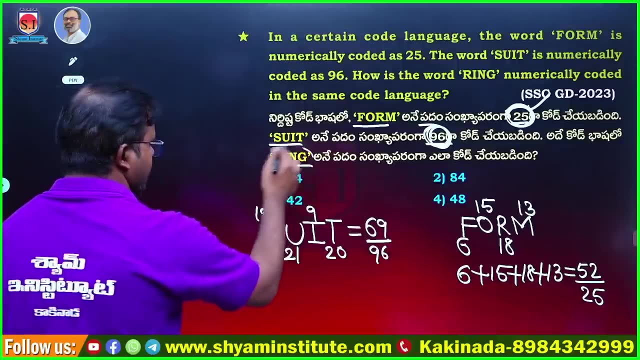 So what did he do? He is changing the digits here. If he changes 69,, it becomes 96.. If he changes 52 here, it becomes 25.. So he is changing the digits here. Similarly, go to the spelling of the ring here. 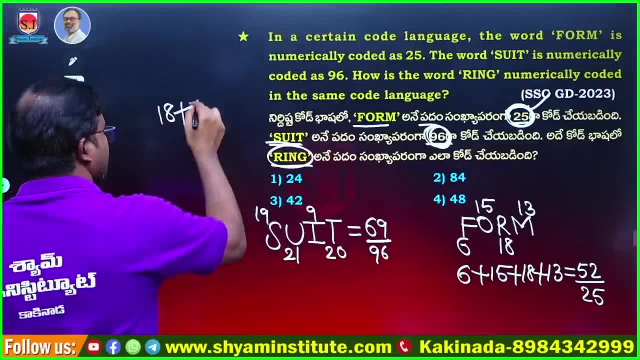 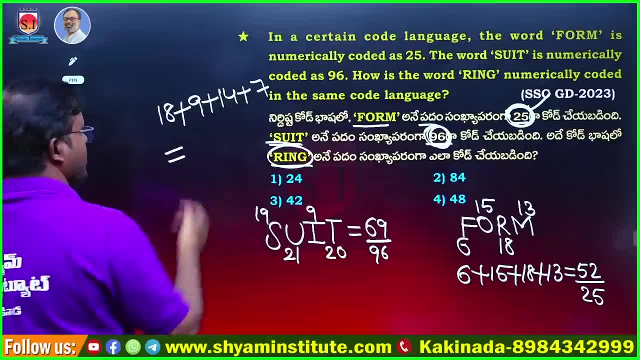 So what is 6 here? It is 18.. What is 5?? It is 9.. What is n? It is 14.. What is g? It is 7.. So let's combine all these, So tell me how much we have here. 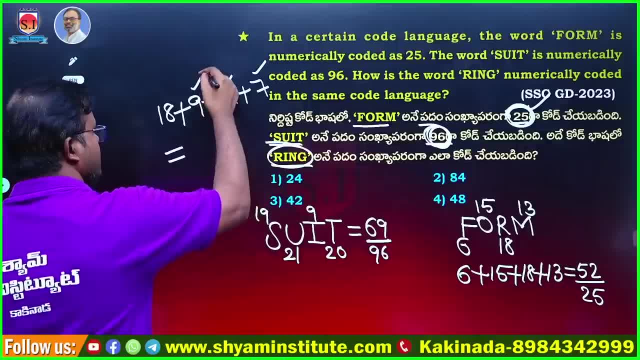 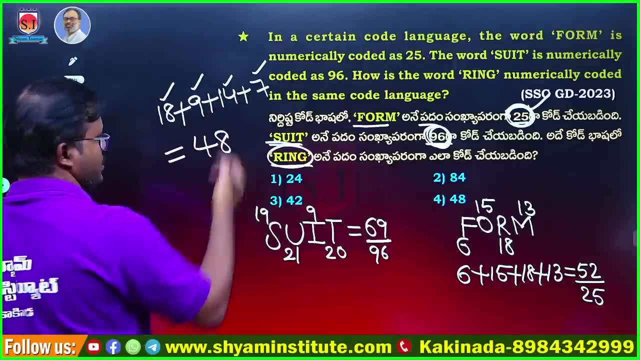 So if you observe here, as you have combined these two, 21 plus 9 is 30.. 30 plus this is 18.. So tell me how much we have here. So we have 48 here. So what do you do with the number 48?? Write it in reverse. 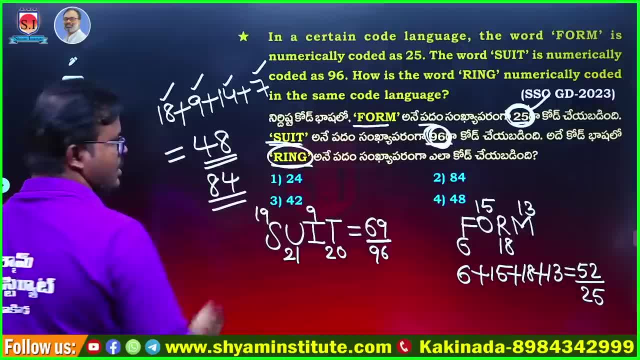 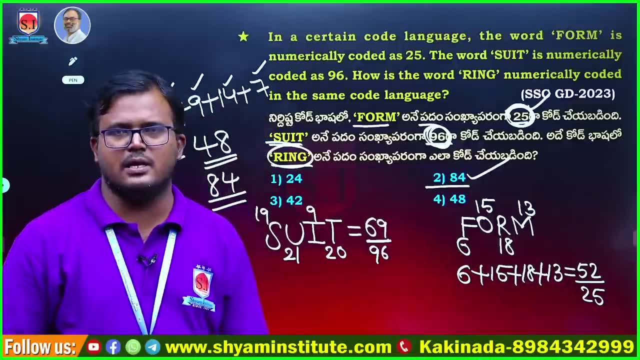 So what is happening here? It becomes 84. So where is the number 84?? It is in the second option. So you do not understand the reason for writing the spelling of form, Because I will tell you one reason. 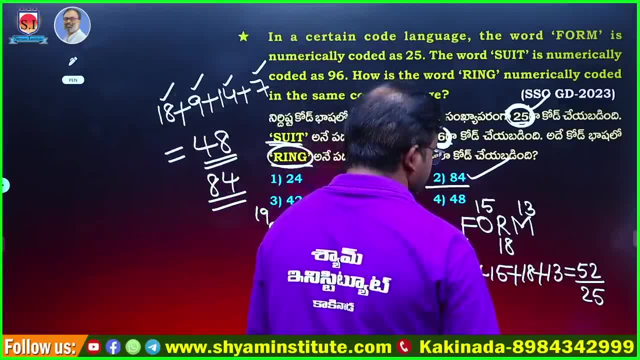 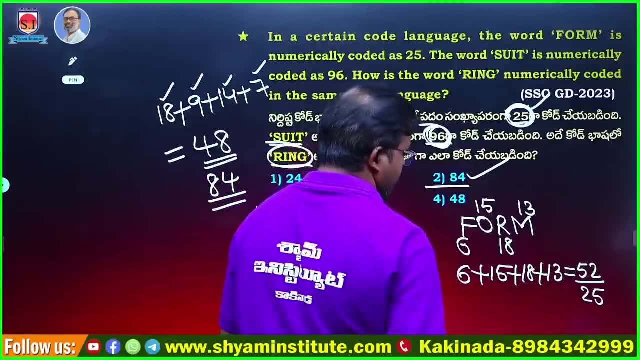 When you take the spelling of form. if you write 52 and write it in reverse, you do not know whether it is coming here or not. You can do it like this also. So you take the number 52 and subtract 2 from it. 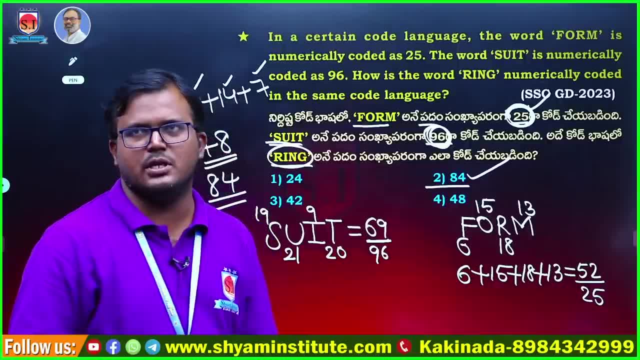 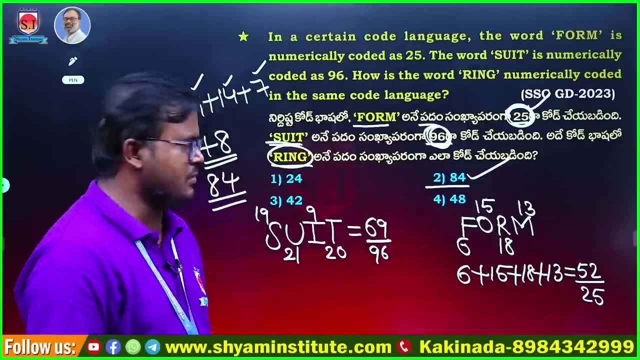 If you divide it by 2, you will get the number 25.. So what we do is we should not answer immediately, We should check the next one also and then we should answer. So everyone gave the correct answer. So, maximum, everyone gave the second option. 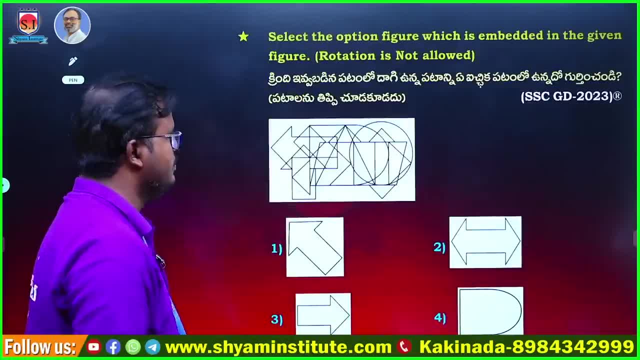 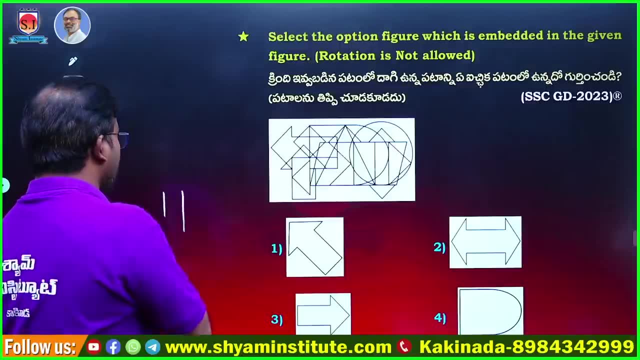 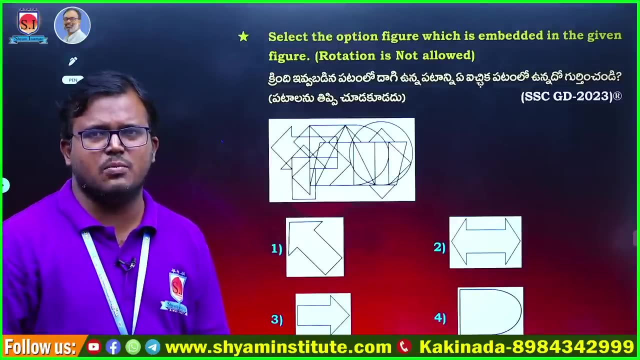 Very good. Next, Select the option figure which is embedded in the given figure. Rotation is not allowed, So what you have to observe is: in SSE GDA exam, we are guaranteed to get 4 questions compulsorily from non-verbal. 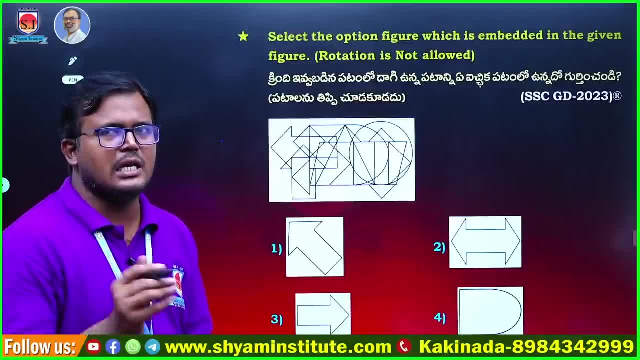 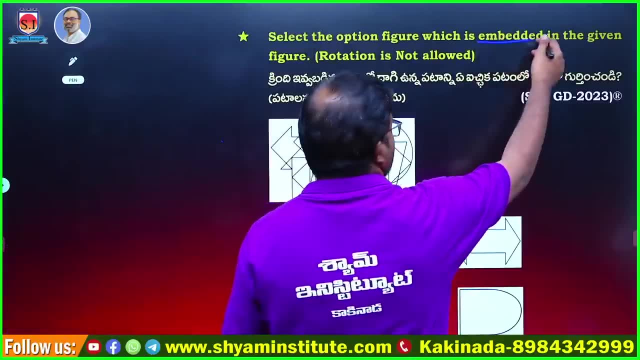 Whatever shift you take, you will get 4 questions. One of them is this. So such questions will come. This is the last year's question. What we will say is, when we come here, we will say embedded figures. So whether it is embedded figures or hidden figures, it is the same. 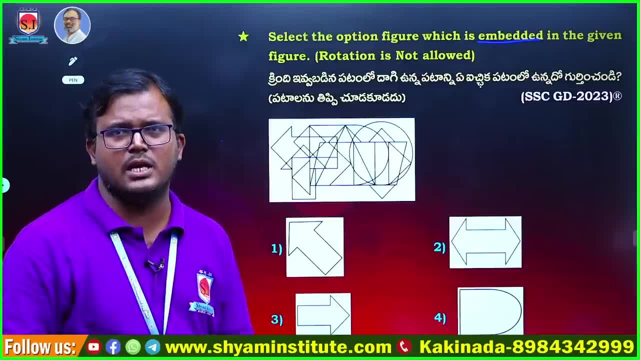 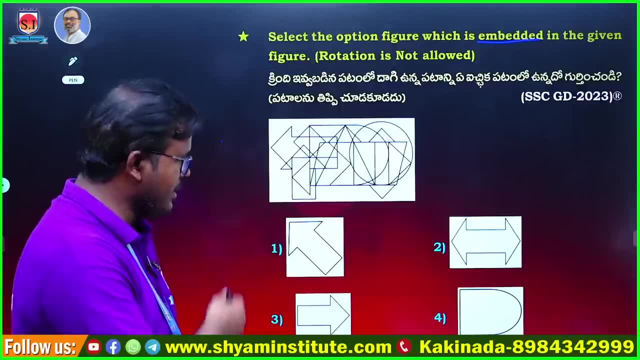 That means in that figure another figure is embedded. The figure that is embedded is given to you. So the answer is: which figure will be correctly set in these options? So now tell me, where is it in this, In the option? 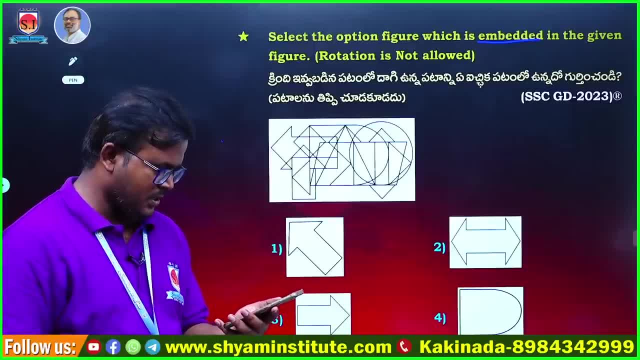 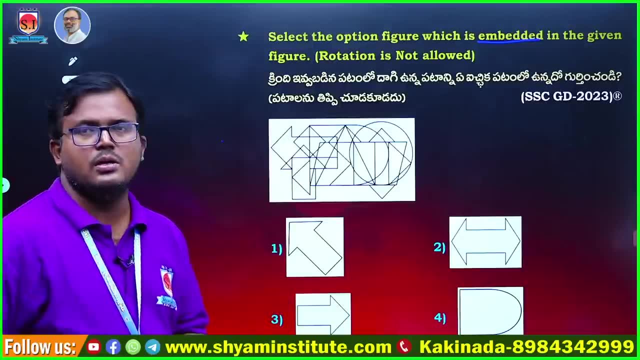 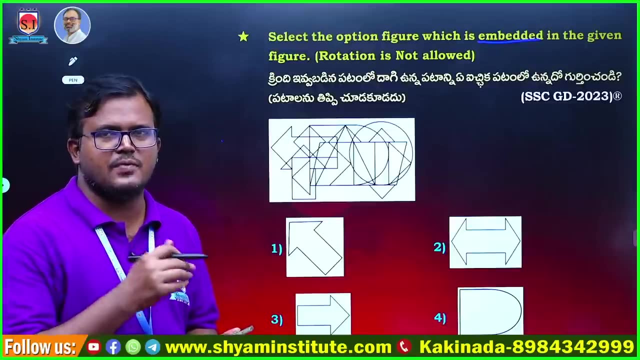 Second option. Third option, Fourth option, Fifth option: I have to tell you more. Last year, SSE GDA exam asked us what these four questions are doing is maximum. one question is given from the mirror image. One question is given from hidden figures. 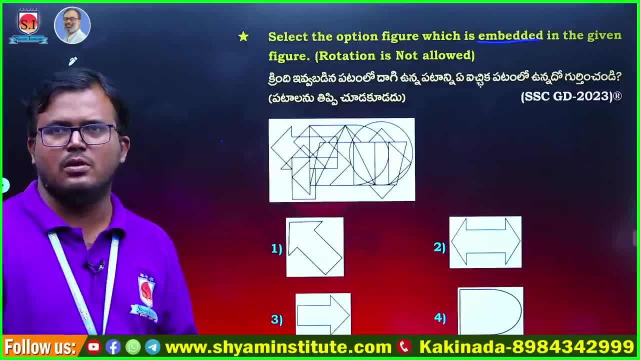 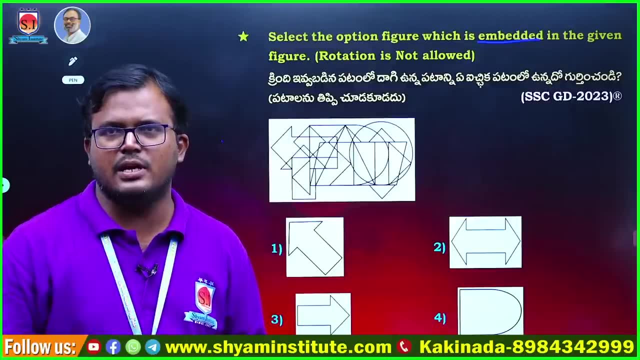 One question is given from paper folding and paper cutting. Another question is given here. So here we have figure series or non-verbal diagram series, Or it is said to be incomplete figures. So from that one question is given to us. 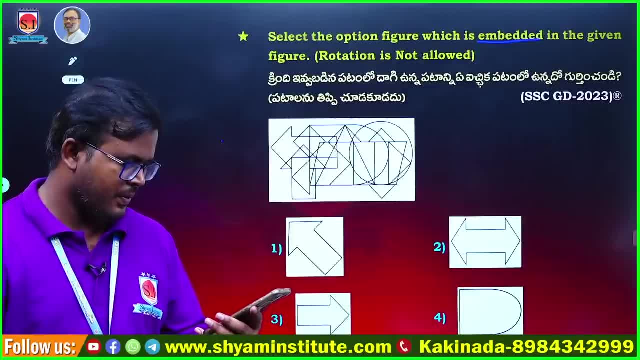 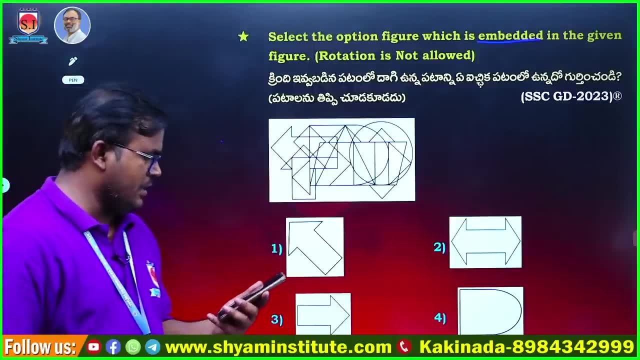 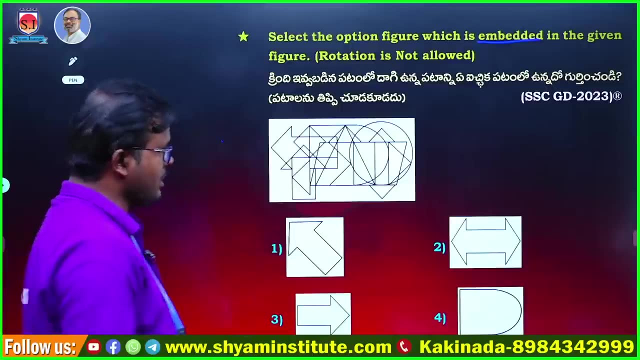 So observe it carefully. So all of you have given us option number four. So, in this diagram, what is the fourth one? Where is it? Search it once. So what is the fourth option? So what is this shape? 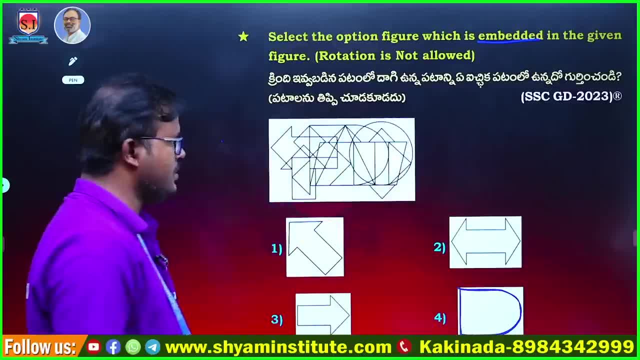 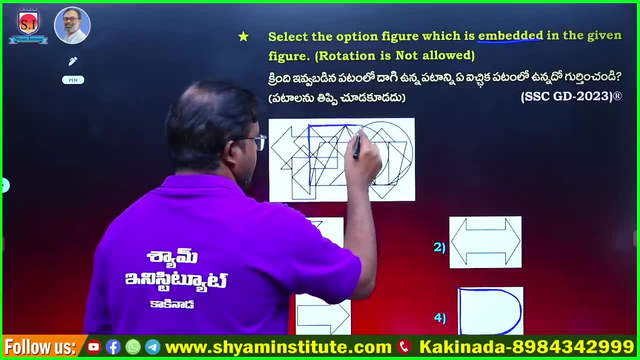 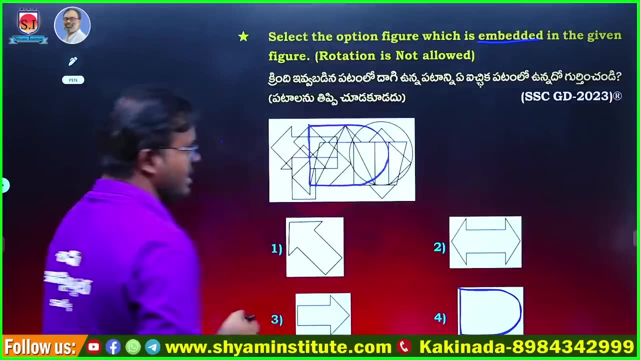 If you can really see it here, let us check it once. Where is it? Look at the first line. So what did he do in this line? So he brought the shape like this: So what is this diagram? He told you to make it a little confusing. 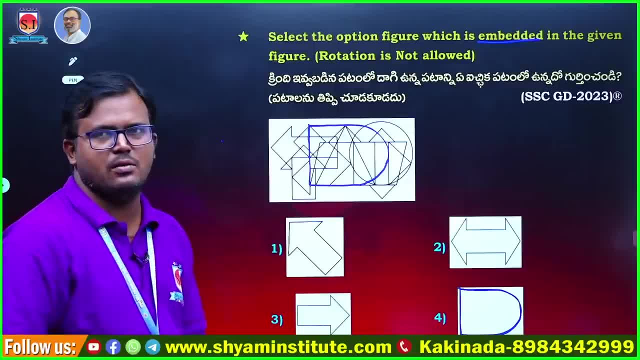 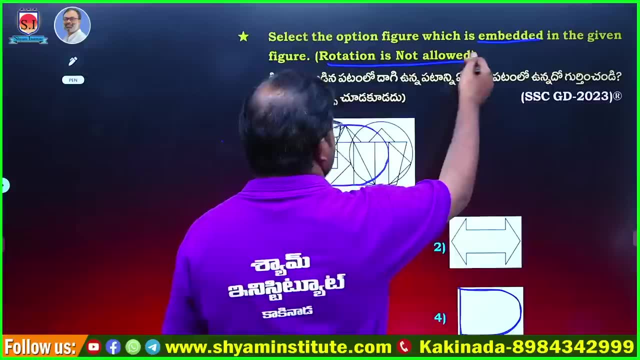 So what did he do? So he clubbed all the lines. Where do you see that diagram in the display? So that is what we can see Here. the first one said rotation is not allowed. We should not look at this diagram like this. 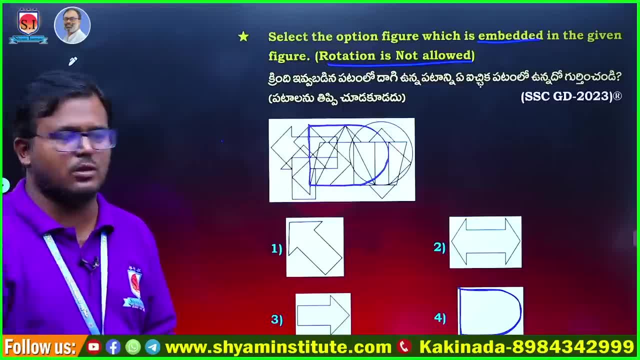 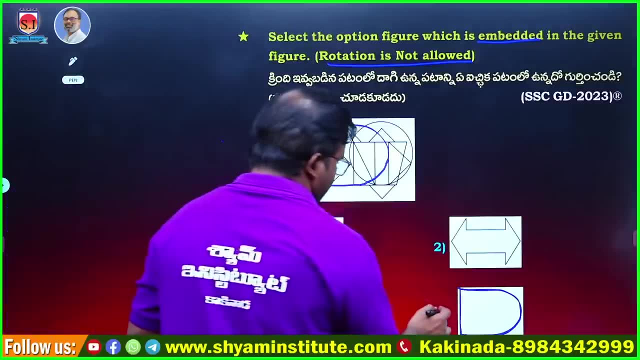 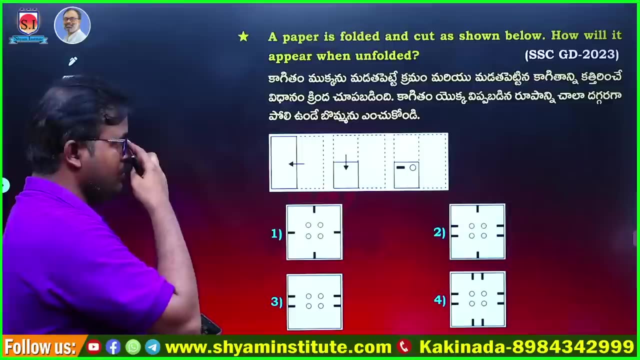 Okay, We cannot see if it is coming in the answer by rotating it. It should look like this: So tell me where the answer is coming in the guarantee. So option number four is the correct answer. So the fourth option is the correct answer. 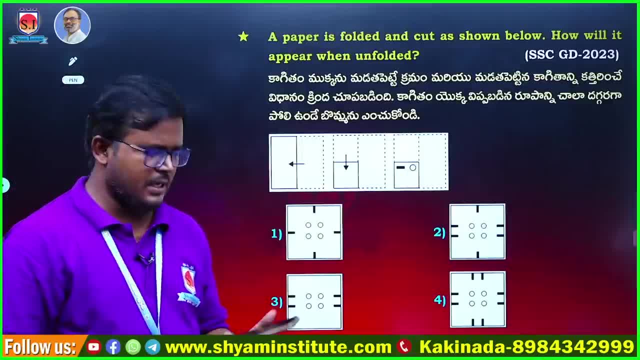 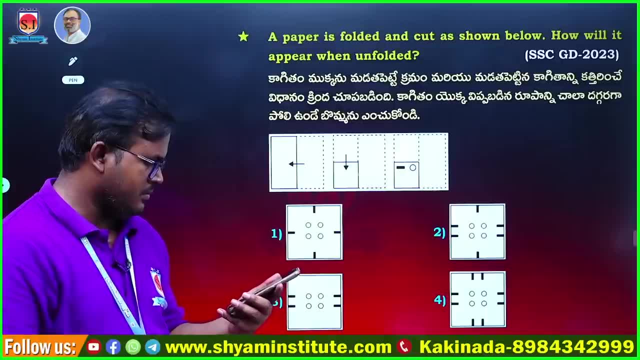 So the next problem is: we got this from the concept of paper folding. So what is the correct answer for this? So you have to tell us in the comment box. A paper is folded and cut as shown below. How will it appear when unfolded? 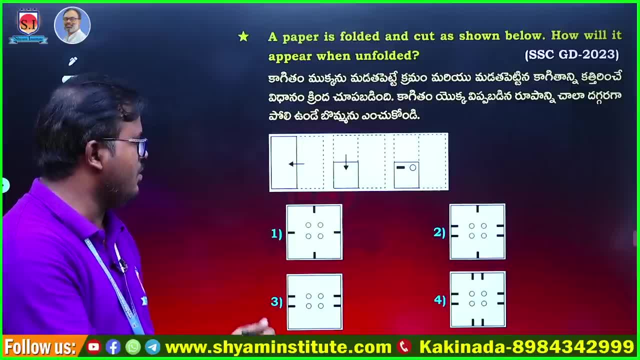 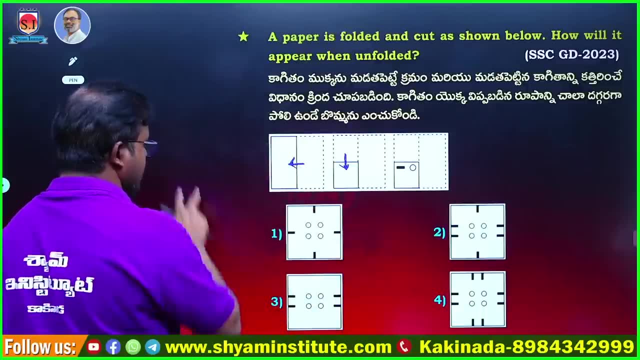 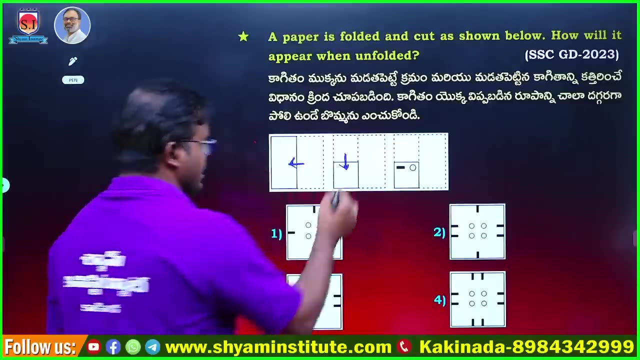 He said: Okay, Here, when we come to paper folding, you have to observe these directions to answer. What are these directions? So we have to answer according to this: Do it When we come first. he gave us the direction like this: 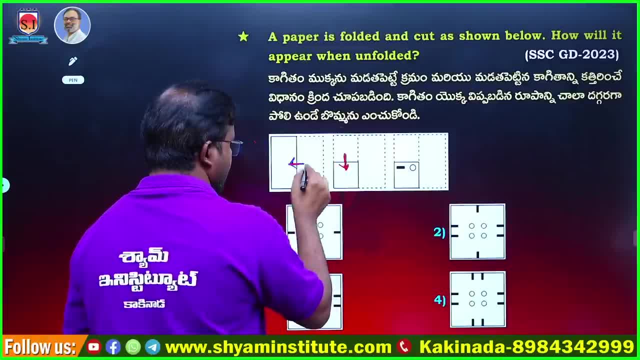 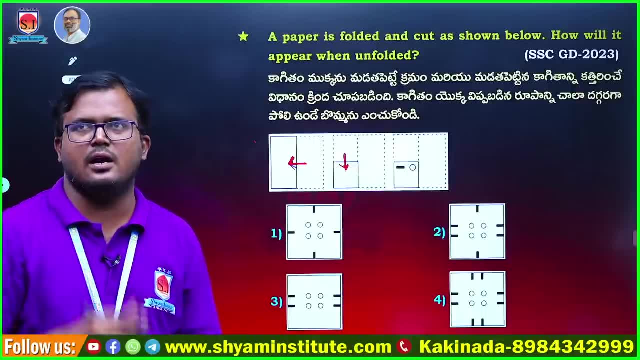 So what did he do? We have a folding from top to down- Here imagine how we are. So there is a folding from right to left. Finally, after cutting there, what are those cuttings? They are in the diagrams. 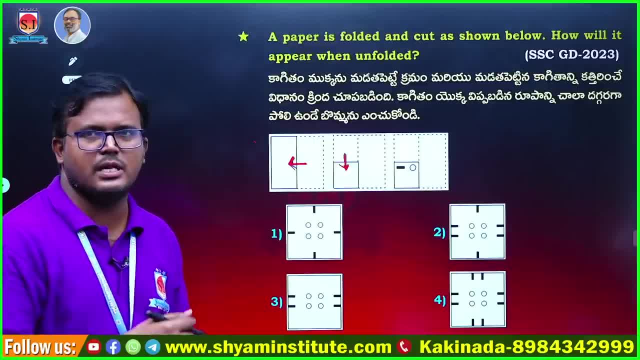 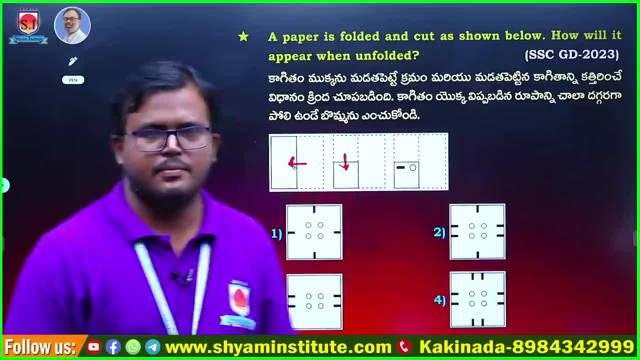 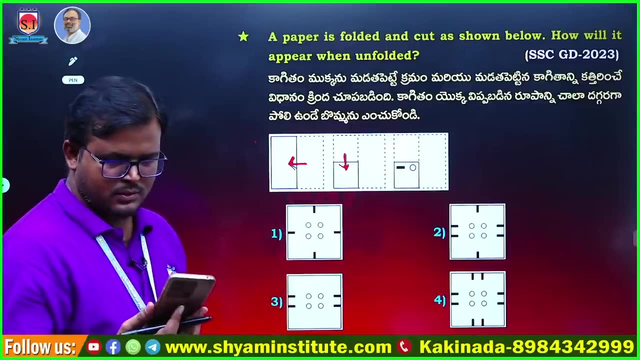 Is the first diagram correct? Is the second correct? In the third and fourth they are talking about which one is set correctly. So once see which one is correct for me, Tell me which one is correct. So once you, once you see which one is correct for you. 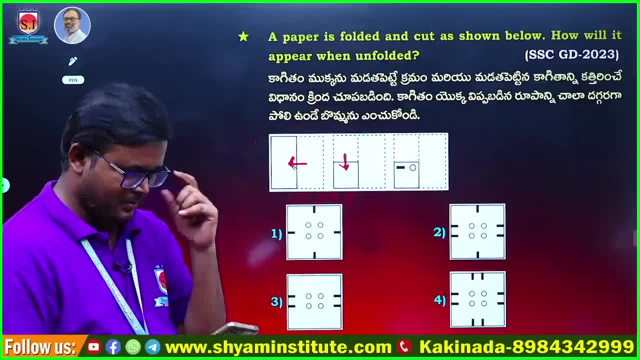 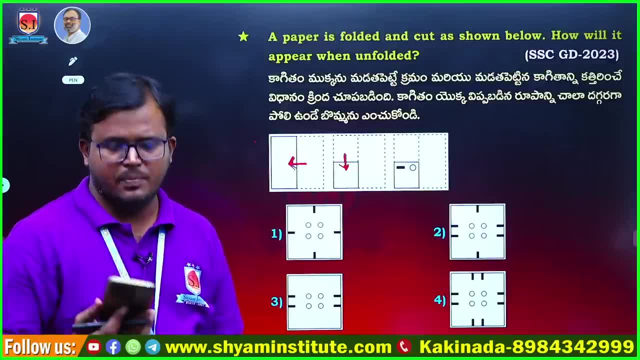 you have to tell me in the comment box. So in the exams that you are going to write tomorrow, these models will appear as a guarantee. Keep in mind Paper folding, paper cutting or hidden figures, or, as I said earlier. 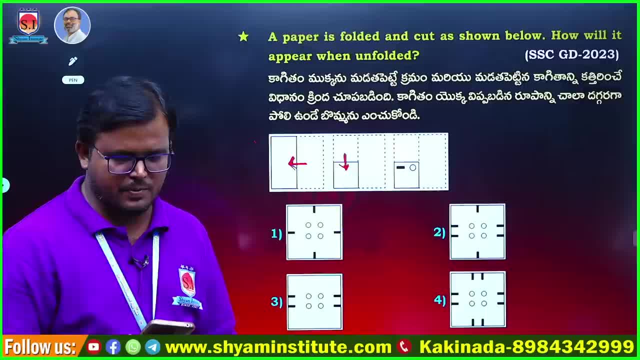 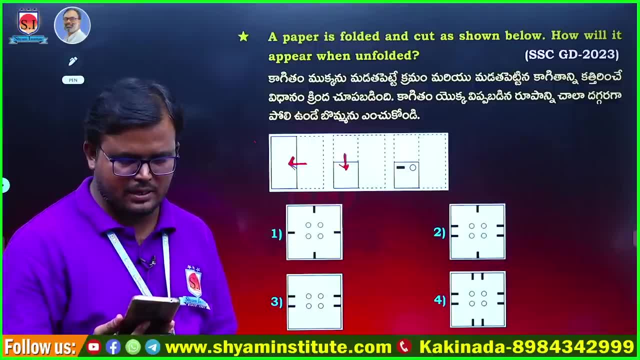 fuzzil tests. all of these are for you, So in the exams that you are going to write tomorrow, they will come as a guarantee. The one who gives them as a guarantee is because he is providing us with a blueprint. you can follow this live session completely. 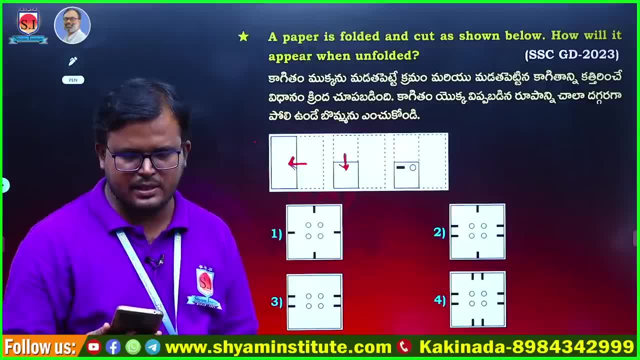 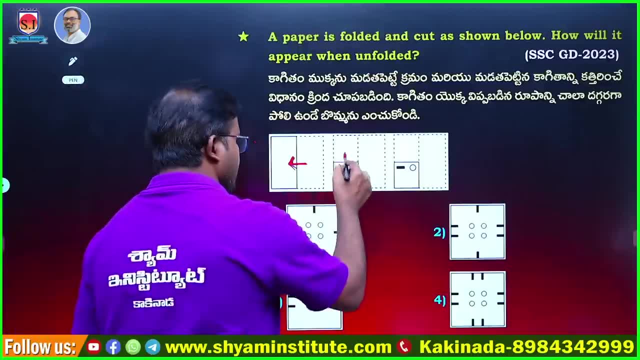 If you follow this live session, you will not miss any of the bits in it. So what do we do first? So let's see the direction. So what is the direction given to us from the top to the bottom? If it comes from the top to the bottom? 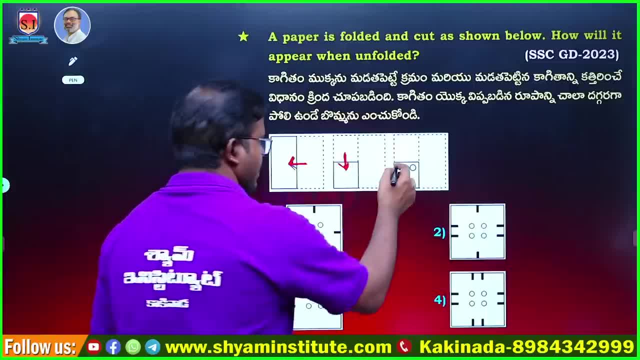 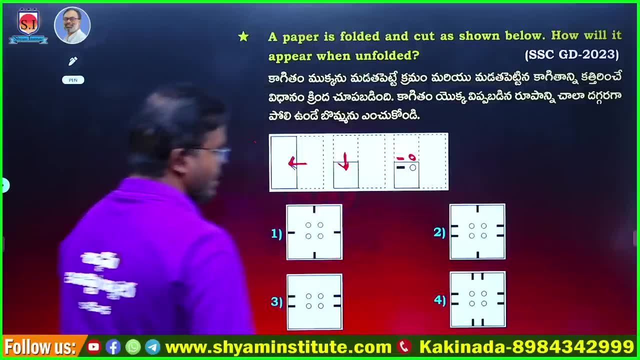 it is guaranteed to be a water maze. If you write a water maze for it first, this black color will come here. This circle will also come here. So what should be guaranteed? There will be two circles. Then where is this black color box? 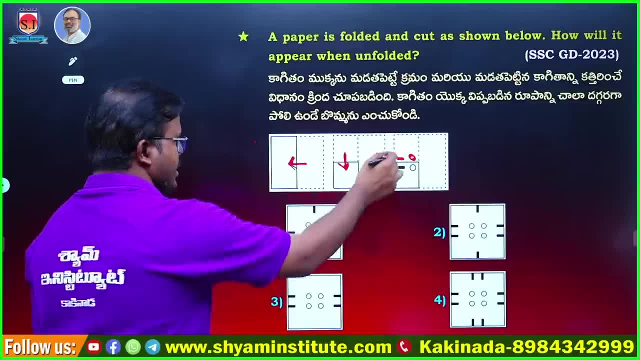 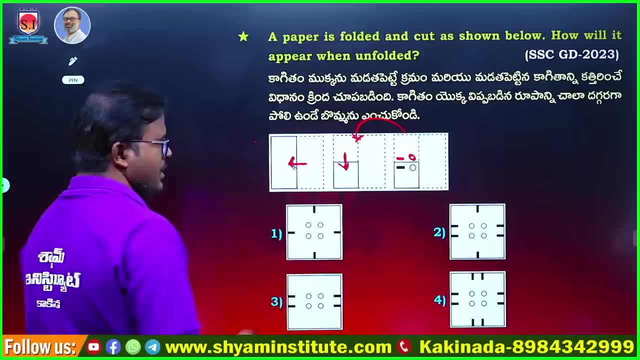 It is the same for both the top and the bottom. So what do we do for this box again? So when we go to the second one, when we go from this third one, what will be the diagram? So if it comes to the first one, 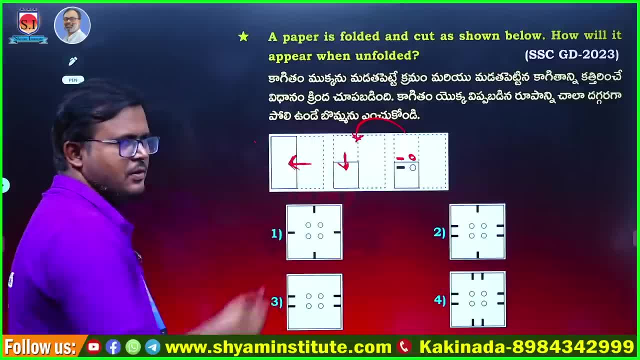 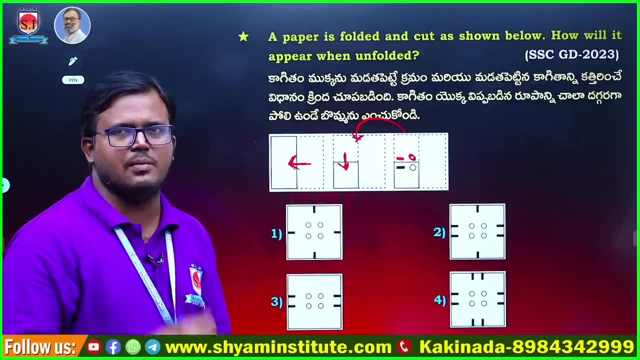 then what happens here? Right to left, So right to left, If it changes from right to left, will it be a mirror maze or a water maze? So you have to think once: Where does right to left change? It changes in the mirror maze. 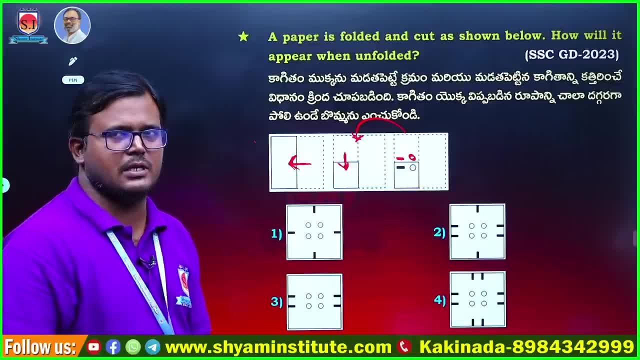 Similarly, where does the top and the bottom change? It changes in the water maze. So the first thing that is written is the water maze. Now what should be written for the guarantee diagram? So we have to write the mirror maze. 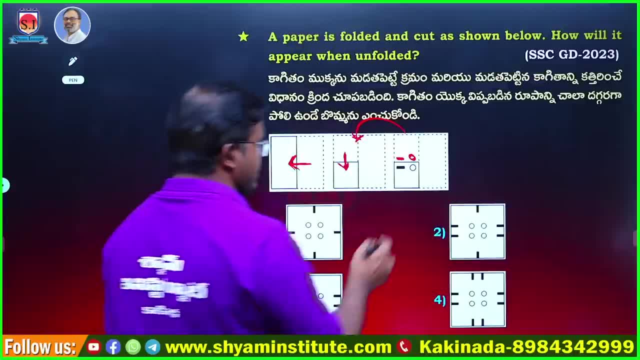 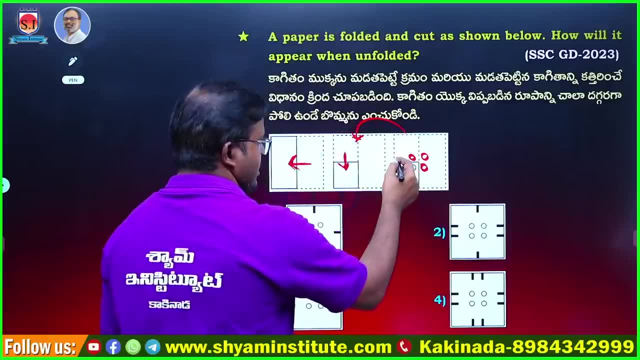 Then what happens when we write the mirror maze? If we write the mirror maze, then this circle will come here again. Next, another circle will come again. After that circle comes, what will happen? Where will they come for the guarantee? 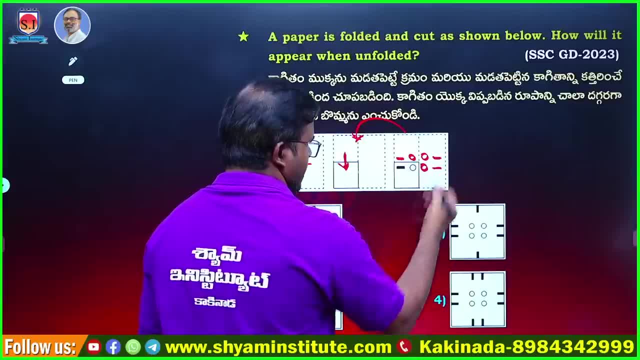 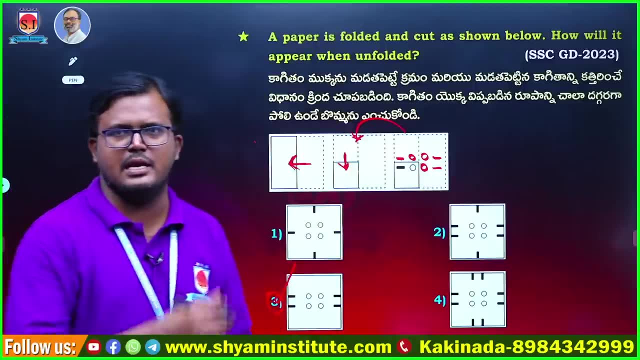 It will come in the ending like this: Now, where is the correct answer for us? So in option number 3, it is correct. So which is the third option That will be the correct answer for us? So those 2.. 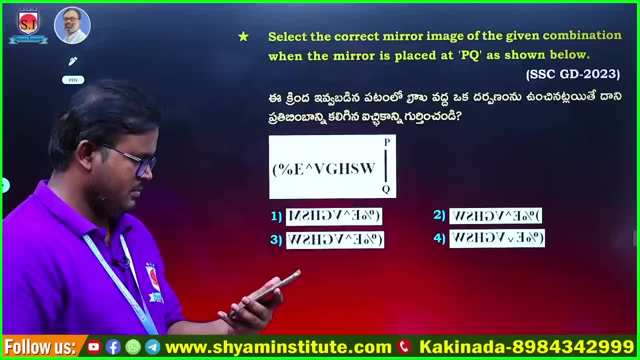 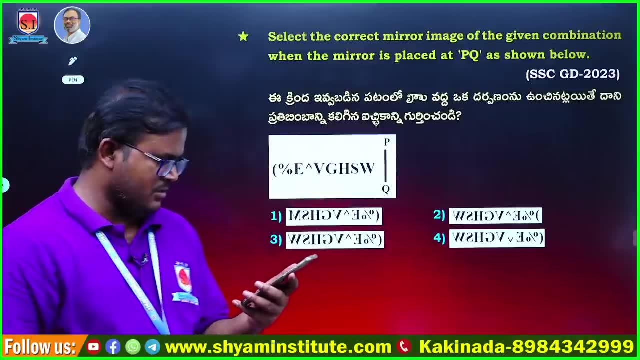 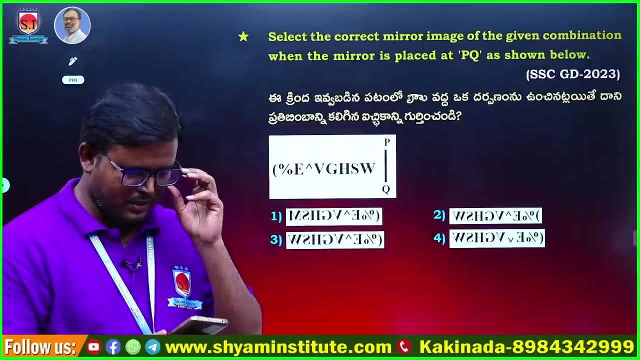 This pull, we will call the second option. This is the third option for us. it will come Next. you can move like this, because that is the start: Do the correct answer at any time Next. So all are doing all the correct answers. 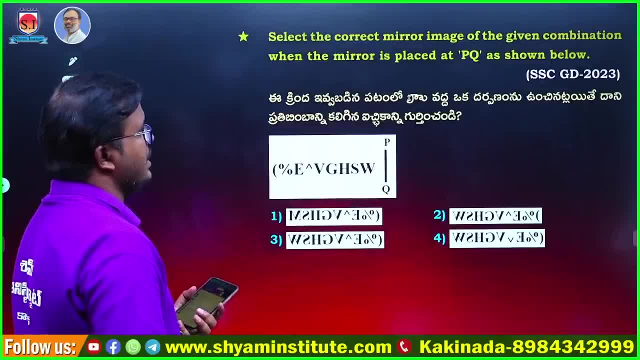 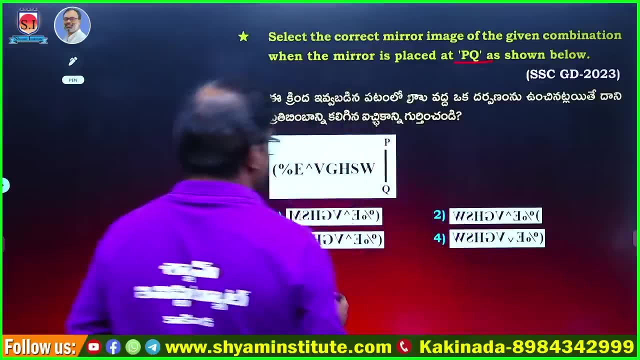 Subhanimaman says: 4 in the middle. Yes, there will be 4 in the middle and combination of the mirror is placed here to PQ on the face and I do. okay, now money kicker of PQ on to you, let us make a ghani and take a place, logan. 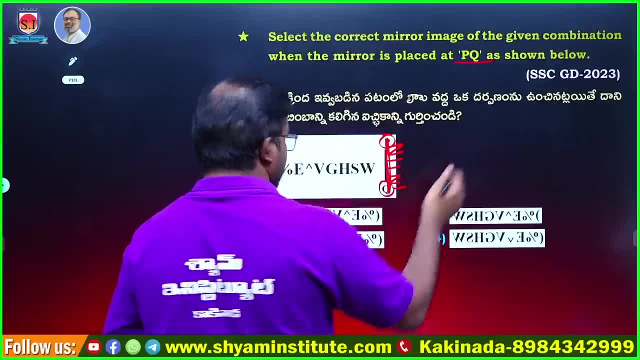 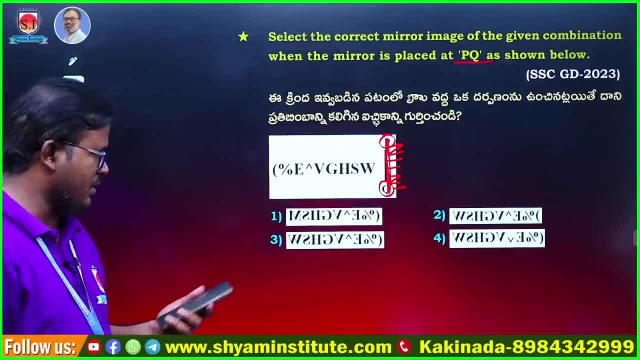 imana mirror. this could not take a camera and a lot is Kunti. any key me sanity wanted a little, though I am a zoom on a kitchen at one T options, low money key. a decryptor's much, Elijah, I'm going to know to check, Jenny Marie. 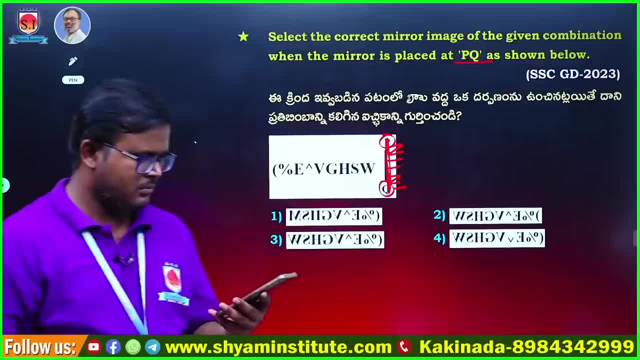 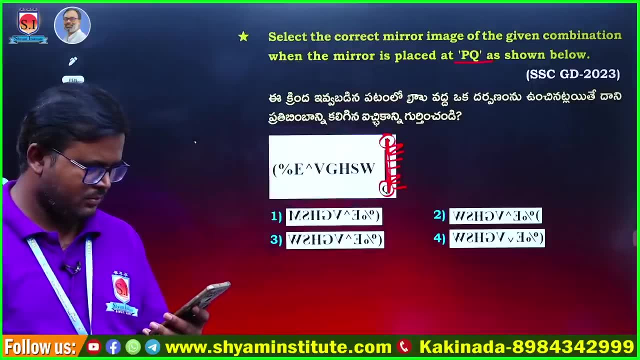 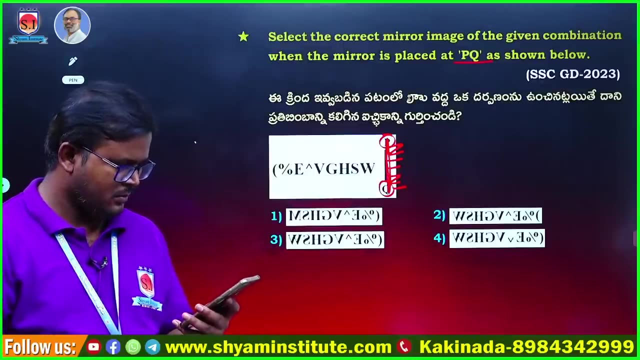 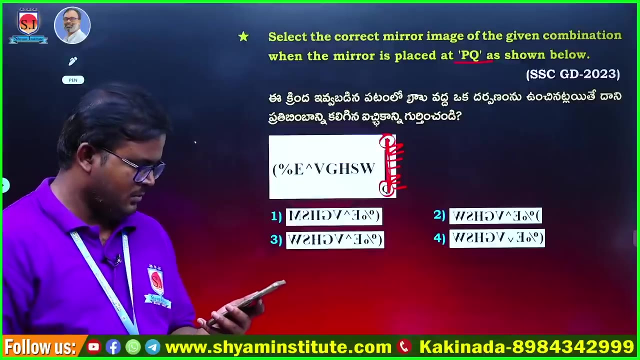 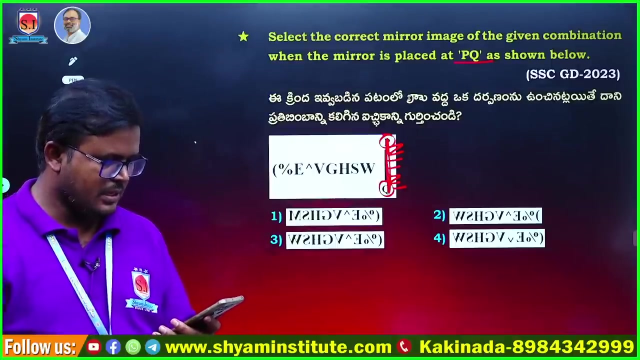 don't care the correct answer or smell any. so first or second or third or fourth or third option in go change option verification that I just couldn't easy guy put on a lot of questions again. I can offer the verification method a best process and they're going to make time on a main. 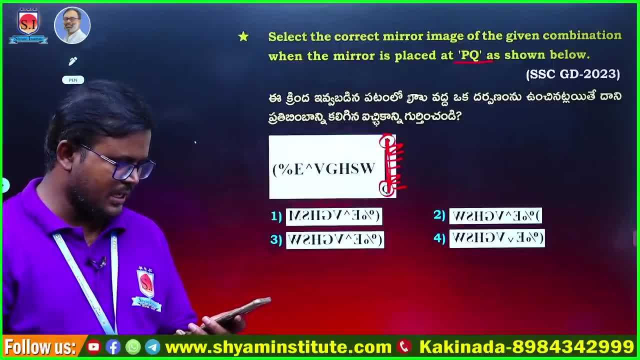 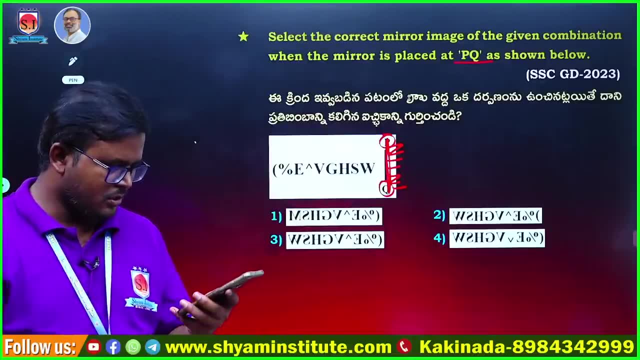 chile mega here each in our absence of money. people coughs and I need a guarantee. came out, the money key completely got wrong. I put a coughs on the middle of a dance, so drugga Bhavani garu thought of snitcher and a society. 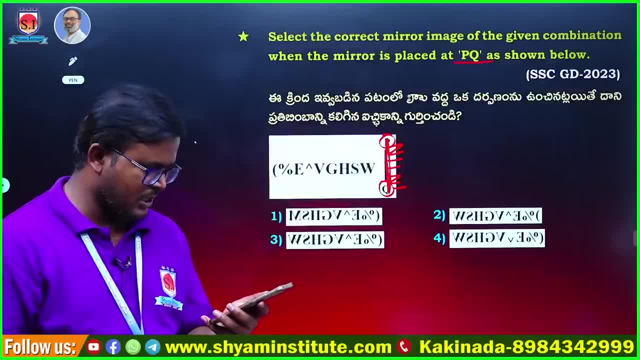 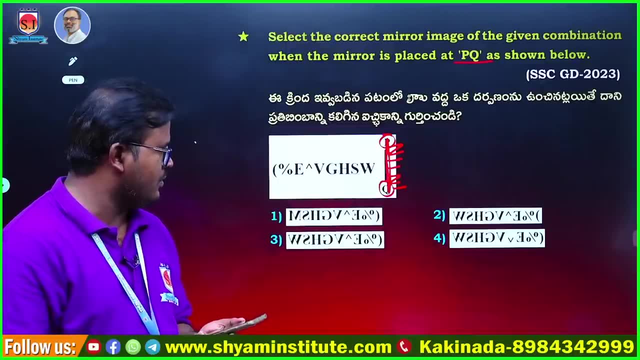 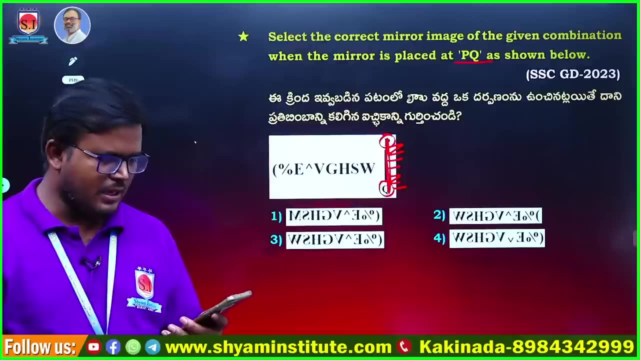 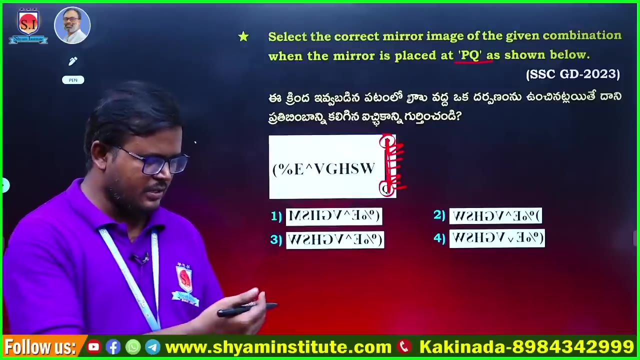 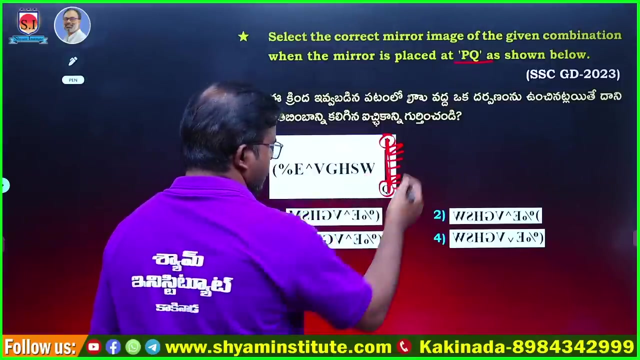 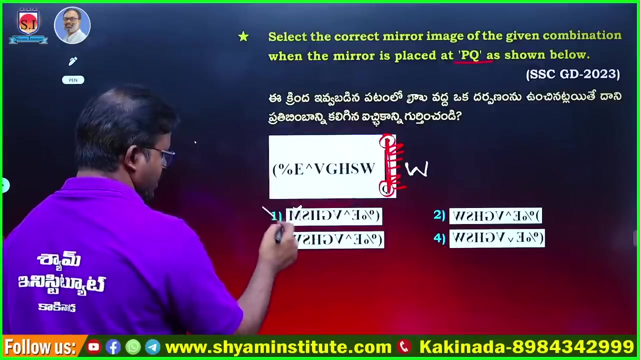 Buddha Allah thought of son Kusumant, fourth of son. so, Andy, okay, my third program, for that's a bunch of Technical kitchen think, But the first thing they do is cancel it. If you observe the rest of the letters, let's see the options. 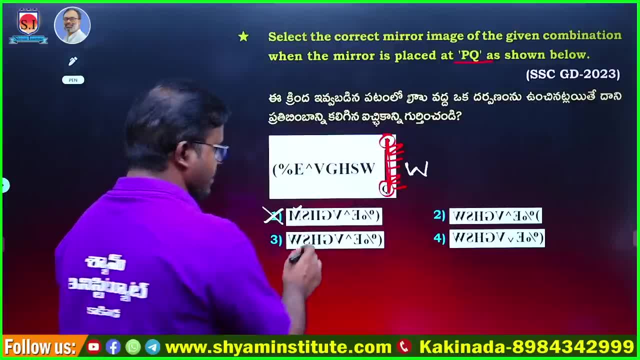 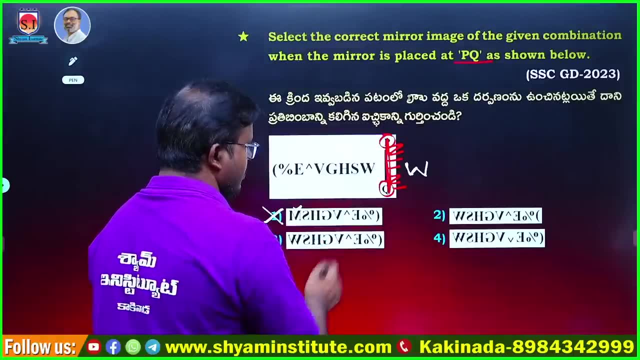 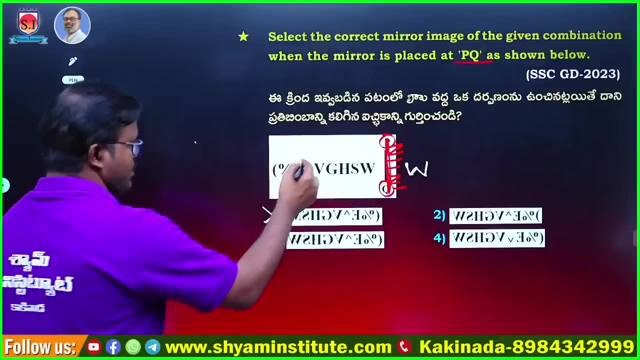 If you go by the options, you can see that the letters S and H are the same. The letters G and V are also the same. What should we do next? So observe this symbol. If you observe this symbol, you can see that it is at the top. 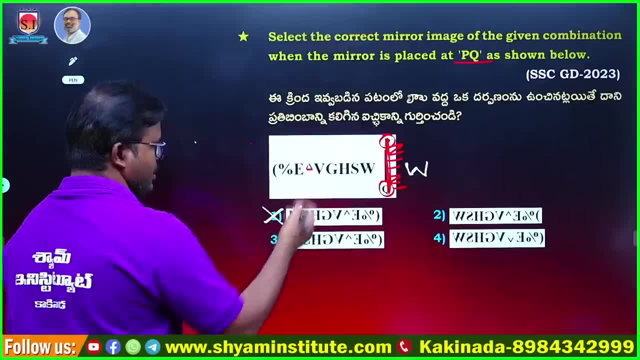 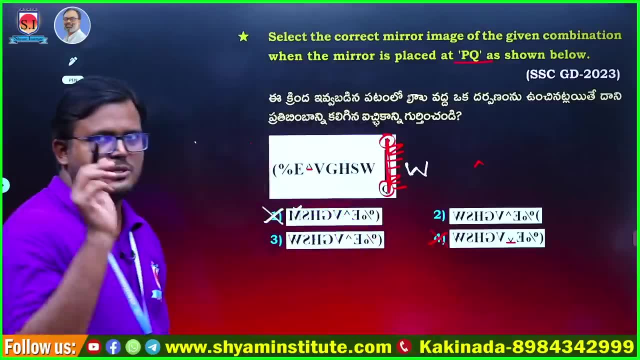 If you observe here, it will come at the top. If it is at the top, what should you do? It should come at the top, But since it is at the bottom, the first one is wrong. As I said, look for the mistakes in the options. 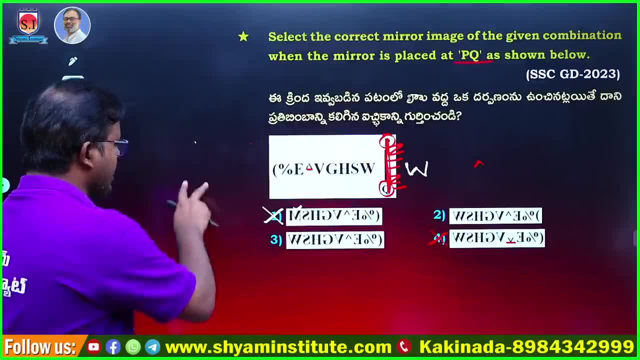 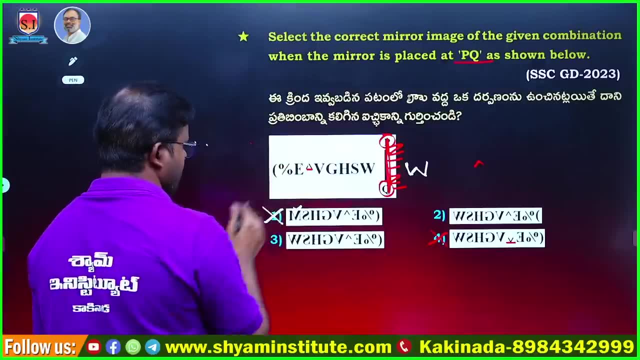 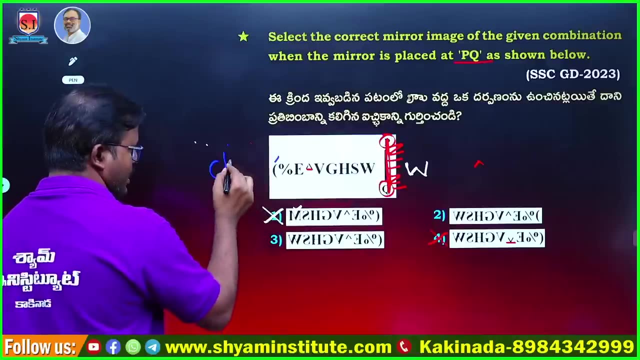 Next, we have two options left. Let's see which is the correct answer in those two options. To get the answer, we have to observe this symbol at the end. Observe this symbol at the end. If you take a mirror image for this, the image will look like this: 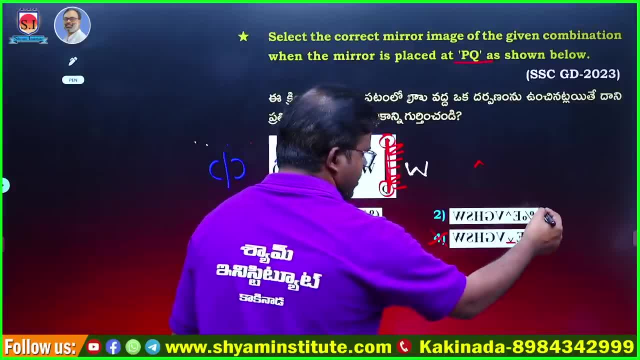 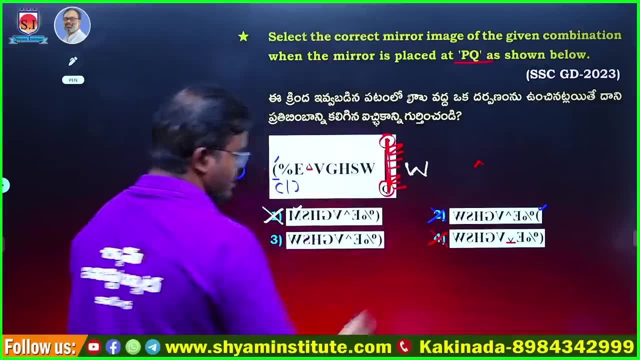 We can see the image here. Observe this: What is happening here? It looks like it is at the top, But since it is at the top of the mirror, it looks like this. So this is also the wrong answer. The answer left here is the third option. 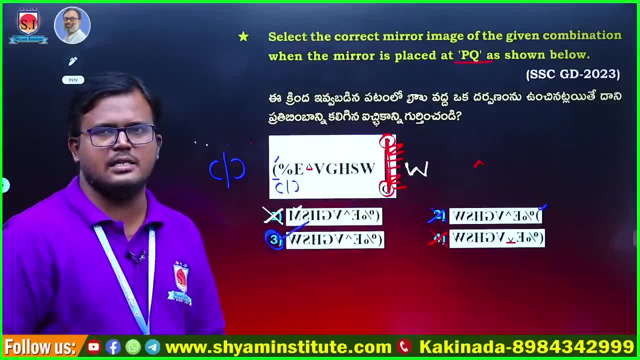 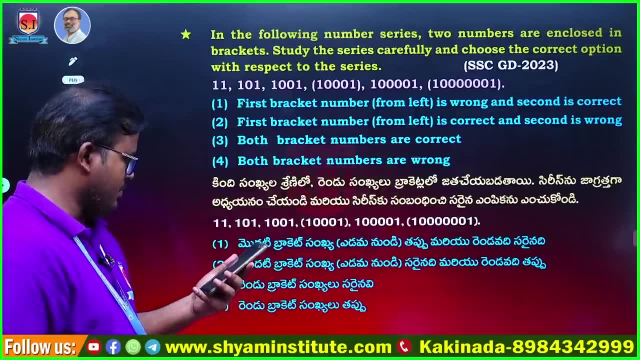 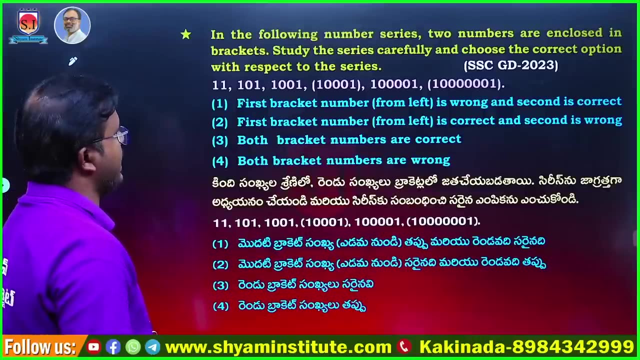 If we take the third option, it is the correct answer. The third option is the correct answer. Next problem. So in the following number series, two numbers are enclosed In the brackets. Study the series Carefully And choose the correct option with respect to the series. 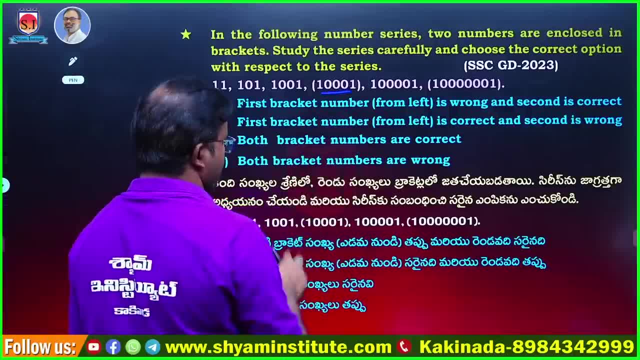 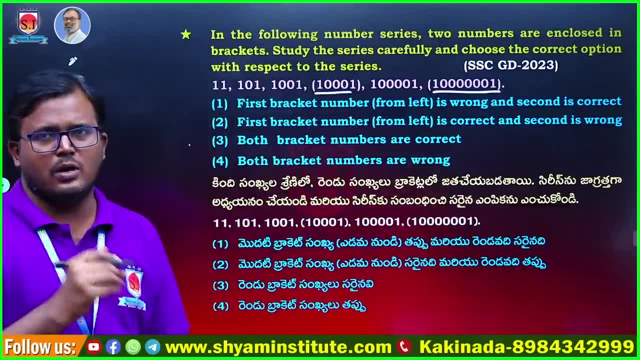 So what he is doing here is: if we observe this series, we have the numbers in the bracket. If we observe the numbers in this bracket, he is saying that there is a number guarantee in this. There may be one mistake in it. 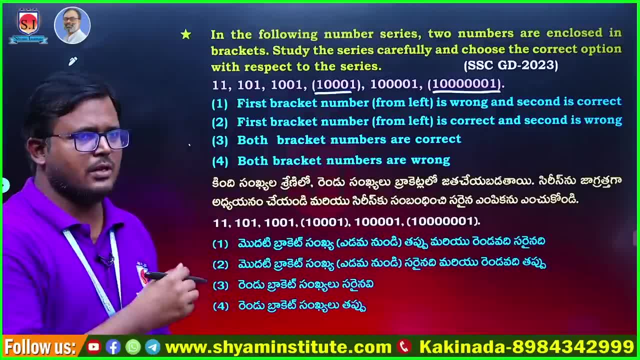 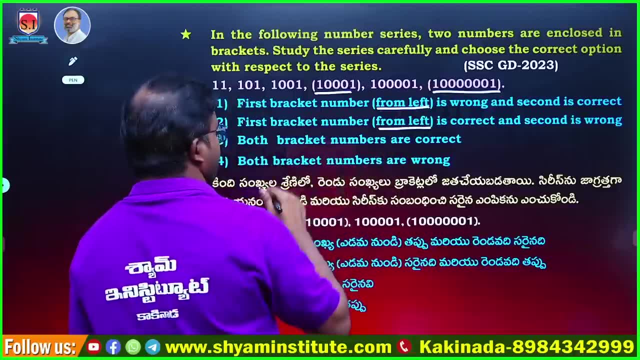 Otherwise, when we come here, there may be two mistakes. And when we come here, if we take it according to the options we are given from the left- That is, when we go from left to right- the number in the first bracket is wrong. 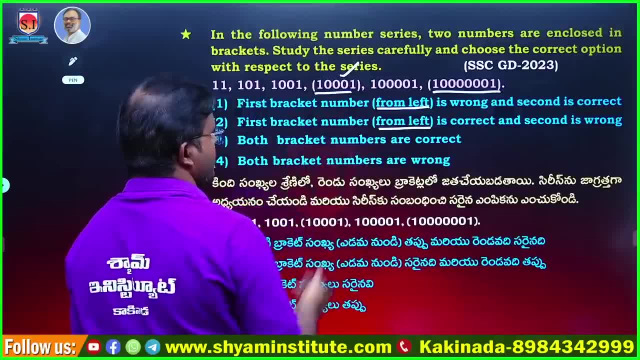 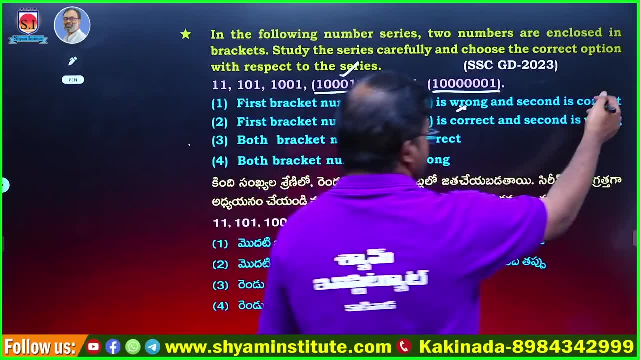 He is giving us the first option. So when we come here, what did he say to us? So when we come to this bracket, he said that this is wrong for the first one. He said that the second one is correct. So what he is saying here is not like that. 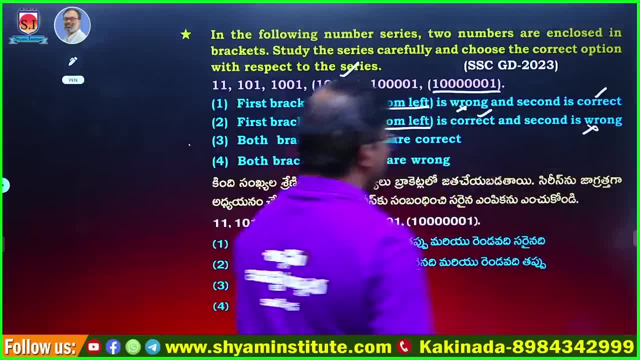 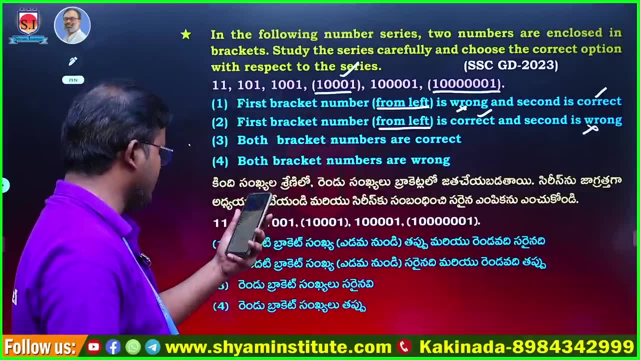 This is the number. guarantee This is correct. This is wrong. Then what is the third option? We have two correct answers. Next time, there are exactly two wrong answers. So tell me what is the answer. Tell me, Tell me which is the correct answer about you. 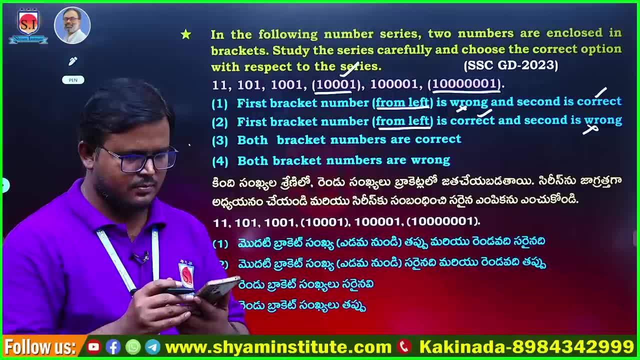 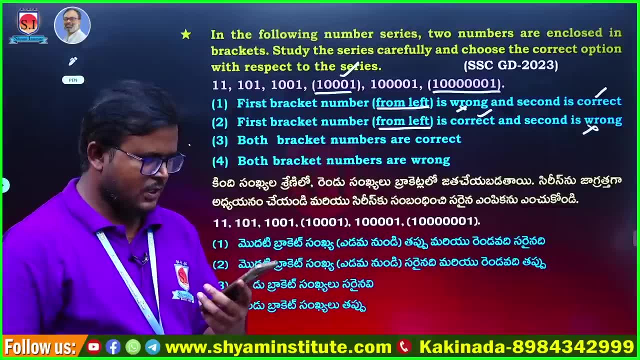 You have to tell me. We have to give you the value of n. So what is the answer? We have to give you the. we rate your fifth Hayes number. Let us write here half one, fifth the three, if you like. 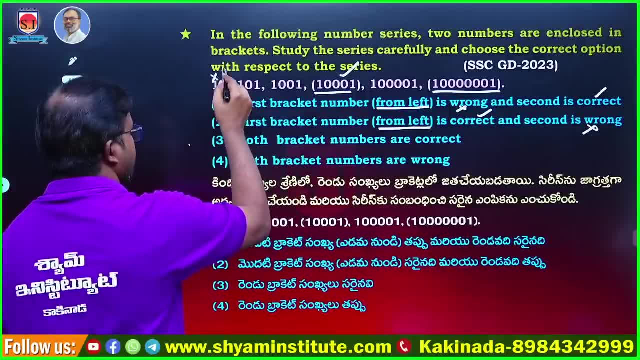 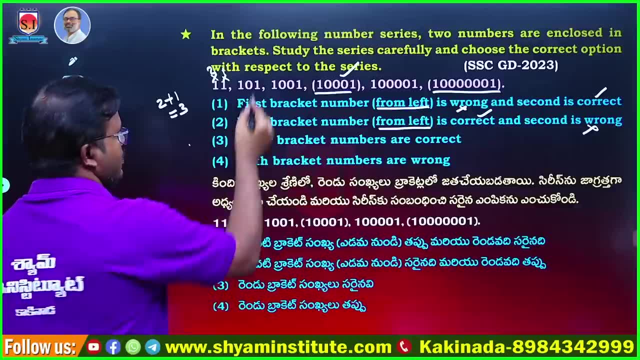 So else, how to we get one? fifth, We still have to do this right, But how? How to do it? So what, we can do this. Let us cut out all this. Let us cut out the two on the Saver here also. 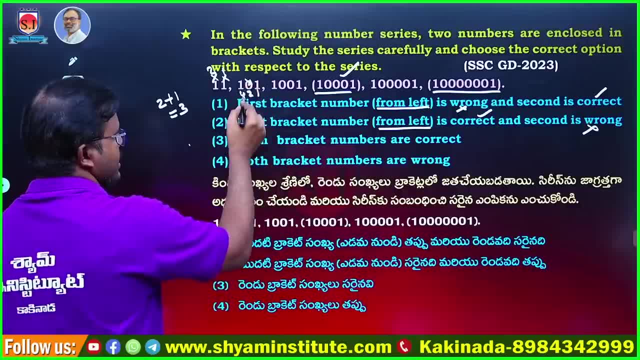 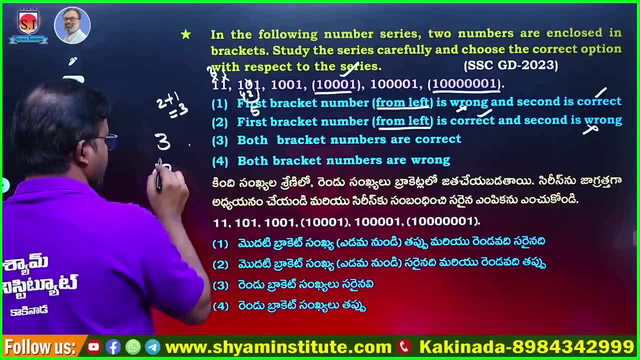 Now what will you do with the number near 0? You cancels it and add these two numbers. How much will 4 plus 1 be? It will be 5.. So the first number will be 3 and the next number will be 5.. 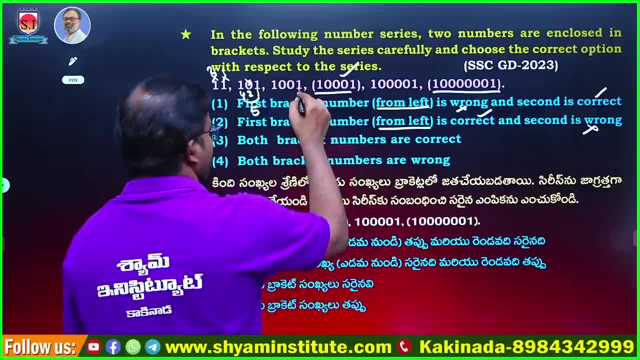 Now come here again. This time, what will happen? 1. If we double it, it will be 2. How much will we get? if we double it? We will get 4. If we double it, it will be 8.. 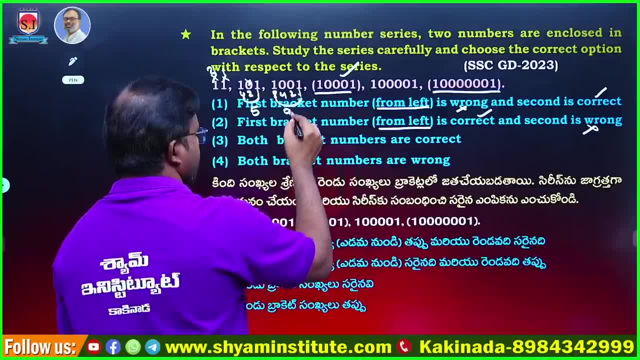 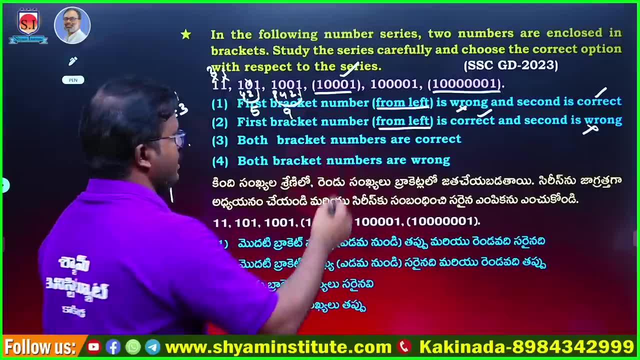 So here what will happen: If we add 8 plus 1, we will get 9.. So, as you can see here, the next number will be 9.. Now what will happen? Come here again. So here what will happen: 1.. 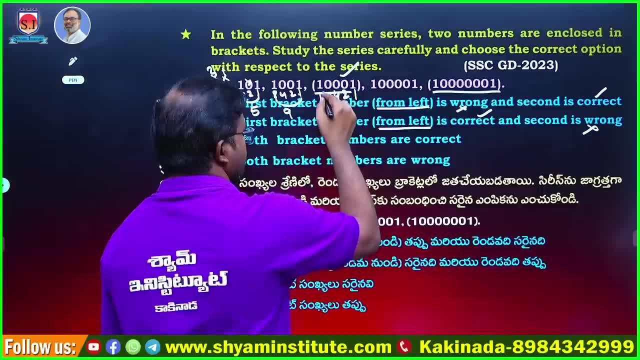 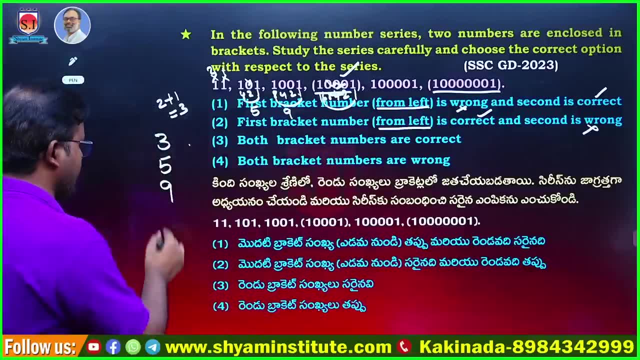 If we double it, it will be 2.. 4. Next, 8. Next, 16.. Now add these two numbers. What will you do with the number near 0?? You cancels it. Now what will happen? We will get the number 17.. 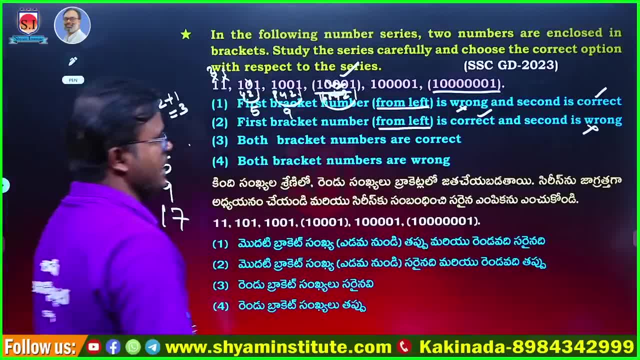 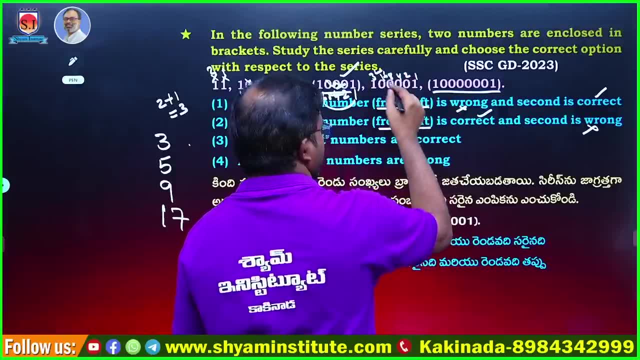 We will get the number 17 here. Now come here again. So, if we take this, it will be 1,, 2,, next to 4, 8,, 16,, 32.. Now, since these are 0s, if we cancel them, we will get 32 plus 1.. 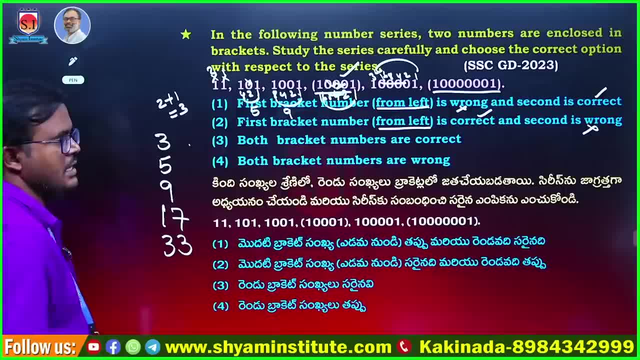 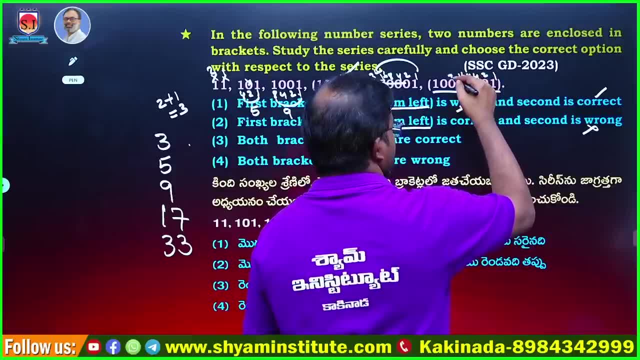 So we will get the number 33.. Now let's go to the last one. If you observe here, first is 1.. If we double it it will be 2.. Next, 4, 8,, 16,, 32,, 64.. 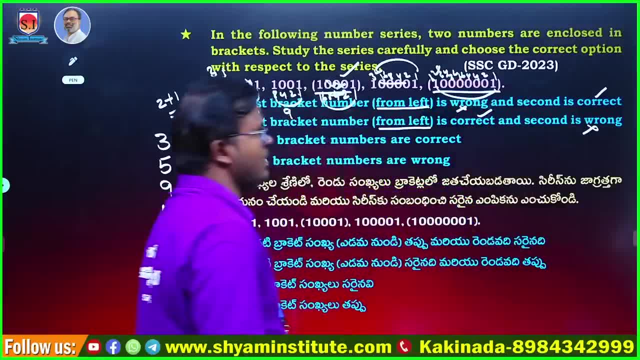 Next, 128.. Now what will happen if we add this? We will get 128.. Now what will happen if we add 128 plus 9? We will get 129.. Now, if we look at the series here, what will happen? 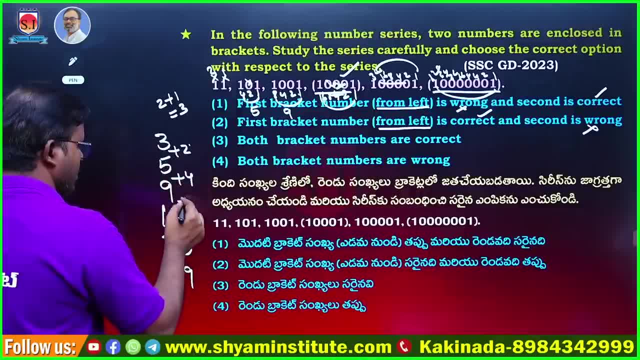 It will be plus 2.. What will happen if we add this? It will be plus 4.. Next, it will be plus 8.. Now what will you do with this? Tell me So. observe the difference 16.. 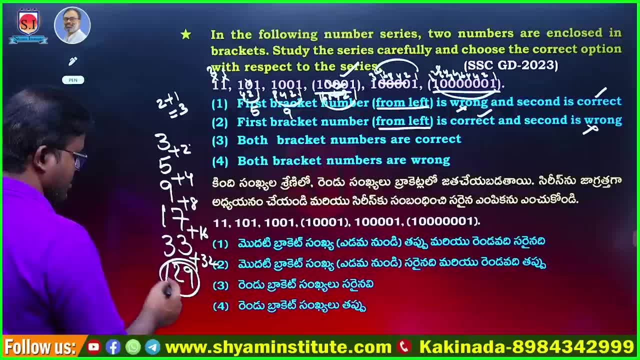 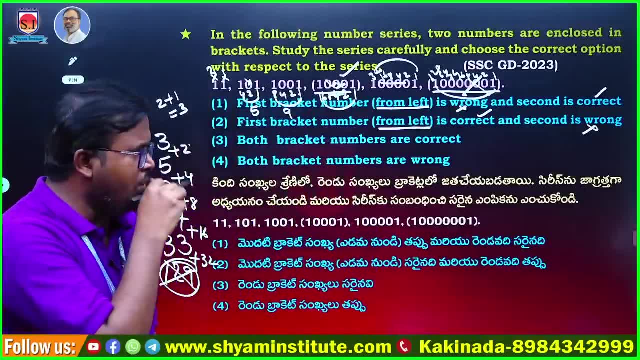 Now, what will you add here? You will add 32.. Now, will you get the answer here or not? You will not get the answer here. Now what will happen here? The number in the second bracket is wrong. So the number in the first bracket is correct, but the number in the second bracket is wrong. 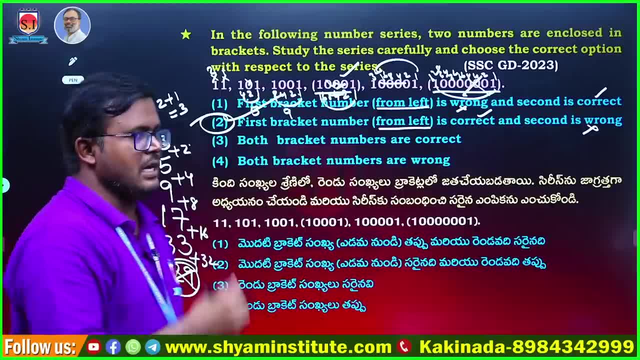 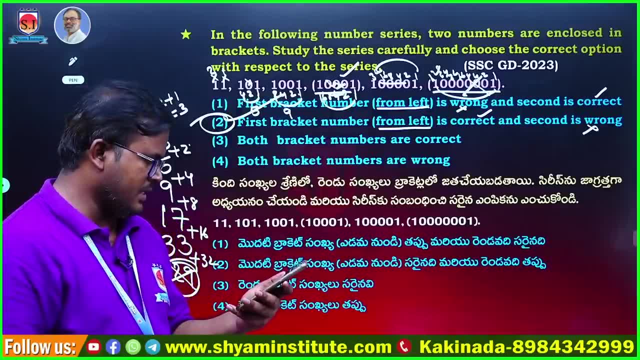 So the second option is the correct answer. So this is our. So the last time we had a problem in the exam In the number series we had to ask for the wrong number series. So Max and everyone else did the correct answer. 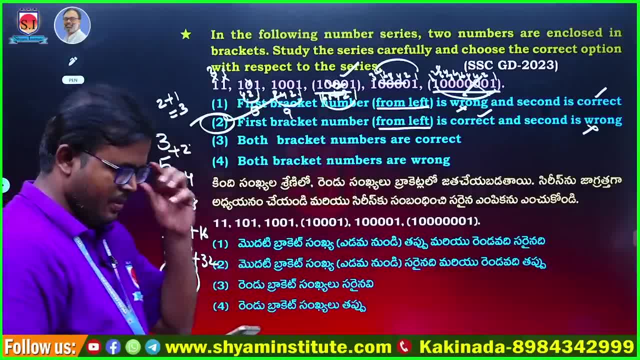 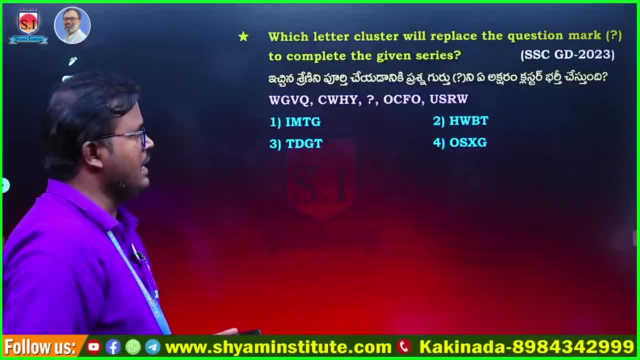 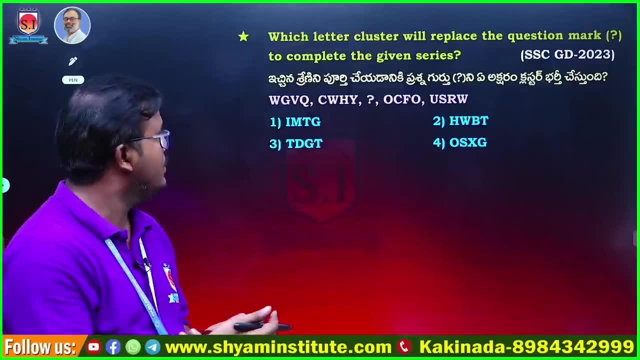 So look here, They also typed the correct answer. Okay, very good, They gave us the concept of binary digits, So we gave the letter series here. Now, what will be the answer to this? You have to type the answer. 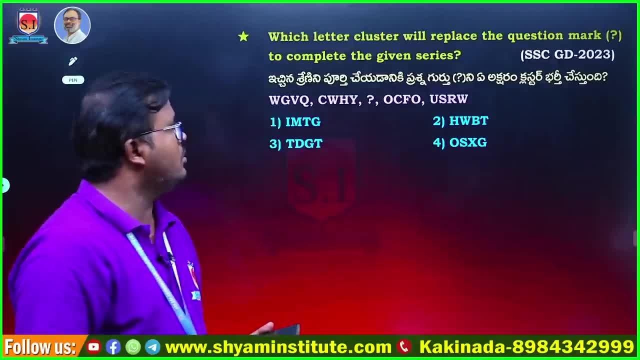 So which letter cluster will replace the question mark to complete the given series? He said, Now, in this series we have to get the answer. So which letter will get the answer? He said and asked: Let us call him. 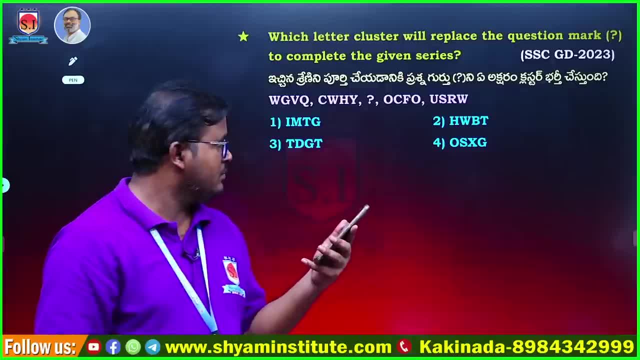 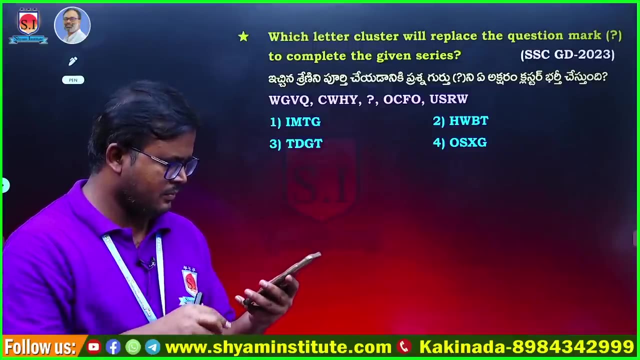 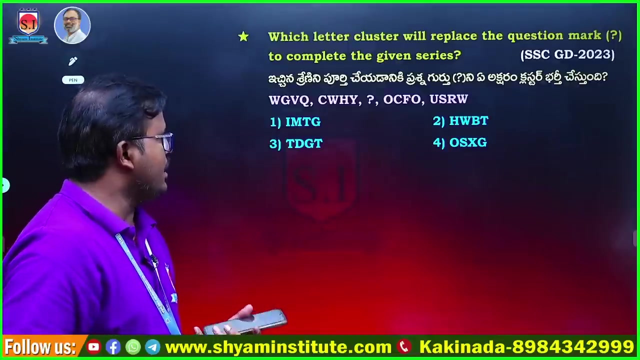 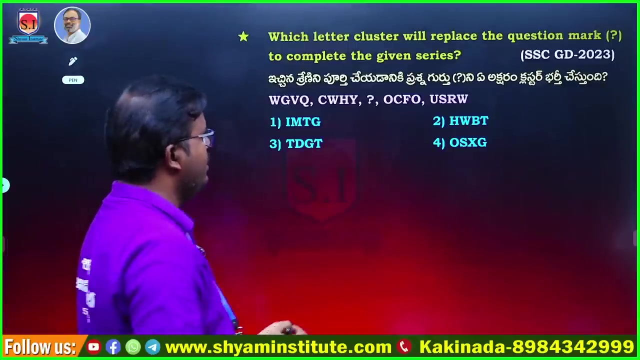 Second, Second, Four, Sai Krishna giving the second option. So which answer will get the correct answer? Share your comments. Remember that this is also a problem given to us in the last year. When we answer this, there is an option here. 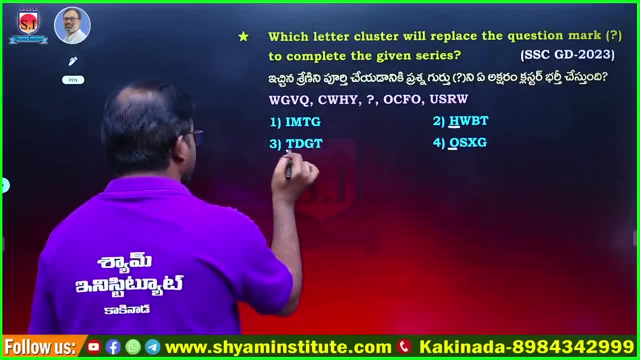 There is a letter O here, There is a letter H here, There is a letter T here, There is a letter I here. That is, even if we say one letter, it is not equal to us. If we do the first letter, the answer is over. 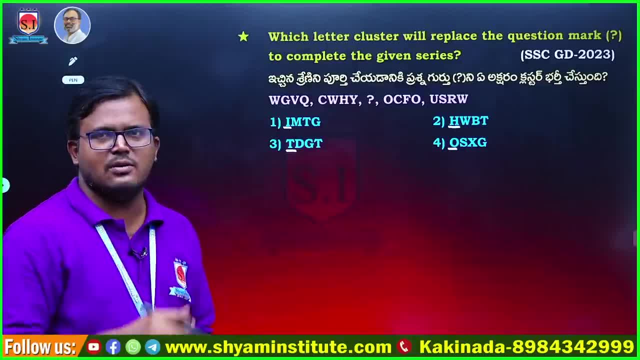 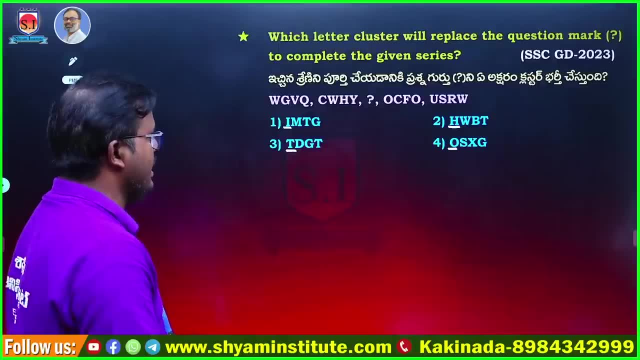 Then do it. What will happen to the first letter? There is no need for anything else. If we do the first letter, the answer is over. If we want to do the first letter, what should we do? Letters and numbers should come. 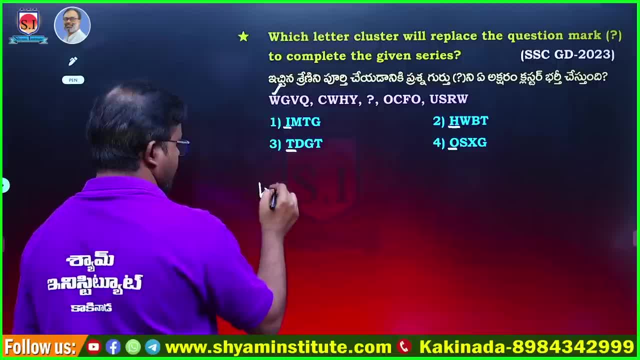 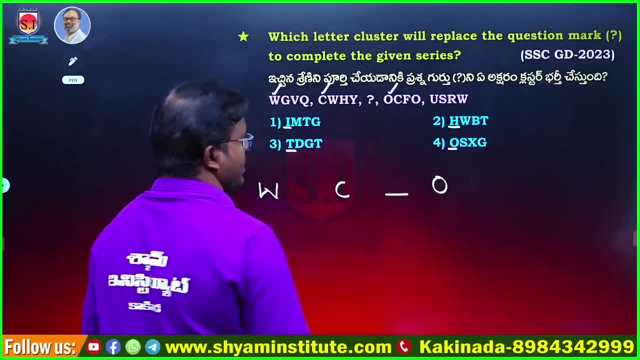 What is the first letter here? There is a letter W here. What is the first letter here? There is a letter C here. There is a letter O here. Since we do not know what this letter is in the middle, take the letter O here. 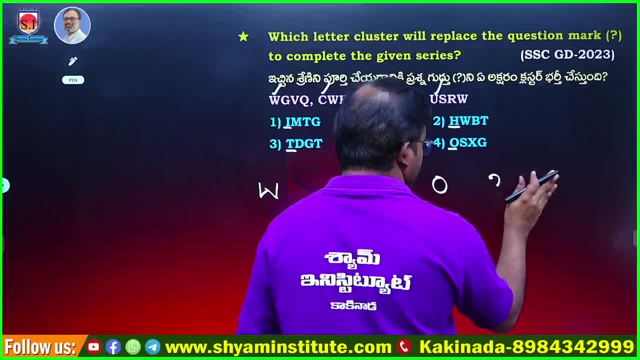 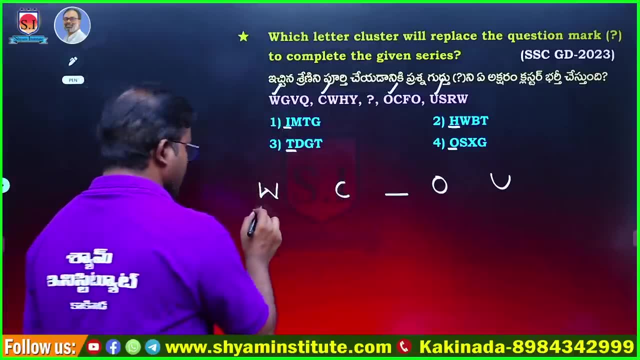 What is the last letter here When we come here? there is a letter U here, Then there is a letter U here. What will you do now? Write a number after the letter C. What is the number? W means 23.. 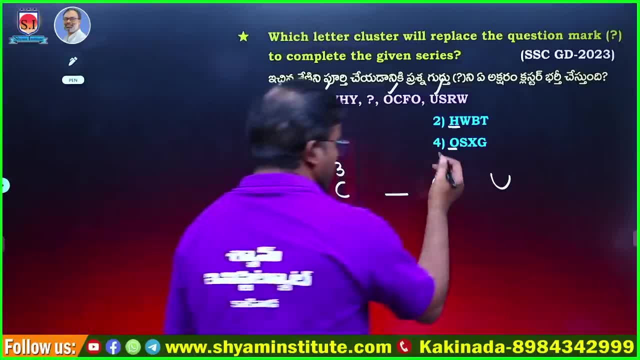 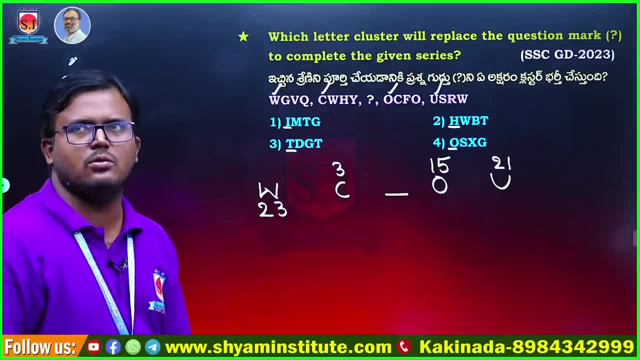 C means 3.. O means 15.. U means 1.. Then there is a number called 21. here. There is a point that you have to observe here. What is that? When you take the numbers A, B, C here?